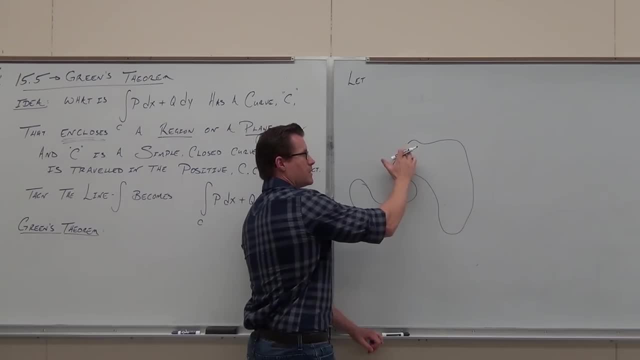 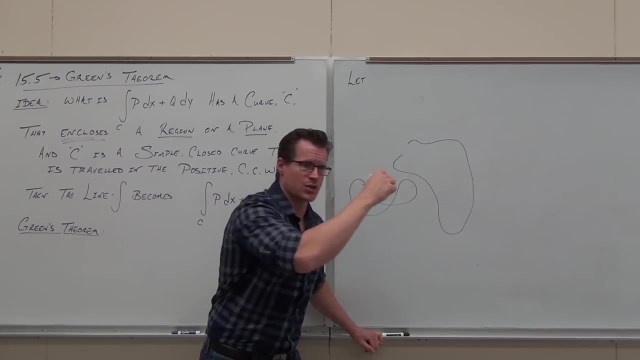 That would be a simple closed curve. This would not be a closed curve. Do you see the difference? Your starting spot and your ending spot have to be the same and you're not crossing yourself. That means that you're a simple closed curve and you're okay with that one. 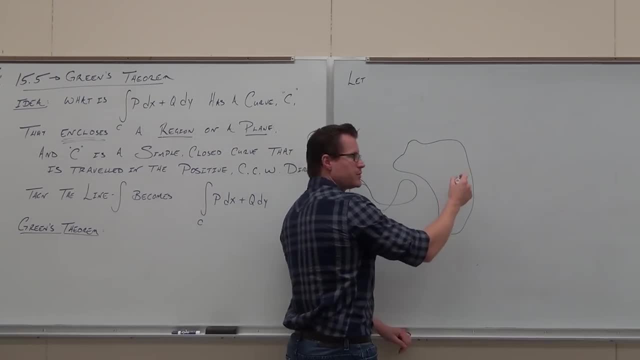 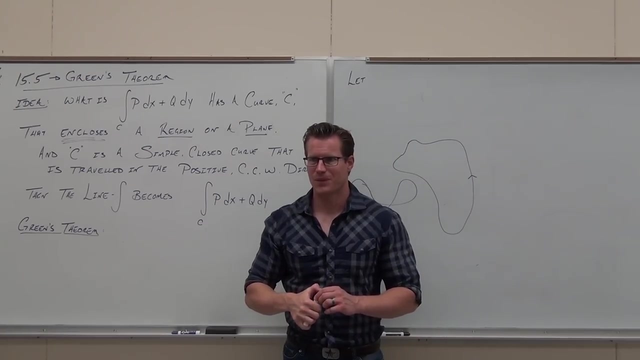 Furthermore, let's assume that this curve is traveled in the positive counterclockwise direction. So we start someplace and go counterclockwise, and that's what that means- counterclockwise direction. So what are we dealing with? 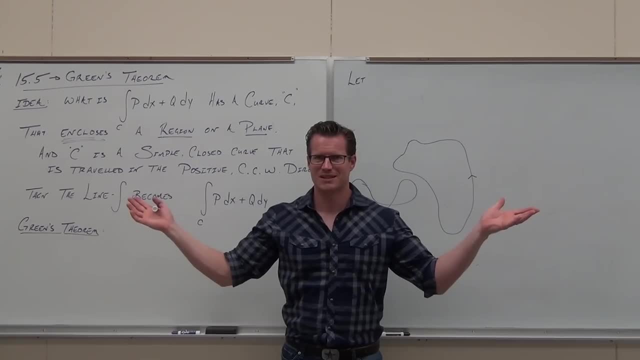 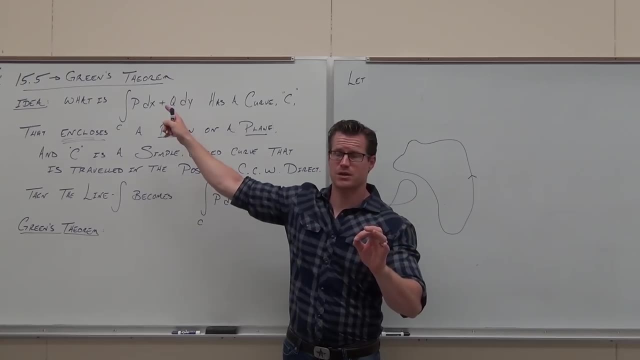 Are we dealing with vector fields? still Well, we're going to find out. Are we dealing with work? We're going to find out. Are we dealing with line integrals? Certainly yes, But line integrals where we have a specific type of curve. 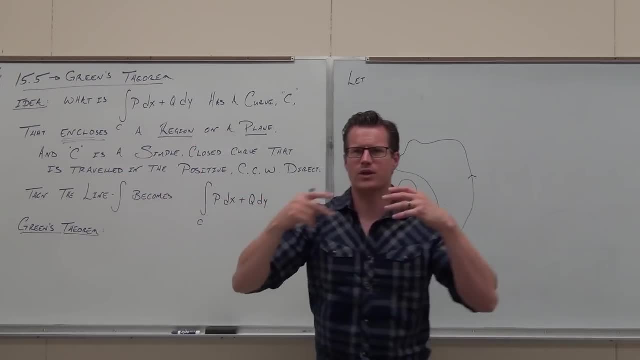 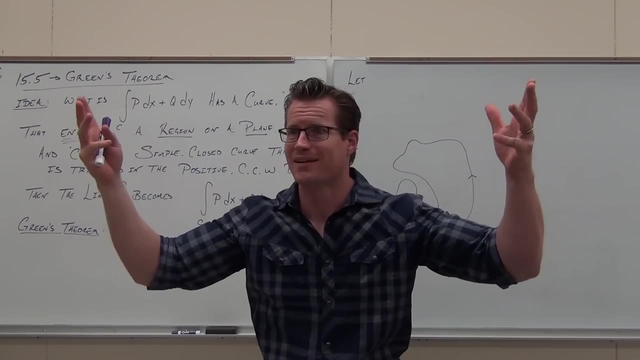 What type of curve are we dealing with in this section with Green's theorem? What's Green's theorem going to have to do with Curves that do what? Oh goodness, This is supposed to be like you got it. Do you understand what C does? 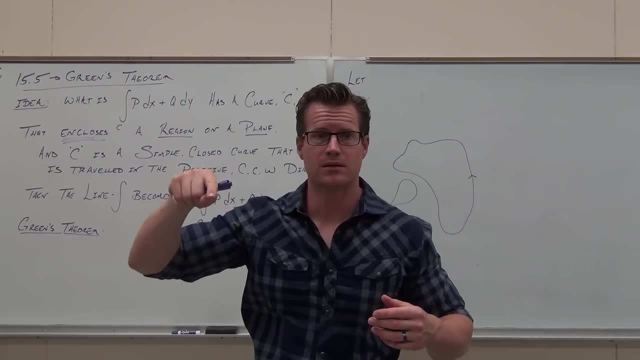 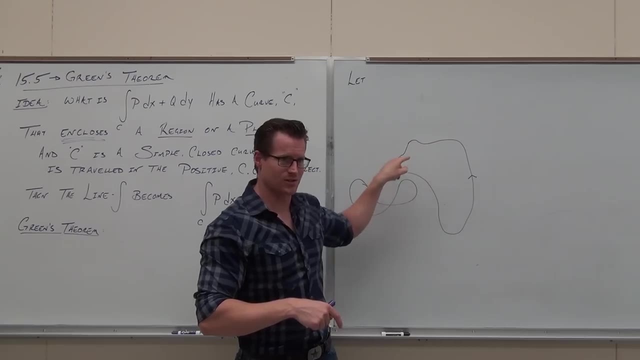 What's C do? It closes a region on a plane. It closes a region on a plane. This is going to come into play here. It closes a region in a plane. It doesn't cross itself. It doesn't close two regions like this does. 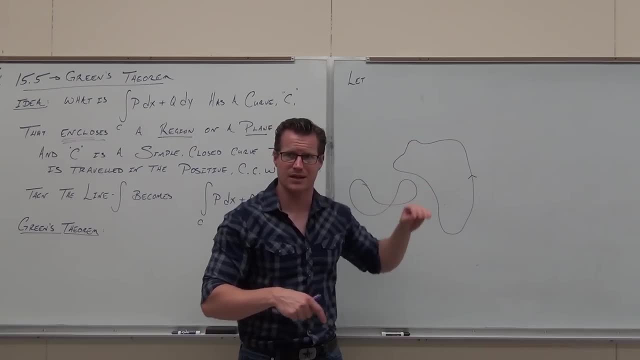 It closes one region on a plane, It starts and stops at the same spot, and it's traveling in the positive, counterclockwise direction. So it means you understand the premise for Green's theorem. Now do you understand Green's theorem yet? 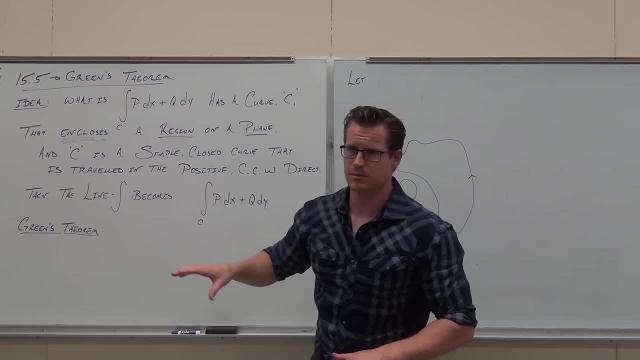 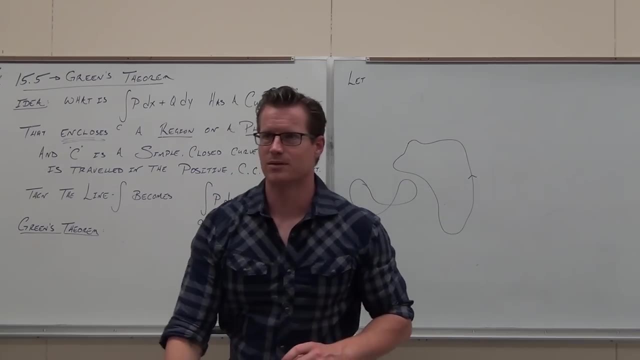 No, but I'm about to show you. So here's what Green's theorem is. It's invented by the incredible Volcker's theorem. It's called the Green's theorem, I'm pretty sure. So that was a joke, Or Bruce Banner? 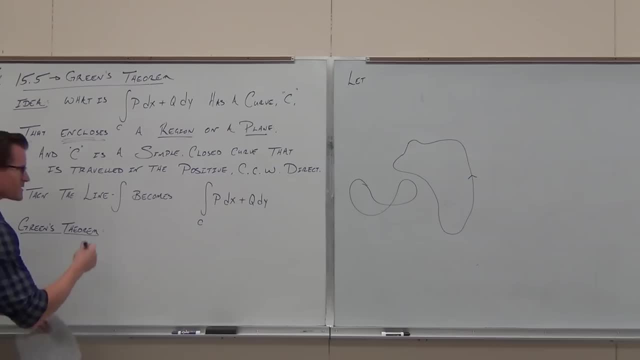 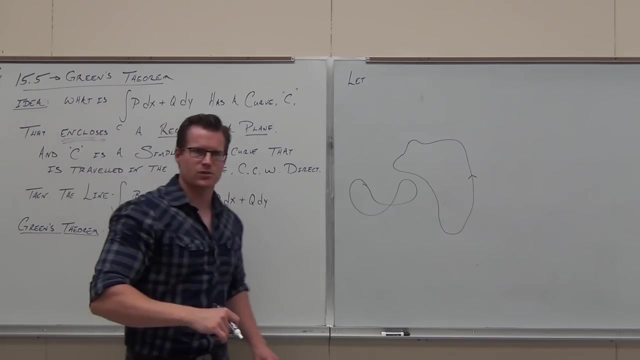 He's pretty smart. So Green's theorem says: well, what happens if our line integral has a simple closed curve? Then really this C is very specific And we draw a circle right there saying that that's a line integral where the C is a specific type of curve. 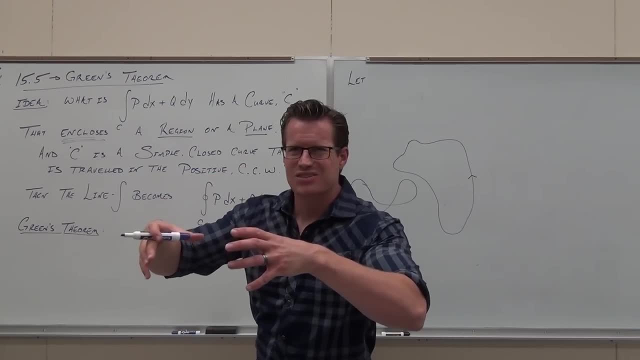 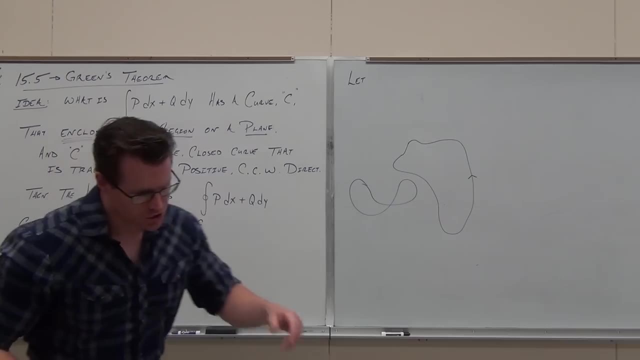 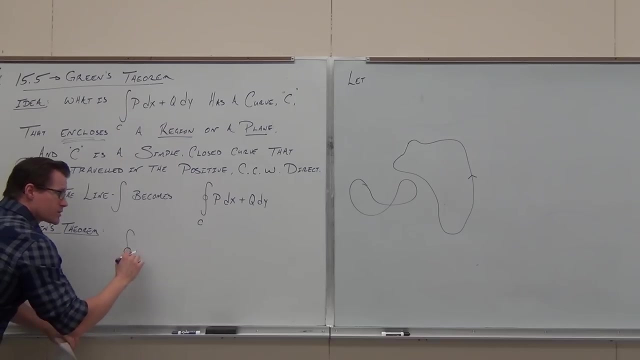 A simple closed curve. that's Containing this region. Containing this region has traveled around the region in a positive, counterclockwise direction. So here's what Green's theorem says. Green's theorem says that this line integral over a simple closed curve. 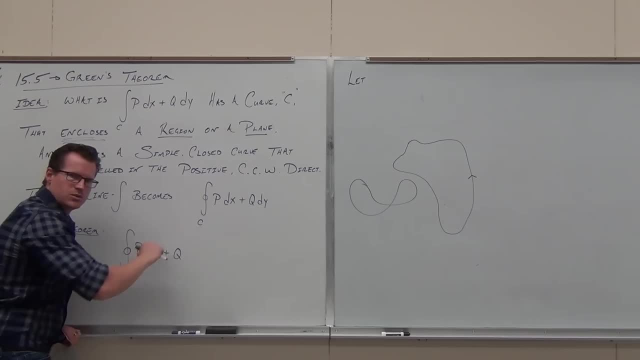 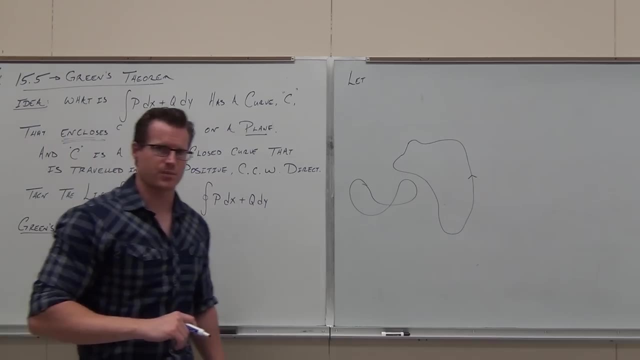 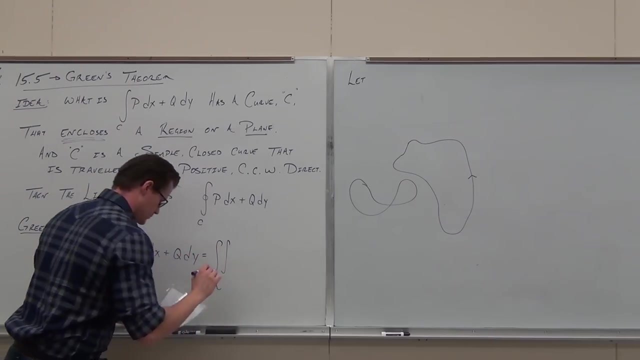 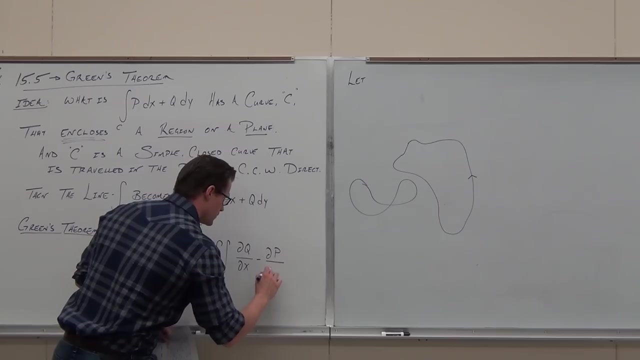 By the way, do you remember that format? having this Pdx plus Qdy- We're about to see where that came from- Equals this. It's going to look a little strange to you until you wrap your head around it. We're going to put our paper back. 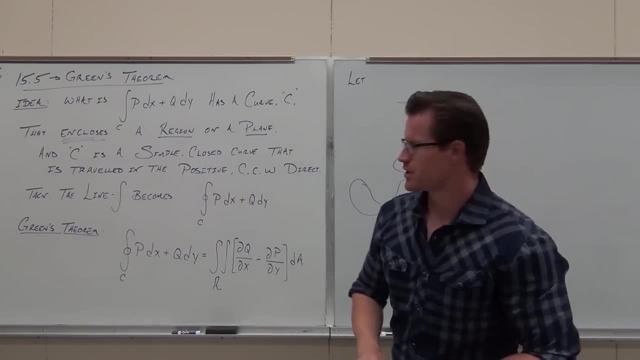 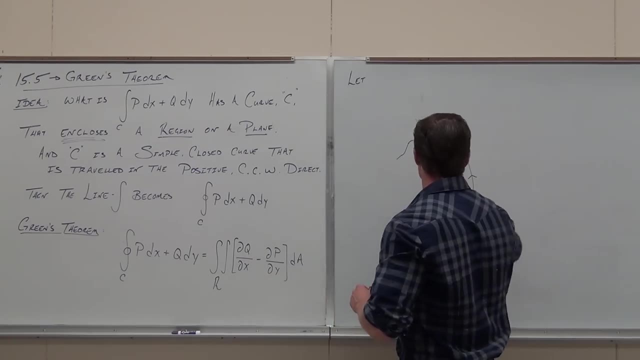 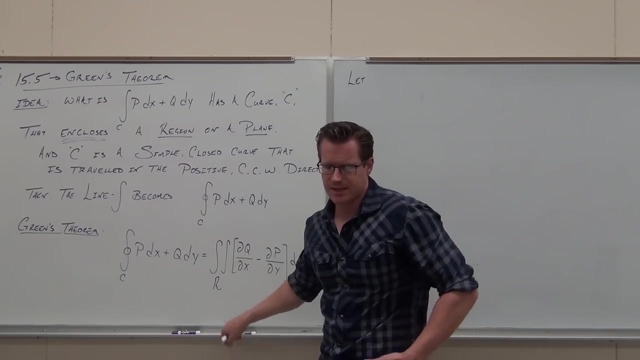 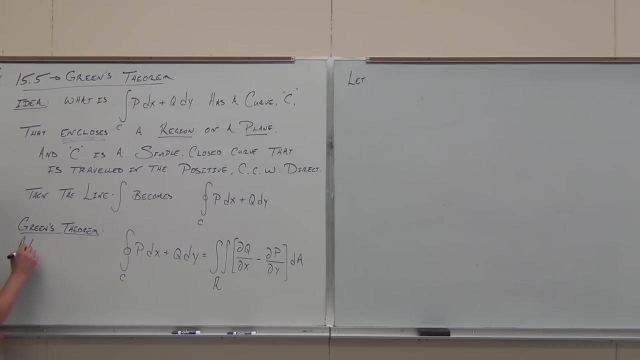 That, ladies and gentlemen, is Green's theorem. Thank you, Thank you What it states? it states this: it states that a line integral for a simple closed curve is equal to well, let's look at it. let's look at it. 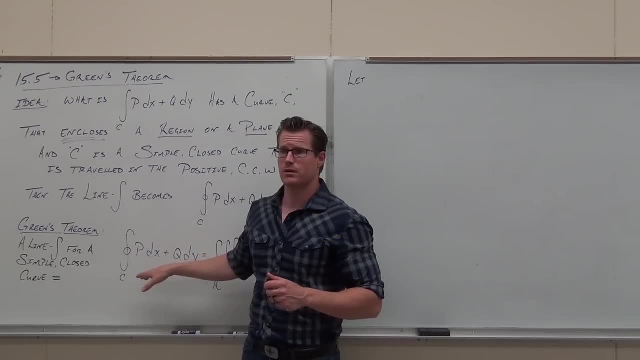 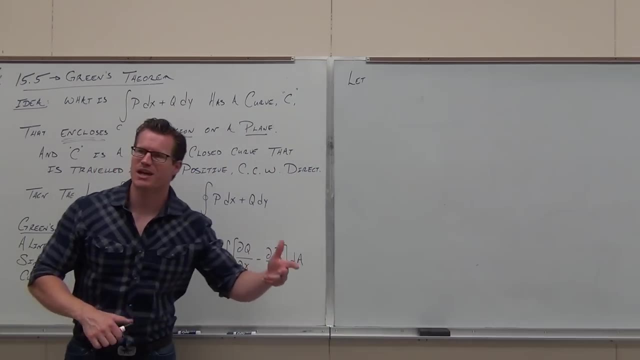 Check out the notation. Firstly, can you recognize line integral here? Simple, closed curve. that's what this says. See the little arrow going positive, counterclockwise direction. Well, let's look at what Green's theorem says. I'm not going to prove Green's theorem. 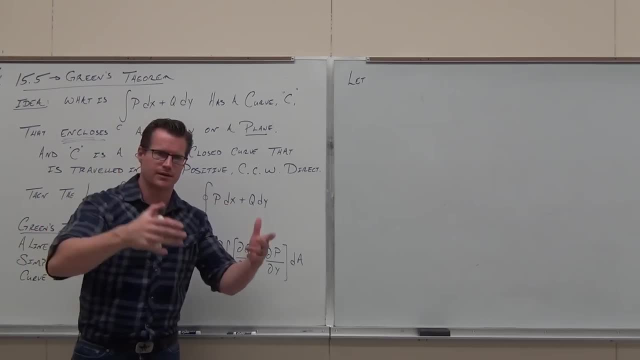 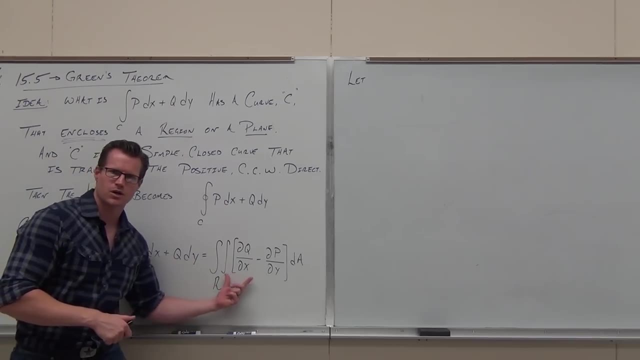 It's kind of beyond our time limit, firstly, and the necessity to do in this class. But let's look at what this, the Green's theorem, says: a line integral over a simple closed curve is equal to: oh my gosh, what is? 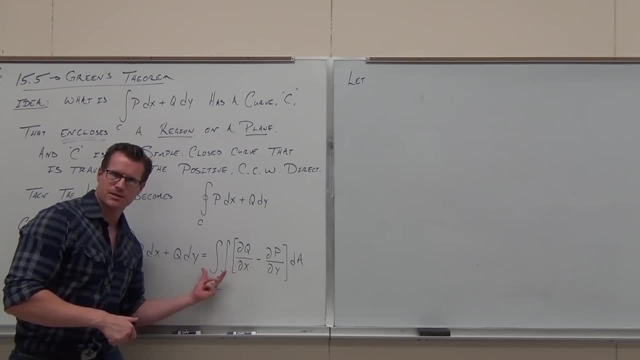 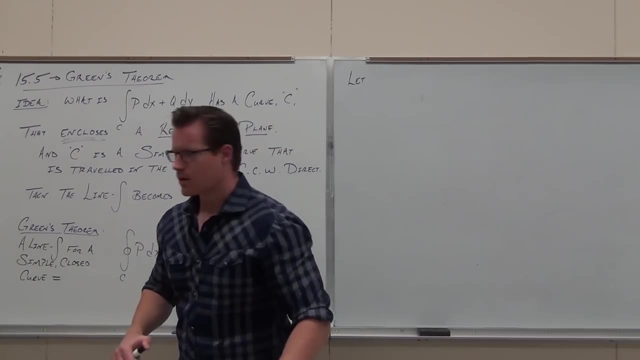 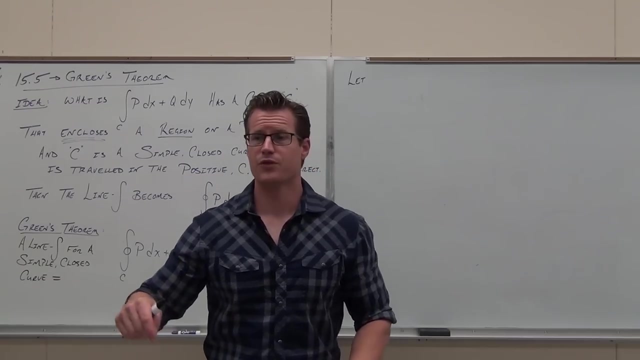 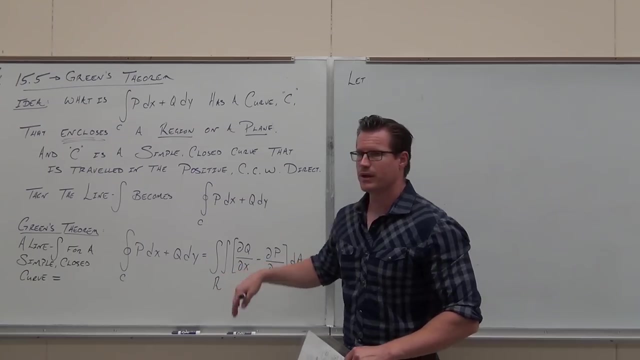 What is this? That's a double integral over a region. It says that the line integral for a simple closed curve equals the double integral over the region that that curve contains. That's what that says. Now, why is that important? Because double integrals are really easy. 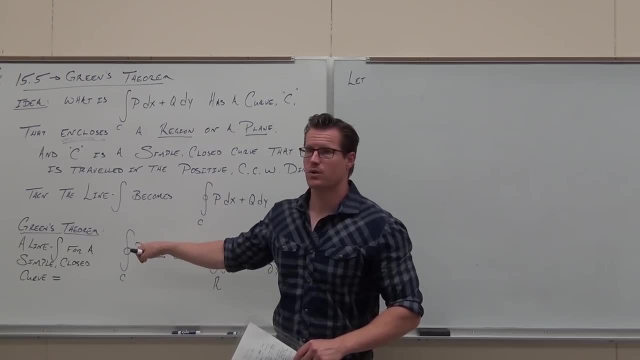 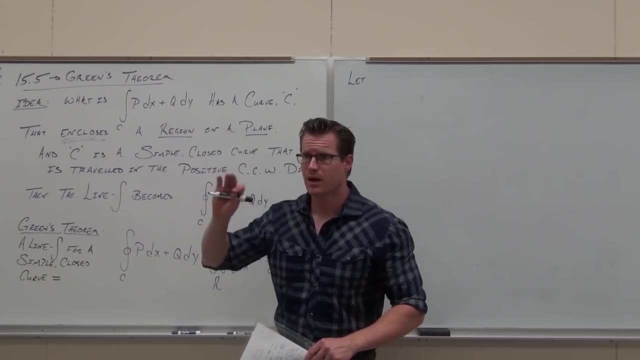 and they're really nice to deal with. And line integrals can be a real pain. When they were conservative they were kind of nice. When they were non-conservative they were a real pain. We had to have a vector function for each different curve. 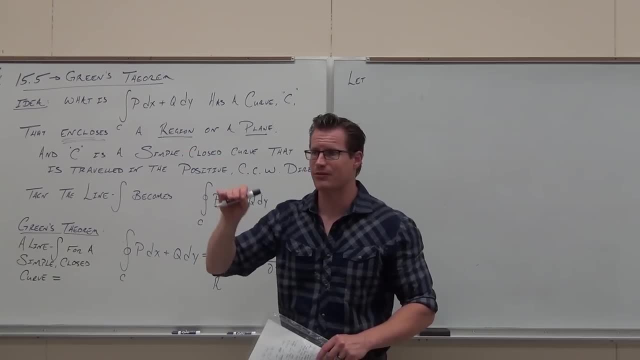 and then add up the different integrals and re-parameterize it and we didn't have a curve. then we were in serious hurt. Does that make sense? That was a problem. We're going to deal with some of those issues right now. 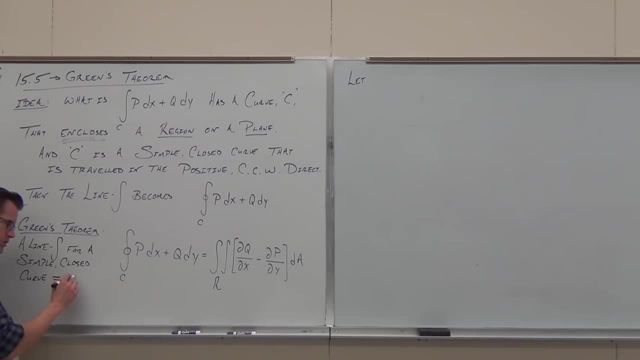 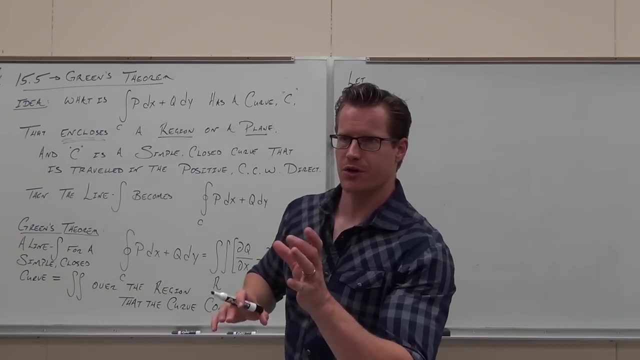 So Green's theorem: blah, blah, blah, blah. line integral for a simple closed curve is equal to a double integral over the region that the curve contains. Now let's use some critical thinking here. Think about this. Why does the curve have to be closed? 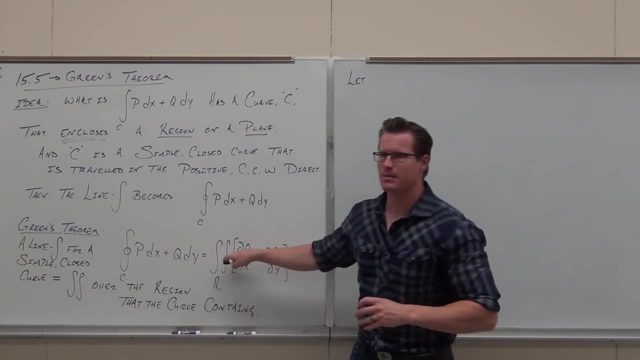 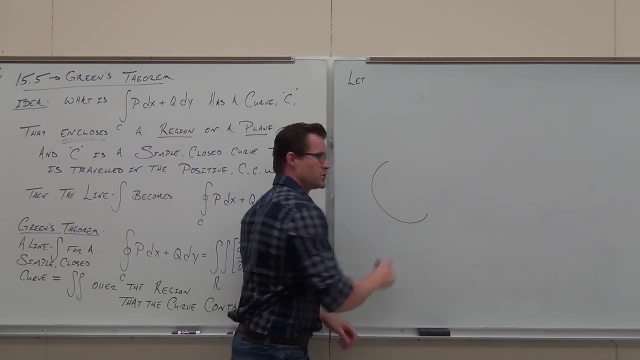 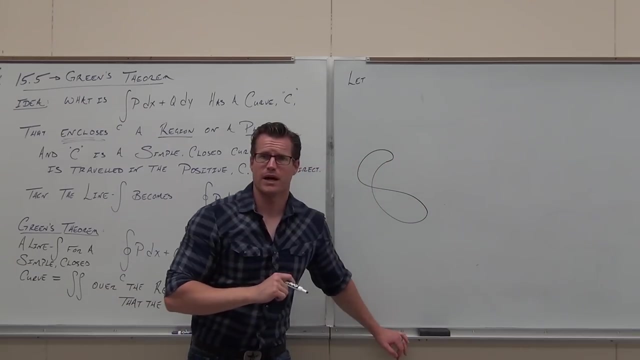 Why does the curve have to be closed for Green's theorem to work, keeping in mind it's a double integral? Why, If I don't have a closed curve, do I have a region? If I start crossing this, how many regions do I have? 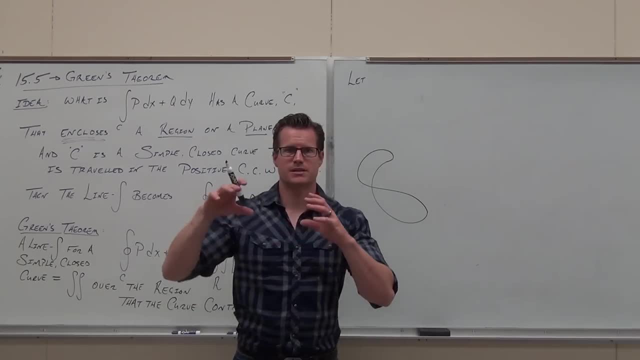 That's a problem. So with Green's theorem you get a simple closed curve, because if you don't have a closed curve, you don't have a region. If you don't have a region, a double integral doesn't make any sense at all. 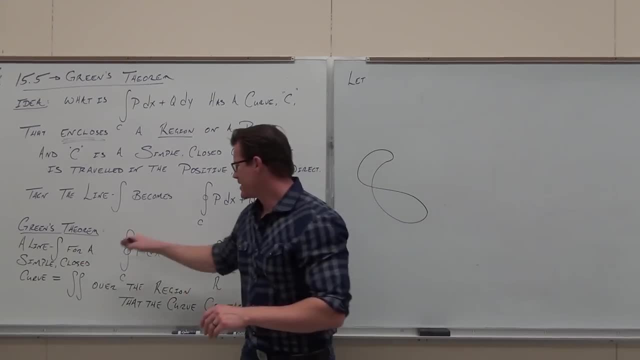 You have to have this. This is all Green's theorem says. It says: hey, if you've got a line integral over a simple closed curve, it equals a double integral over the region that that simple closed curve contains. That's it. 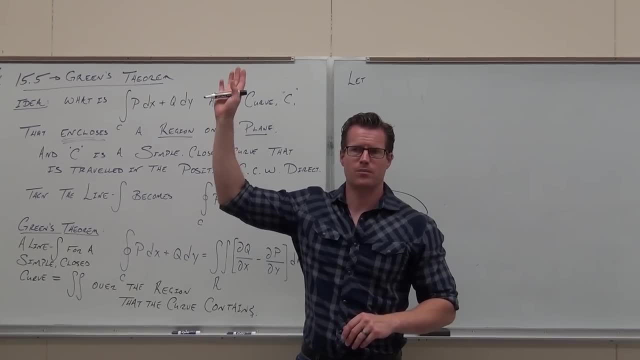 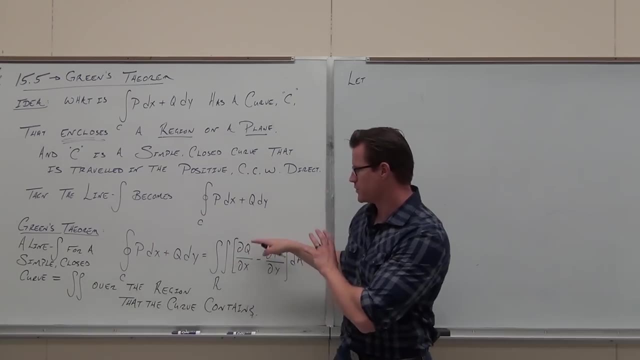 That's literally all it says. Show of hands if you feel okay with that Now. now, what is all this junk and where is it coming from? This is Green's theorem and I'm not going to prove that, but I'm going to show you where this stuff comes from. 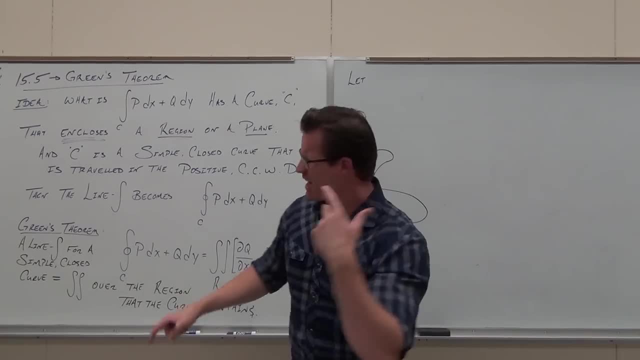 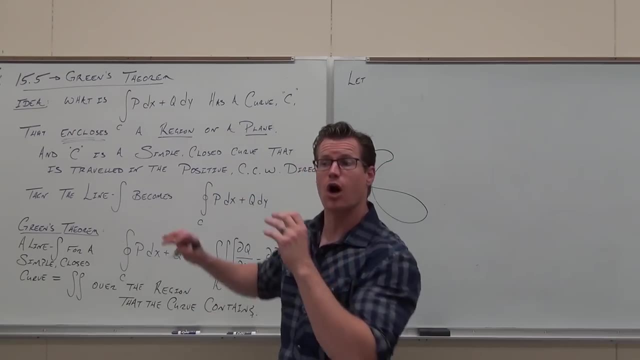 because we've seen it before and I said this. I said just kind of think about this as ds being split up by the nature of that derivative, but we're going to. I only said that because we hadn't talked about this yet. 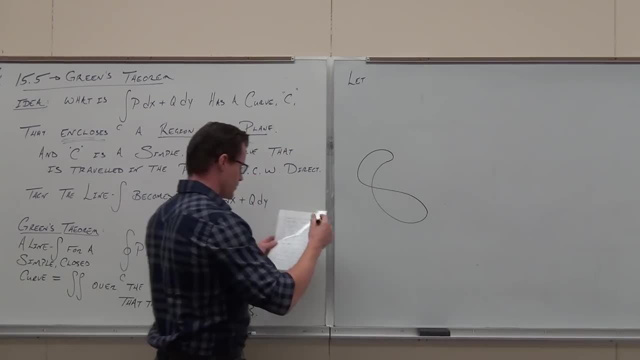 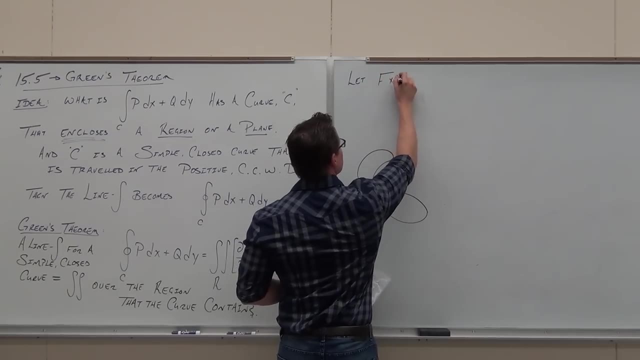 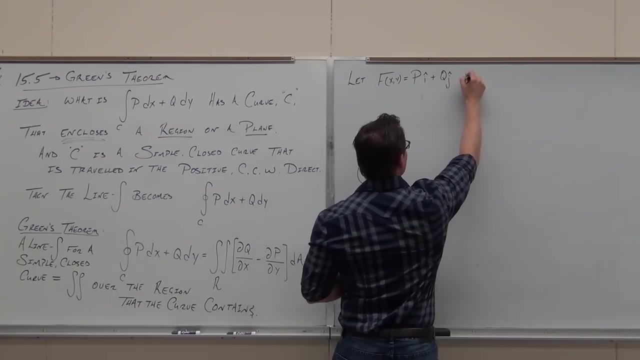 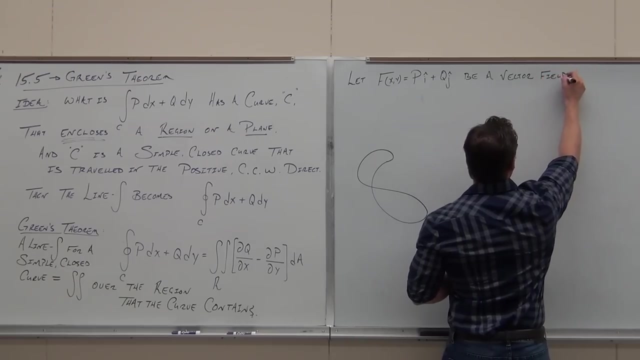 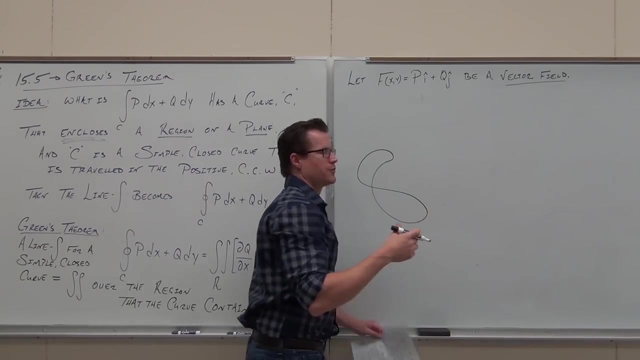 I'm going to show you. I'm going to show you where it comes from. So, let's, let's find out where this comes from. Let's, let, let's, let a vector field be defined. And, furthermore, if, if we have a vector field like that, 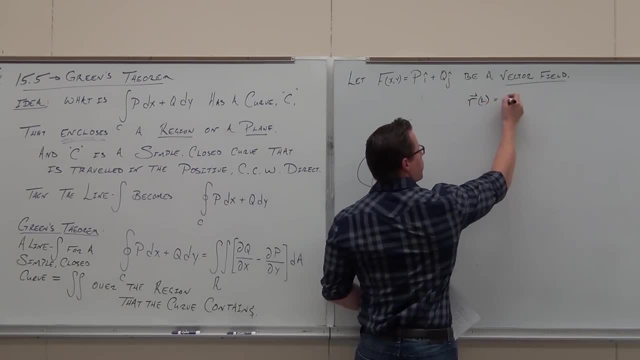 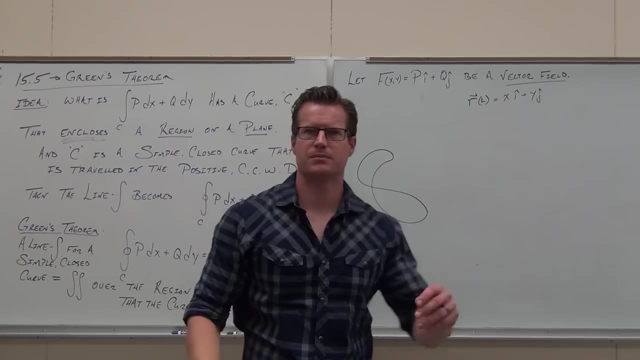 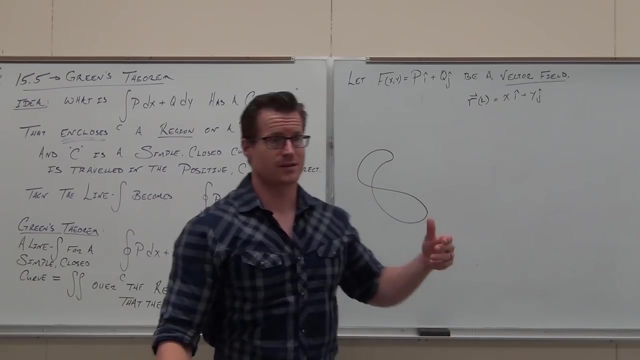 let's define a curve. Remember doing that, This note, Remember having vector fields Moving back to to a while back vector fields and we had these curves through the vector field and that was like two sections ago. and then we said: 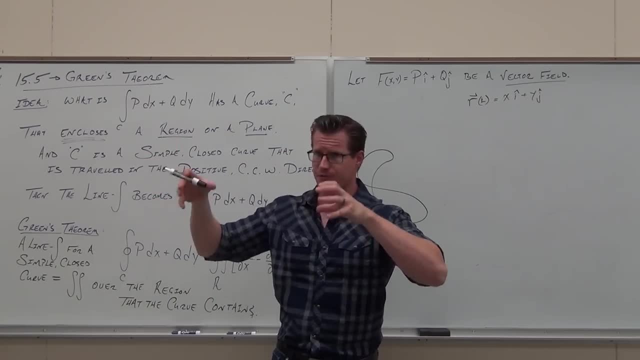 what about conservative? Oh, we don't need a curve, But before that we had to have a vector field, We had to have a curve. I didn't know that. you understand that We had to have both. That's our vector field. 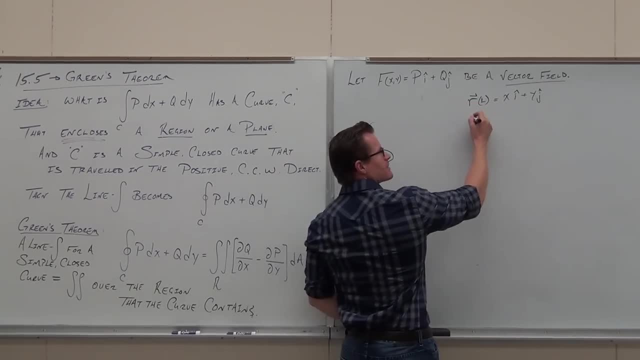 That's our curve. And then we said, well, well, wait a second. We we did a lot of stuff with dr, And dr was well happened to be the partial derivative of this with respect to x and the partial derivative of this. 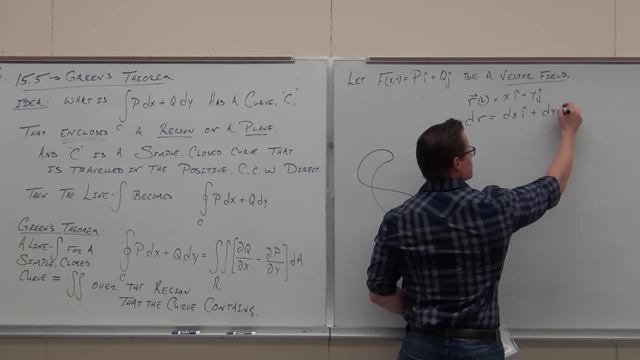 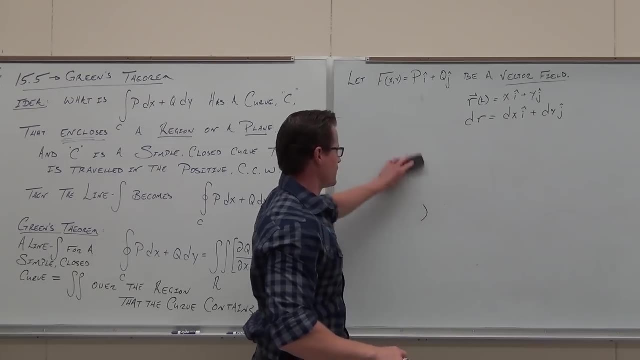 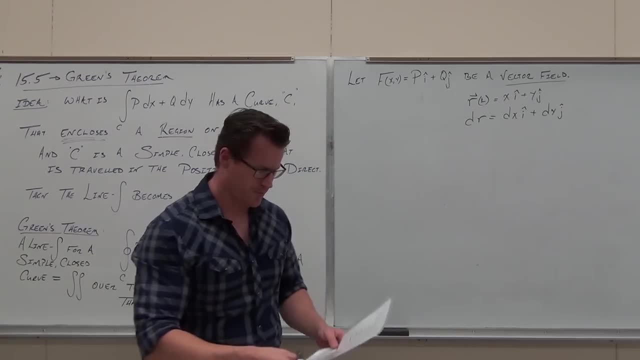 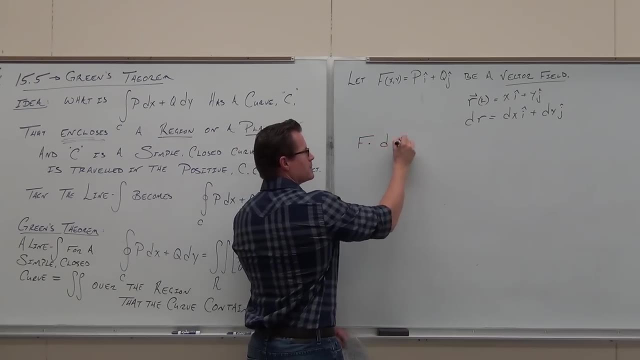 we're going to use a different notation for the partial derivatives, but that's where we got that from, And so well, wait a second. What would happen if, if I took f dot dr? if I did that? Well, if I take f dot dr, then that's pi plus qj. 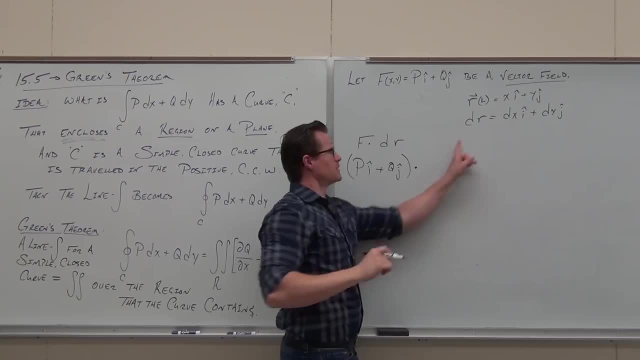 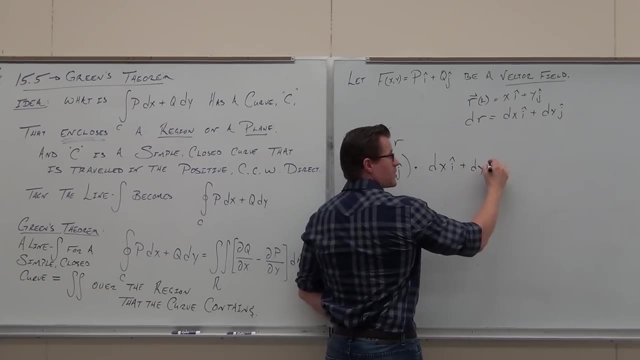 That's, that's our vector field, dotted with this thing that I just got the dr. Hey, firstly, is a dot product going to work here? Explain why or why not. Is a dot product going to work? Yes, Why? 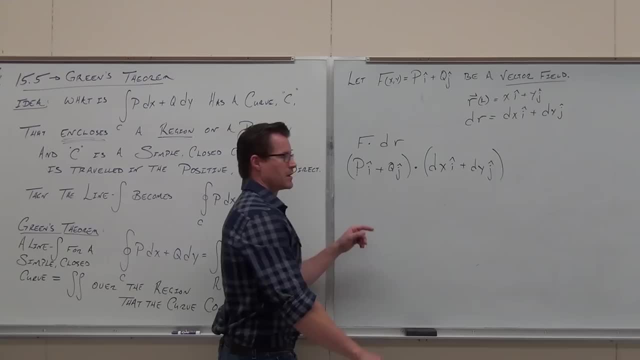 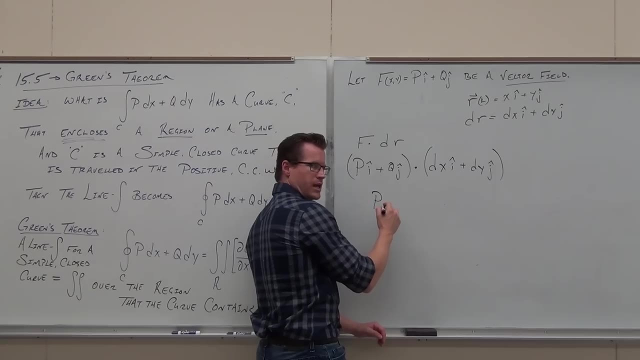 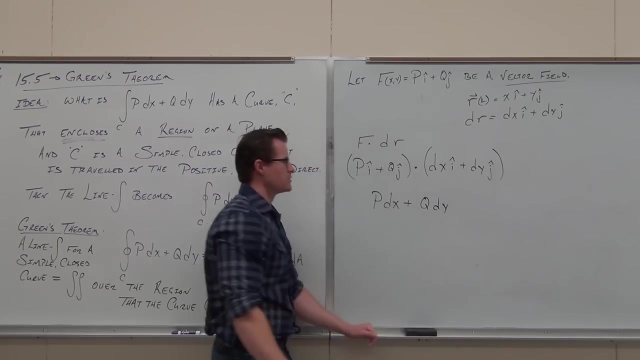 Because it's a vector, Both vectors. If I do the dot product, then we end up getting. well, you can see it. component- no, i's no j's. Component- no, i's no, j's. Here's what we just got out of this. 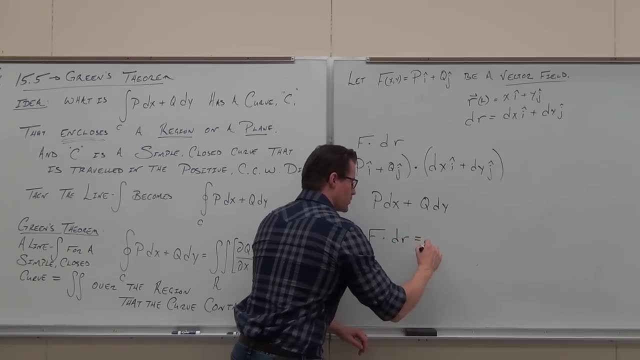 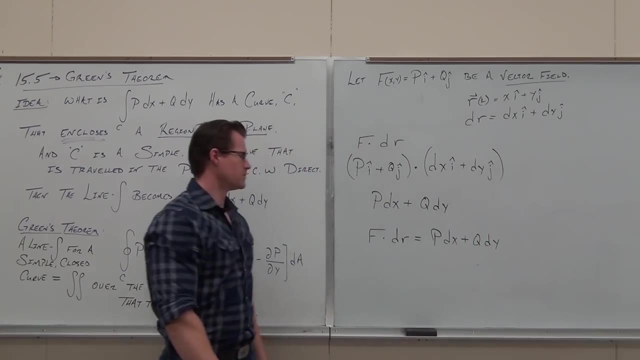 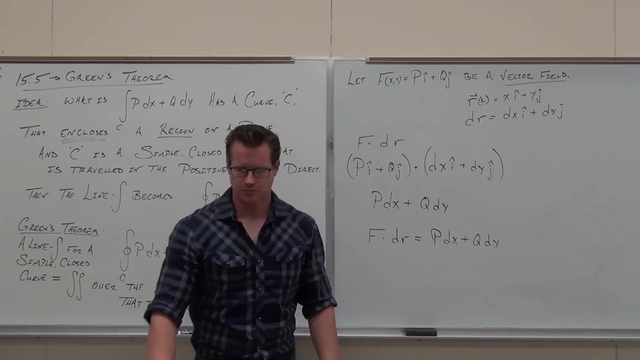 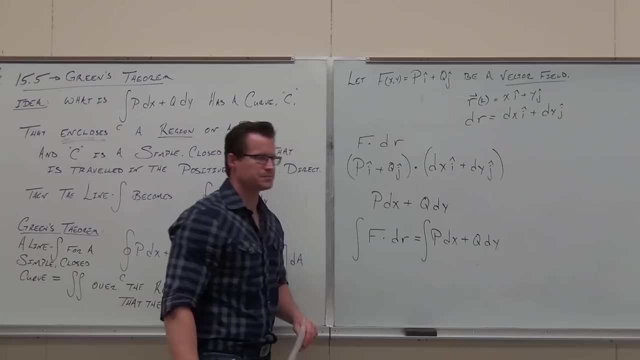 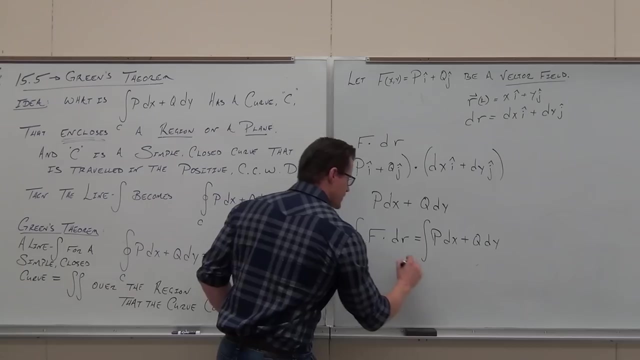 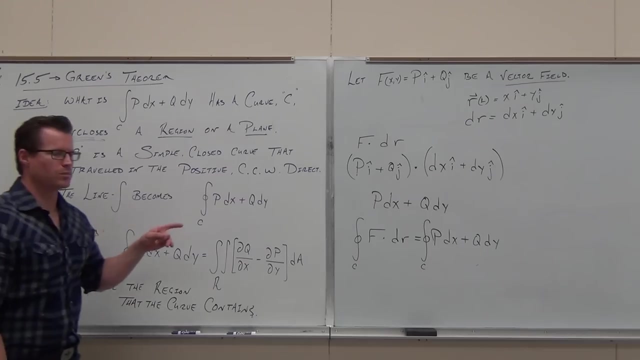 We got the f? dot. dr equals This right. there is okay on where that that came from. Now let's integrate both sides. Let's talk about that Furthermore. let's integrate across a simple closed curve, But wait a second, wait a second. 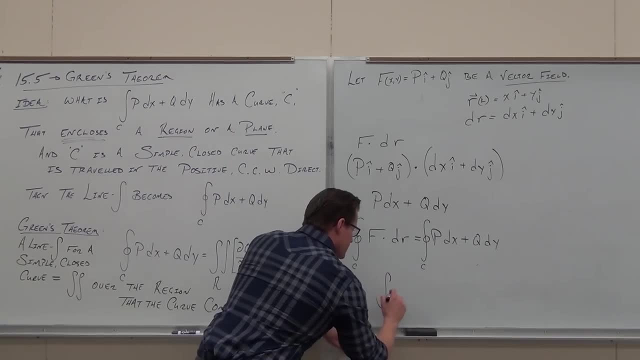 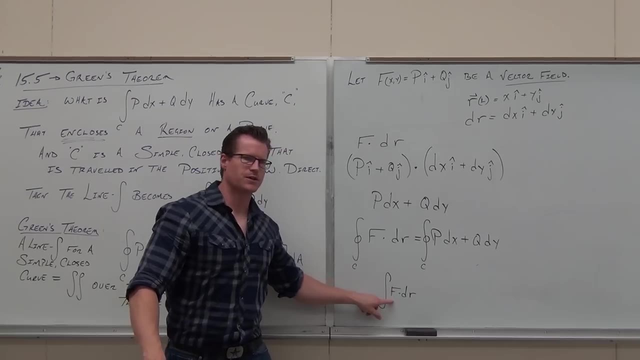 Wasn't, wasn't this? hey, do you remember what that was? Do you remember what that represented? Do you remember what we did when we had a vector field dot dr over a curve? What did it mean? Work, This was work. 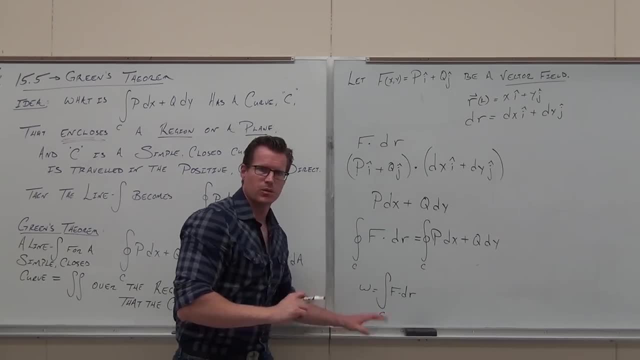 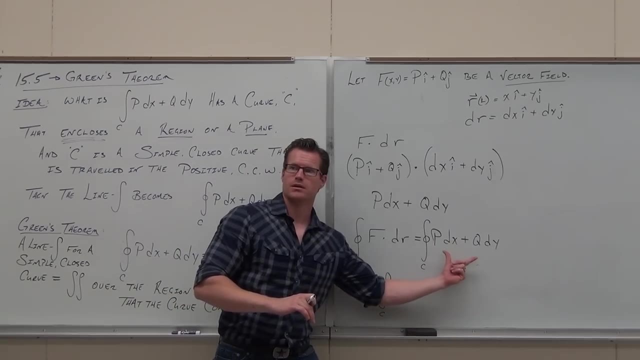 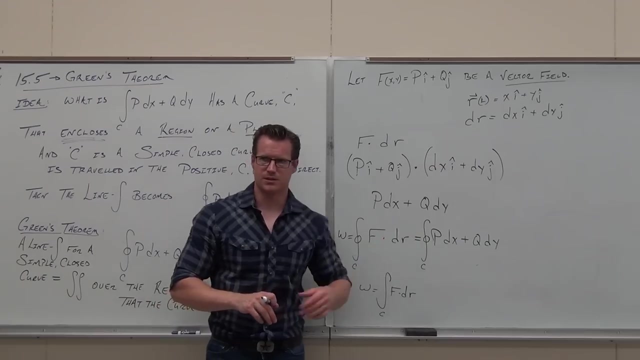 But, but wait, wait, If this is work, look at this. Is this also work? Is this also work? Yes, Yes, It's just a specific type of work. What this means every single time. you see it. this right here, this is work. 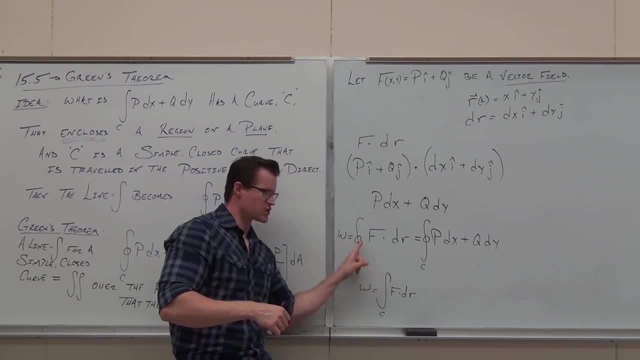 This is the same exact thing that we had for work. It's just our curve is specific. Our curve here is a simple closed curve that bounds a region. That's, that's what that means. Well, if that's work and I have them equal, then this is also work. 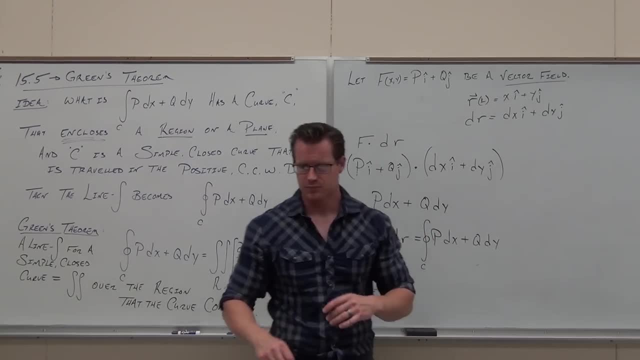 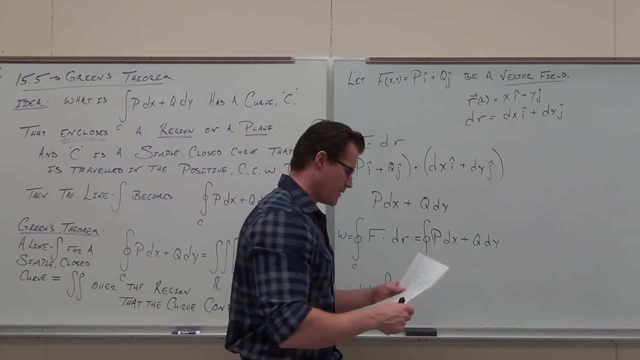 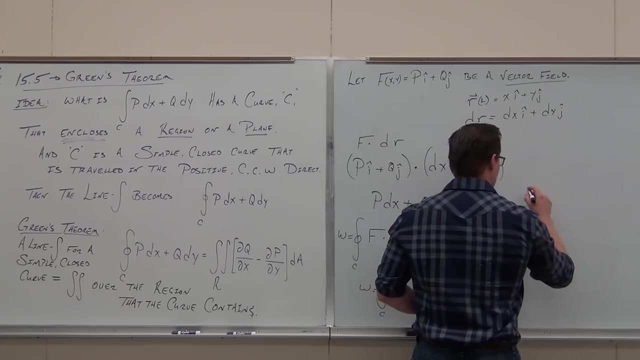 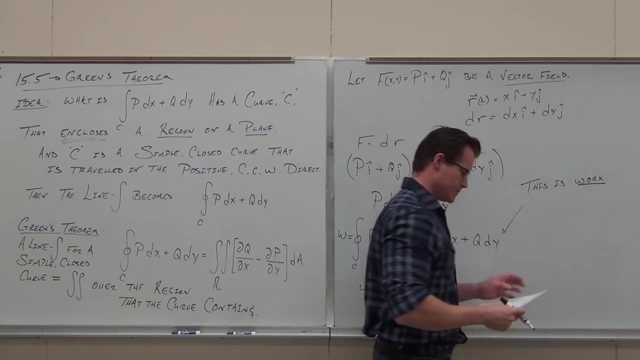 This is work. This is work done. This is work done over a simple closed curve through a vector field. That's what that means. Does that make sense? So every time you see that, that's what that means. So this is work done. along C, Some curve. 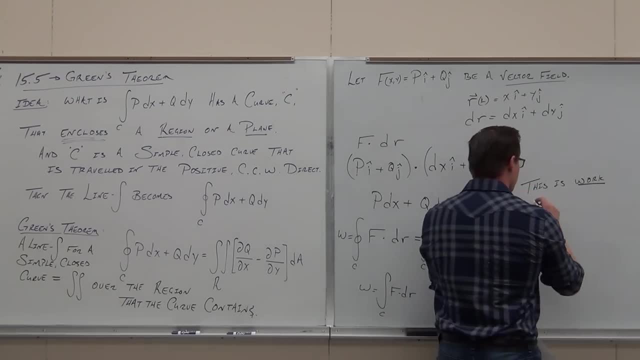 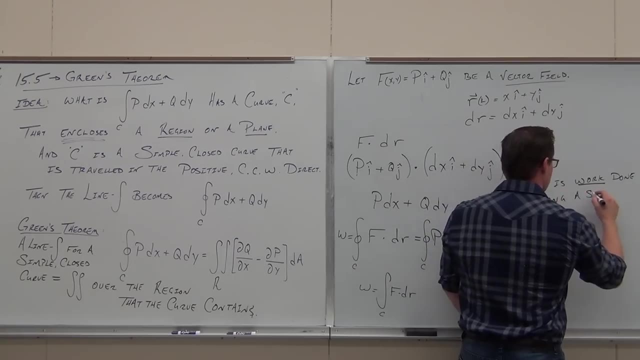 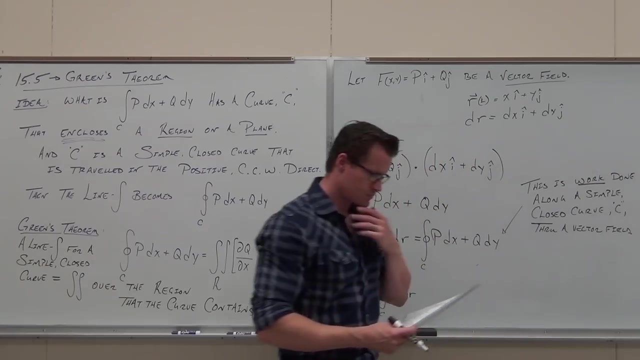 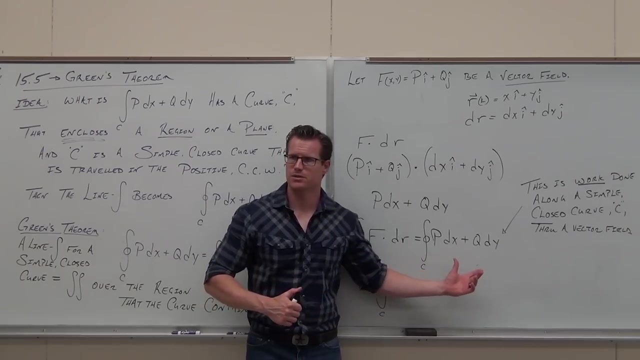 C, Some simple closed curve C Through a vector field. By the way, and this is where I can make the statement, This is where all that stuff. if you think back to two sections, we had ds and then all of a sudden I changed it. 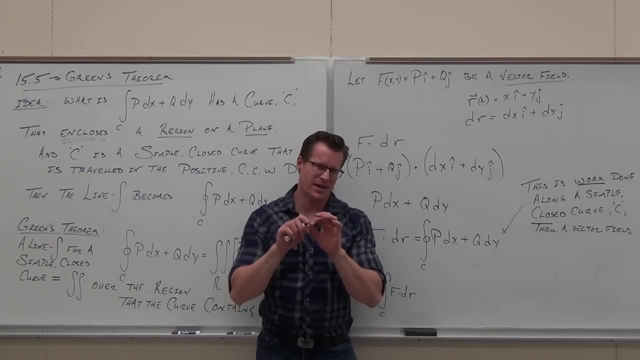 I said: oh, now we have dx and dy. And I said: just kind of think about it, as your ds is in two spots and you're kind of breaking up, that derivative sort of The dt is kind of broke up. 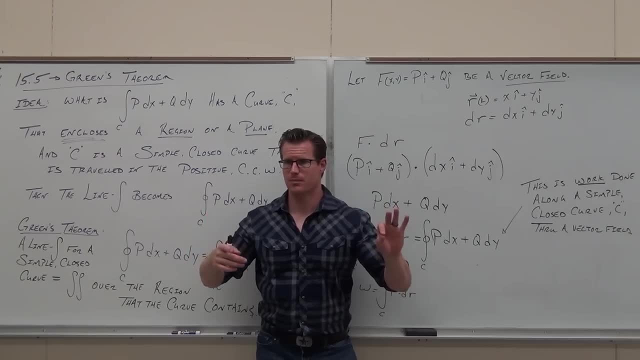 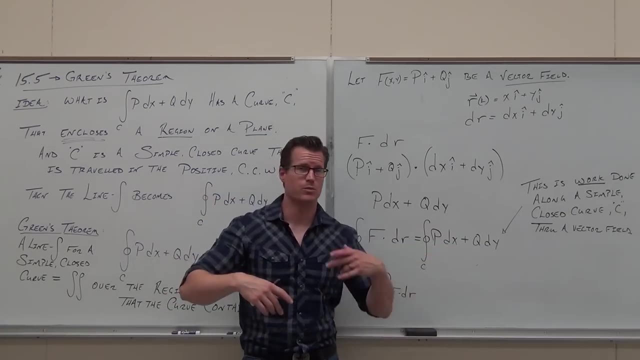 I did it so you wrap your head around it. What it's really coming from is this idea. So every time we saw that two sections ago, when we first started talking about line integrals and then we put them through vector fields, we hadn't talked about putting them through vector fields before we got some of this. 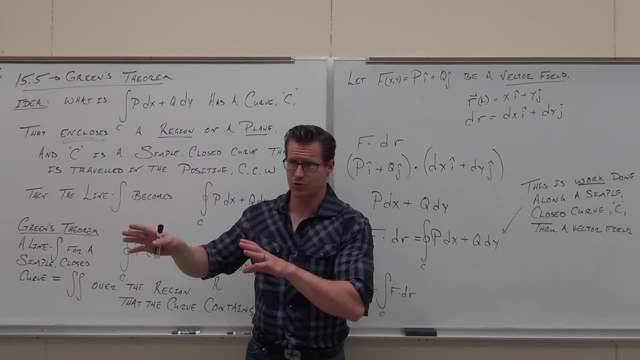 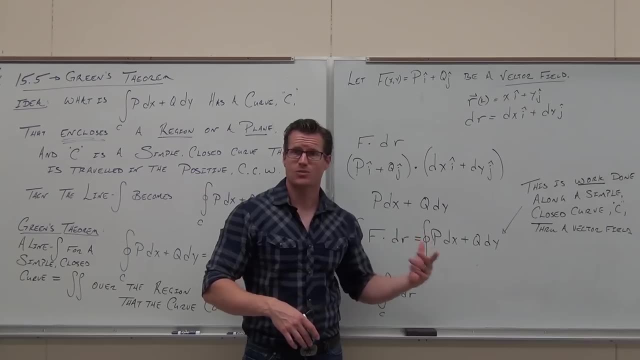 This is where that came from. So every time we did the line integral from before and we had the pdx plus qdy. Do you guys remember that stuff from a while back? We've already seen it. That represented a vector field already. 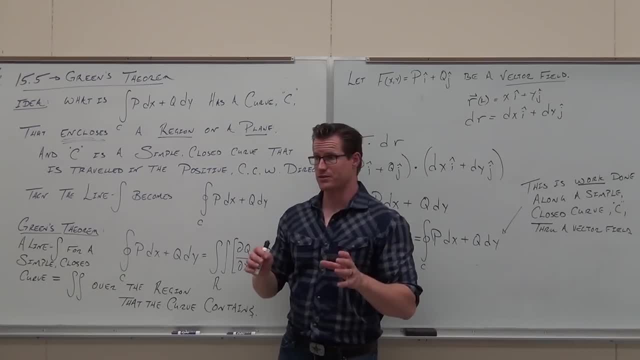 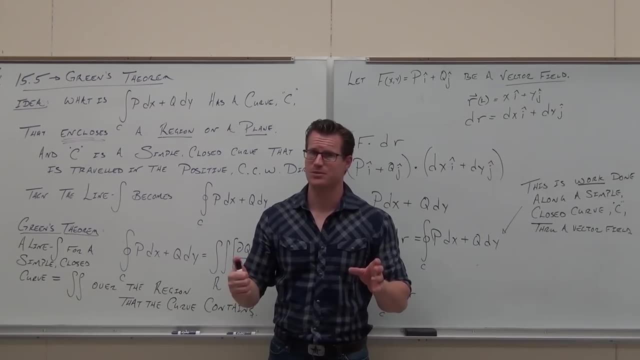 It's just I couldn't explain it because we hadn't talked about work done through vector fields. You guys see what I'm talking about now. Are you alive? still, I need your focus. I really do. Green Stereo doesn't have to be that hard, but you have to focus on it. 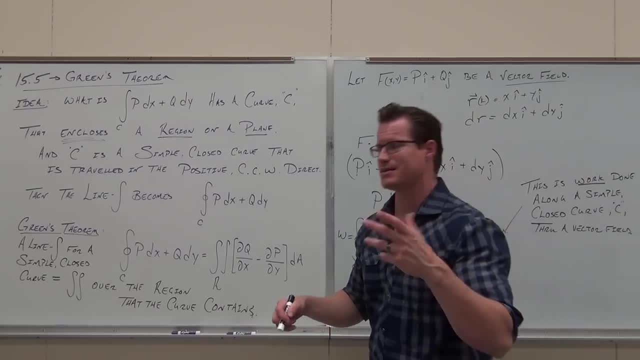 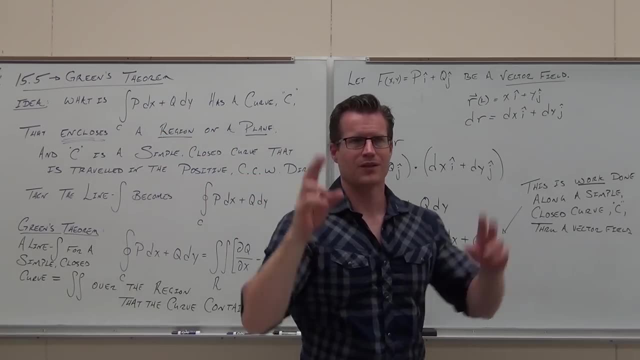 So let's go through maybe like a 45-second recap here to make sure we get the idea. The idea is: we have had line integrals for a long time now. What if we have a specific type of curve? What if the line now for our line integral is a curve that creates a simple closed curve? 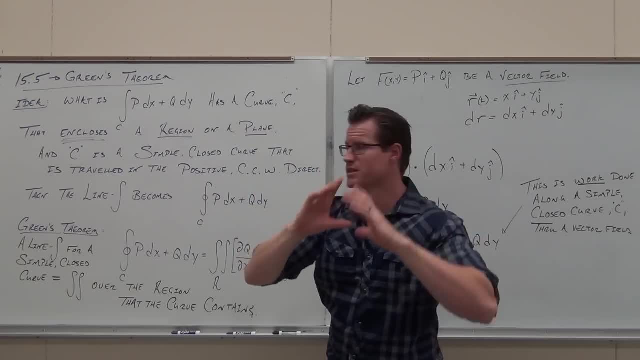 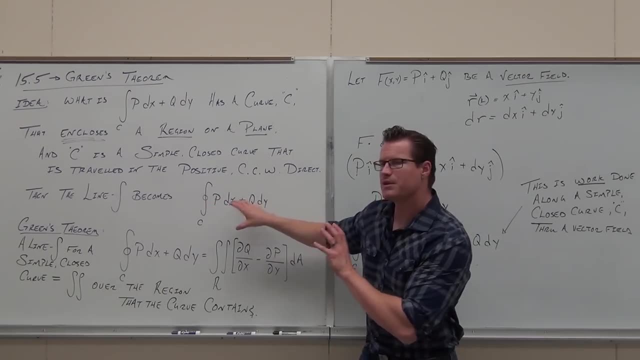 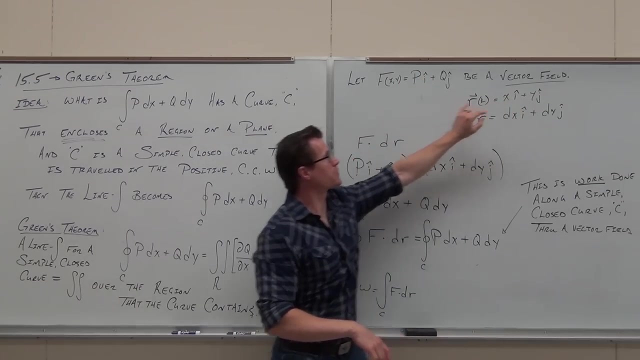 that bounds a region. So this region's in there and we're traveling in a positive, counterclockwise direction. Then we have now a different look for it, But it's coming from the same place Where this comes from. it's just coming from, hey, a curve through a vector field. 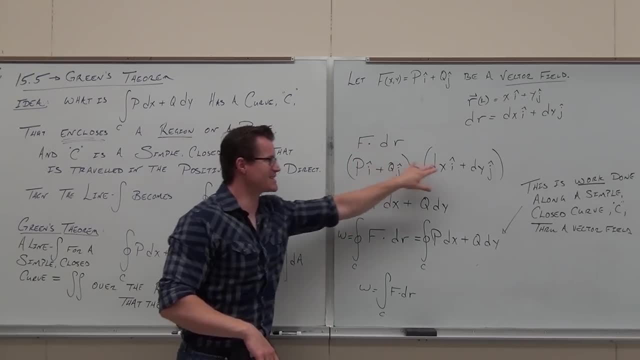 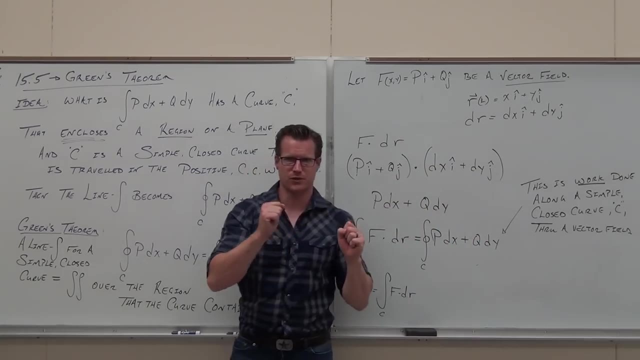 that happens to be a simple closed curve. It's done. Here's the dot product. It's exactly the same thing. It's coming straight from that. You guys see that all this is is work done through a vector field Along the simple closed curve. 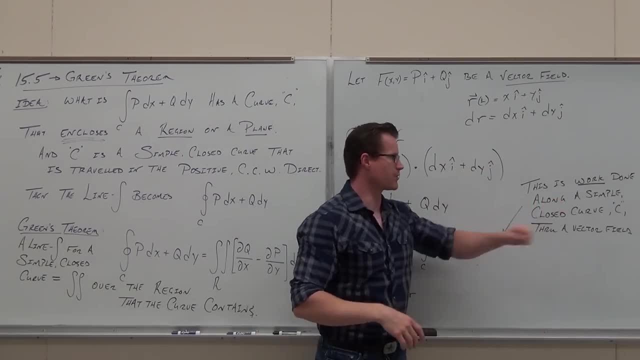 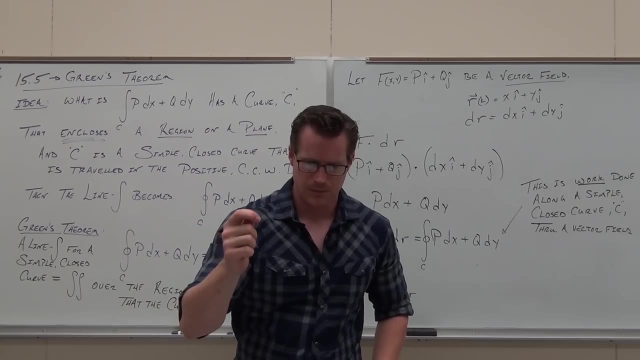 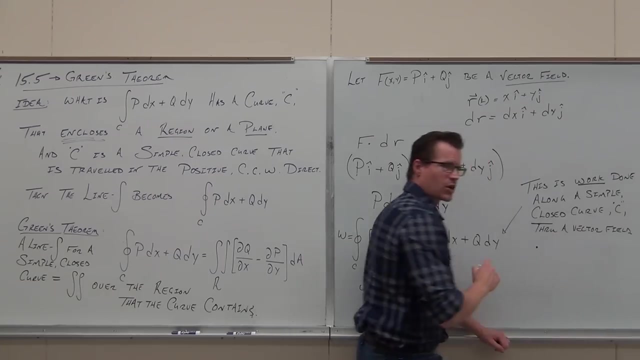 That's what that means. So this is work done along a simple closed curve through a vector field. That's what we're doing every single time That we have that. But but but wait, Wait, a minute. Wait, You tell me we're starting at a spot, right? 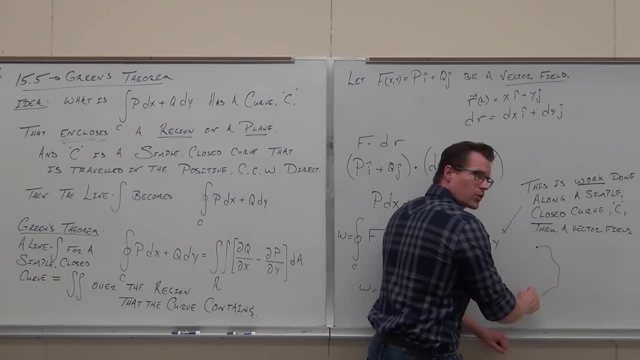 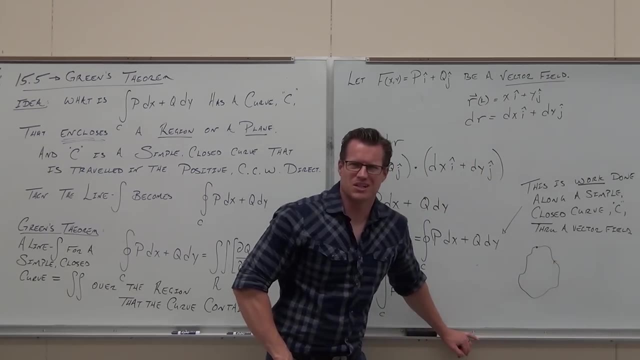 We're going through a vector field And we're doing work And we're coming back to the same spot. Isn't the work just zero? Isn't the work just didn't we find that last time We did the exact same thing. 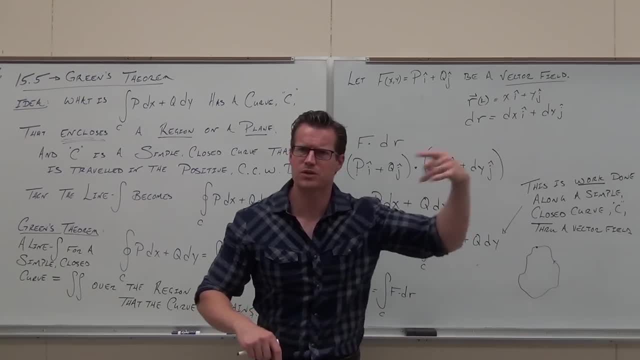 Oh yeah, the work is zero. Because if you, if you do work along a simple closed curve, then if you, if you're moving a particle from one spot back to the same spot, aren't you? aren't you doing no work? 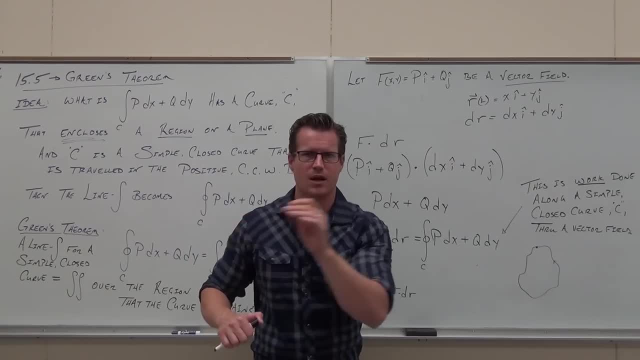 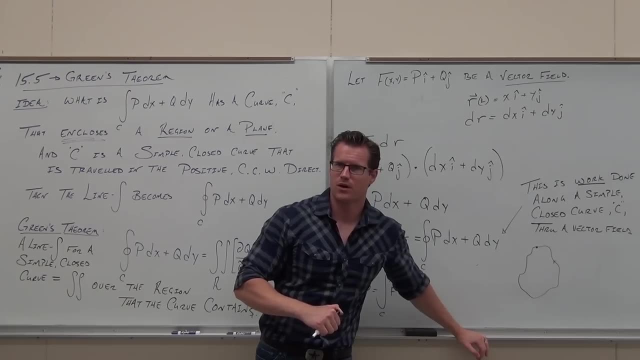 Because I literally showed that in the very last section. But no, I said something there. I showed that in the very last section. Is the work done on a simple closed curve? if I go here and go back, Is that always going to be zero? 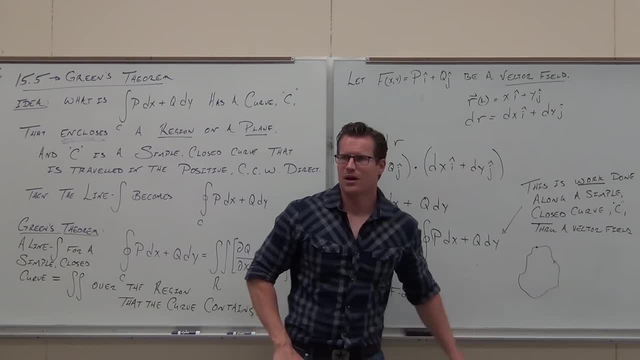 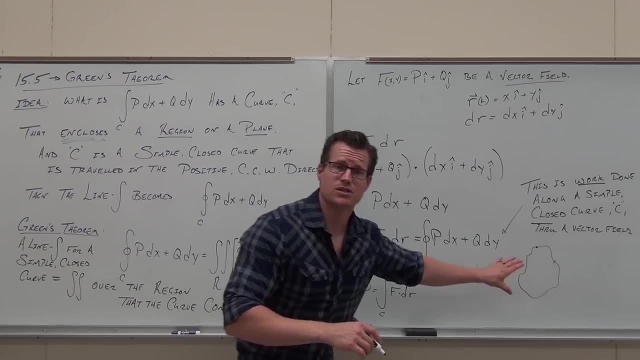 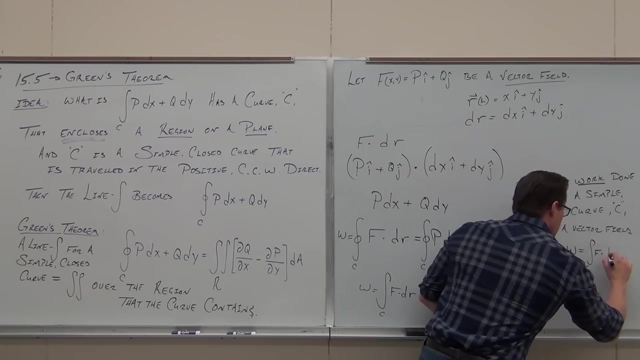 What did the last section have to do with it? Zero in the vector field. That's the whole key. You listen carefully right now. okay, The last section said: yes, the work done here is zero for a simple closed curve, If you have. what type of vector field? 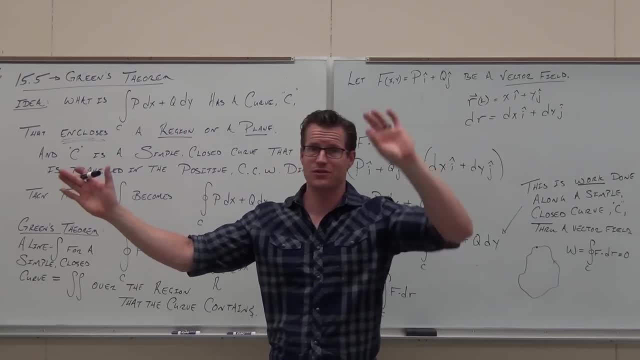 If you have what type Conservative Conservative, That makes sense. If it's conservative, You're going to get zero. You're going to get zero. You're going to get zero. You're coming back to the same spot. You've done no work. 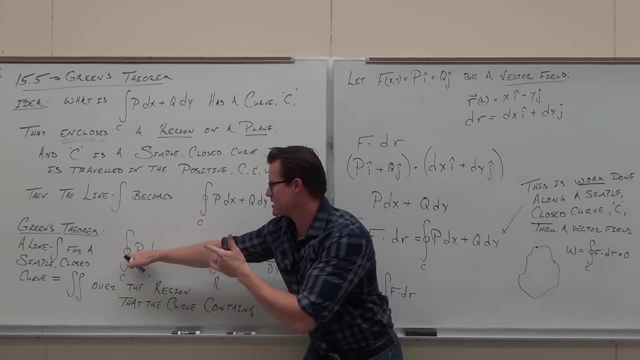 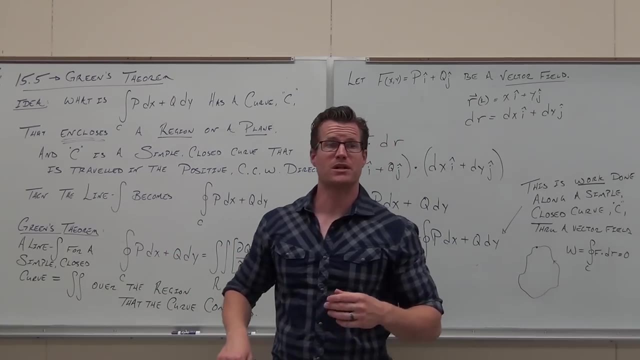 So here's the, here's the thought. now, If this is dealing with simple closed curves over vector fields, which I've just proven that it is, what's the type of vector field that we have for Green's theorem to take place? Is it conservative? 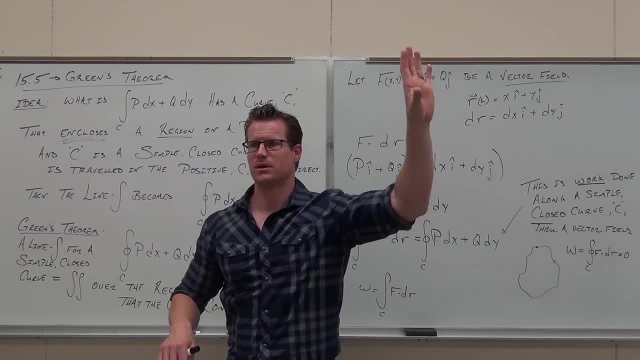 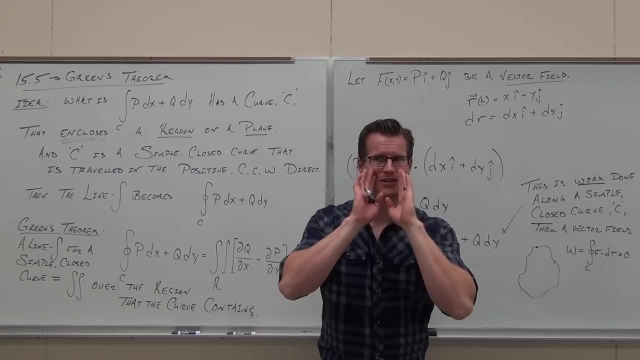 No, If it was, they'd all be zero. So I'm going to go through it again, because some of you didn't get it. Simple closed curves on conservative vector fields would give you work at zero every time. This was for conservative. 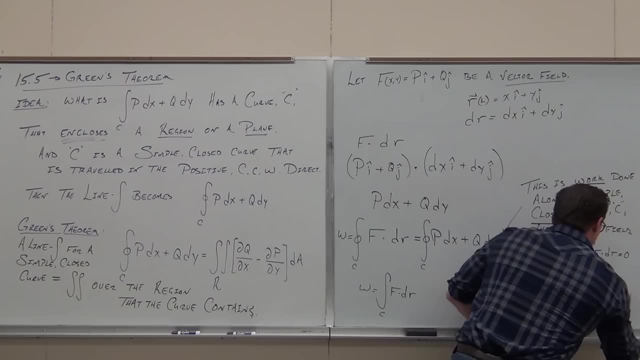 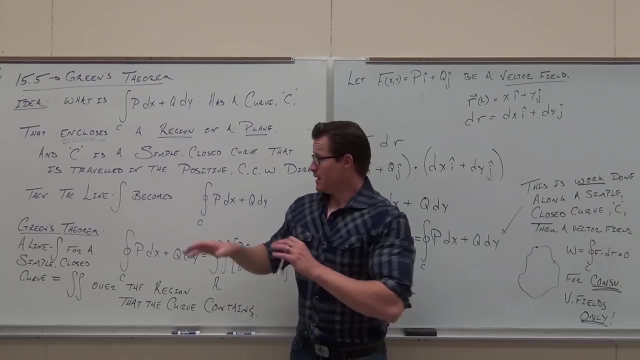 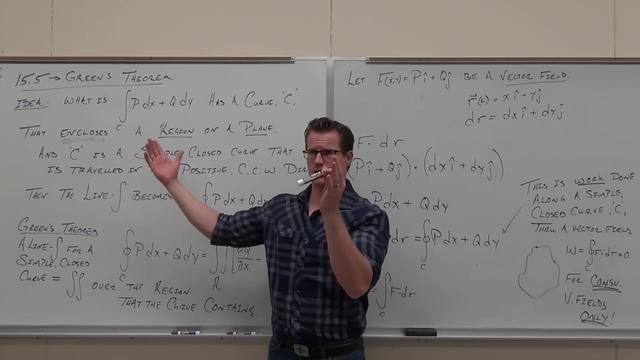 Conservative vector fields. Only That was for conservative vector fields. So then let's put it this way: If these are all conservative vector fields, how much would all of these line integrals over simple closed curve be Zero? It'd all be zero. 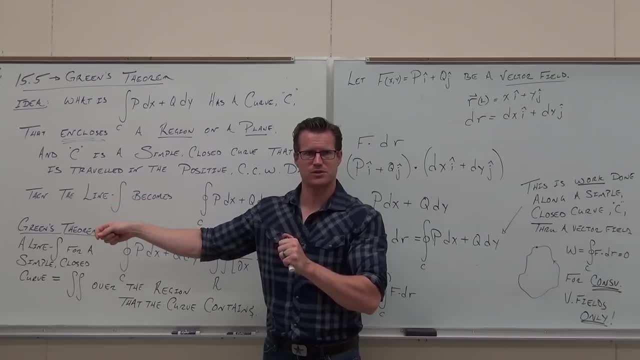 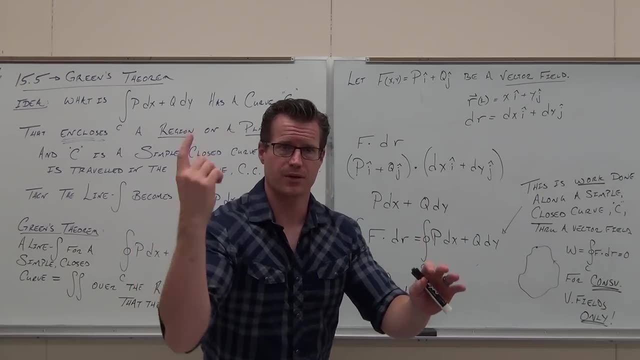 So does Green's theorem generally deal with conservative vector fields? No, No, That's where Green's theorem comes into play. So I'm going to say it one more time: Get your head wrapped around it If you have conservative vector fields. 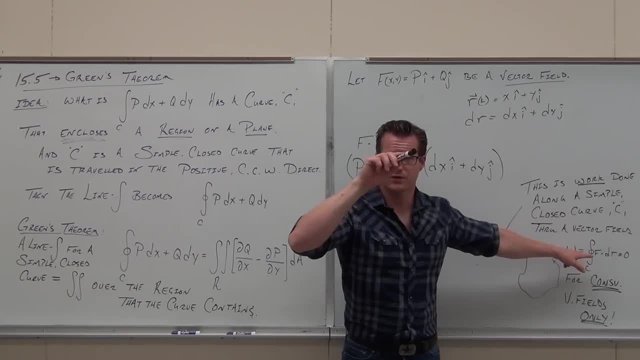 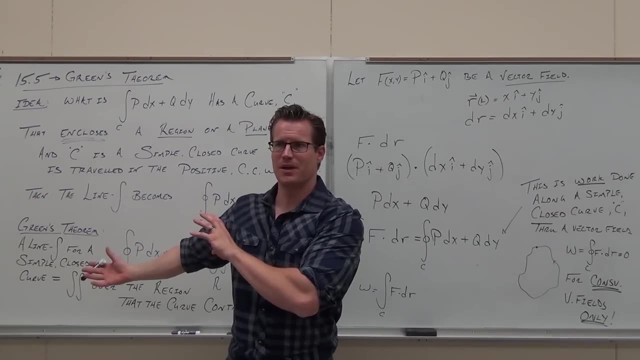 the line integral through a conservative vector field of a simple closed curve is zero. If you have non-conservative vector fields, Green's theorem shows us what to do. In fact, I was going to wait until later, but I can't handle it. 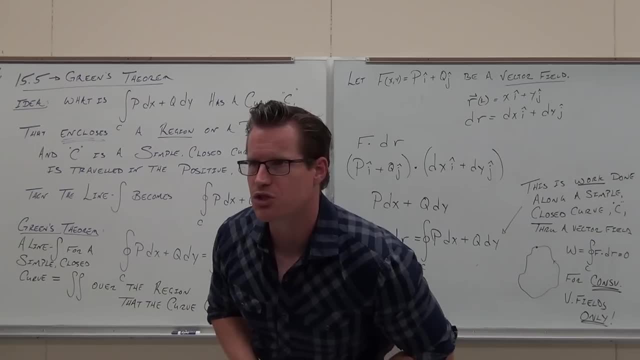 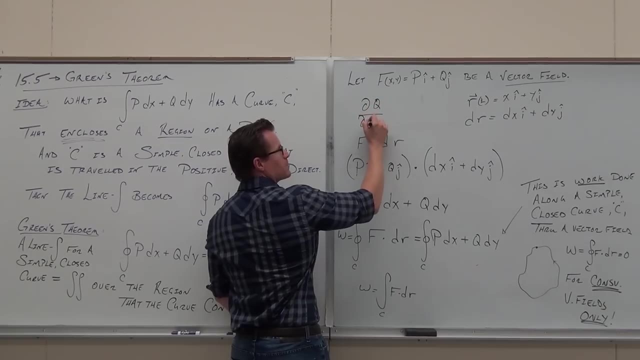 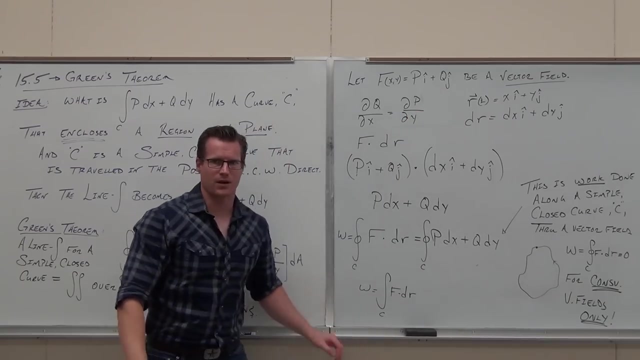 The suspense is killing me. Do you remember how to show that vector fields are conservative? Do you remember how to show that? this right here, that that right? there is how you show that vector fields are conservative. Do you remember that? Subtract this side. 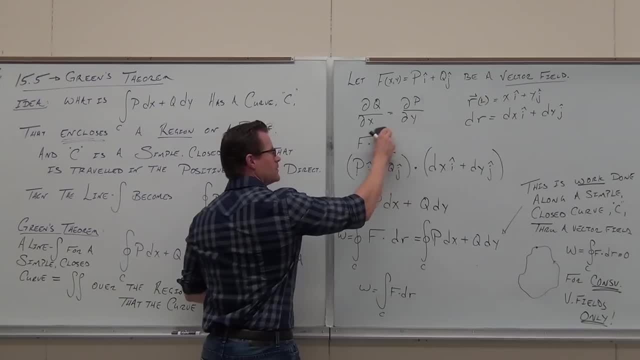 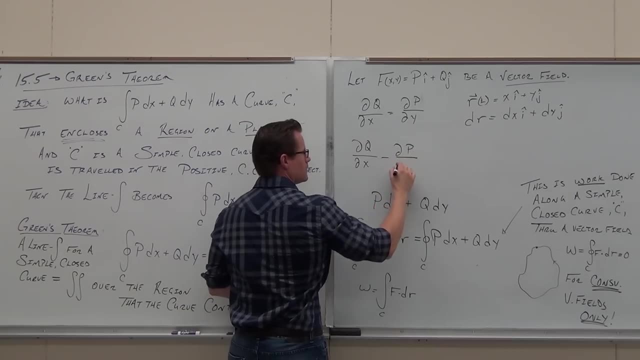 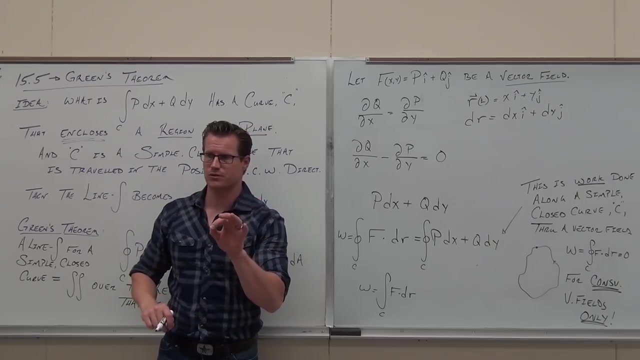 Subtract this from both sides. Subtract this from both sides, and you're going to have a conservative vector field of zero. I will prove it to you right here that Green's theorem does not deal with conservative vector fields. You ready, You ready. 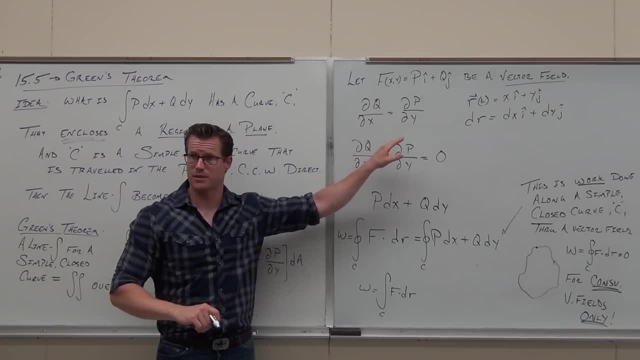 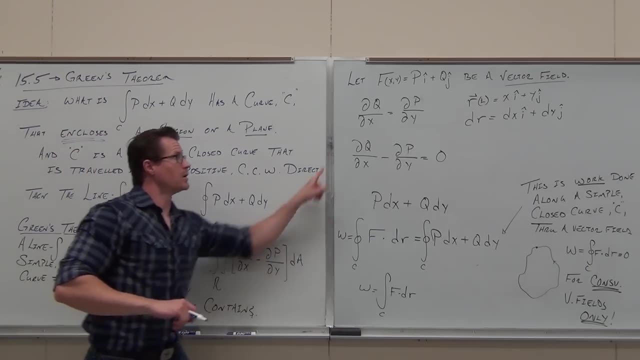 You ready? I hope you're looking. If you blink, you're going to miss it. You understand this concept right? This proved conservative vector fields. If we have a conservative vector field, this would be zero every single time. In fact, we use that in Green's theorem. 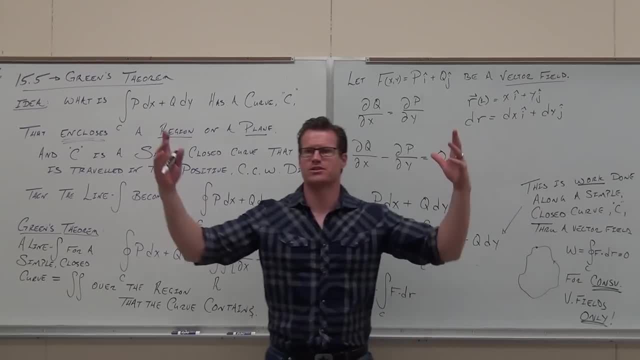 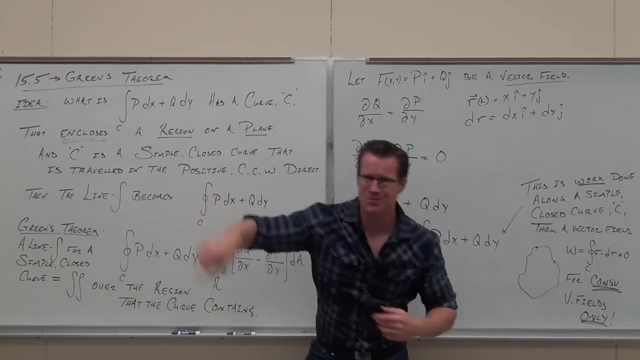 We say: hey, If you ever get a zero in here you're work done. zero because it just proved that your vector field is conservative. And if you just proved your vector field is conservative for a line integral over a simple closed curve through a conservative vector field, you got a work done of value zero. 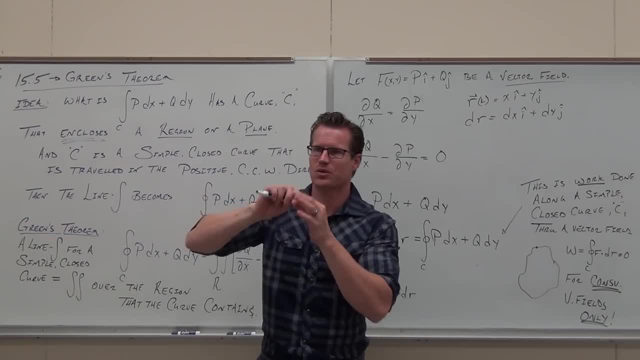 Isn't that kind of cool, right? Is it starting to make sense to you? So we get these line integrals. that were just random pieces. We did that two sections ago. Then we said: let's assume that we have line integrals. 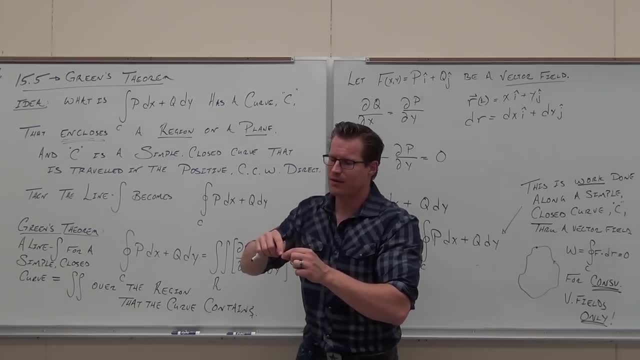 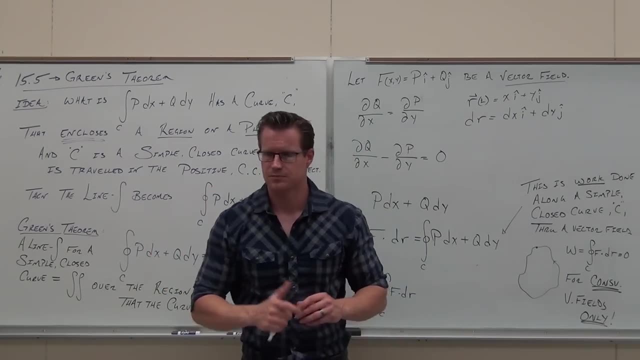 but it's over conservative vector fields. Now we did that. Now let's assume that we have these curves that connect, but they don't have to be conservative. That's where we're at right now Question. So can we use this to prove a vector is conservative? 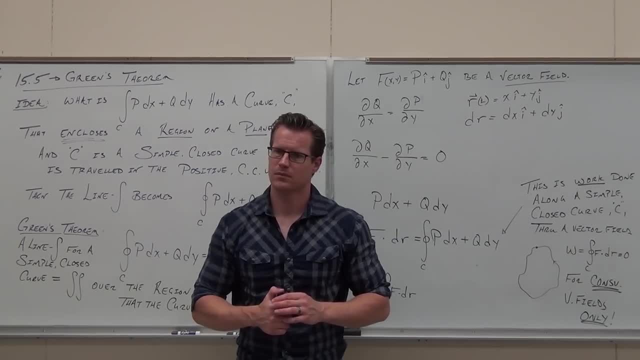 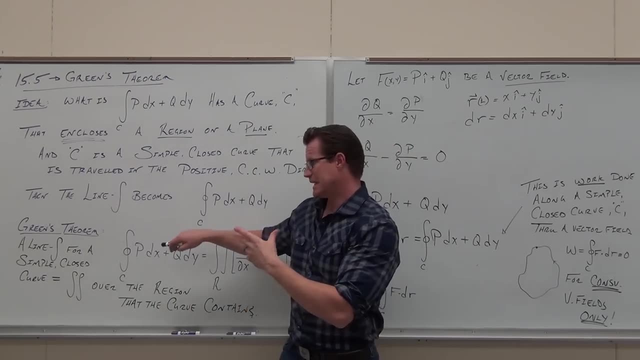 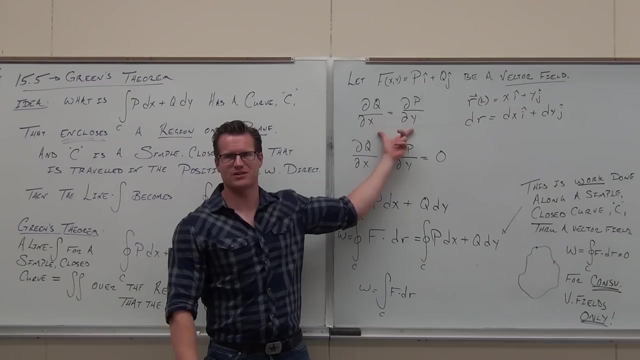 if we want to use the conservative vector function. A vector field is conservative. Yes, It would be a lot easier just to do that Right. You kind of do it intrinsically in Green's theorem, Do you guys see it? Do you guys see that this is conservative vector field? 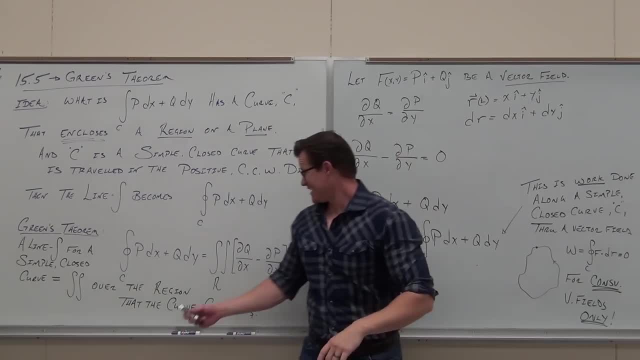 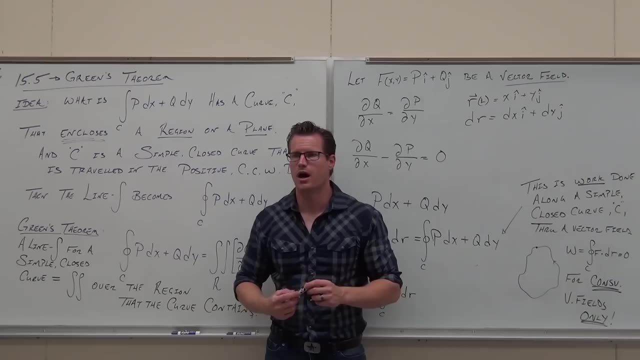 You see, the subtractable size gets zero. Do you see that this piece? It's zero, It's in there. That's what I'm saying. Do Green's theorem? It's going to show up whether you have a conservative vector field or not. 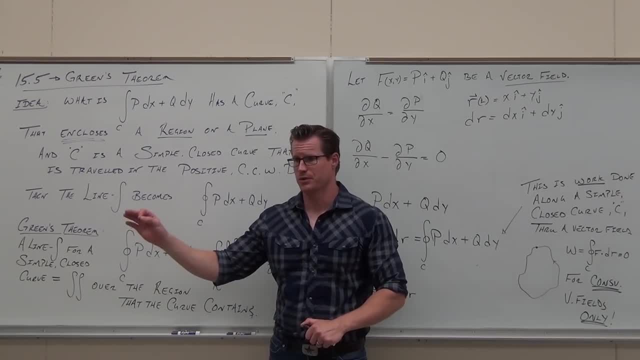 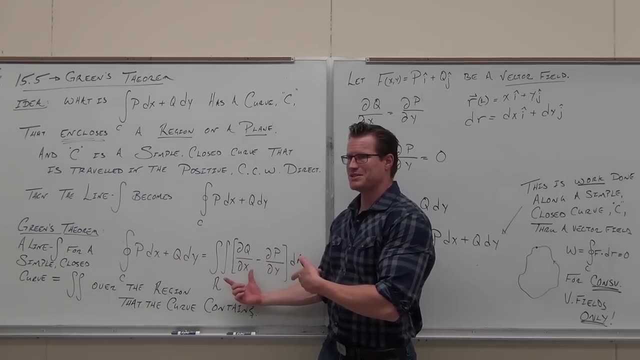 If you get zero conservative done, Just put zero, You're done for Green's theorem. if it's a simple closed curve, You guys get it. If you get something in there, you have a double integral over a region that's really easy to define. 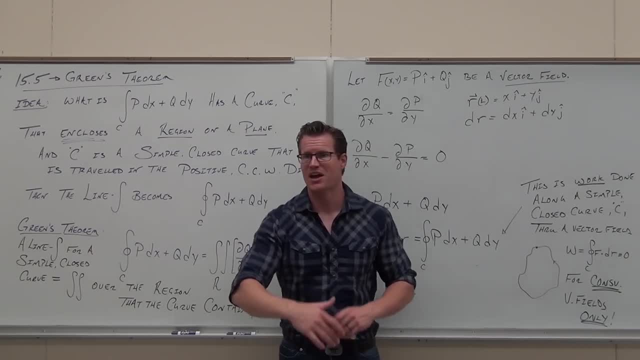 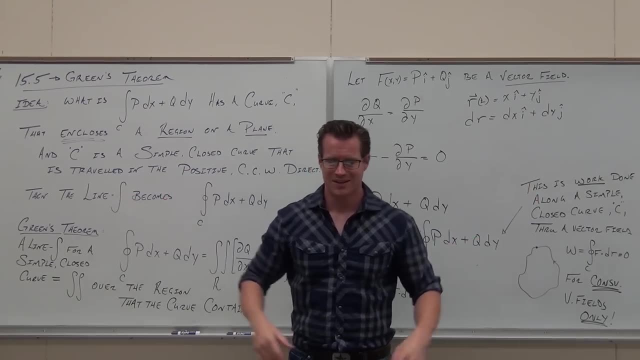 And like half your variables are generally gone because you're doing partial derivatives. It's freaking awesome. Okay, It makes your life easy. Green's theorem is awesome. It's cool, It's a cool thing. So here's our walk-through one more time. 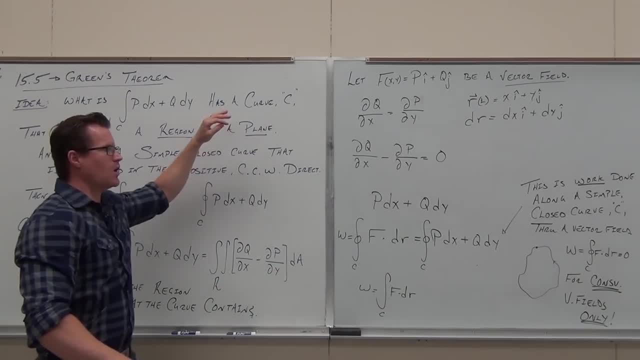 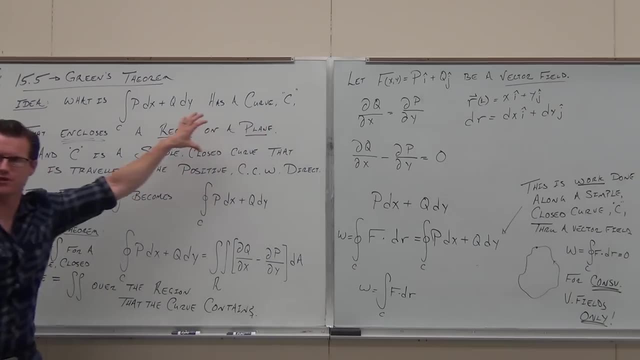 Our walk-through says that simple closed curve for line integrals over conservative vector fields gives you work done of zero Over non-conservative vector fields- Green's theorem. So I'm going to write one statement out. You need to write it down. 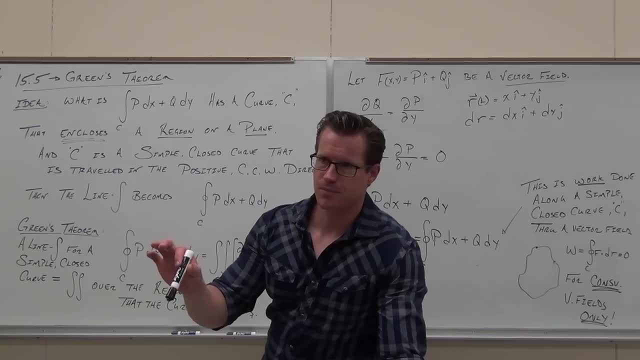 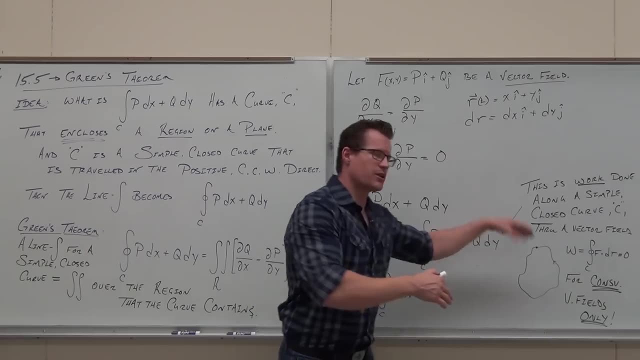 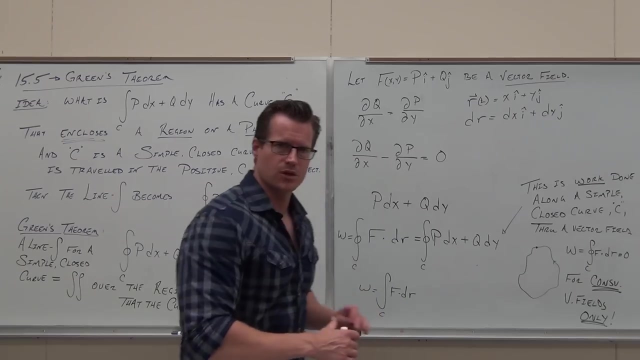 So Green's theorem deals with line integrals of simple closed curves through non-conservative vector fields, Because if they were conservative we would get zero every time. Write that statement down, would you? Green's theorem deals with line integrals of simple closed curves through. 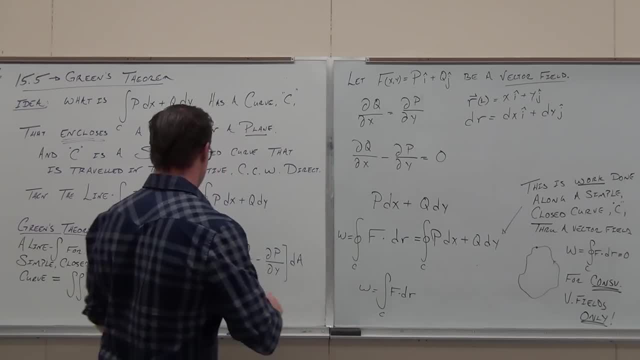 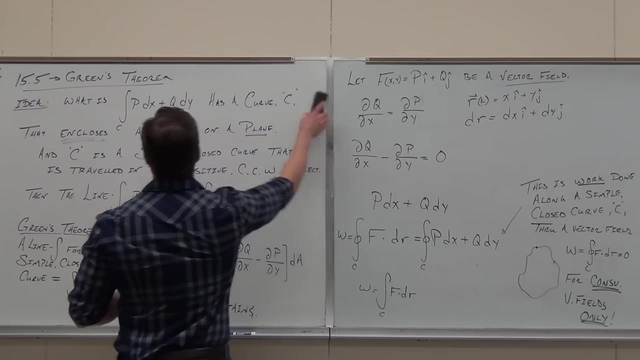 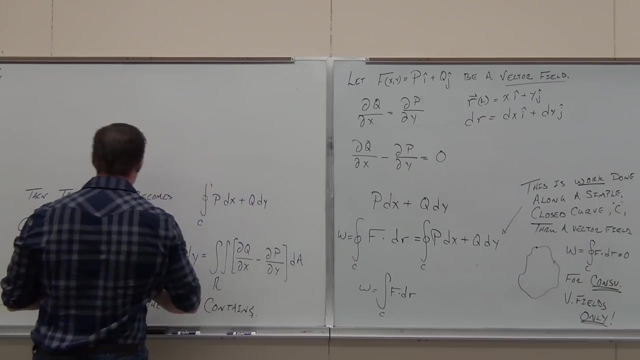 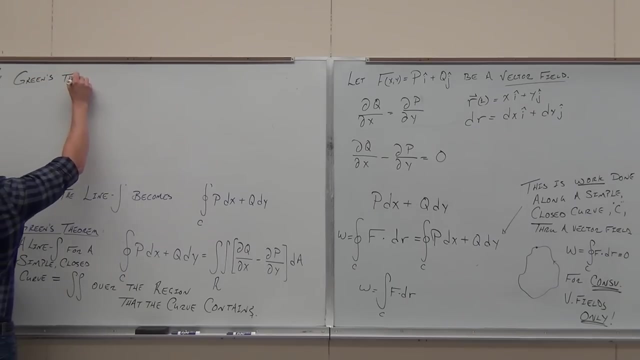 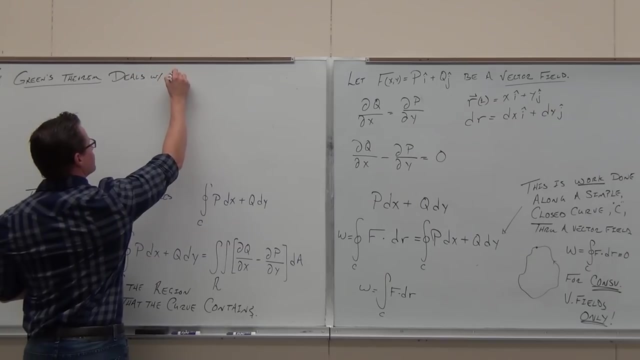 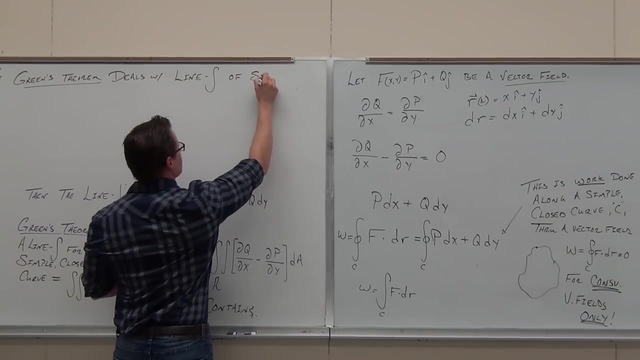 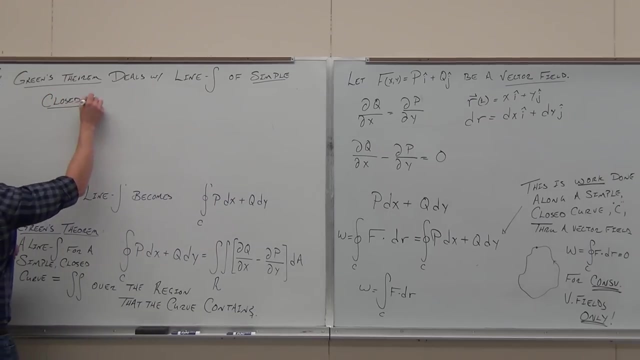 of a simple closed curve through non-conservative vector fields But among nonconservative theisine of one bunk of non-conservative weight accumulation, which is the weight of r, is positive. r. Theионic Theimouth Thumbnail. 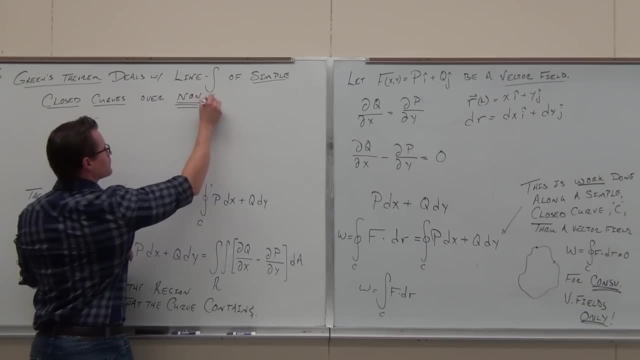 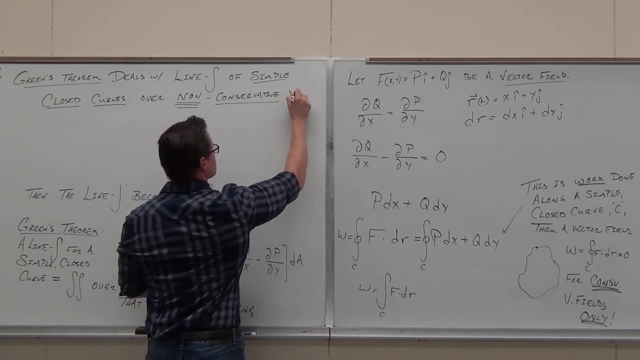 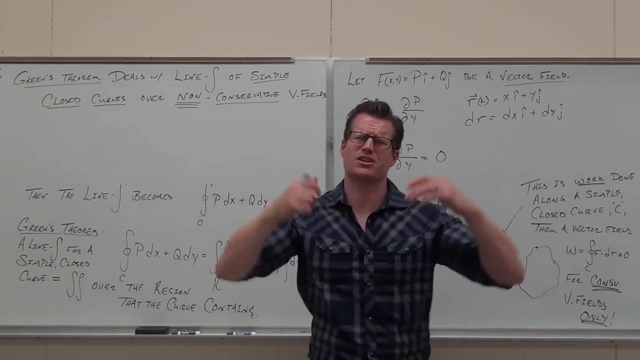 Less stlaf Circle Curve. Let's say: screw it up. let's say that you go. oh my gosh, I did Green's theorem on a conservative vector field. Is it a big deal? Yeah, Not really, because you're just going to get zero. 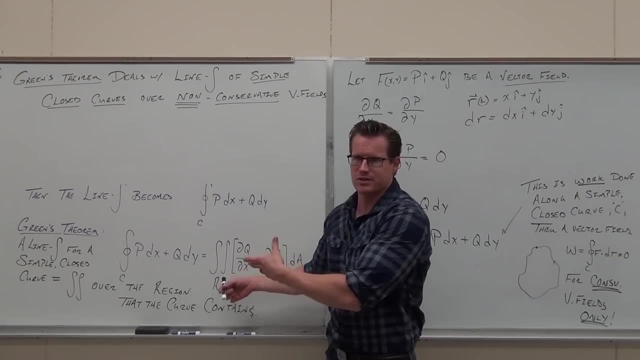 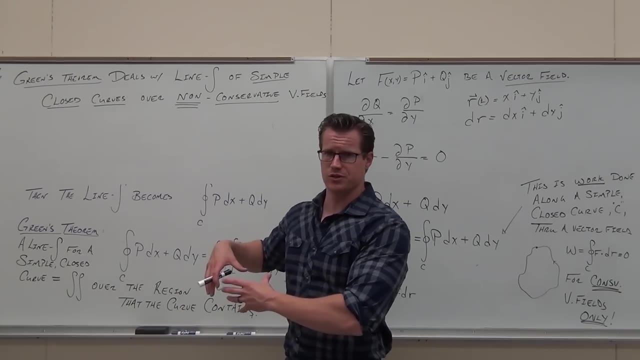 Because this is the proof right for a conservative vector field. So if you just go through Green's theorem, you're just going to get zero. So it's not even that big of a deal. All I'm saying is that Green's theorem is relevant- relevant for non-conservative. 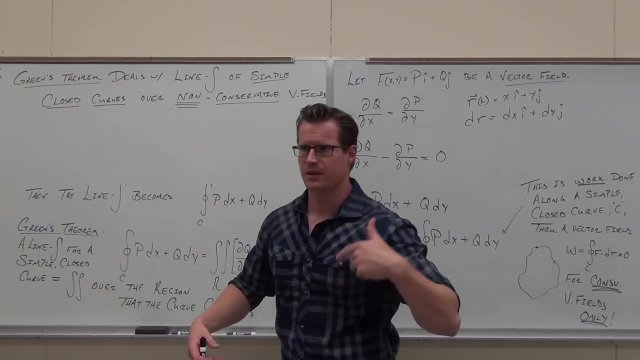 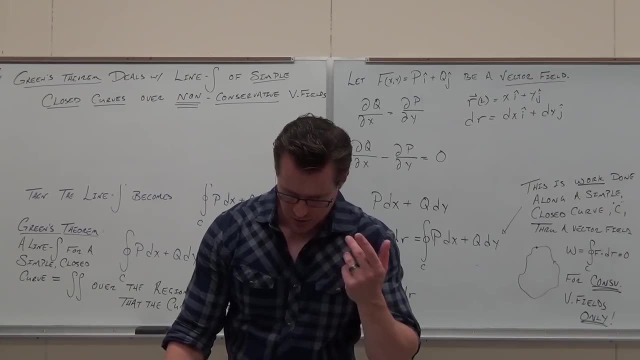 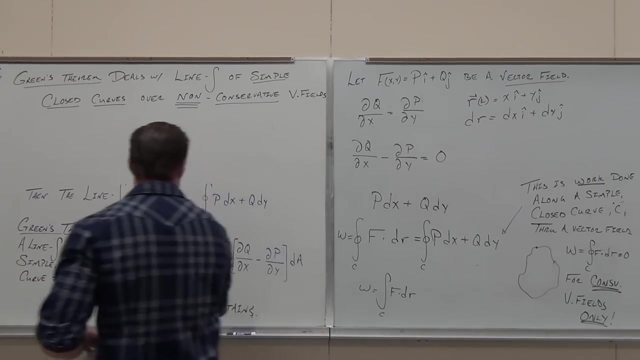 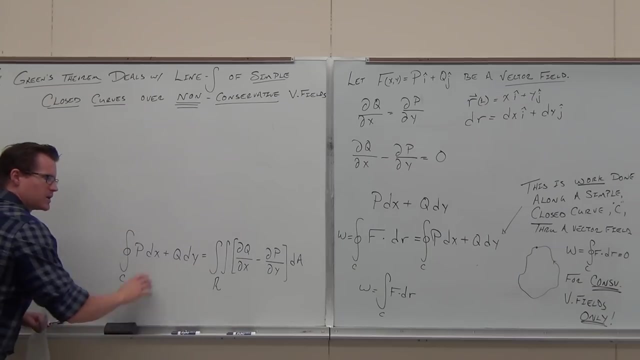 It's not really relevant for conservative because we get zero anyway. Does that make sense? That's it. That's the whole theorem, part of this stuff. Honestly, right now, all we have to do is practice. So the thing that we're going to practice is how we change. 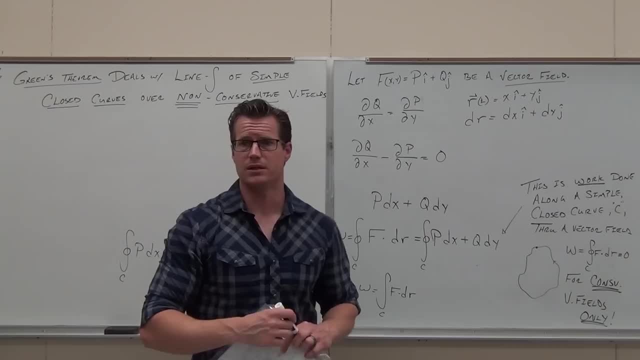 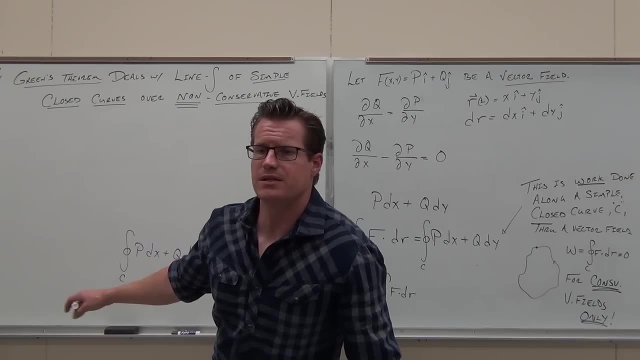 from here to here. There's only two things that we need, Actually, only really one thing. You need a non-conservative vector field which is going to show up no matter what, And you need a simple closed curve. That's the biggest idea. 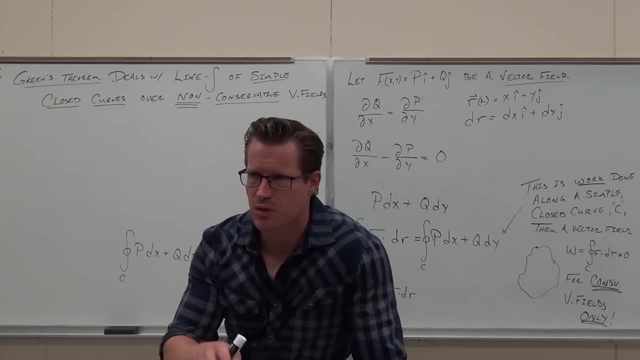 So we've got to show that we have a simple closed curve. You guys understand the idea: If you don't have a simple closed curve, you don't have a region. If you don't have a region, you can't do a double integral. 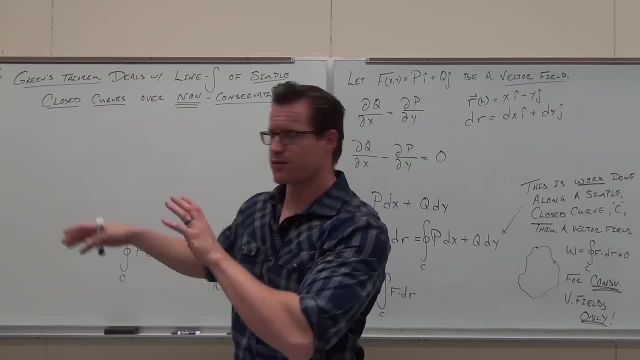 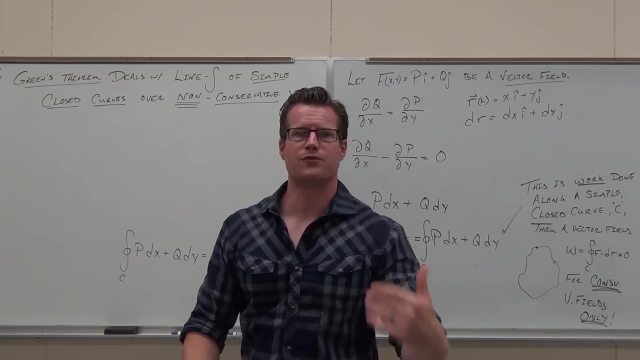 So that's the whole premise for Green's theorem. The whole conservative vector field thing is going to show up when you calculate that. So I'm going to show you how to do it. We're going to set up a ton of them. We're only going to work through a few of them. 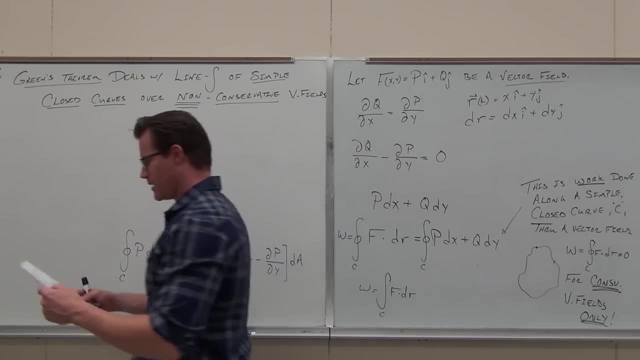 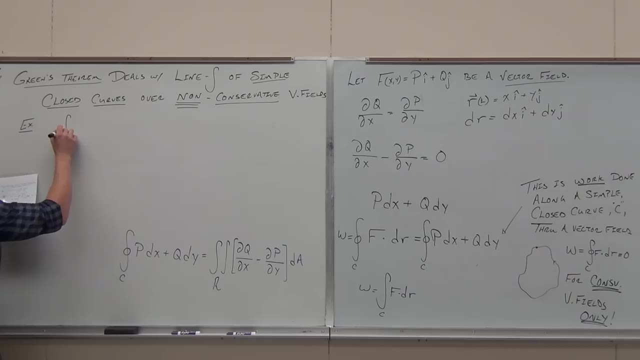 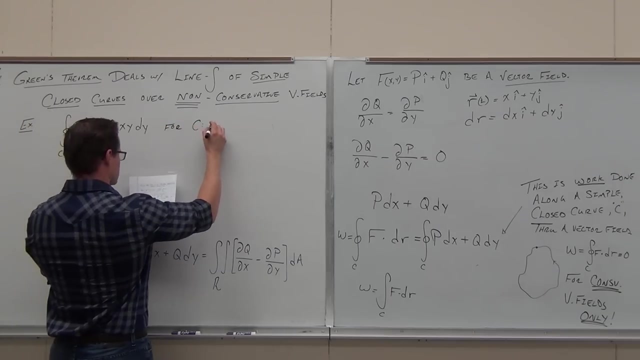 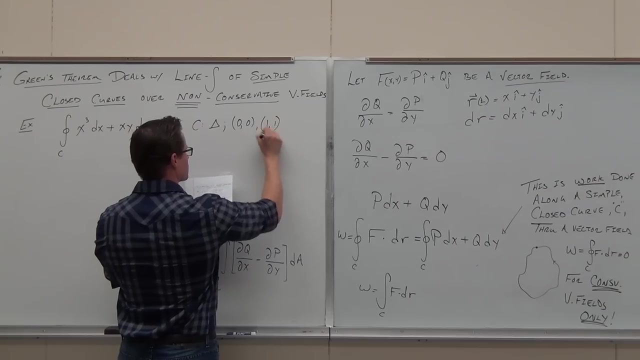 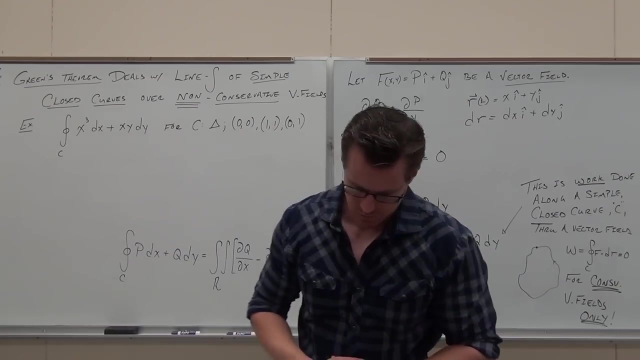 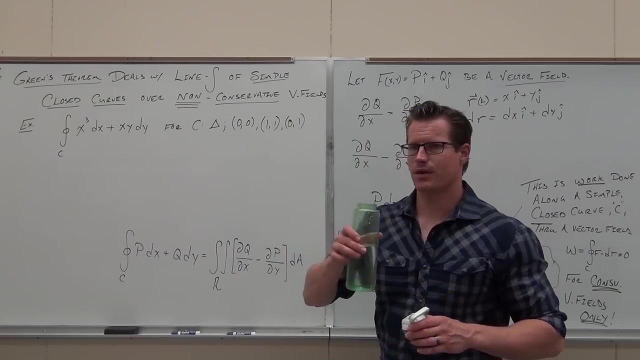 Again, this is all about the setup. You guys can do some basic integrals here. Let's start with this one, Okay, Okay. So let's take a look at the line integral. What's that say right there? What's the line integral telling you? 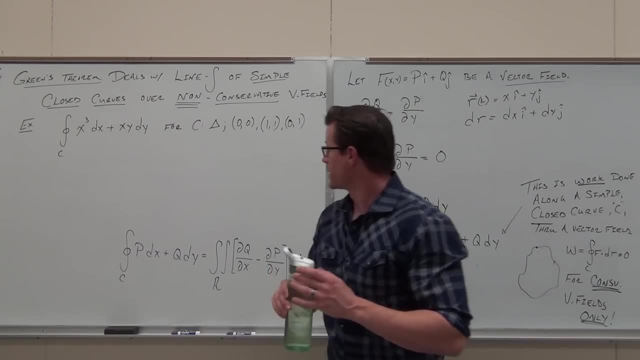 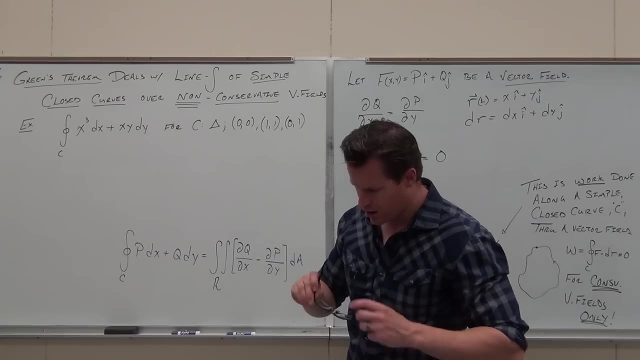 It's going to have a simple closed curve and then it's going to give us that curve. Here's what I want you to do. I want you to do a few things about this. Number one: I want you to draw that simple closed curve every single time. 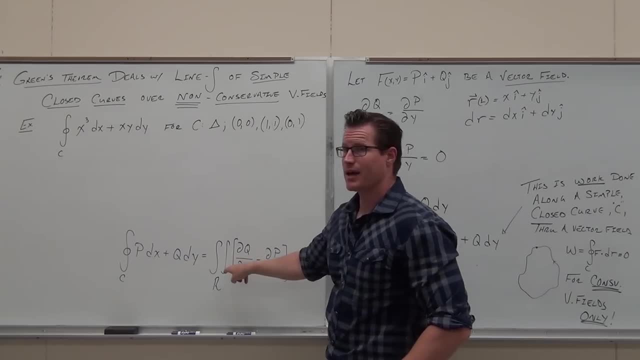 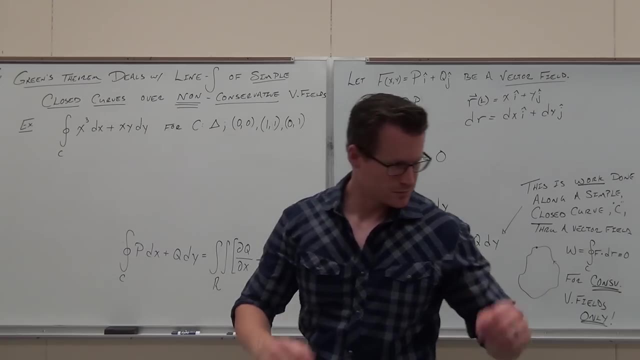 Every time. Why? Because that curve has to contain a region, and how we set up our double integrals is draw the region every single time. So can you please take some time to draw that triangle? There's some water all over that. 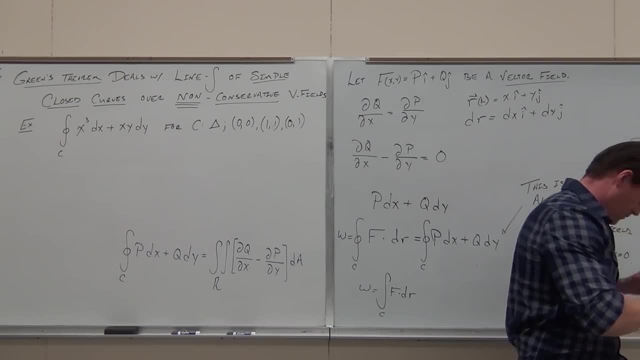 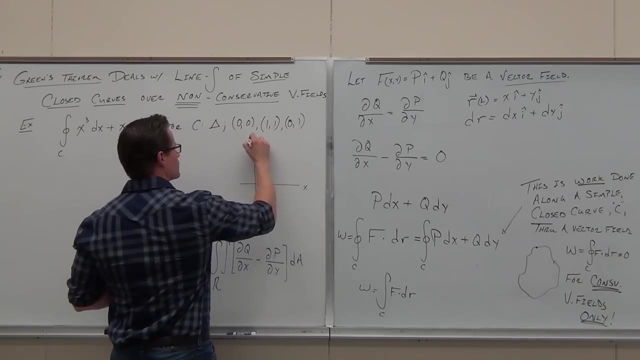 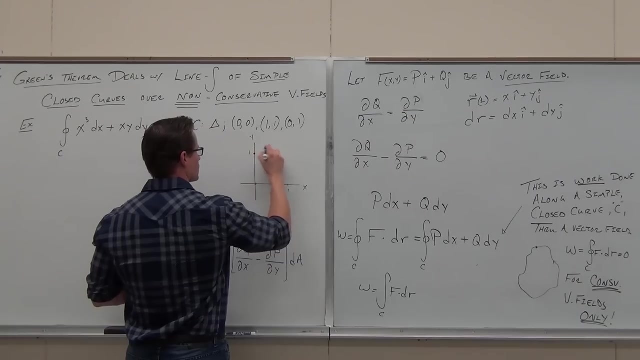 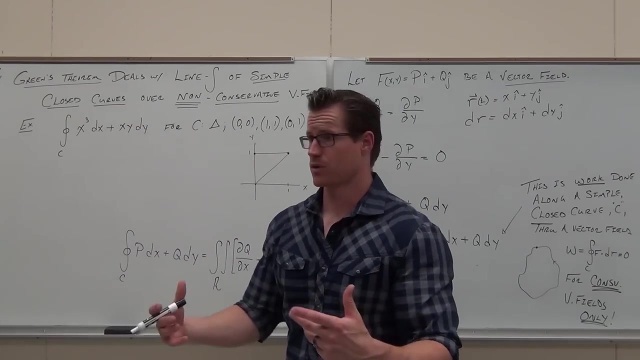 Okay, Okay, Okay, Okay, Okay Okay. I only have this very small triangle. It's not a, So I'm telling you it's a triangle. so I'm telling you triangles are simple closed curves. We're starting. it doesn't really matter. 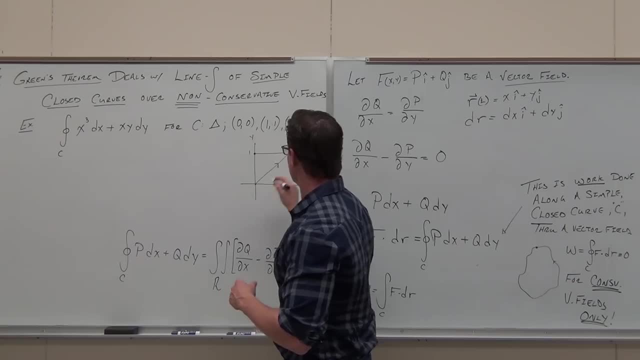 We're going, Bur sagt, We're going positive counting. So now when we draw our triangle, are they such a good triangle, Positive, counterclockwise direction? that's a simple closed curve. Can you guys see the region that it contains? 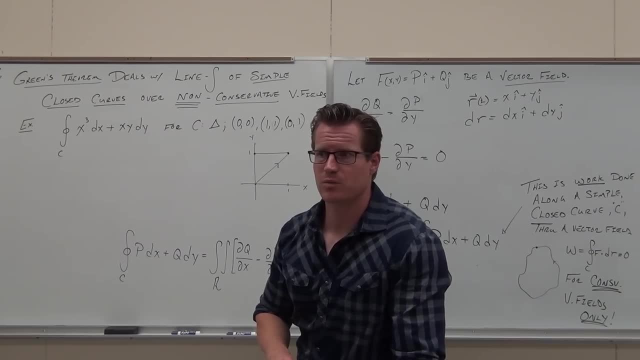 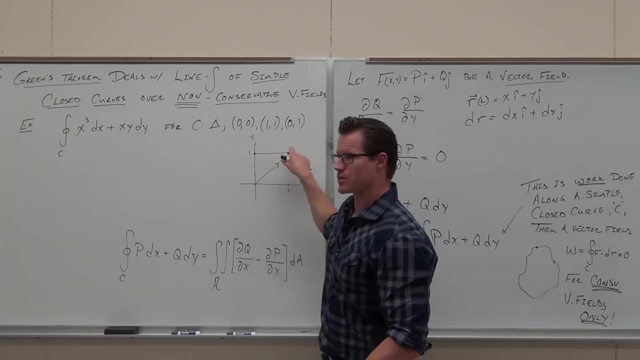 If it wasn't a simple closed curve, we wouldn't have a region. That brings me to one point here real quick. Please listen, Please listen carefully. Let's say that I didn't tell you it was a triangle. Let's say that it was just these two segments right there. 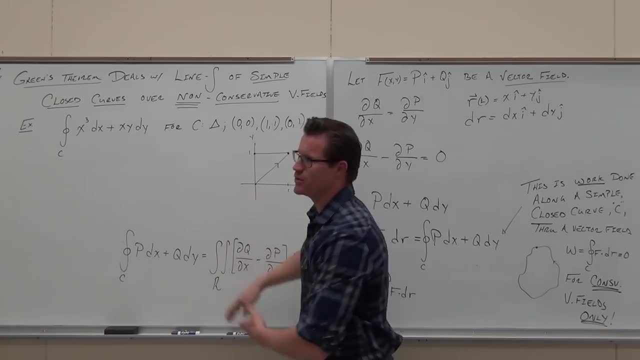 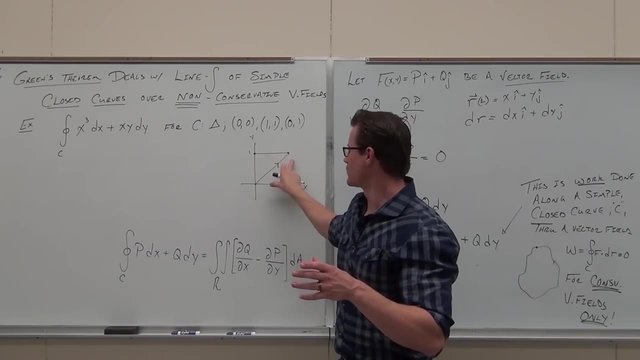 If I don't contain a region, I can't use this. I fall back to two sections. I'd have to redefine segment. Remember doing segments. Remember doing that Vector function of segments. One of them, two of them, two different integrals. 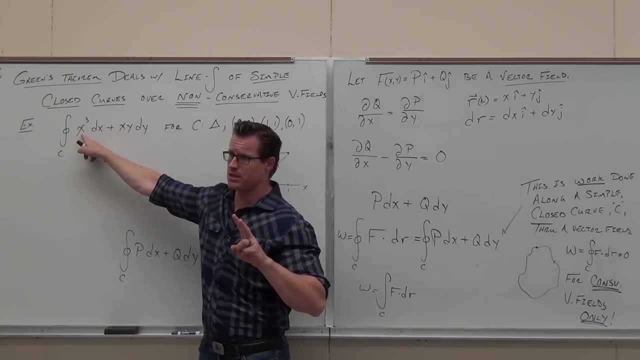 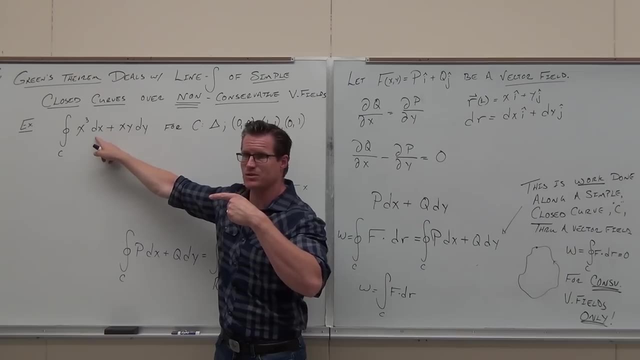 and you'd have to do it, redefine all that stuff in terms of t and then dx in terms of t. Remember doing that stuff where you plugged in t's. for here You took a derivative. plugged in the dx equals something dt. 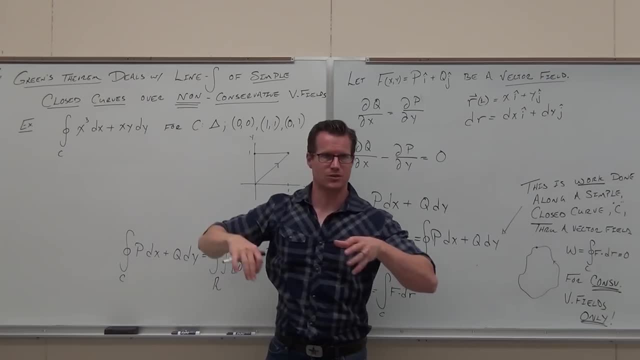 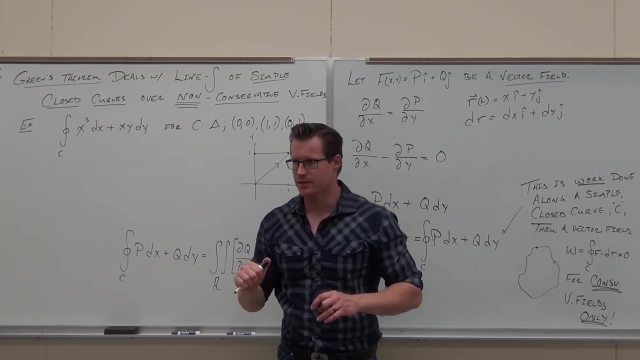 t's, t's, dy equals something dt, and you did that integral. You'd have to do that for two of them. So is Green's theorem going to make your life easier? You better believe it, yes, if we have a simple closed curve. 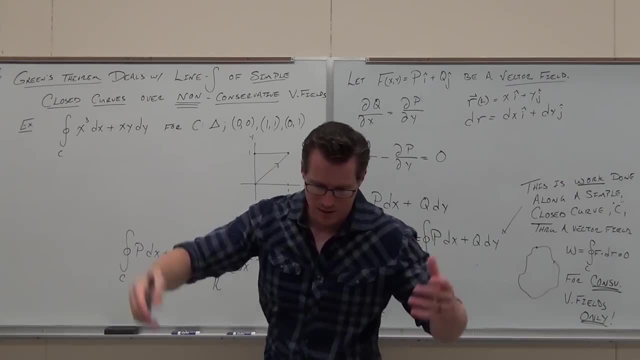 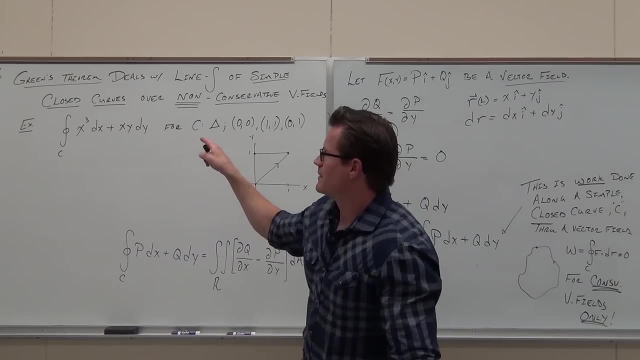 So if you understand that concept, that's a big deal, But we've already done it, just so it would suck. Also One thing I want you to do here. the second thing: sometimes- and I hate it when they do it, but they do it a lot- 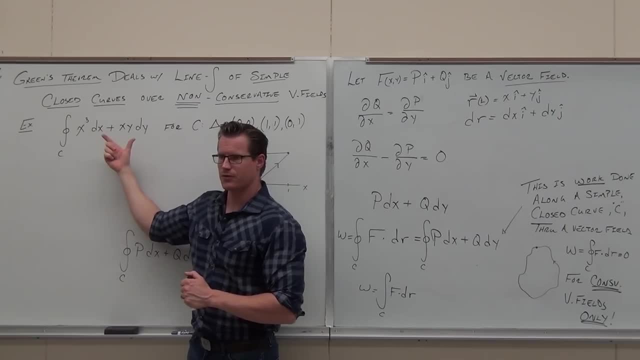 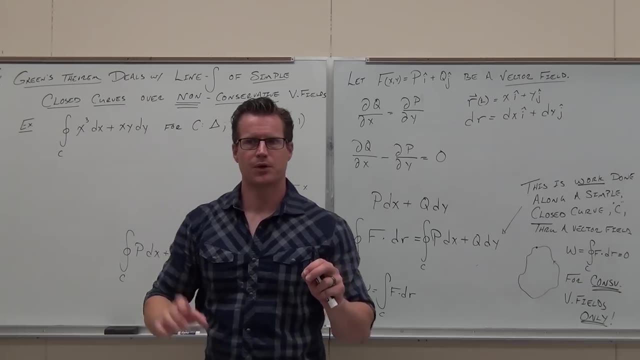 Books will have these switched up. I will always write a dx dy for you, but some do dy dx. blah, blah, blah blah. they switch around. Would you please be very careful and right now put a p above the part, right before dx, and a q right above the part. 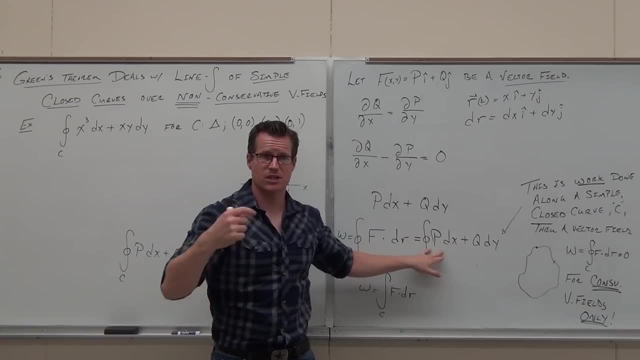 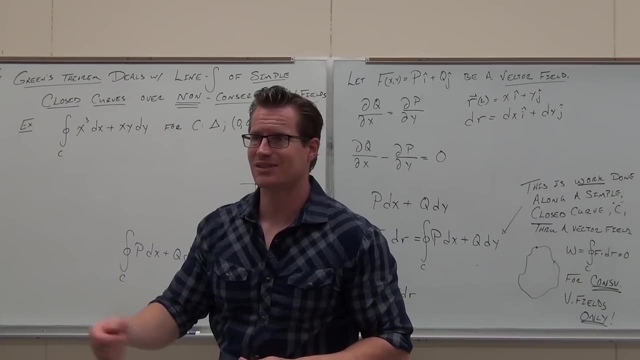 before dy. that's what this is saying. here The p is associated with dx, The q is associated with the dy, So put that up there somewhere so you don't get lost. Is that a good idea? Yeah, it's a good idea. 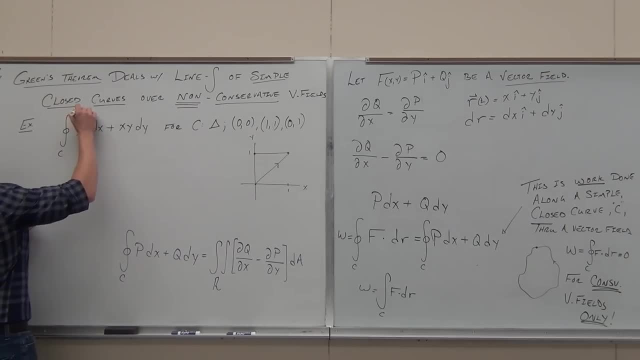 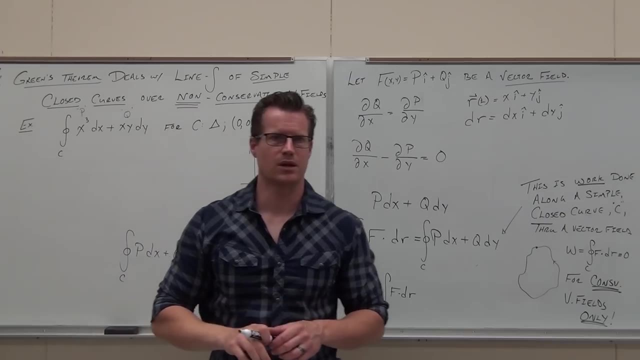 So this right here says which one's this one D and that's the q, just so you don't get lost on this stuff. I don't know if you're okay with that one, By the way, if you wanted to. 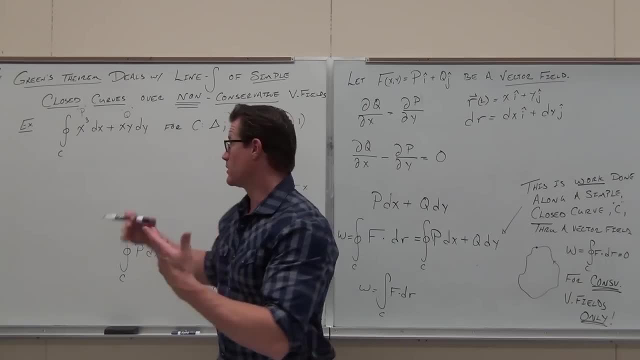 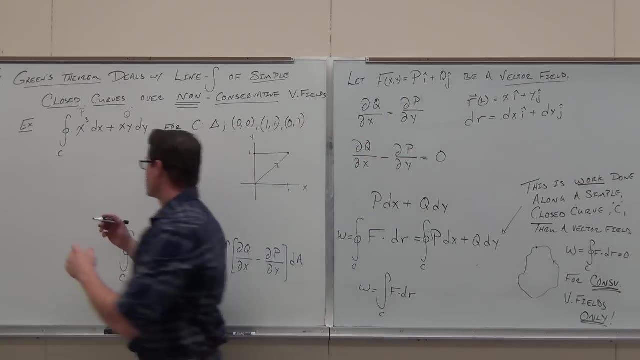 you could find the vector function that's creating this right now. if that's p, look if that's p and that's q, the vector function is just pi plus qj, if you wanted to. I'm not saying you need to. 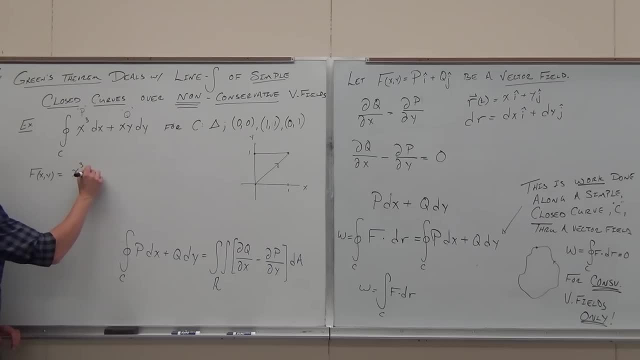 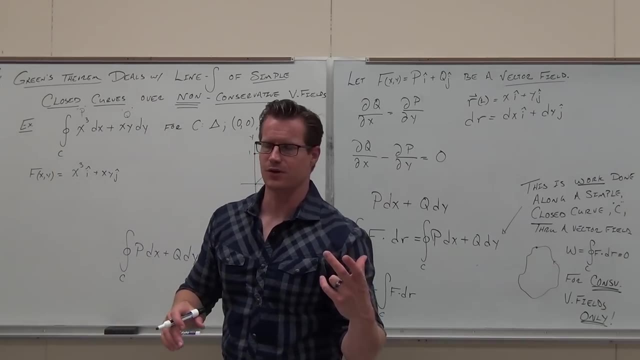 but your vector function right here is x cubed i plus xyj. It's coming from something, It's coming from the vector. I think it's a function, but it's coming from the vector. that's what that is. That's the part of it. 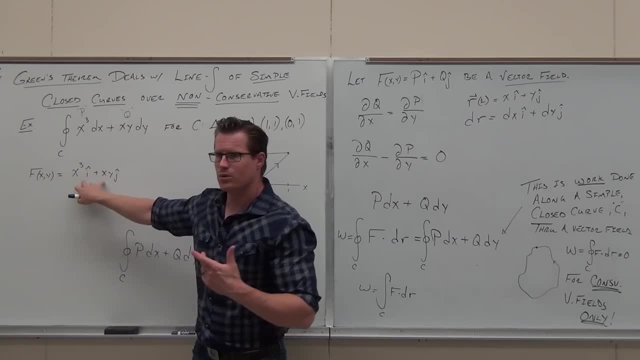 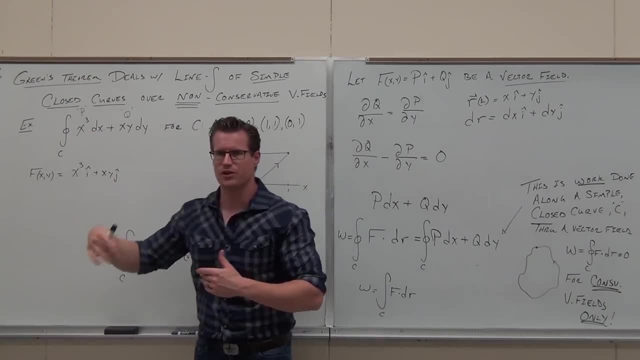 I don't know if you're okay with that one. That means that you could show whether this is conservative or not. you don't even have to write it, but this is where it's coming from. It's why this part is relevant to being conservative or non-conservative. 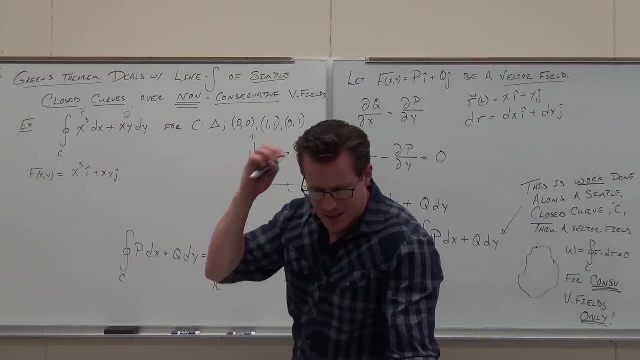 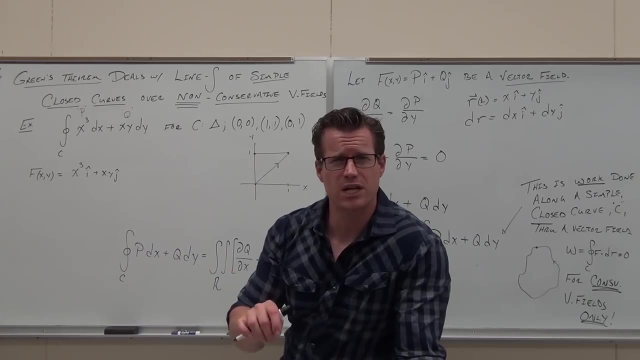 So let's go ahead and let's see if Green's Theorem applies. Firstly, is this a line integral over a simple closed curve? Then Green's Theorem applies. Can you define the region that that curve encloses? Then we can create a double integral. 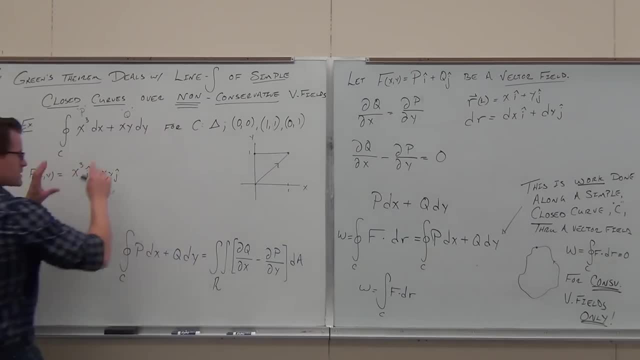 So here's how it works. It's honestly not hard. What Green's Theorem says is that for this particular simple closed curve, all I need to do is create a double integral over some region. I'm going to take the partial derivative. 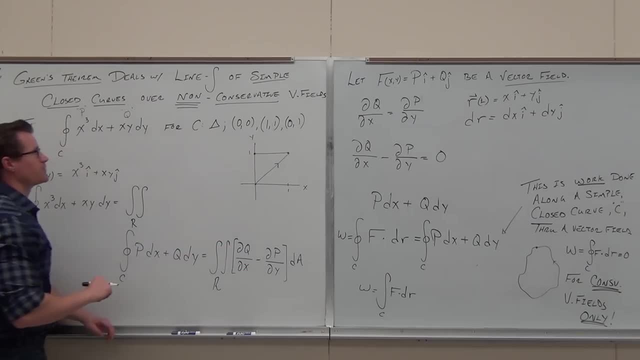 of the Q component with respect to X. Can you tell me what that is, please? Partial derivative of Q with respect to X: This: This is why we write it this with respect to X. Remember that It's kind of like the backwards thing that we did. 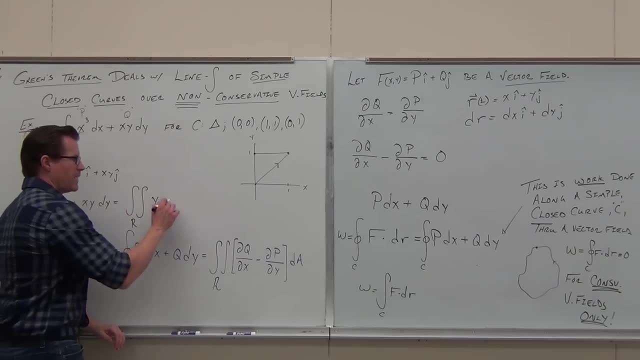 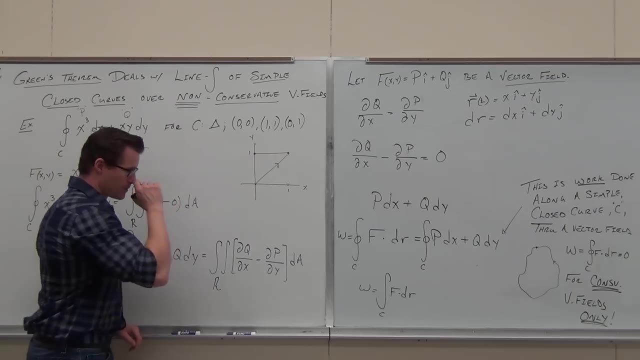 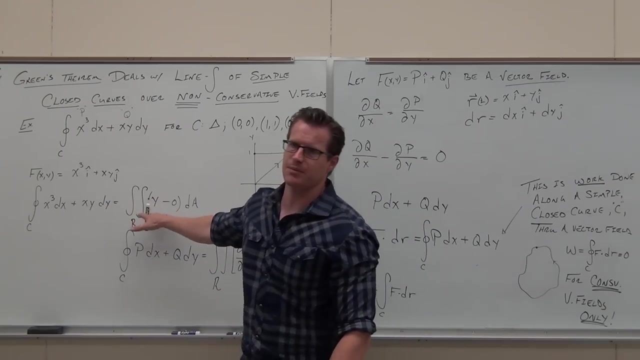 for checking conservative. this with respect to X minus this with respect to Y. What's that? Do yourself a favor. do yourself a favor, do me a favor, because I've got to grade your stuff. okay, Don't ever skip this step ever. 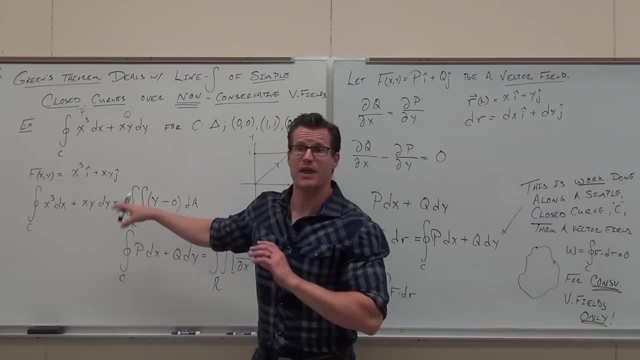 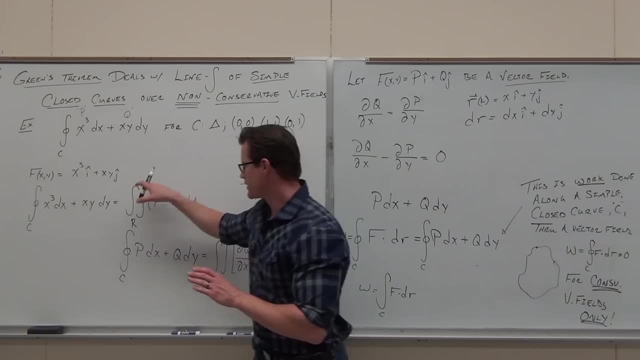 Always, always, write out this to your double integral without worrying about your region, yet Always, always write that out. Can you guys agree to do that for me? Always write that out, Always write out this integral, just like that. Now what's it say? 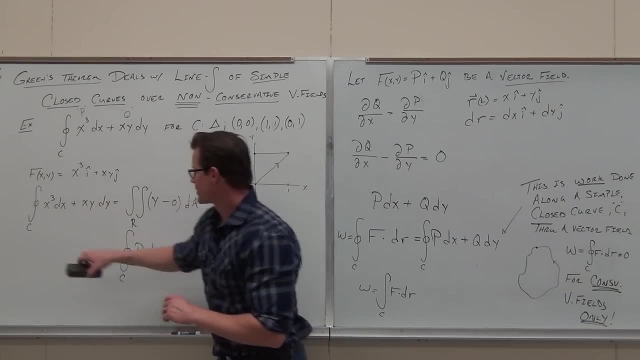 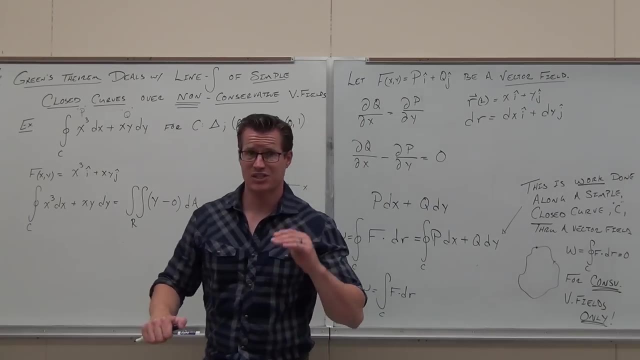 Man, it says something really nice. What it says is that this line, integral or simple closed curve- is equal to the double integral over the region that it contains. Hey, now if I had stepped back an entire chapter and gave you this problem with that picture. 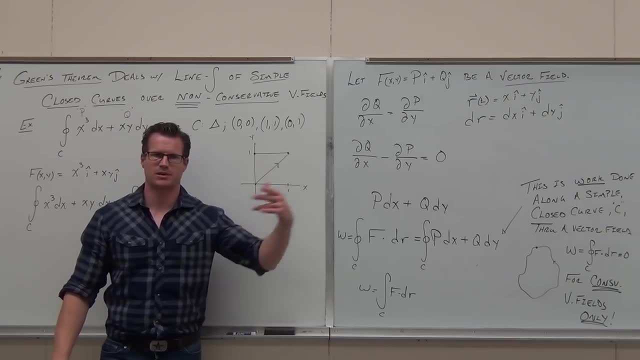 could you do the double integral? That's what Green's theorem does. It takes us back to a chapter, So it goes: hey sweet. That's why we don't skip the step. It says this is literally just a double integral. 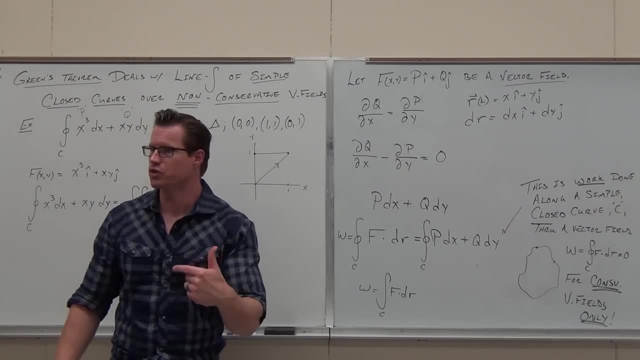 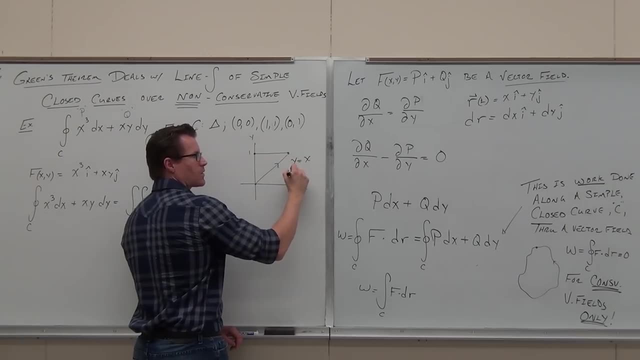 Can you define it? Yeah, I'm going to move quickly here because we should be really really good at double integrals. The first one is: if I'm going from zero zero to one one, my line is y equals x or x equals y. 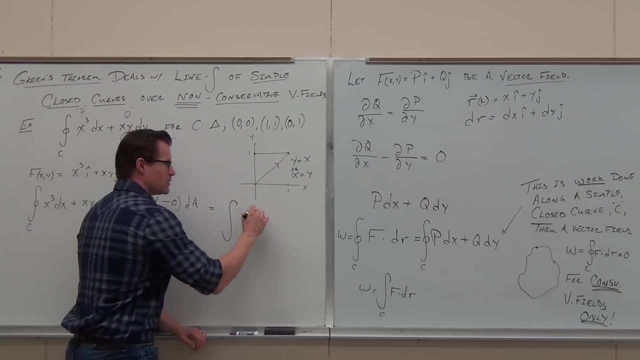 Does that make sense? We'd say: well then, this is a double integral. You know about double integrals because I taught you. We have y in here, You go d what? Well, I don't do the da yet. 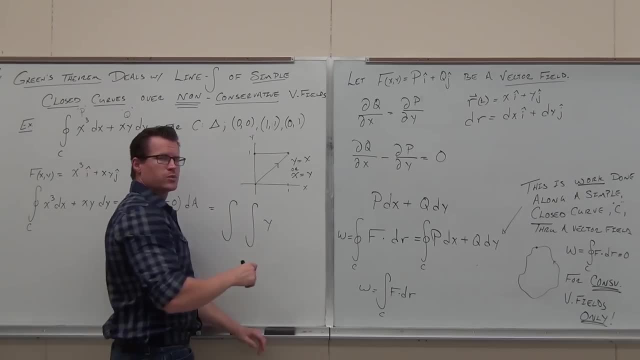 I do the. it's either x or y, but I got to deal with this first. Which way would I want to go? Y first or x first? Y first is between two functions that are not zero. I would go. I would go x first, for sure. 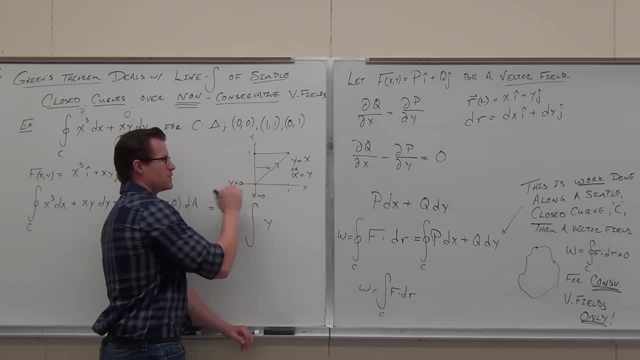 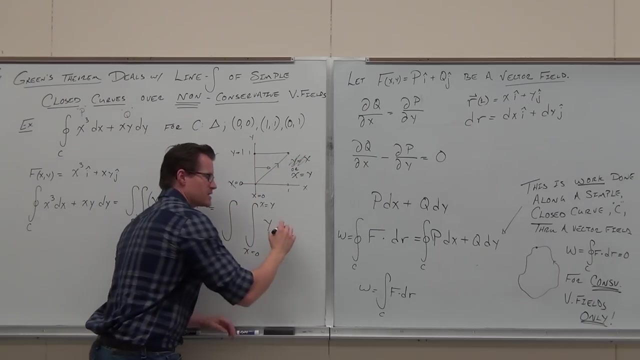 This is x equals zero. This is y equals zero. This is y equals one. I would go from x equals zero to x equals y. I'd ignore this one. I want x, and that means I'm going to do dx. Is this ringing a bell for you? 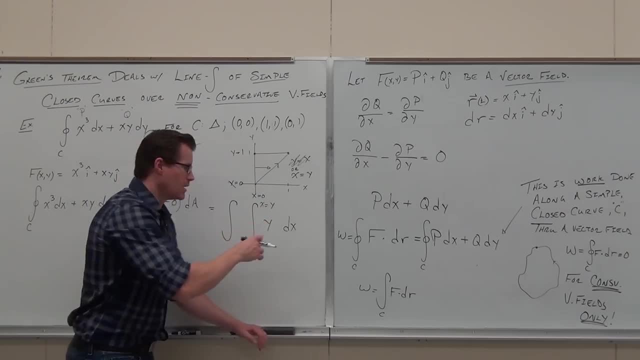 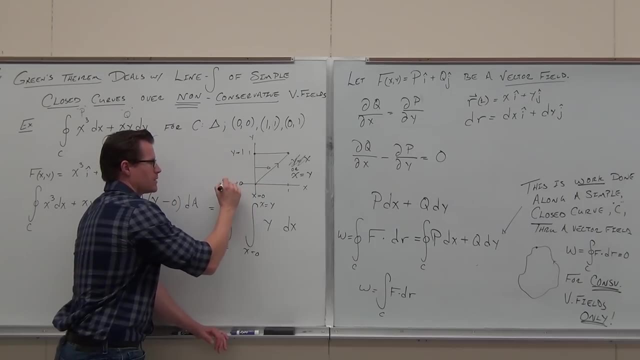 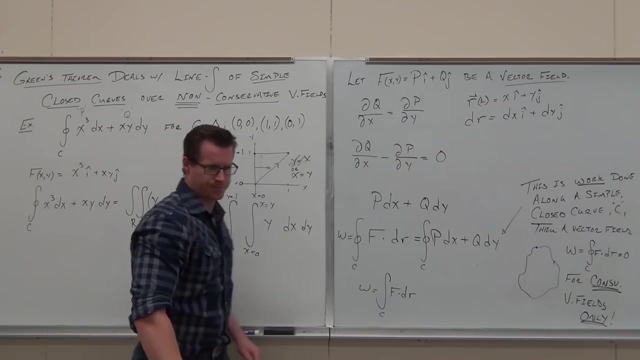 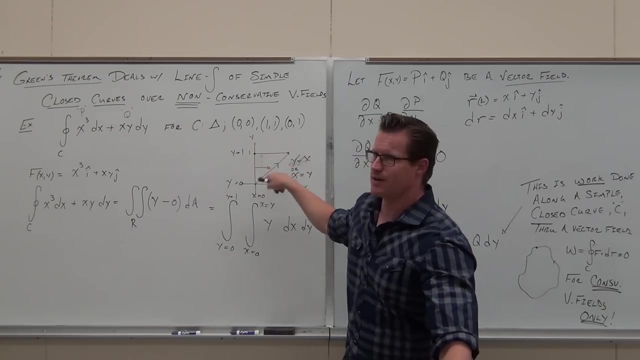 I don't have time to reteach double integrals. Are you guys okay with that one? Then our y's would go from From where to where. Yeah, the rectangular numbers. there is zero to one. That's it. D y, So r, that region, r is now just the inside of that thing. 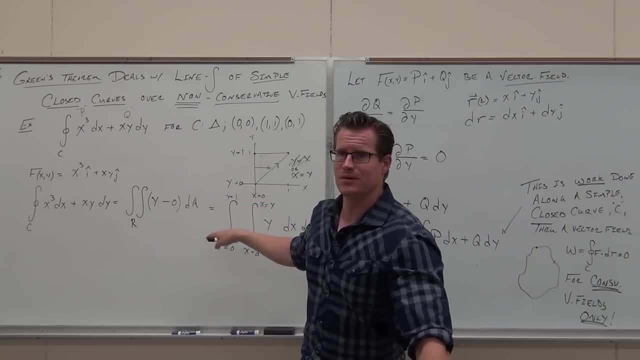 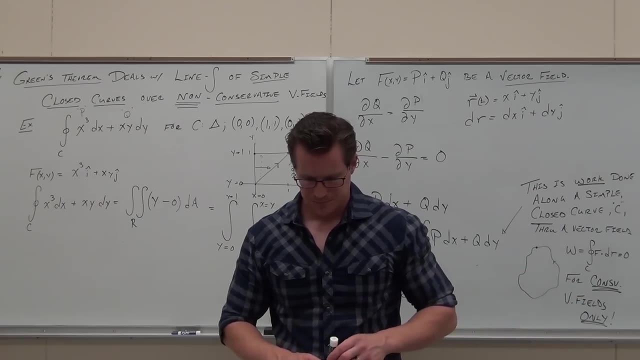 that space that you're containing. Can you do this? It's integral. Go for it. See if you can do it. This is like the one that we're going to do. Ah, something on my mind, I forgot it, I don't remember. 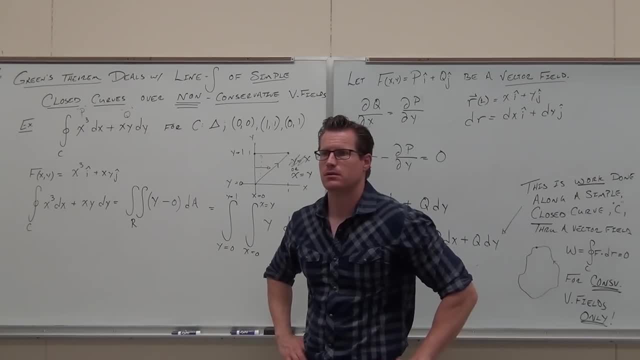 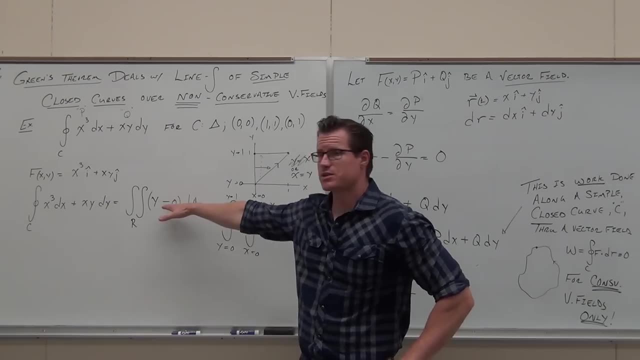 Oh, I had it. Is f conservative? No, Is f a conservative vector field? No, Why not? What would it be for zero? This would be zero, and then you'd be done. You'd say, hey, zero, conservative vector field. 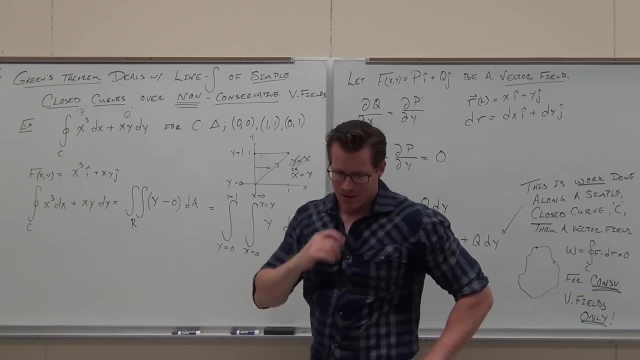 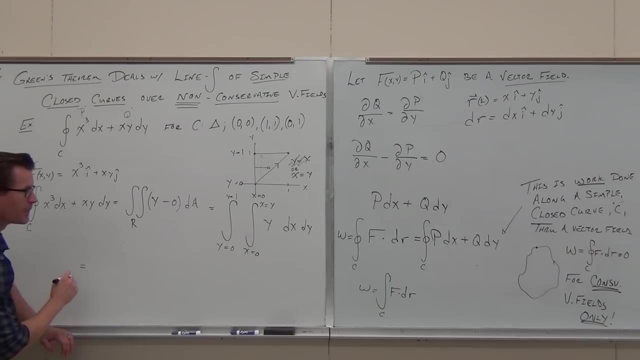 simple plus curve done. Does that make sense? Kind of cool. Let's see Zero to one. let's see, here We'd have x, y and we're plugging that in, for x equals zero and x equals zero. 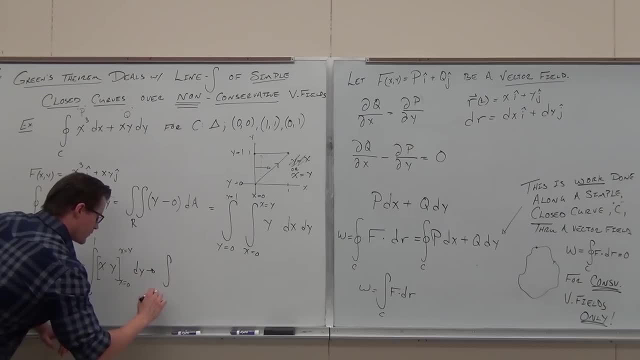 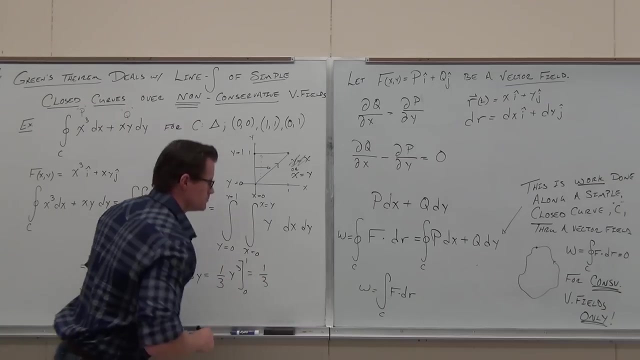 Y equals y, and then we've got that dy hanging on. So integral from y equals zero to one, and we have y squared. dy Looks like one-third y cubed from zero to one one-third. We haven't had one that nice in a long time. 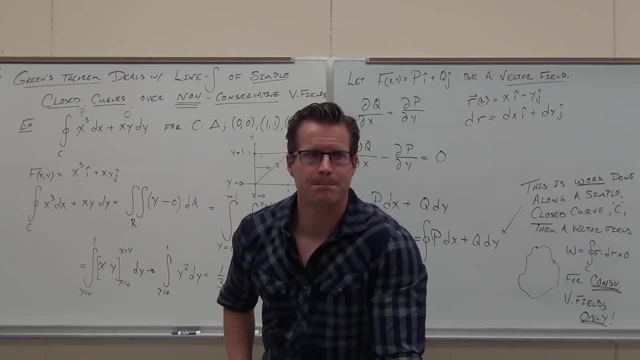 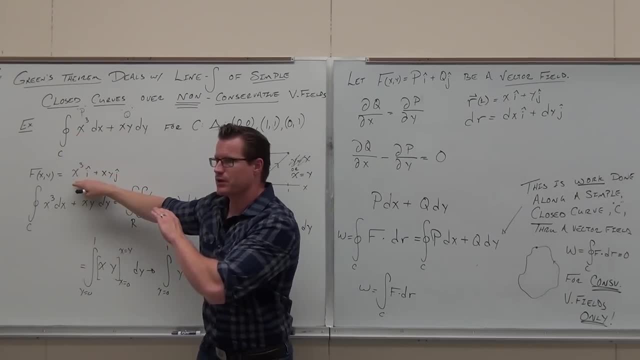 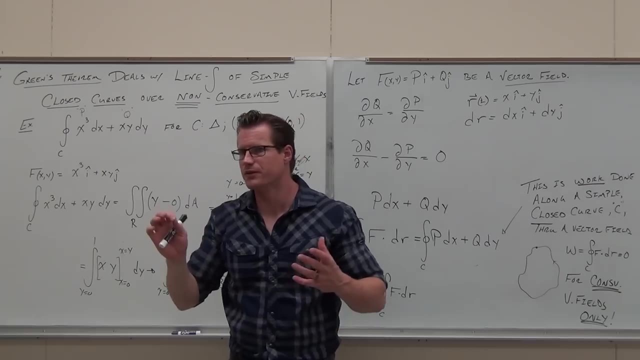 Through that vector field that you could find right, Just from your line interval, Through that vector field on a simple close curve, This particular simple close curve, So moving a particle around that curve, one loop, if you will, in a counterclockwise direction. 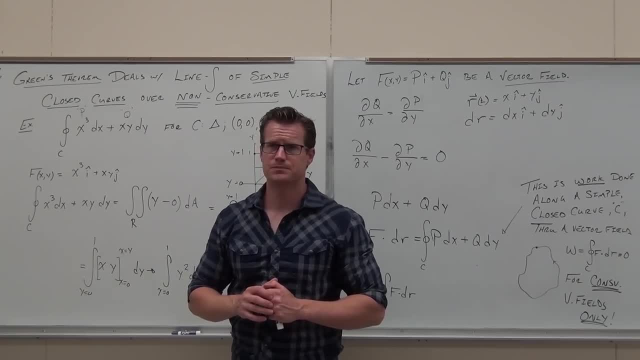 That's what's happening here. Are you okay with it? What happens if we reverse directions? It'd be negative. Just a sign of a change. That's what happens if we reverse directions. Also, one more thing: If this equals zero. 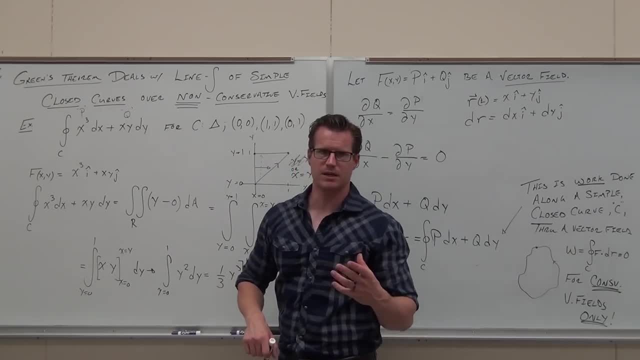 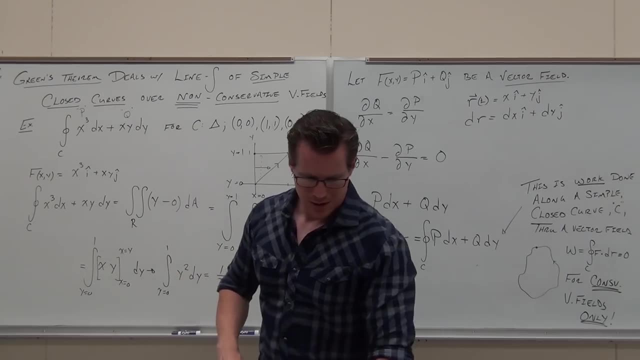 It does not necessarily mean that you have a conservative vector field. That would show up right here. So if this thing ain't zero, you don't have a conservative vector field. Is this all making sense to you? Are you guys okay with this one? 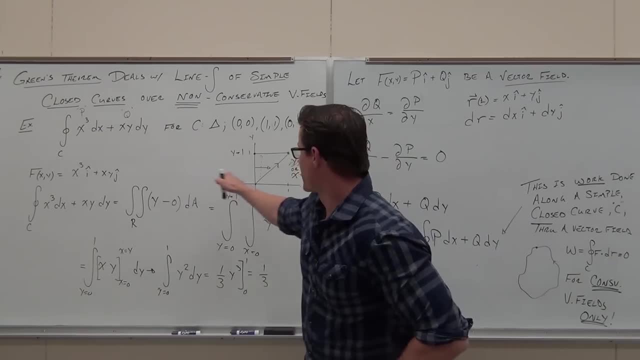 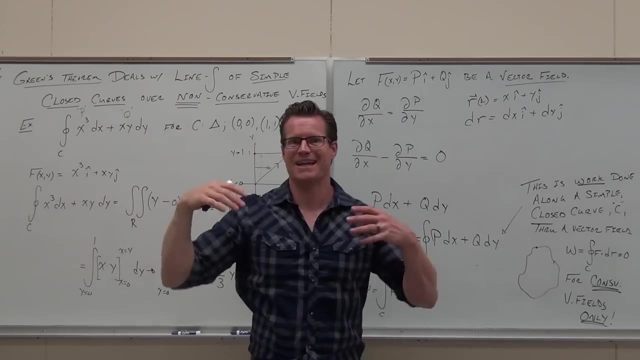 By the way, could you have done this a different way? Could you have re-parameterized these three segments, done three different integrals by re-parameterizing this three different times and added them all up and got one-third Yes, Would it have sucked? 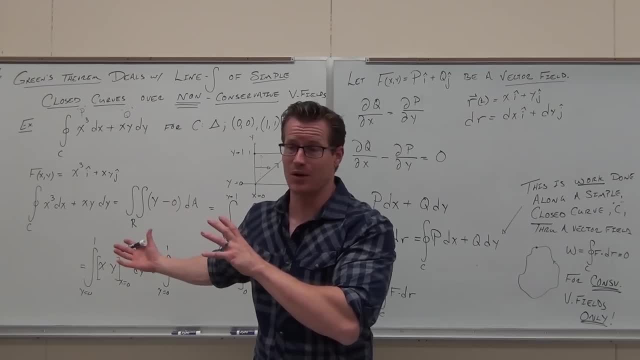 Oh my gosh. yes, Do you have any questions? Do you have any idea how much headache I am saving you or how much headache green is saving you here? It's a big deal. It's a cool theorem, Is it hard to do? 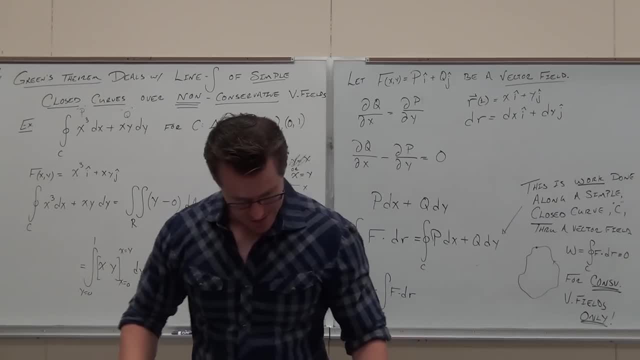 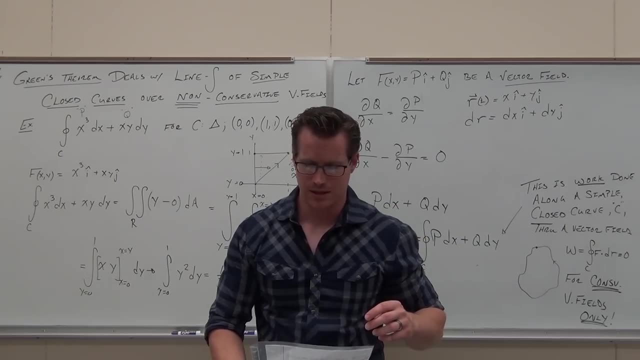 I don't know, Was that hard? Not really so much. Tell you what. Let's do. one more example and then we're going to take our break. By the way, if you're asking, well, if you're asking, why in the world didn't we do this before? 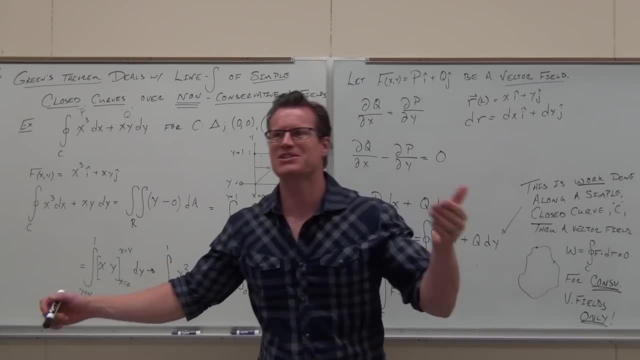 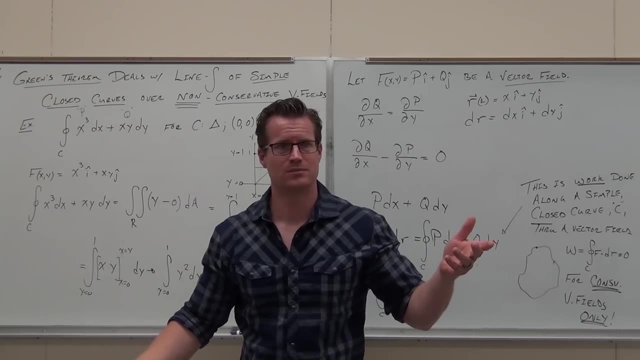 Why didn't we do this before? This is so nice. Why not? Why didn't we do it before? Good, We weren't on the section Very good, Why really didn't we do it before? It only works for simple closed curves. 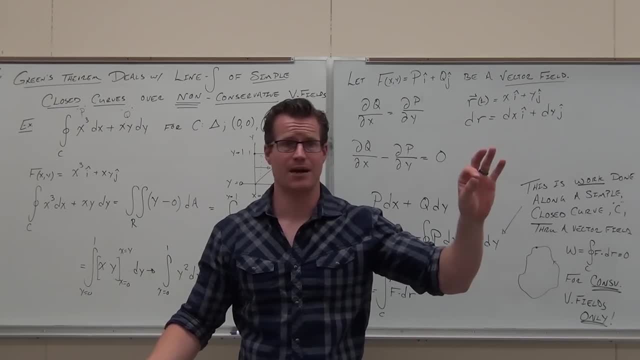 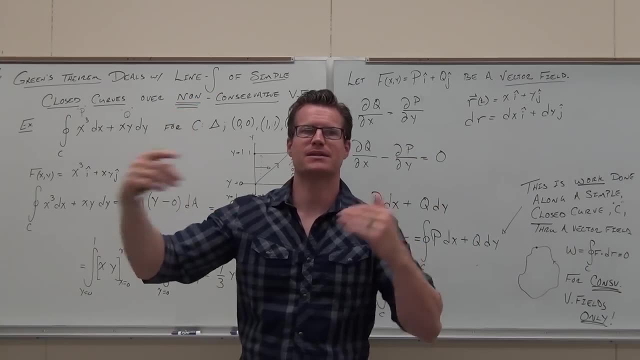 It does. It only works for simple closed curves, And two sections ago we didn't have those. We just had segments or we had things that were not connected. It wasn't a connected region. And then in the next section we had conservative vector fields. 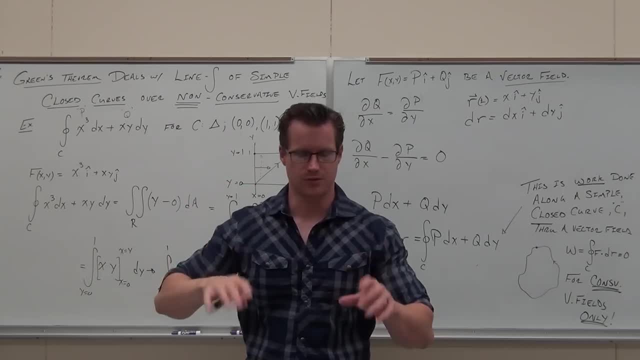 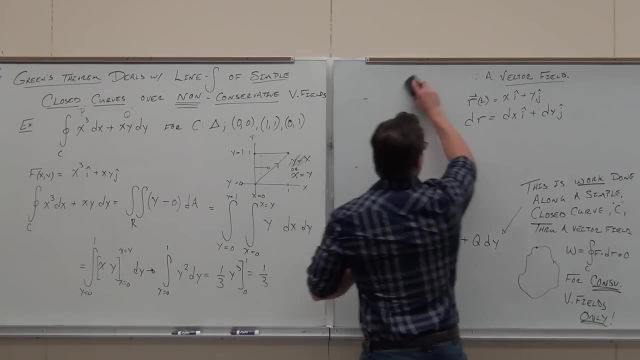 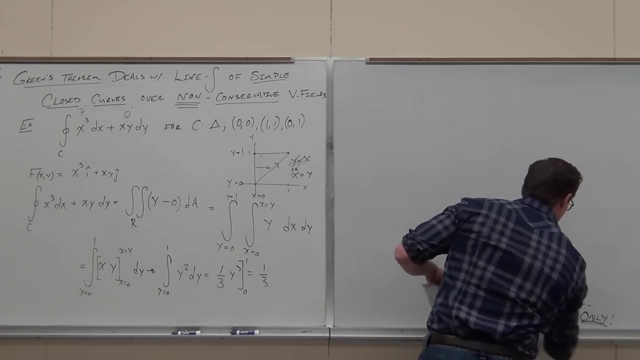 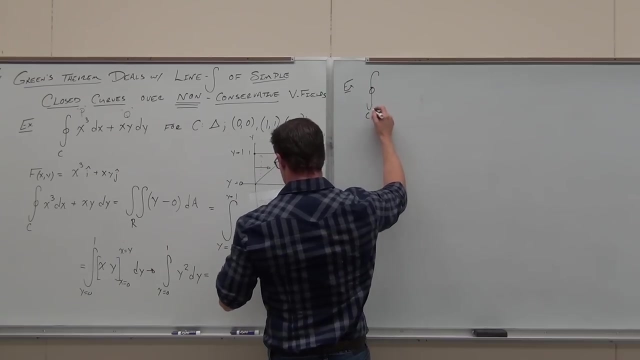 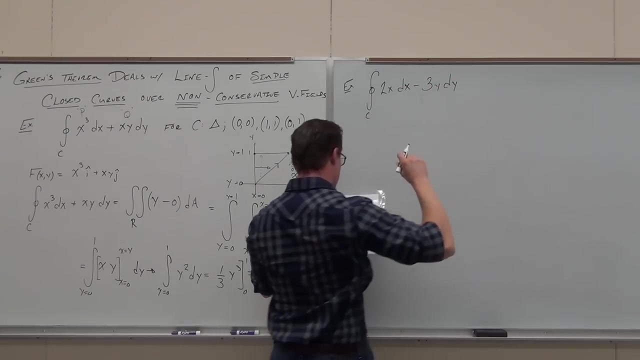 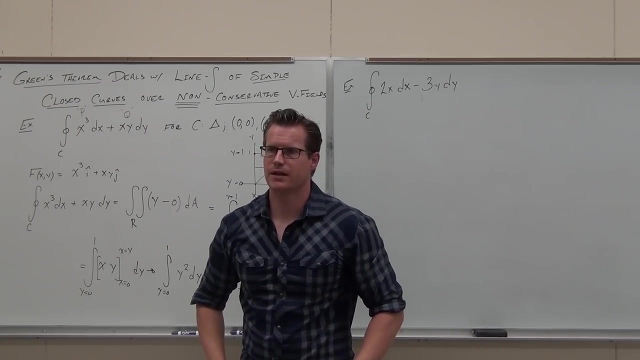 So this is dealing with things that are connected, but non-conservative vector fields. That's why we didn't do it. How about the last one and then take a break? This is going to take about 30 seconds. I want you to find the line integral. 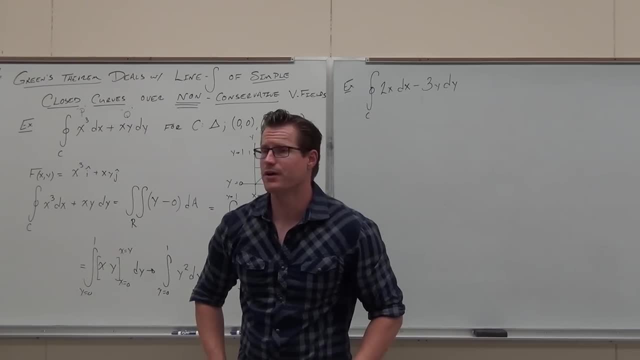 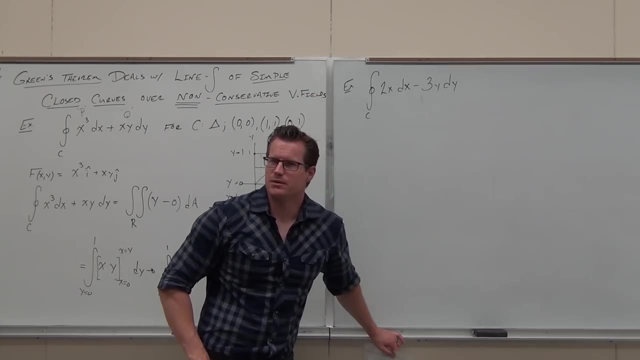 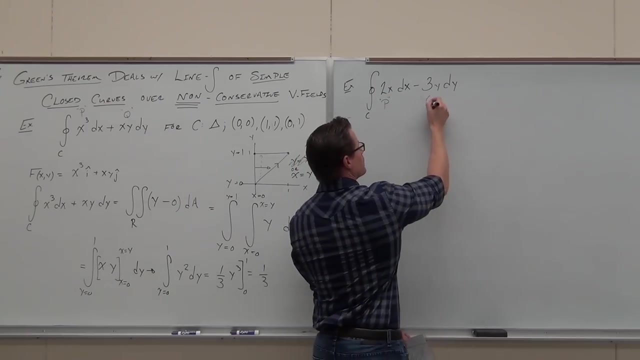 for that vector or through that vector field over any simple closed curve? Can you identify what P is? Can you identify what Q is? This problem is here for one reason: Make sure you actually got something about what I was just talking about. 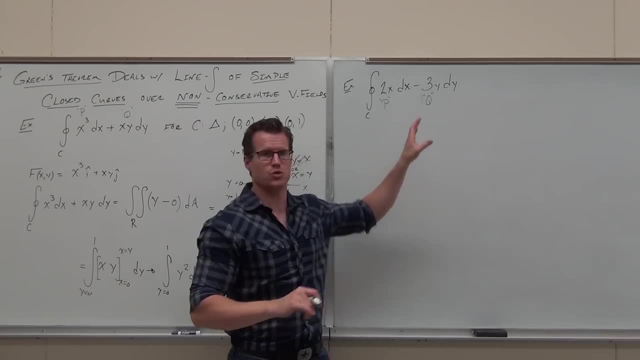 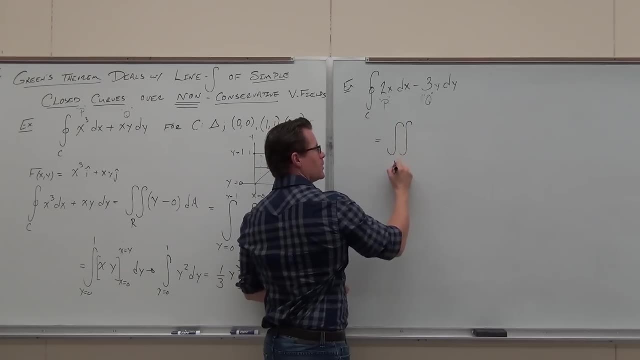 Is Green's theorem going to apply If I tell you it's a simple closed curve, is it going to apply? So this would equal a double integral over region. Don't ever skip this step. Do not go directly to identifying the region. 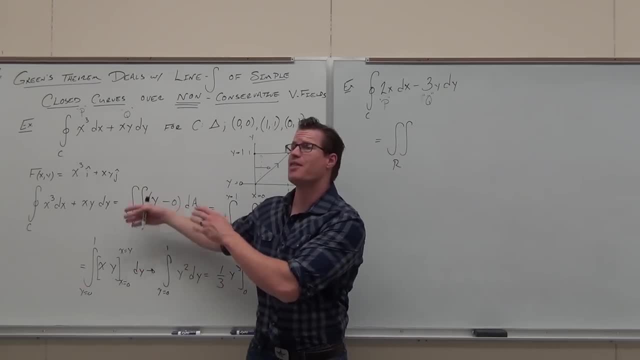 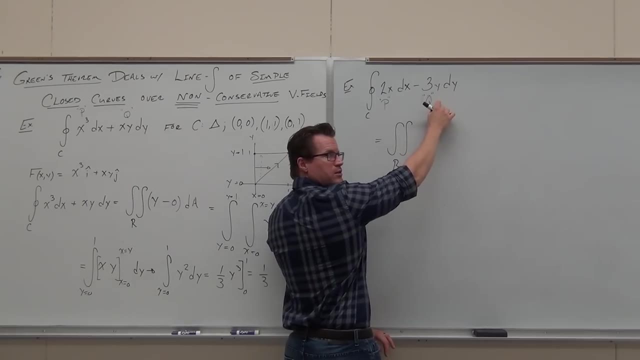 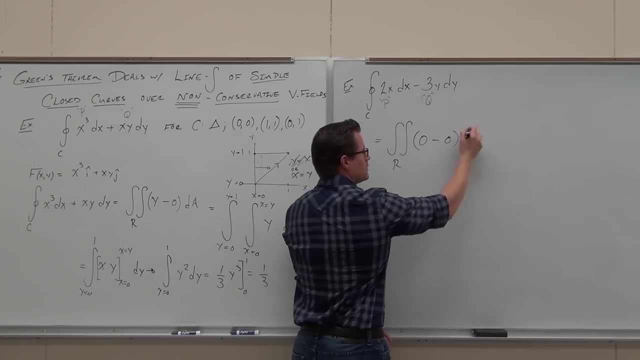 because sometimes you can save yourself a lot of time by just identifying this and then working on your region. I would find the partial derivative of Q with respect to. I would find the partial derivative of P with respect to. I would find the partial derivative of Q with respect to. 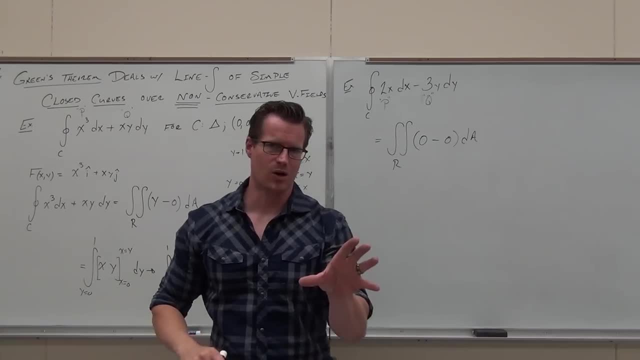 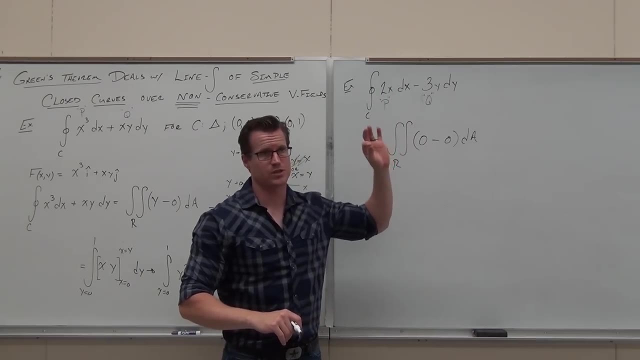 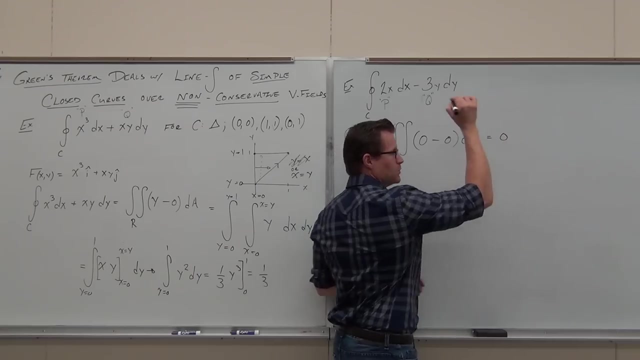 tell me something right now about that vector field. Tell me something about a line integral that's a simple closed. oh well, so a line integral for a simple closed curve over a conservative vector field. You don't work this, do you? 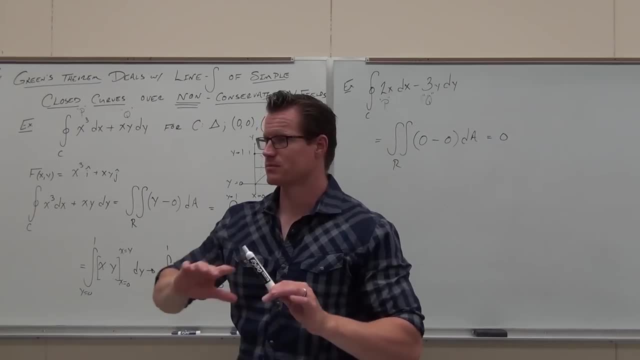 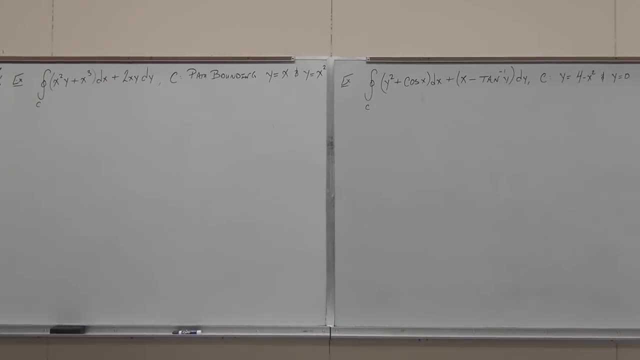 Oh, 0.. Pretty easy. So when that happens, 0.. I'm going to take a break and come back in a bit. So for right now we have a whole lot of practice on how to use Green's theorem. Again, Green's theorem says: hey, simple, closed, you all right. 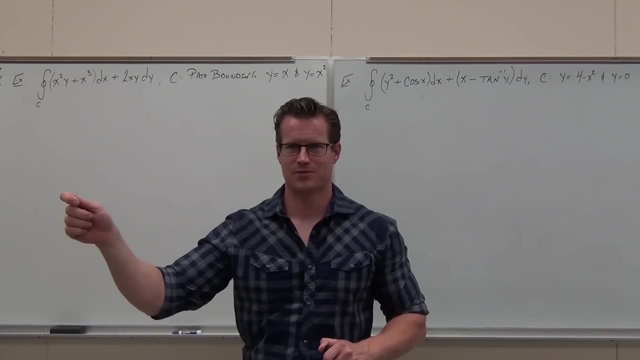 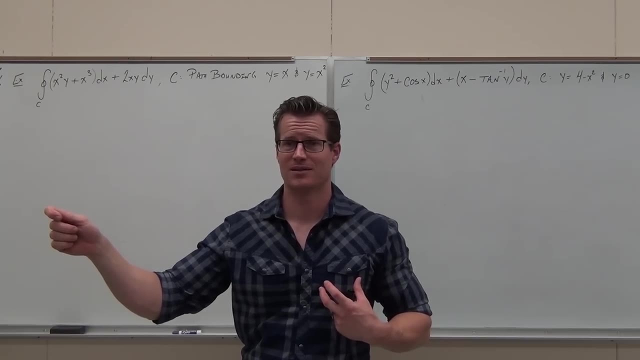 Good. so I'm going to give a heart attack. Jeez, warn me. all right. Freaking goodness, I've got too much caffeine and my heart is thumping. No, it's not good. Back to normal. I've got to breathe. 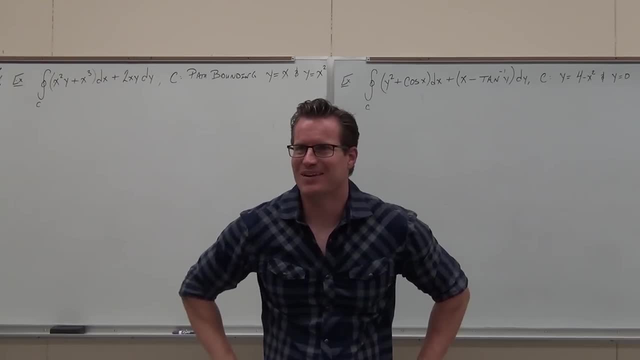 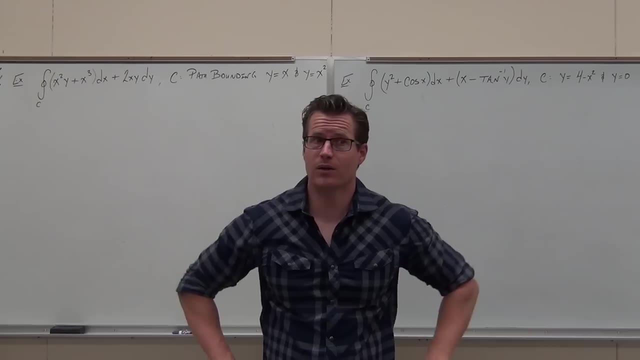 So what was I even talking about? Green's theorem: right Happens over simple closed curves. Does it matter if they're conservative or not? Not really. It only is really relevant for conservative. but don't even worry about it. 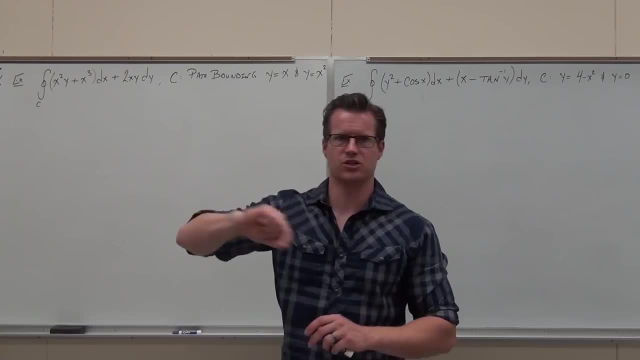 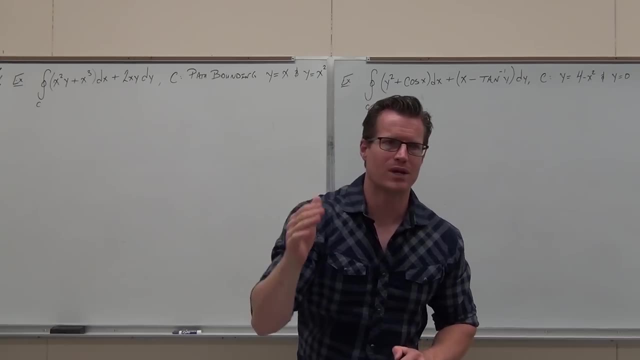 All I really want you to worry about is that the curve encloses a region that you can define. So your number one step right now is: you look at that curve and you draw the region every time. Why- Why would you draw the region every time? 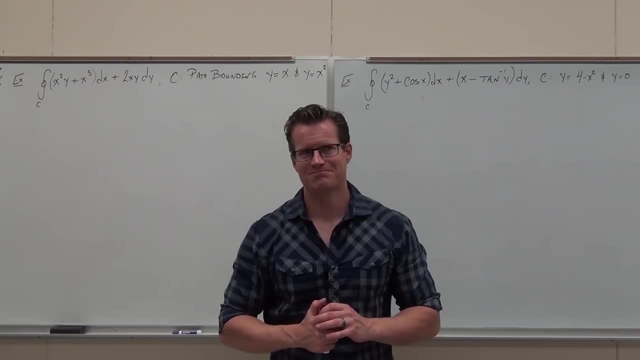 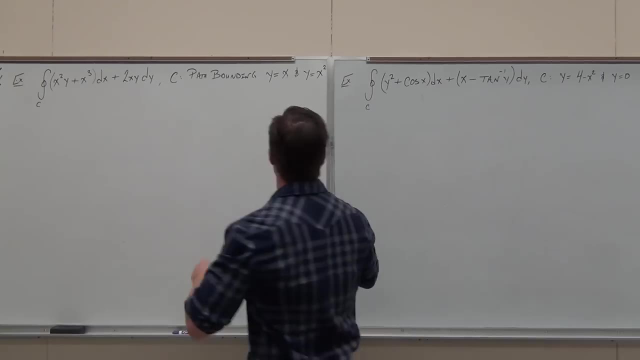 Because I told you. so Why would you draw the region every time? So you can set up your double integral and to make sure it's a simple closed curve. Does that make sense? So draw it. So when we draw it, So when we draw this, and listen, I'm not going to spend a whole lot of time doing it. 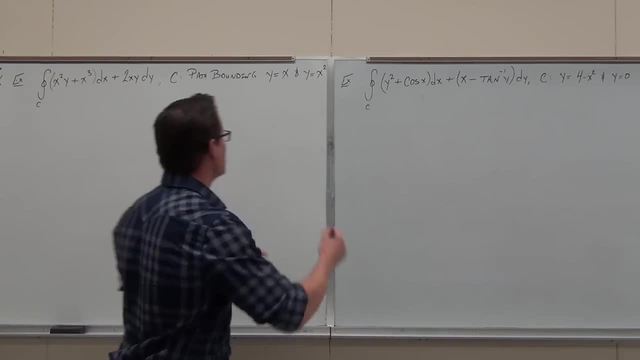 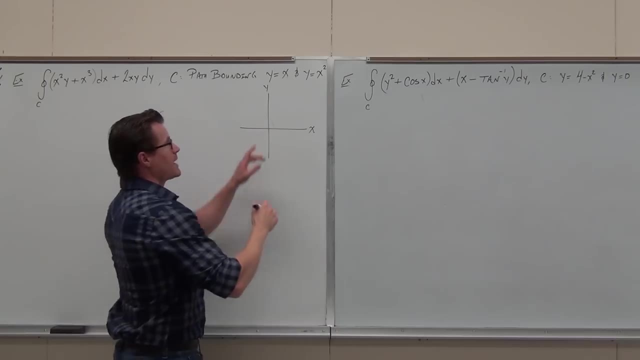 because we've done, we've killed double integrals, Like we've been up to death. So we're going to go really fast on this stuff. but of course, if you have questions, you let me know. So this says that I have this pathway that's bounding these two curves. 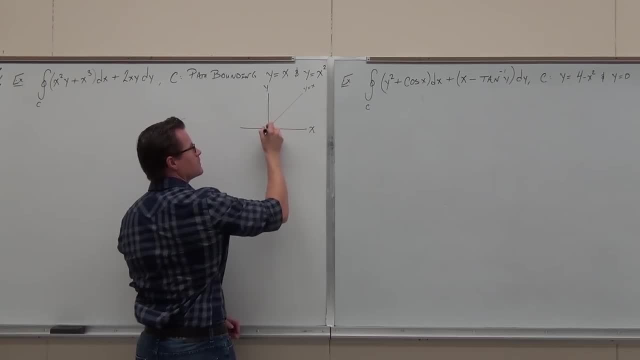 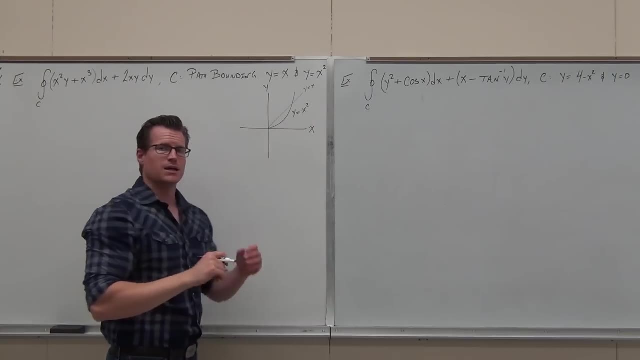 There's y equals x. Here's y equals x squared. If you were to do the intersection, these things intersect at 0, 0 and 1, 1.. We're just focused on one loop Again. simple, closed curve. 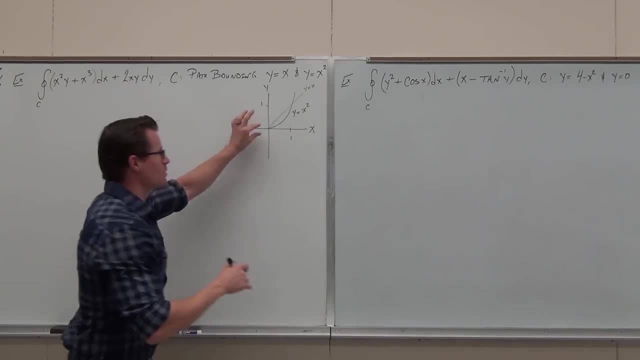 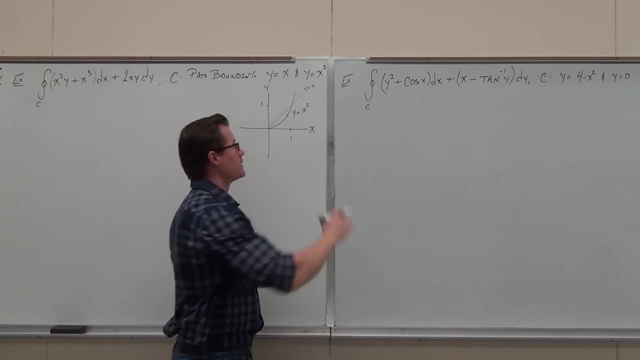 Hey, it's got to be simple, right. It can't cross, which means it can't go down here, Otherwise it wouldn't be simple. We'd have just this one and we're going around the loop like that. Can you guys picture the loop that we just created? 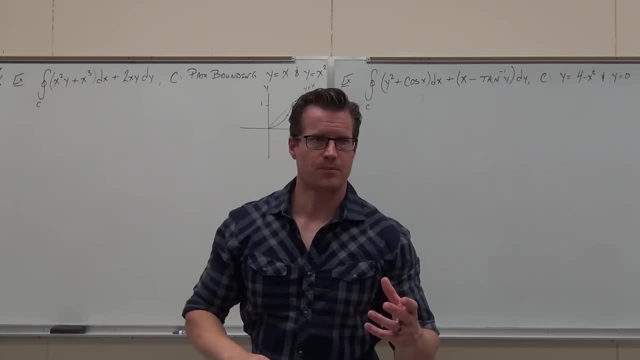 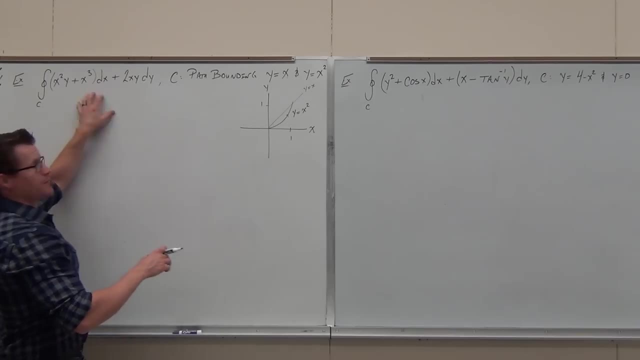 Head nod, if you can. Okay, Is it a simple closed curve? No, Simple closed curve. Yes, Does Green's theorem apply? Yes, Let's set up Green's theorem. What Green's theorem says is that this the work done of this line integral. 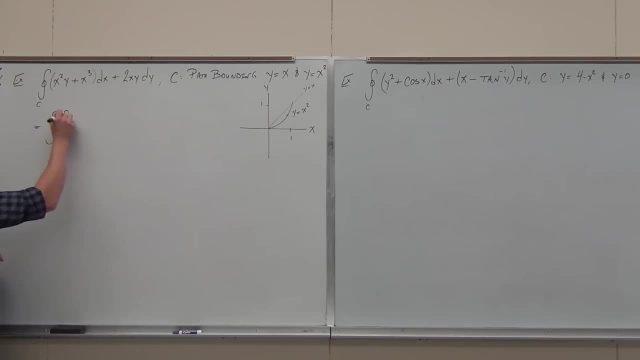 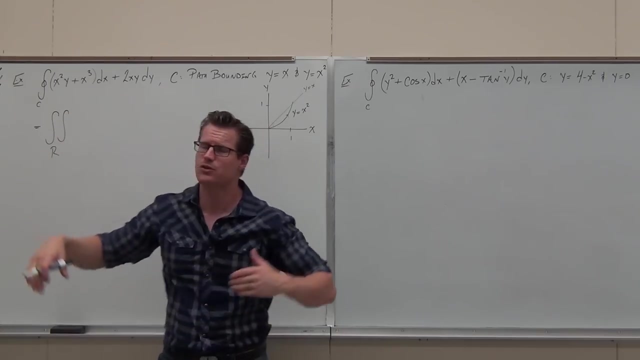 of simple closed curve is equal to the double integral over the region that it contains, this region. Don't skip this step. Write this every time, Even if you know what the region looks like. you write it every time Because I want you to deal with the pieces in here before you start setting. 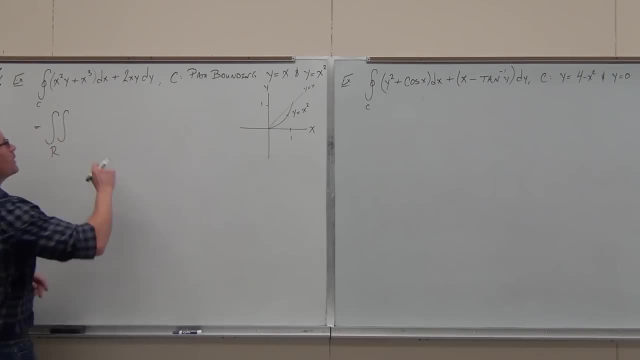 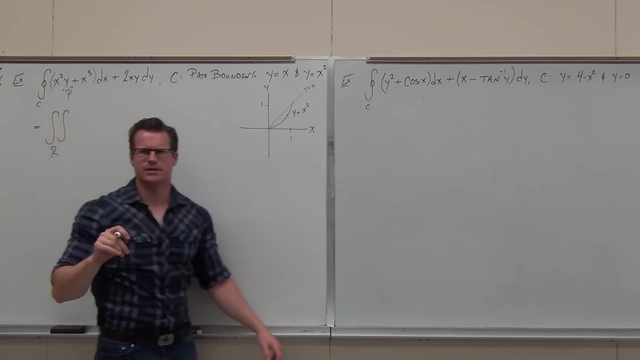 up the double integral. okay, I want a two-part setup. What's your piece? B here, by the way, B here, by the way? Did I mention to you? I don't know if I did. did I mention to you? 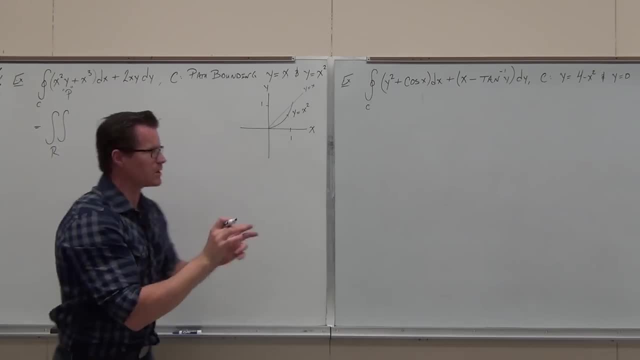 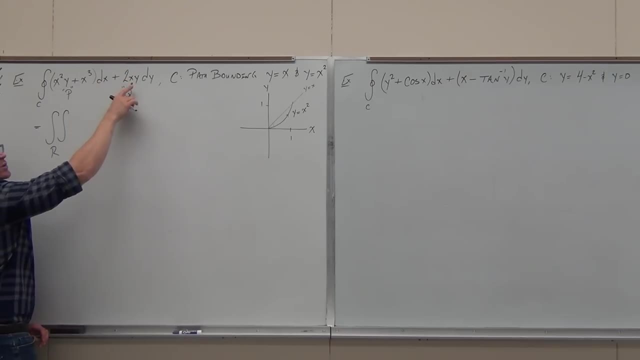 that sometimes they flip-flop these things. label P and Q every time. That way you don't accidentally waste a whole lot of work. So the partial derivative of Q with respect to what- Excuse me, 2y Yes, Minus the partial derivative of P with respect to. 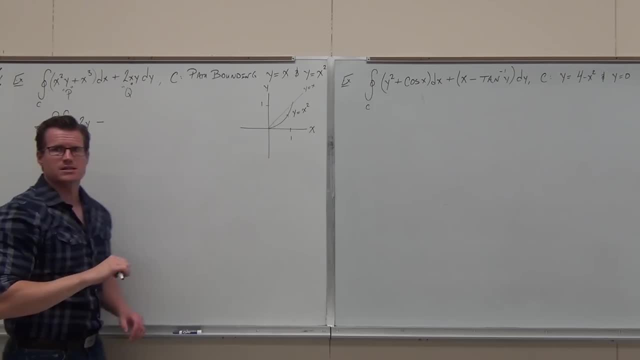 It's easy to get it confused. It's the y with the x, it's the x with the y. So partial derivative of this with respect to x is 2y. Partial derivative of P with respect to y is That's it. 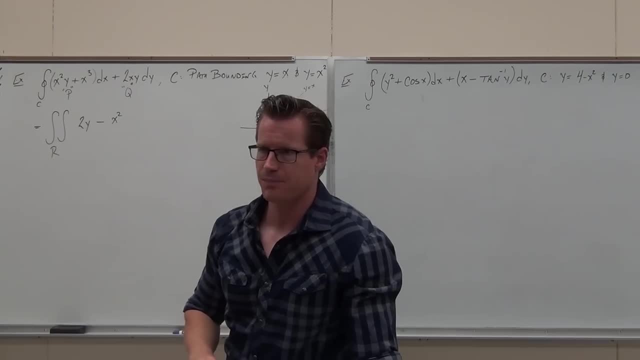 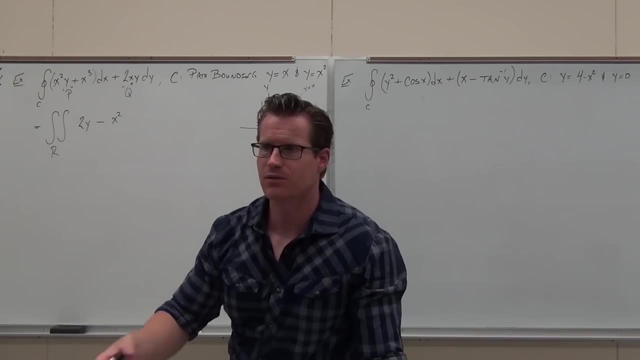 Also, if you haven't noticed this yet, if you haven't noticed this yet, there's no reparameterization at all. Green's theorem takes care of all of that. You don't need a t, You don't even need a vector function. 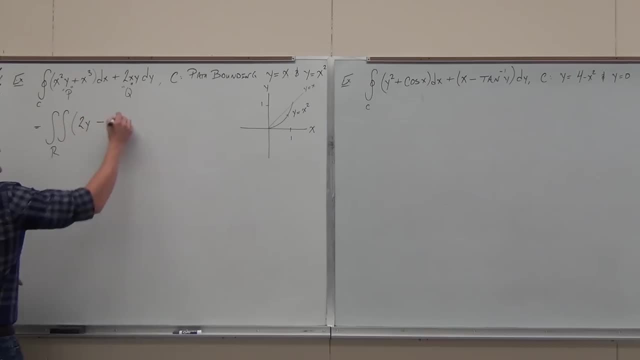 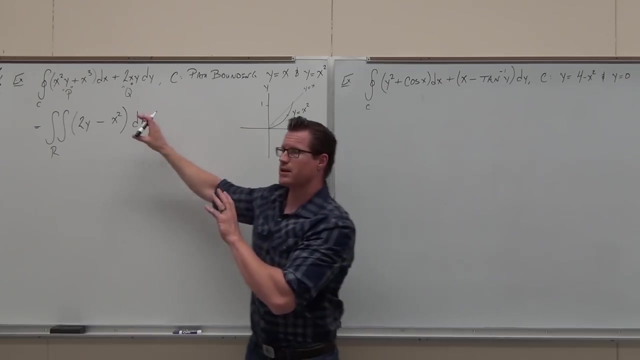 It's done for you. It's so nice, And this is d a. Don't ever skip this step. This is number 1, and then you use the region that you just drew to fill out the rest of it. Let's try that right now. 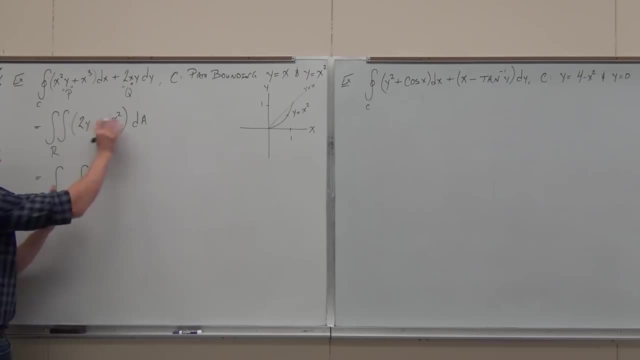 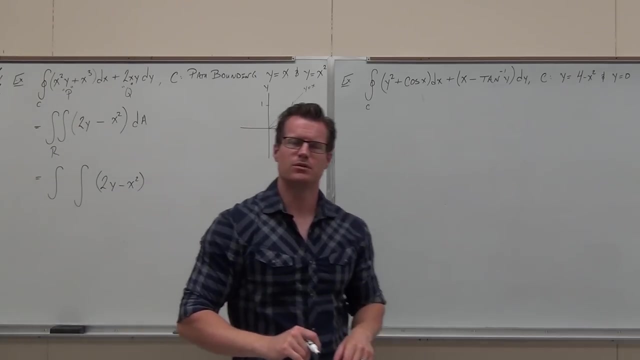 So I'm going to keep the inside of this. I'm going to leave this alone. I'm going to look back at my region. What would you do? Would you go along the y direction or the x direction? What do you think? 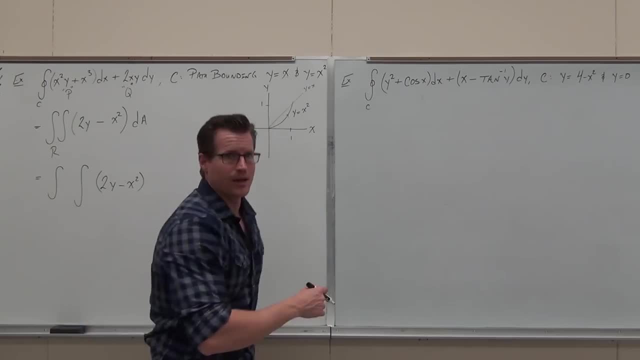 I'd go y simple first, because they're already solved for y. Does it really matter? No, But if I had to solve them for x, I don't really want to do that, So I'd go here first. The region: this is why we draw it. 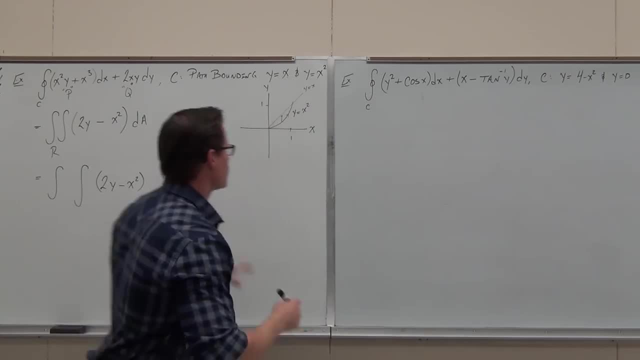 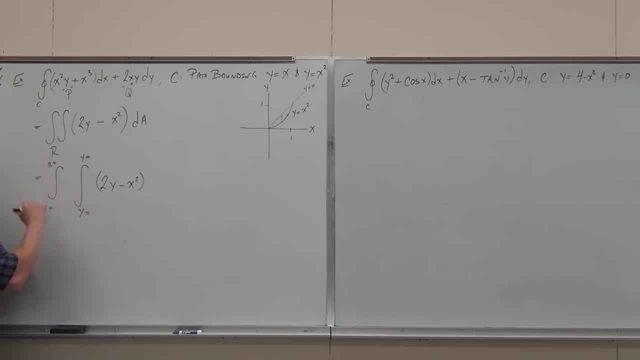 It always shows us what's on top, what's on bottom and where to go. It's really nice. So our y simple says: I need y equals and y equals, x equals and x equals, And I'll be going d? d, what. 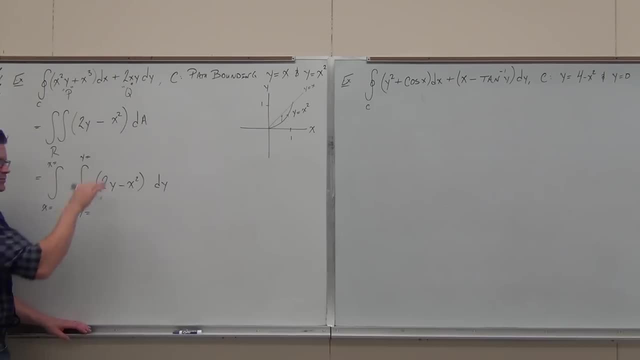 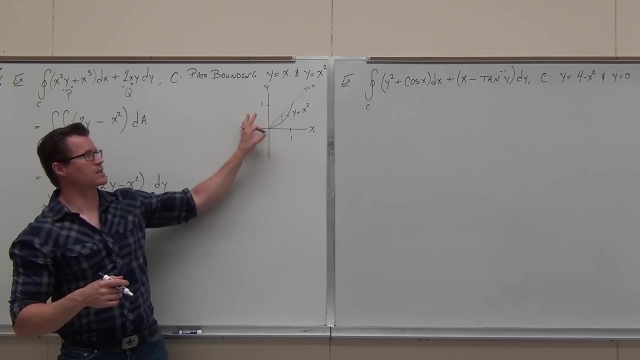 Dy, dx, Dy. What's the smaller function, X squared- And the larger one, X? Perfect, It matches up. We're going from y equals x squared to y equals x. That's the region that's enclosed by our simple closed curve. 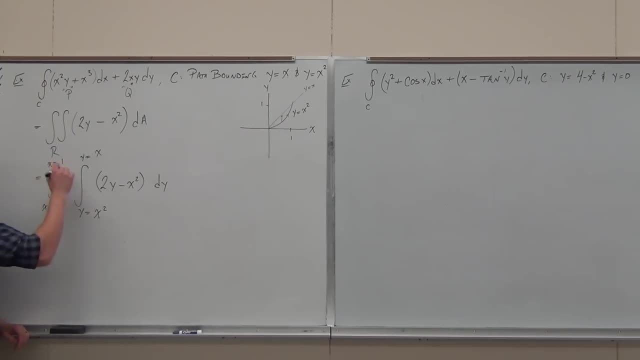 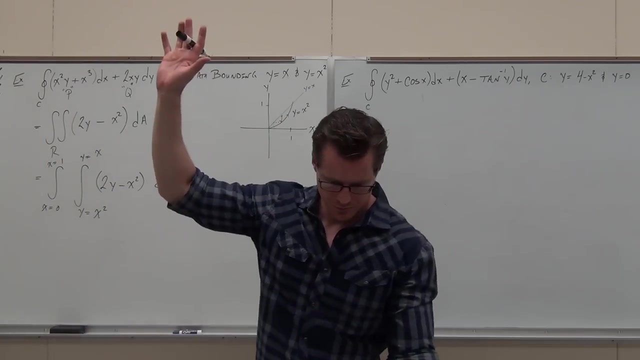 And then I'm going from x equals what to what please, 0 to 1.. Across this way from the constants 0 to 1.. So your fans feel all right with that one. Yes, no, yes, Yes. 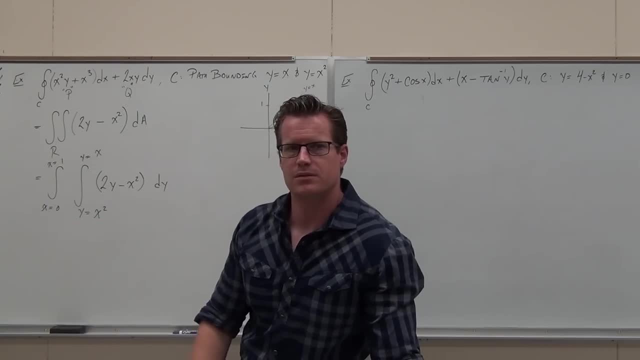 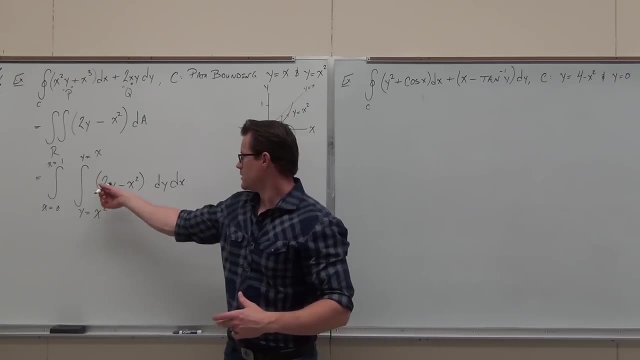 We're going to leave a lot of them just set up. Would you know what to do after this Integral with respect to y first, so you get this: Y squared Y squared minus x squared y. you plug in for y, distribute, do dx plug in for 0 and 1,. 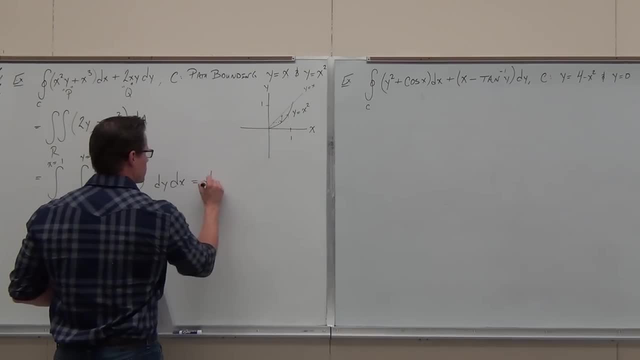 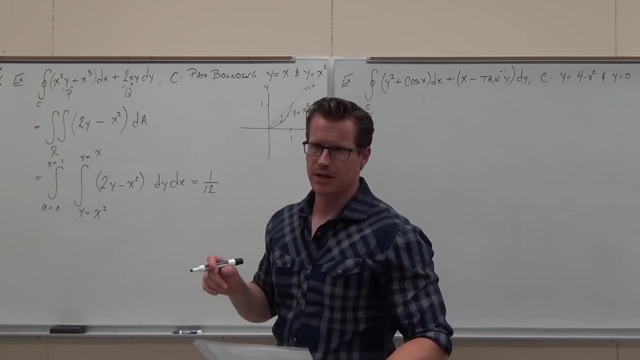 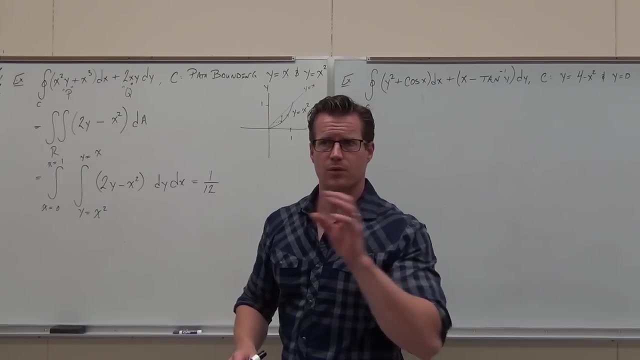 and hopefully get 112.. Work done, Work done. By the way, if I asked you to, if I asked you to do an interpretation, I would ask you for something like this: Tell me what you did. You'd found the. what does that give you? 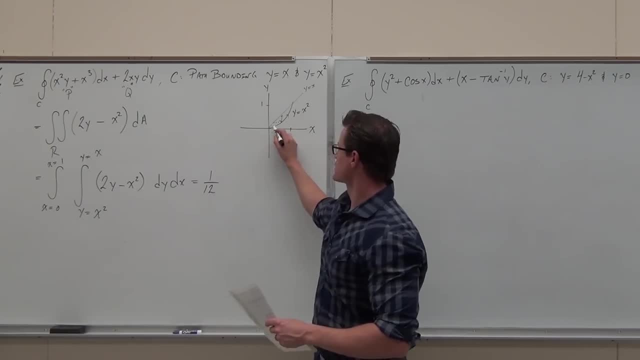 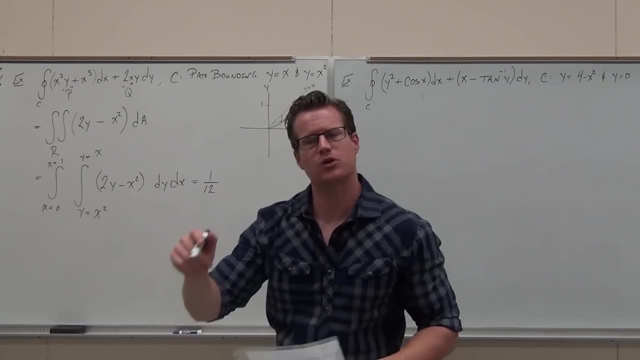 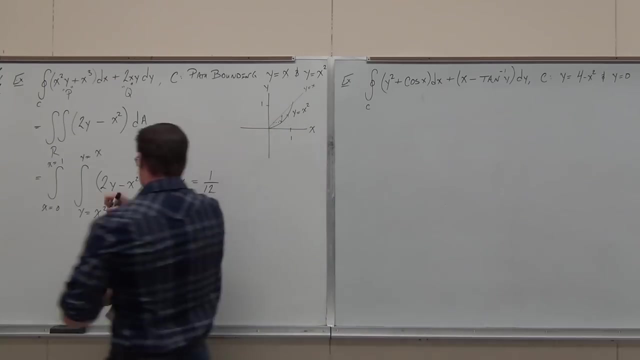 Work, Work done along this simple closed curve Through what? What vector field? What vector field? That's the point. What vector field? Could you find the vector field from this? Yes, Yeah. So this is the work done along this simple closed curve through the vector field, which is just p, i, q, j. 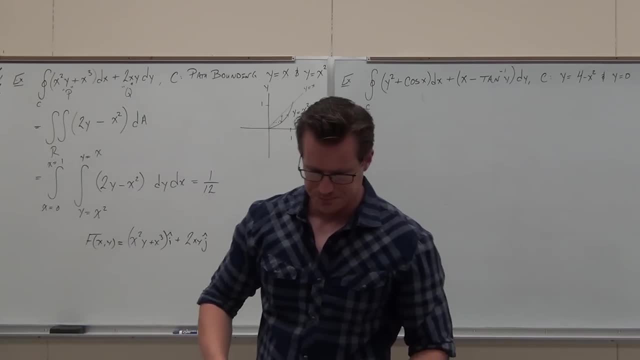 And that's what we're doing, That's what we're interested in, That's what this theorem does, And that is what we are doing. Ladies and gentlemen, is it making sense to you? We're going to kind of crush probably three, four examples here. real quick deal with something. 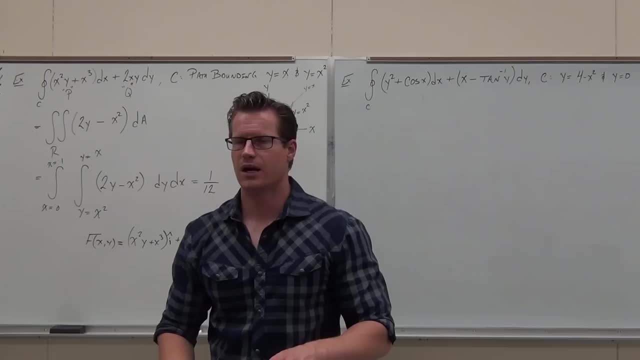 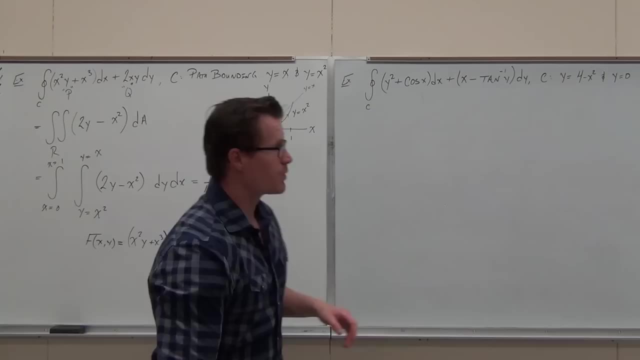 kind of really interesting. We're going to prove the formula for area of an ellipse, which you probably haven't seen before, So we'll deal with that And then we'll probably have to call it a day after that, But we want to get through as many as we can. 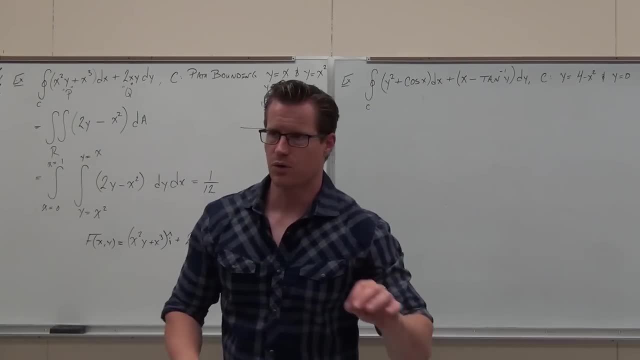 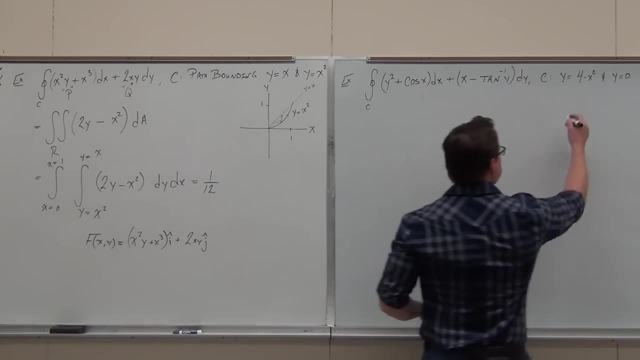 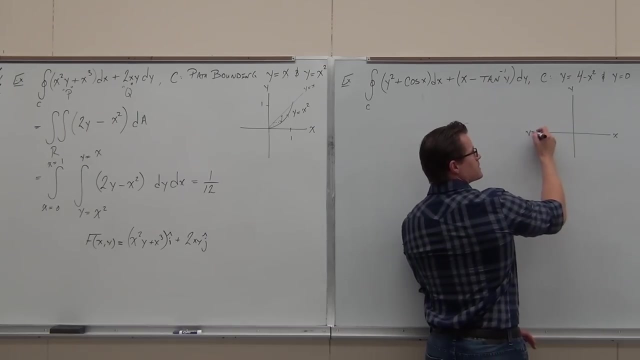 So, firstly, what's the first thing you do every single time you're given a line integral And I tell you that, What are you going to be doing? Draw the curve, Draw the curve. This one says that y equals 0.. 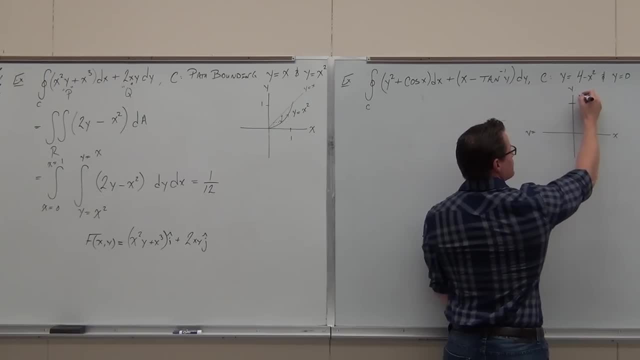 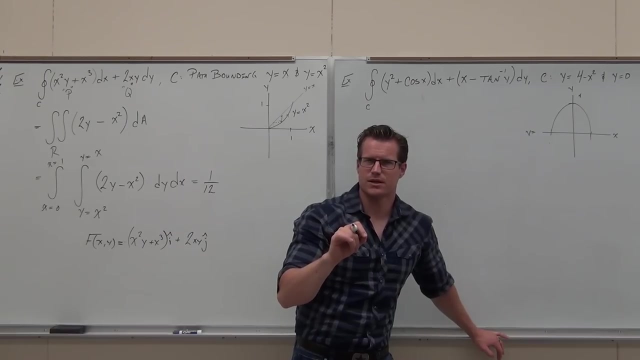 That's the x-axis. That's fantastic. This is a parabola that has a y intercept of 4 opening downward. Do you know or could you find where that intersects the x-axis? Where does it intersect the x-axis? Good, 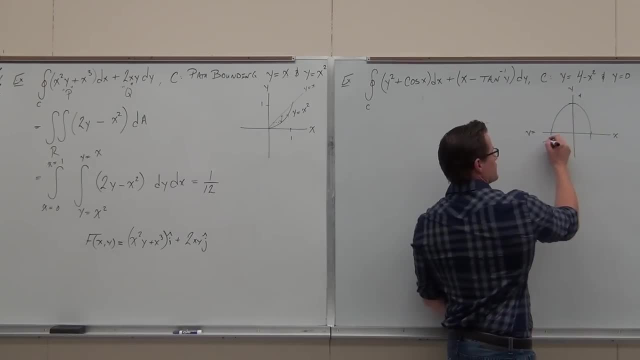 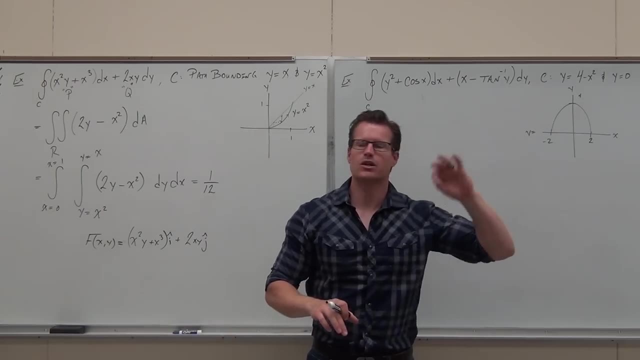 If you said these equal to each other, we'd find the intersection. This is negative 2 and positive 2 and x-axis. I don't know if you're OK with that one. Hey, does that region enclose a simple or is it enclosed by a simple closed curve? 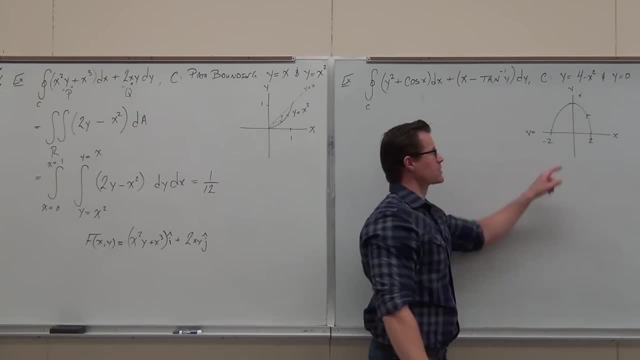 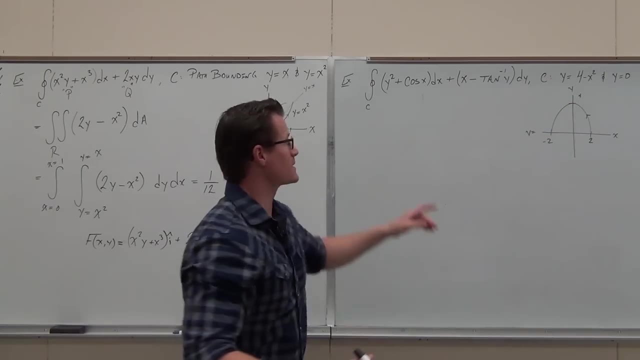 Yeah, that's fantastic Show. it's a simple closed curve. It's going right around there And we have a region right inside of it. I want you right now to try to set up Green's theorem, Since this is a line integral over a simple closed curve. you've drawn the curve. 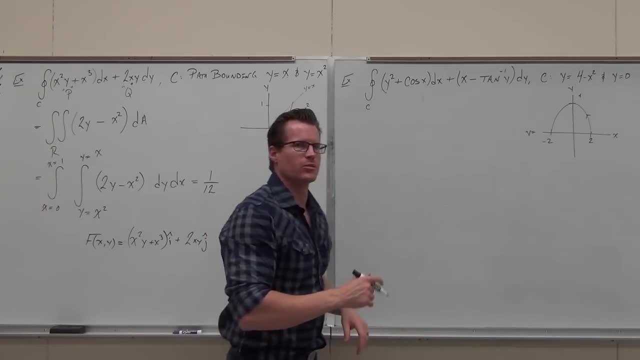 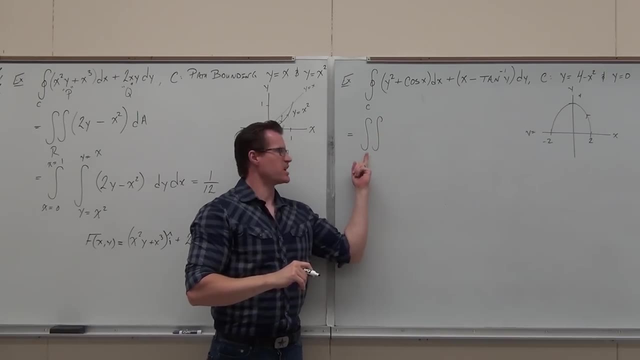 We already have the region. It's fantastic. Just do Green's theorem, Let's set that up. So our work is going to be equal to a double integral. What do I put right here for right now? Just right now, Just put R. 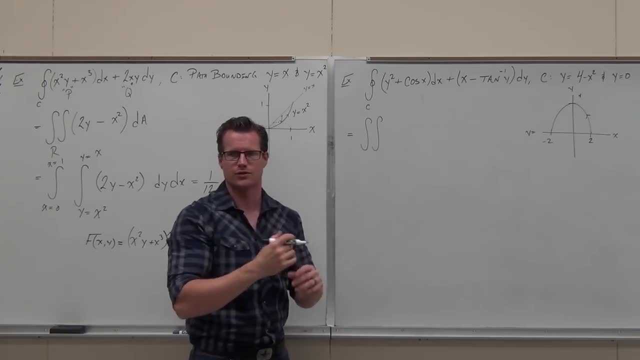 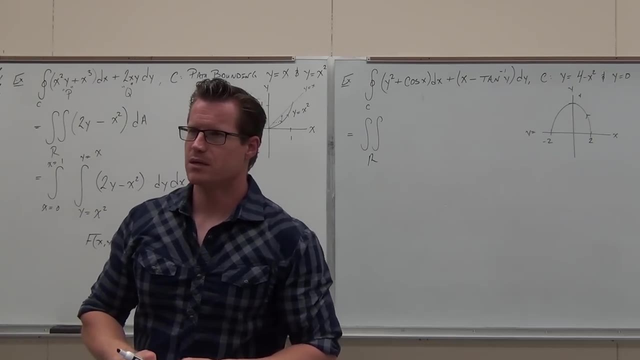 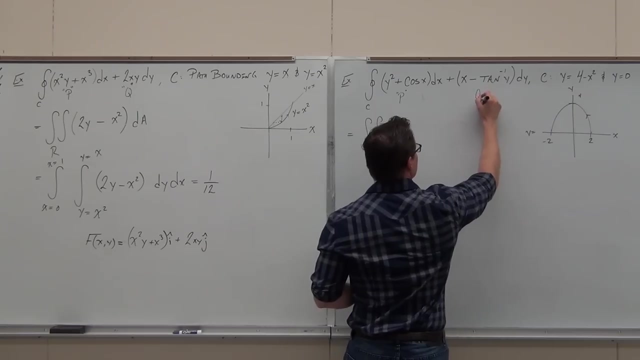 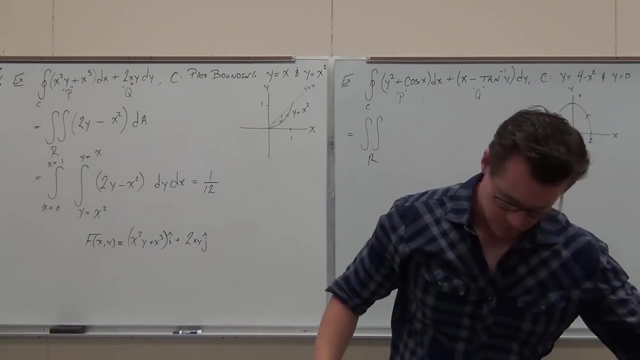 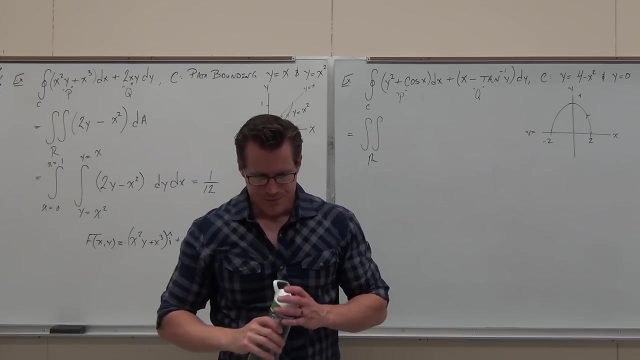 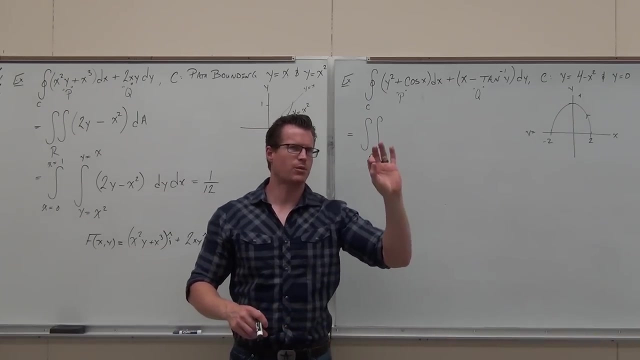 Leave it for a second. Leave it until you determine it's non-conservative. You might want to label P and Q before you begin. Can you tell me what the first part is, Tell me where I get the first part and then tell me what it is? 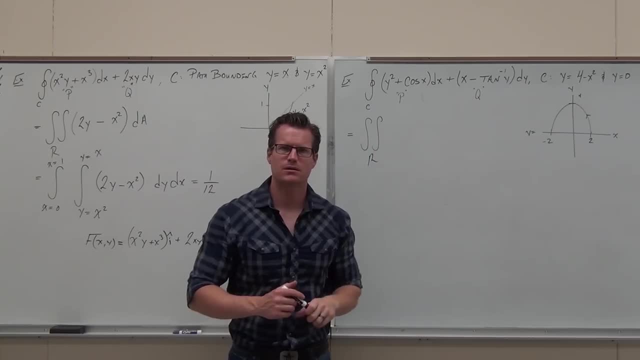 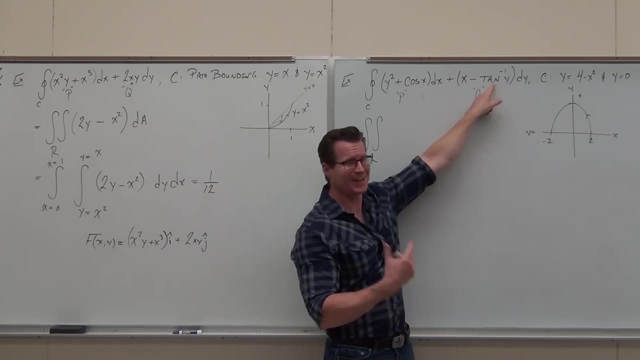 What should I get? One One, Why? How do I get it? The part you would do with respect to x, X, That's great. That doesn't even matter. I love that. It's just one. Partial derivative of Q with respect to x is one. 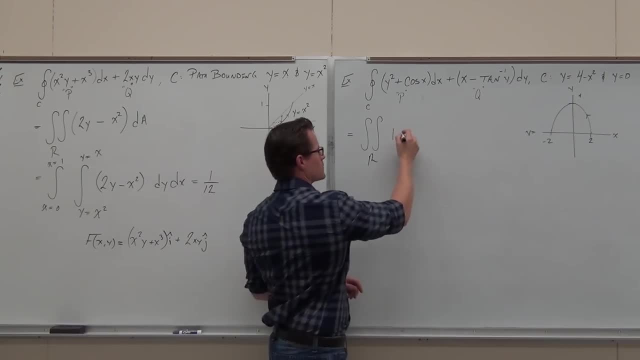 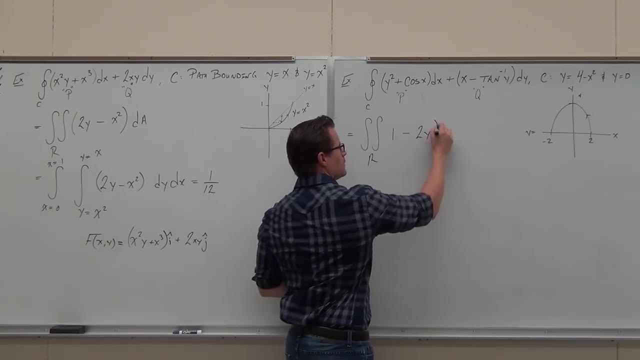 And then do I add or do I subtract? Subtract, Let's make sure we get that right. Partial derivative of P with respect to Y. Y, Which gives me Two In parentheses. what's the next thing I should have? 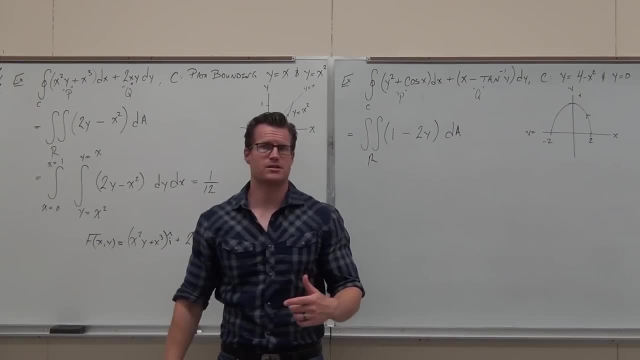 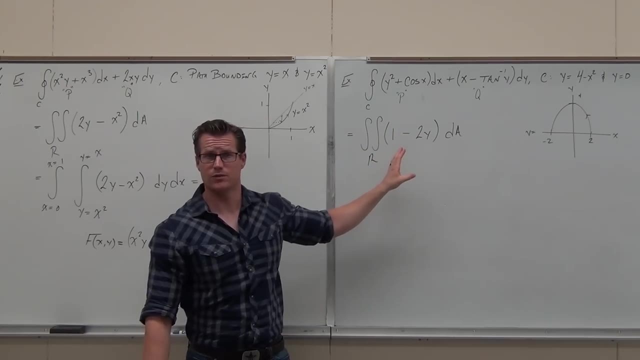 DA, DA. Okay, so let's practice something Now that we've. by the way, can you write down? don't do it, but could you write down what the vector field we're working with is? Yes, This I plus this J With me. 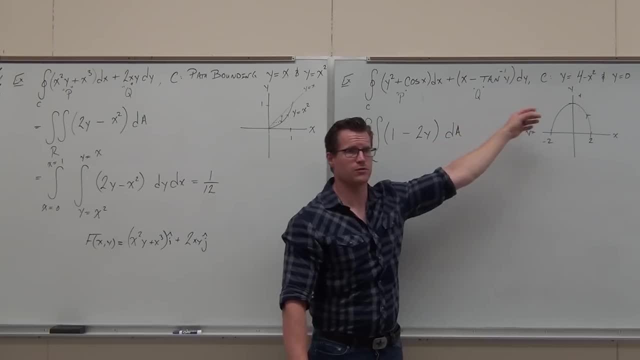 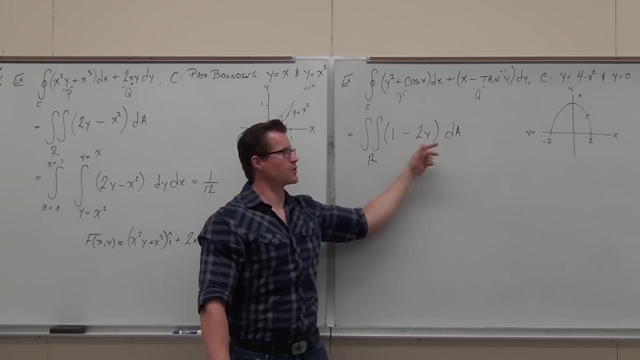 So we could do that. We're finding the work done along that curve, through that vector field. That's exactly what this does for us. It's given to us by a double integral. Write this down every time before you start working with the region. 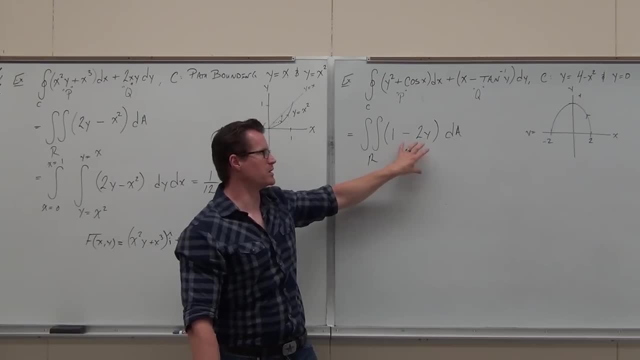 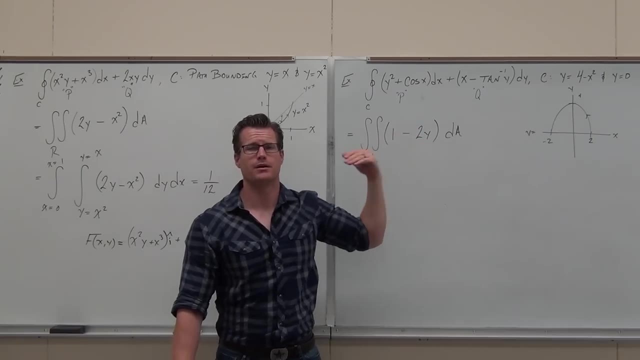 We've just determined that. the reason why we do it is because if we get zero here, we're done. That's conservative. Is this a conservative vector field? No, Otherwise we would have got Zero. Good, Go ahead and set the region up for me. 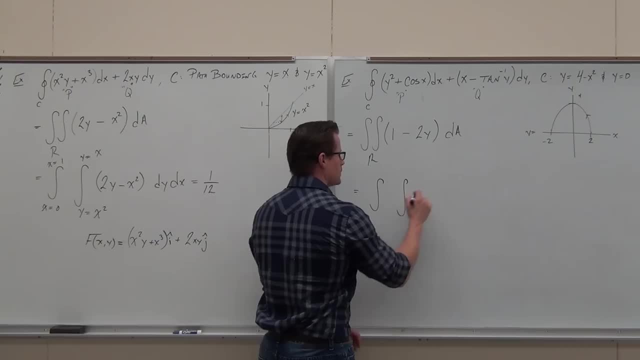 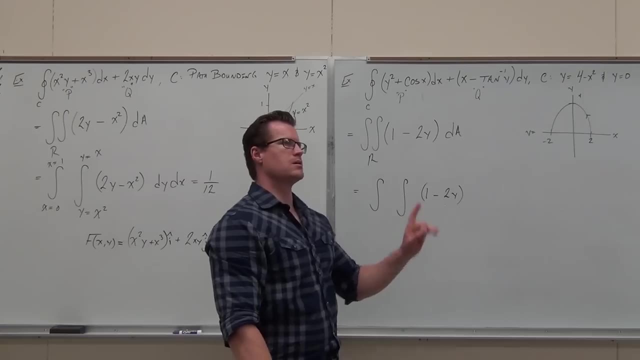 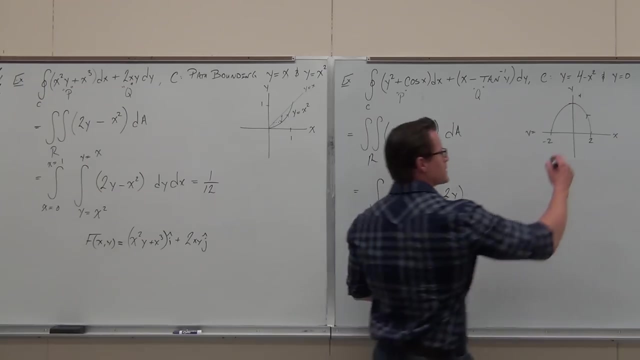 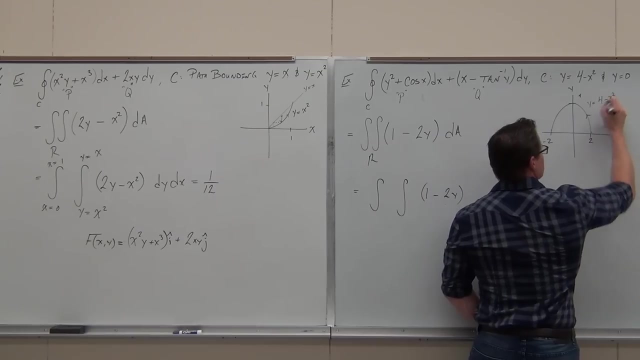 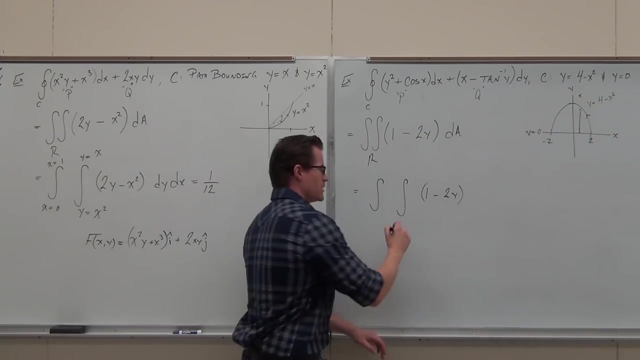 Now we're just back to double integral. Andy, Would you go in the x-direction or the y-direction? What would you do? Y-direction, Absolutely the y-direction first, Since this is all one function. We'd go from y equals zero to y equals four minus x squared. 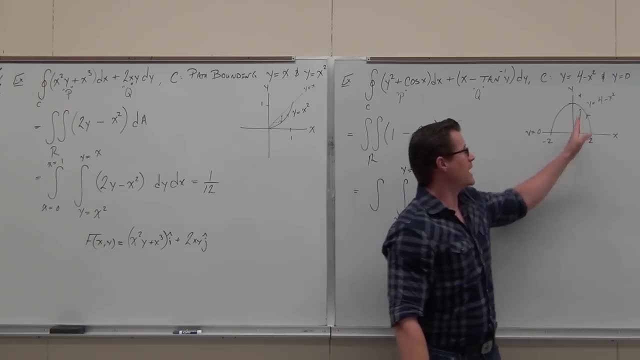 Look, if we went the other way, it would be possible, but you'd have to break that up And I don't want to do that. I don't want to break that up into two functions. Does that make sense? Make it as easy as possible. 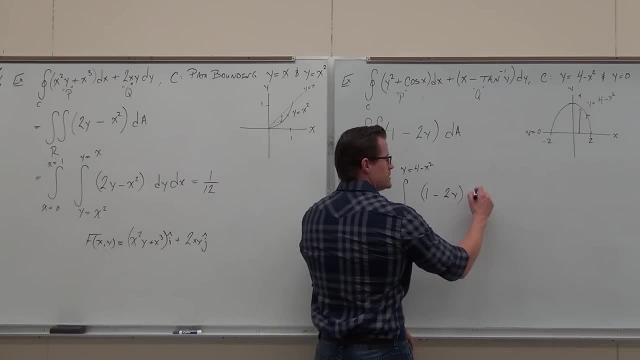 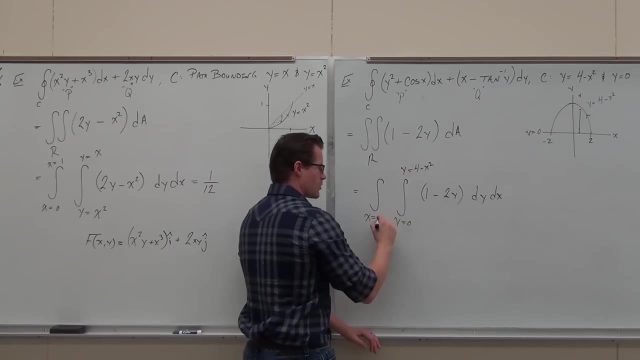 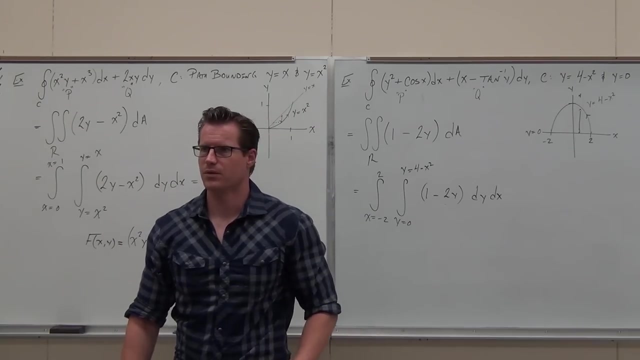 Don't start switching functions. That would be d, y minus x. That's what we solve for Negative two and two. I don't know if you're okay with that one. Would you know how to solve that double integral? Yes, Integrate with respect to y. first, 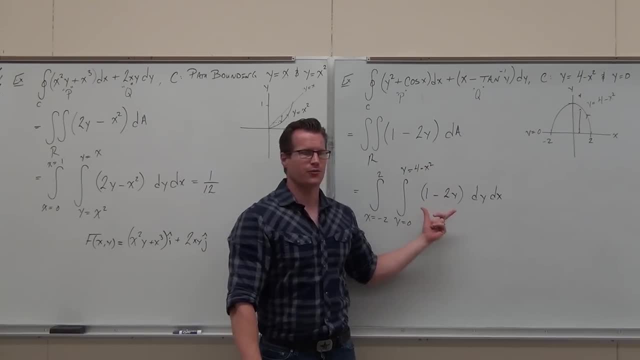 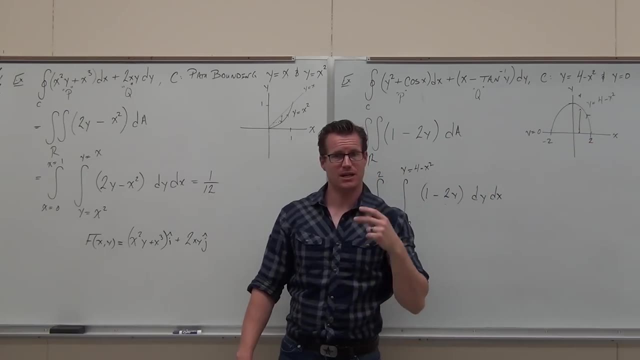 Man, honestly, compared to that, that's really easy. If we had to re-parameterize this curve and that segment, that gets nasty, And then we'd have to integrate two times after switching all the variables to t and then add them up. 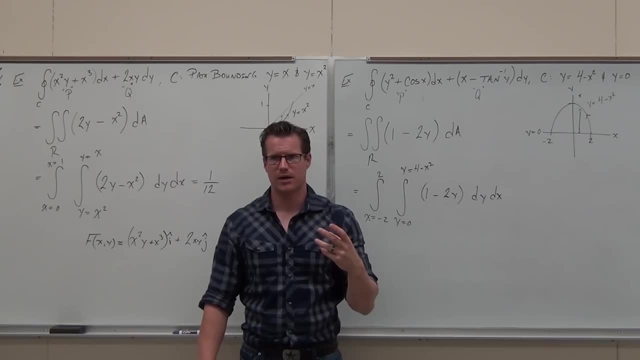 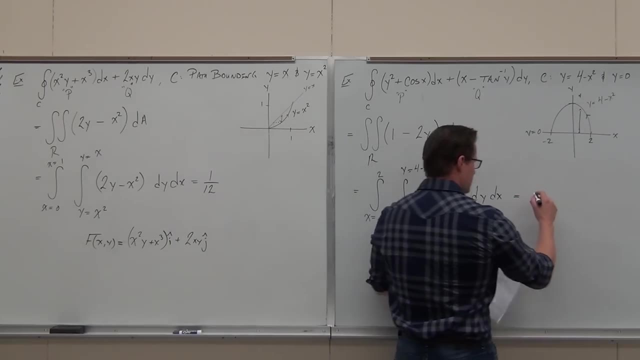 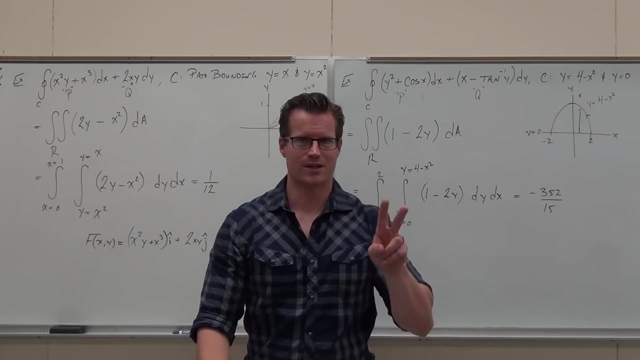 Gregg's theorem just saved us a tremendous amount of work. A lot, That's nice. The answer here, if you want to check it yourself, is negative. three hundred fifty-two over fifteen. Two things, What is it? Work, Work. 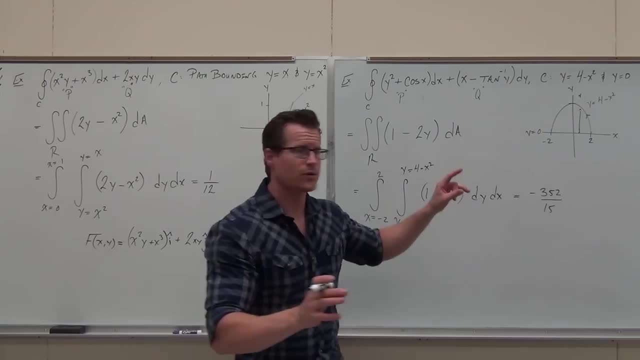 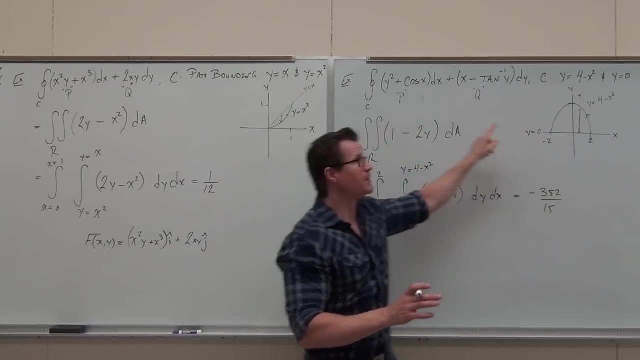 Work done over this curve. Well, along, Let's say along this pathway, the positive component's direction, Through, Through, Through this vector field, This vector field. That's what we're doing. What if we reverse directions? Positive work: 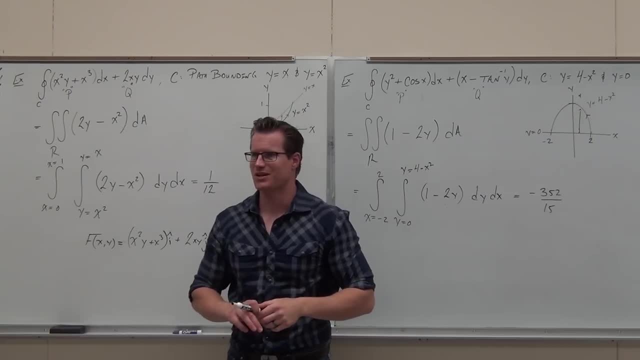 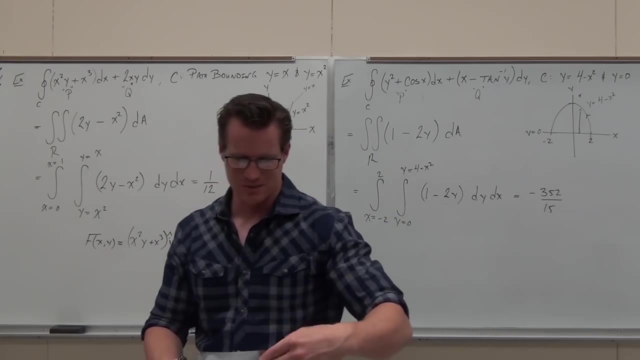 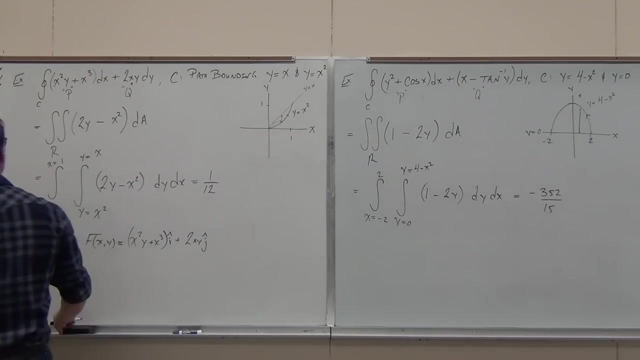 Positive work, Yep, Change of signs. That's all I got to get you to know. Let's do maybe two more kind of easy ones and we'll talk about an interesting idea. Then, if we get back to it, we'll do a couple others. 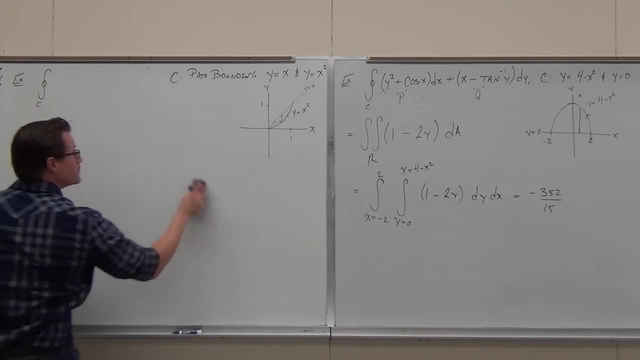 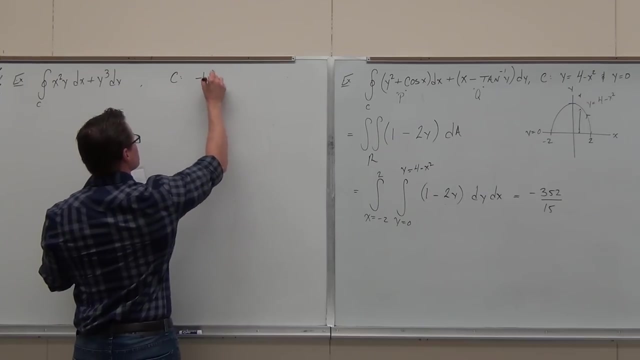 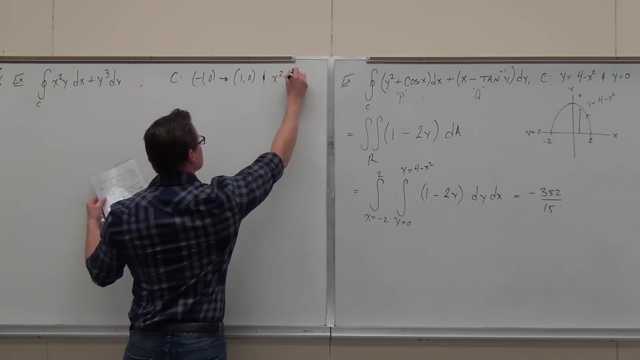 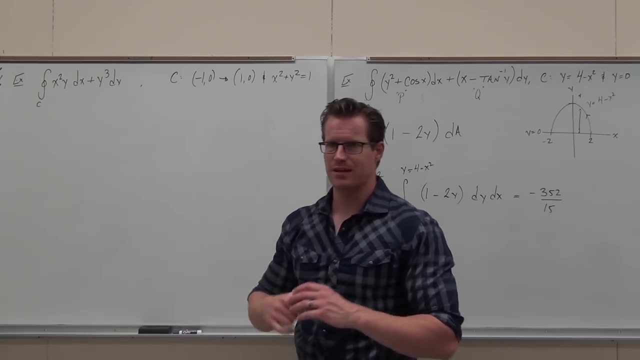 Let's go ahead and do the first one. Okay, Okay, Okay, Okay, Okay. we got a line integral. I'm telling you. it's a simple closed curve, which means that you have to have a connected region there. It's got to be bounded by those two things. 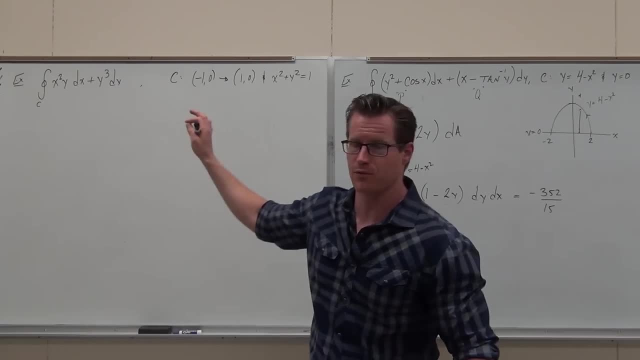 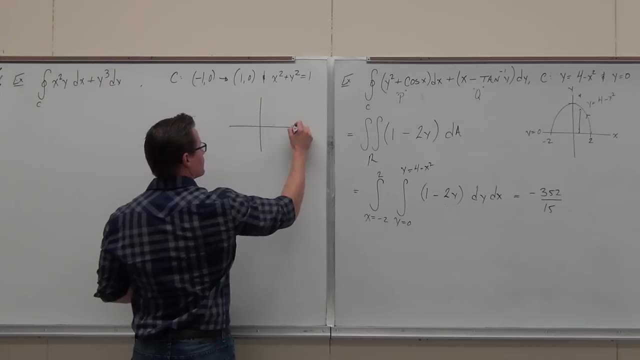 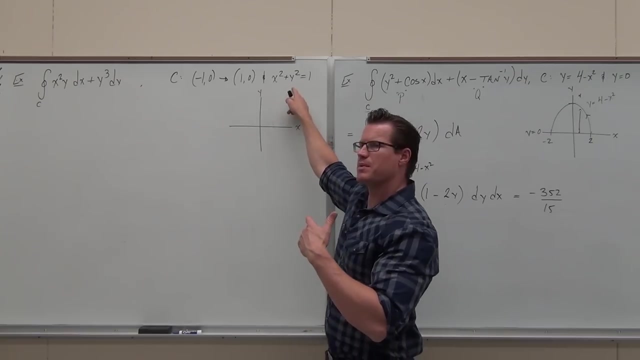 Well, it's the first thing you do every single time. when you have a simple closed curve over a line integral, Let's draw that. Hey, let's start with this one. That might be a little easier. What's that, Radius? 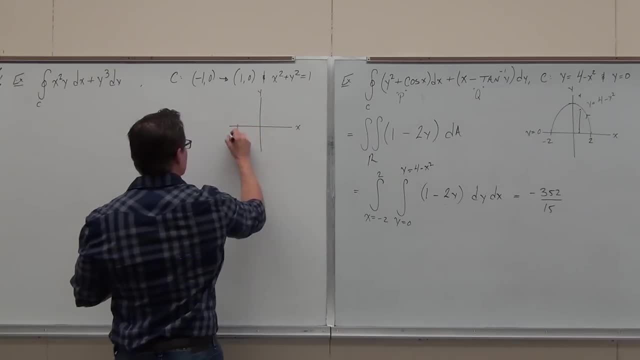 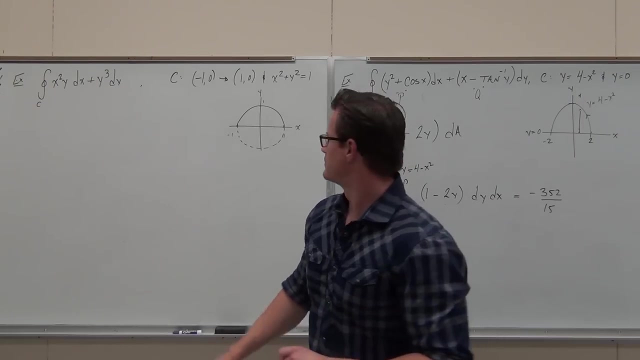 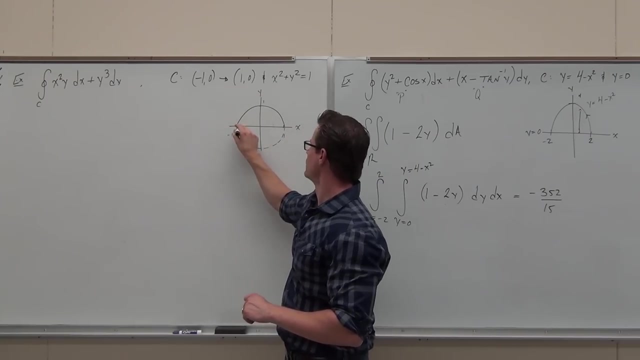 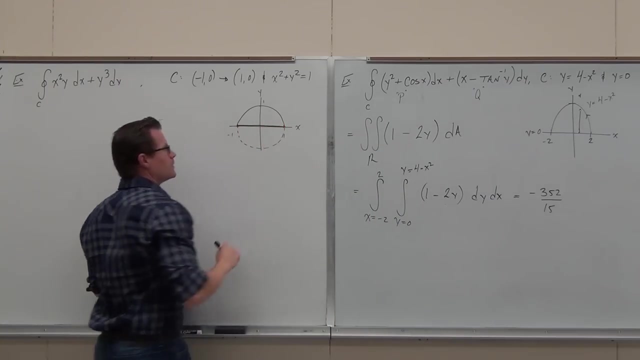 Center. Well, that's the worst circle that I've had in a long time. That's that circle. Now I'm drawing a dotted line. Why? Well, what's that? This little segment, this segment that goes from negative 1, 0 to 1, 0.. 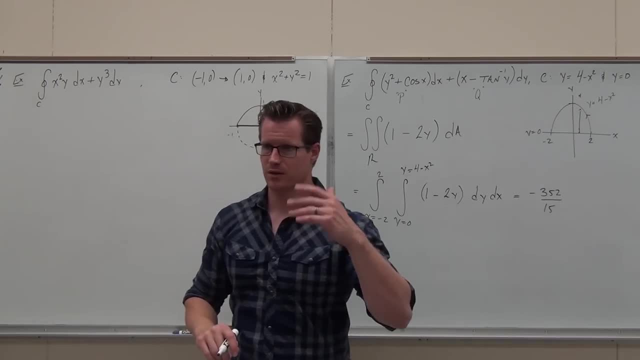 So we're going to make a choice here. We're going to pick the upper half circle versus the lower half circle, but we don't have two regions. We have only one region that's bounded either the top or the bottom. We're going to choose the top one. 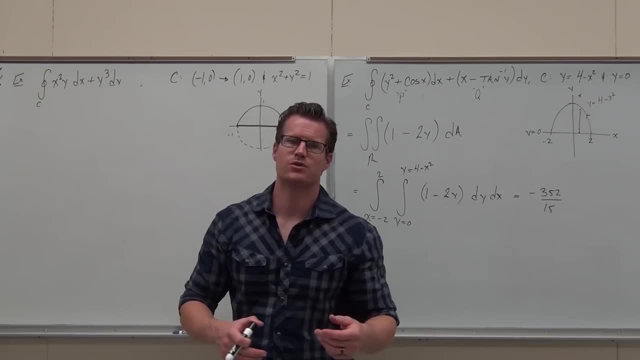 I don't know if you're okay with that one. Do you guys see the simple closed curve? Do you see why we draw these things all the time? If we draw them all the time, we get a really nice picture What's going on. 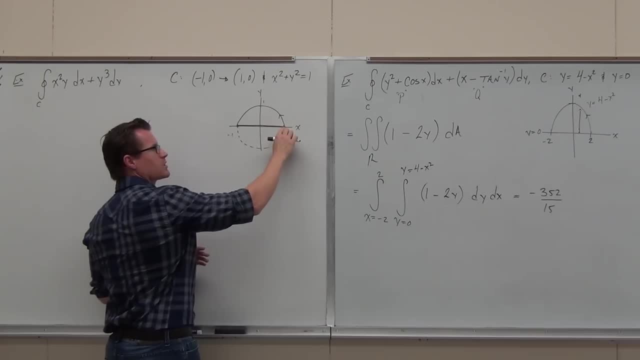 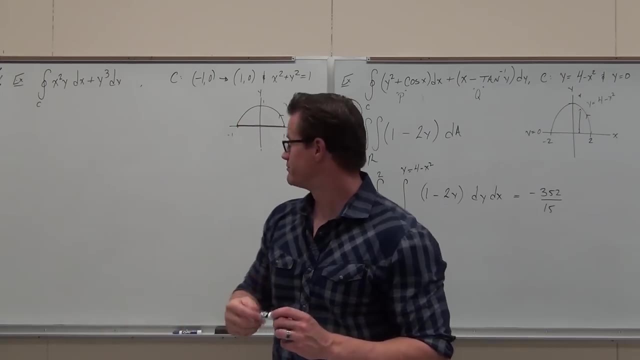 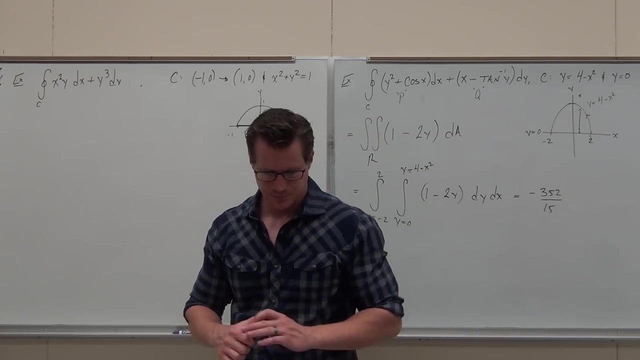 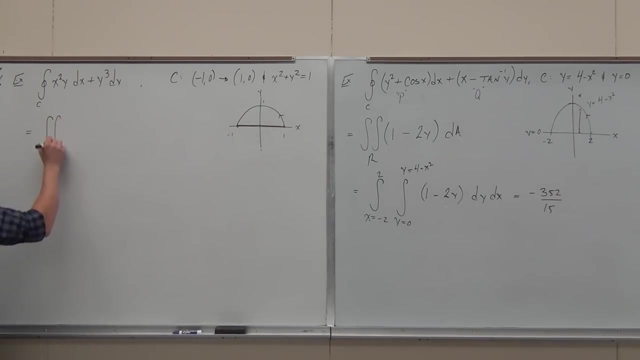 This right here is our simple closed curve that contains a region. Is Green's theorem going to apply? Yes, Let's go ahead and set up Green's theorem, please. Okay, Well, I know that's P, I know that's Q. That's kind of nice. 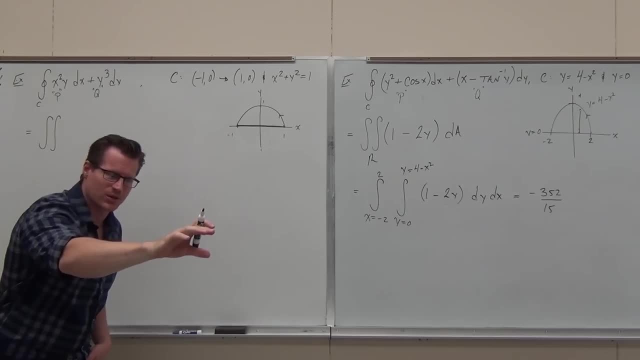 What's the first thing I should put? I'm going to talk about Y in this example. It's why we do it, One of the reasons why we do it. We set this up first. What goes right there? R. Don't write anything but that until you take a look at your region. 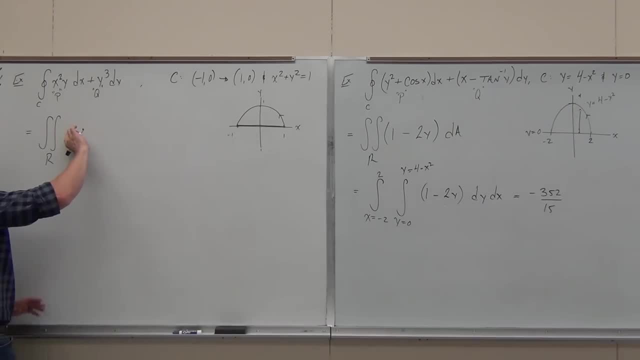 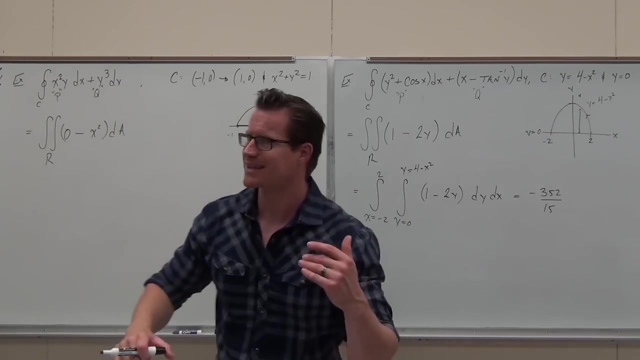 Okay, So we have this: We have the partial of this with respect to X, minus partial of this with respect to Y, And then we have a DA A D. A, Not a D, anything else, Not a DX, Not a DY. 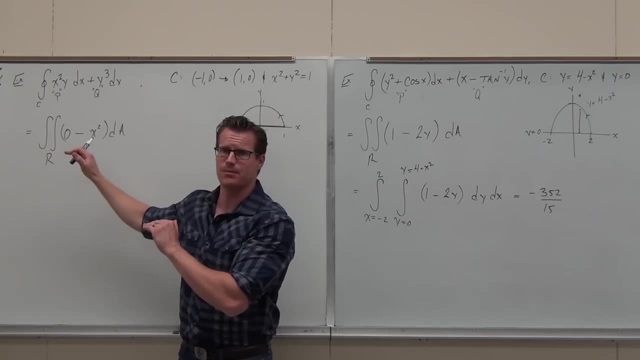 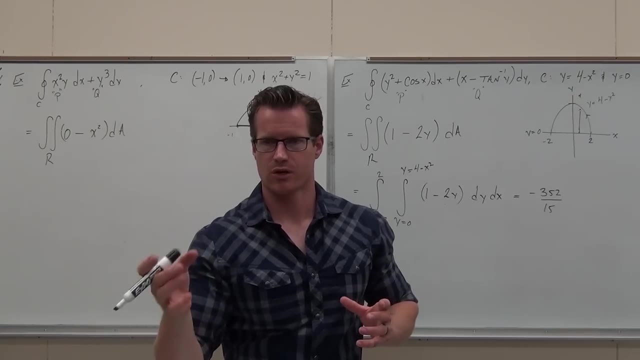 A DA, Don't ever. I said it four times: Don't ever skip this step. Y. Here's the cool. One of the coolest things about Green's theorem is it changes curves into looking at regions. When we did line integrals before we did a right half circle. 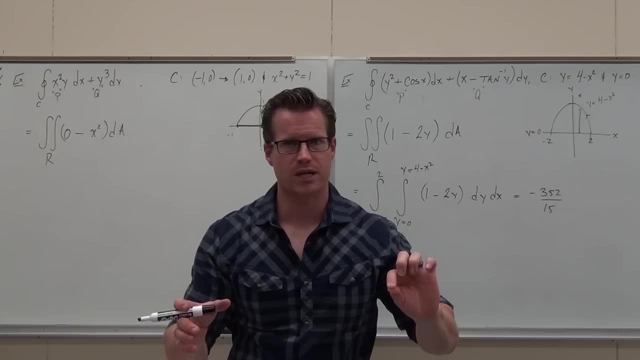 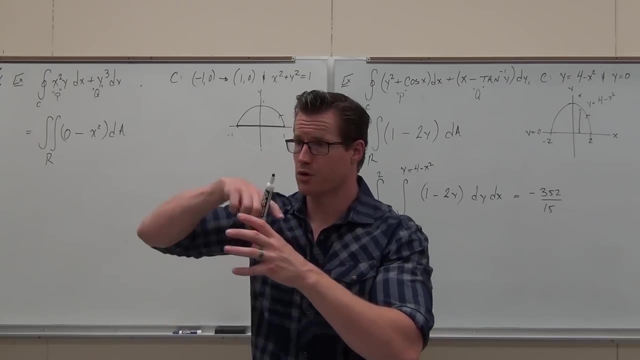 Do you remember that? And we couldn't use polar because we didn't have a region? Do we have a region? Yes, Green's theorem lets us change from a curve to region that that curve contains. If that's the case, we're now back to basic double integrals. 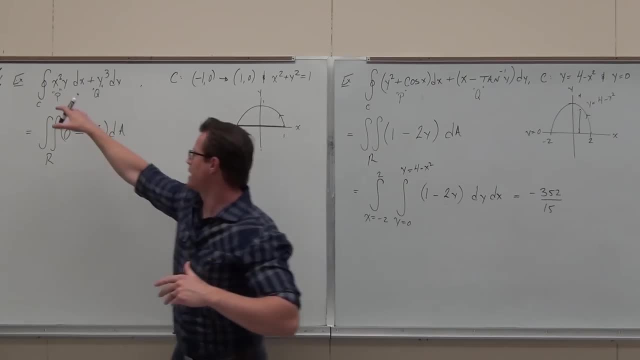 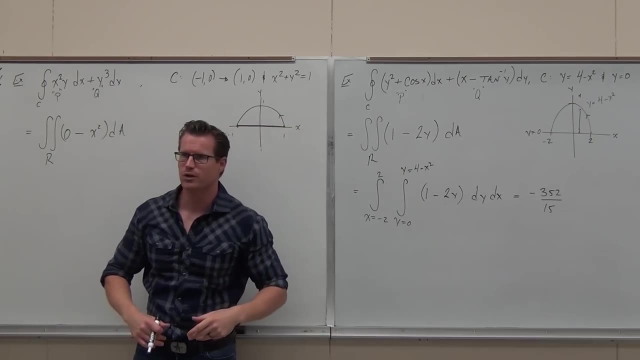 So the reason why we write this is because it switches your head. It says line integrals, no Double integrals. yes, What's my double integral? look like That. What's that? look like Polar. Make sense. We now get to use stuff like that. 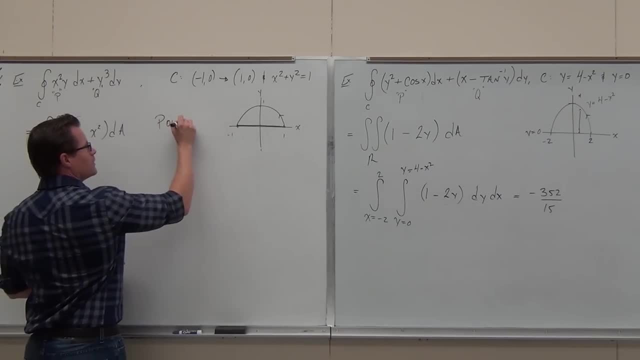 That's brilliant, Fantastic. So for polar, well, I know that X squared plus Y squared equals X squared. So I know that X squared plus Y squared equals X squared. So I know that X squared plus Y squared equals R squared. I know that R equals 1.. 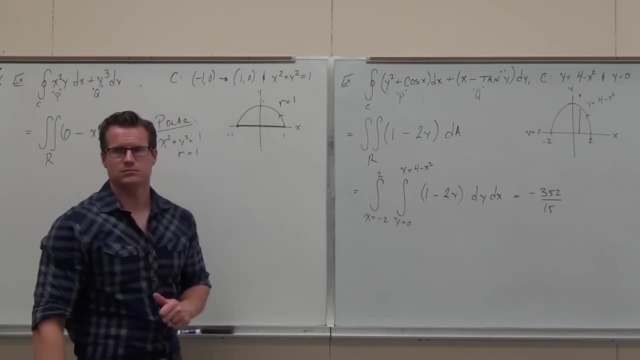 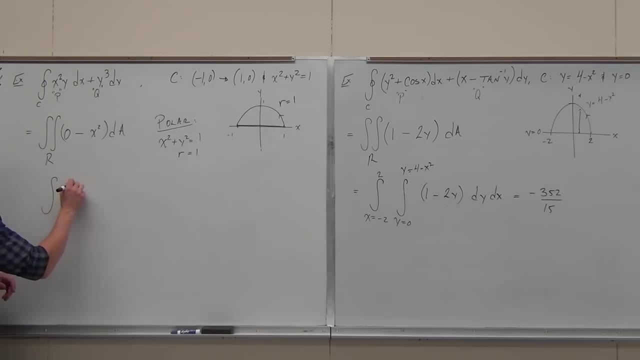 R squared equals 1.. R equals 1.. That was pretty easy Make sense. I know that if I'm going to set this up, I have a double integral of something inside. We're going to do it the same way every single time. 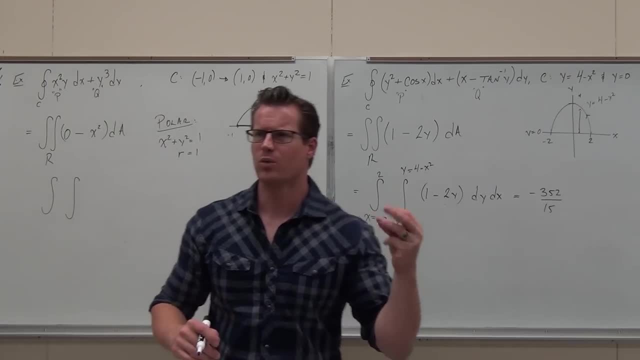 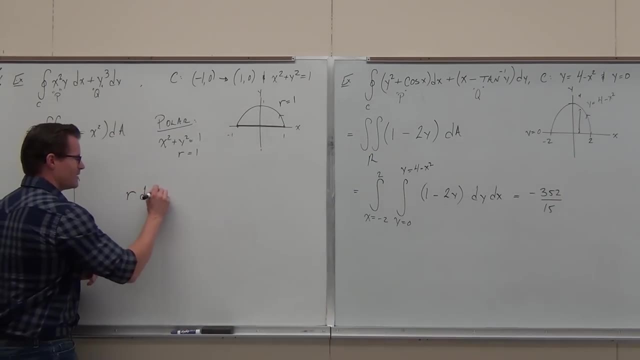 I need to go, oh hey, for polar. oh my gosh ringing a bell, Polar. what do I have to have when I do a DA into something else, Into the polar? Hey, You remember it. That's why we write the DA. 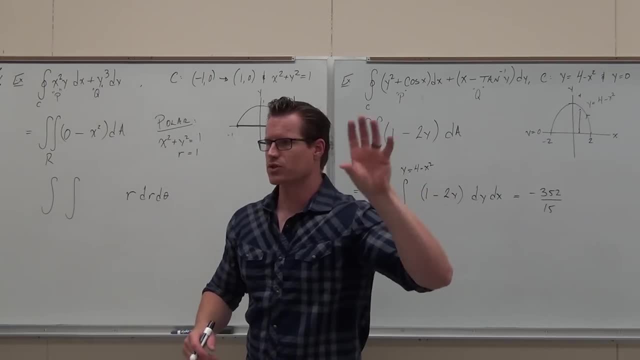 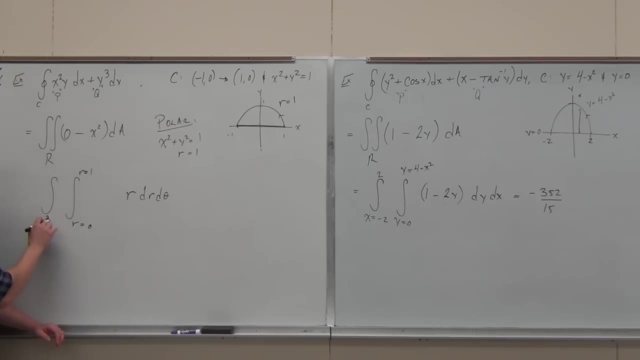 So it rings a bell and you go, DA. changes to RdRd theta. We're now just working with double integrals. We're doubling over 1.. Here we have to go R first. R goes from 0 to R equals 1 theta. 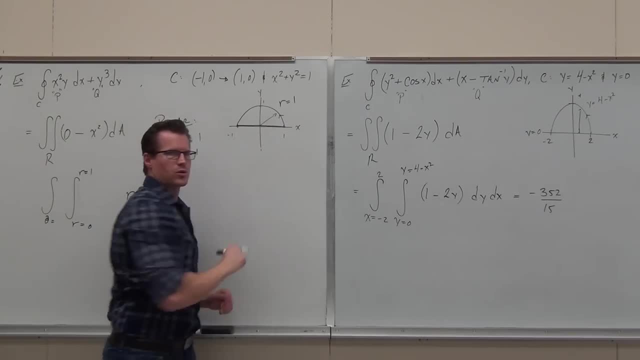 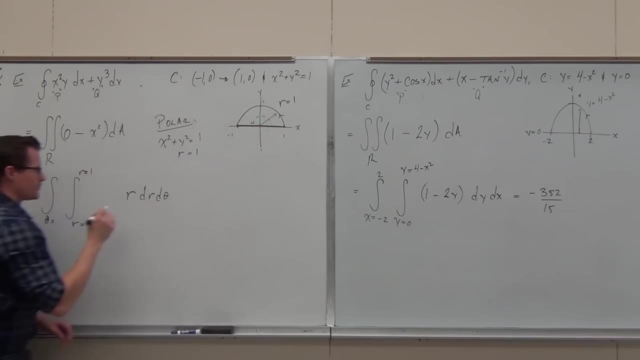 Oh, theta. Firstly, are you guys okay on the R portion of it from 0 to 1?? Talk about my theta. Where's it going from 0 to Y? Good, It's not a full circle. So fancy. we learned that one. 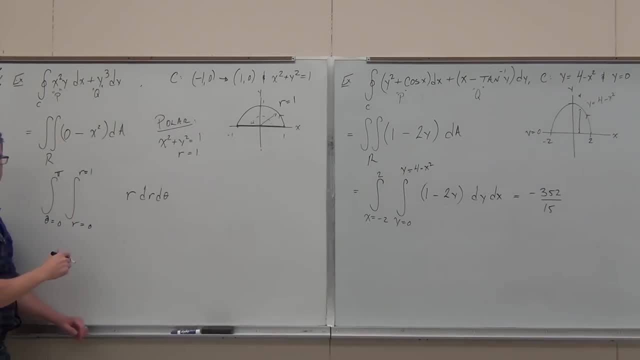 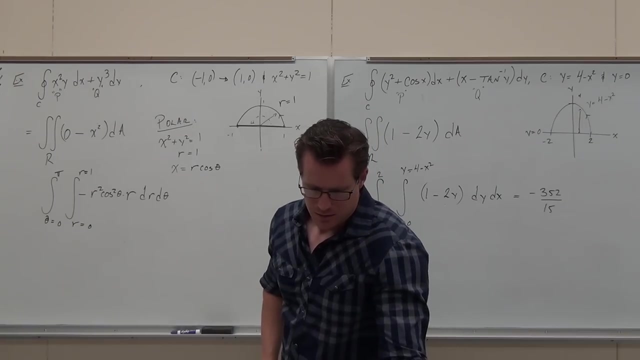 Sweet, Let's keep on going. Let's narrow it down. not X's, Okay. R cosine theta. therefore, this would be negative: R squared cosine squared theta. Negative that: Are you buying into this stuff? You're all right with that one. 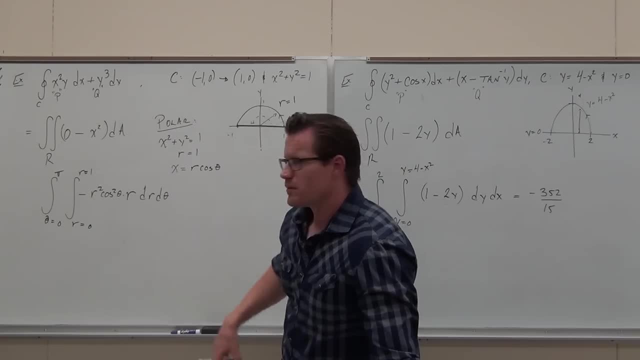 Yes, yes, yes, yes, yes. Okay, Could you work it out? What's the first thing you'd do? Combine the R's, Combine the R's, Get R cubed, You get a negative 1. fourth R to the fourth cosine, theta. 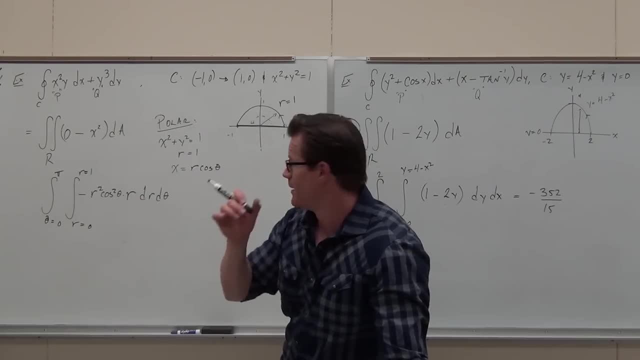 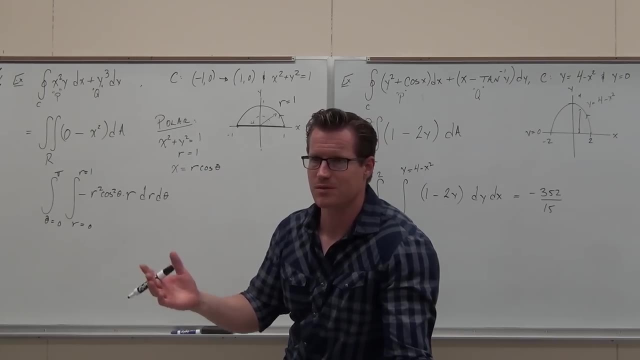 Plug in for 0 and 1. Get a 1 fourth out of that And then you get this cosine squared that you'd have to deal with. Okay, So that's those even powers of cosine. Probably use 1, half 1 plus cosine 2 theta. 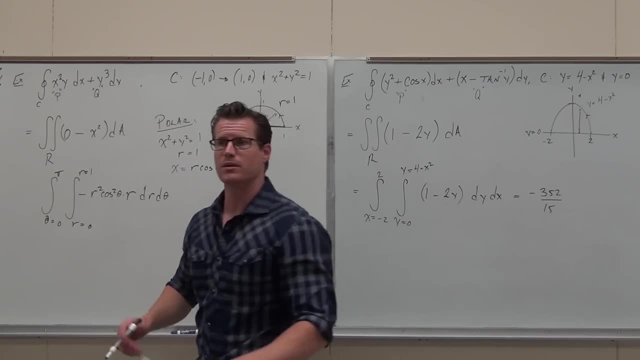 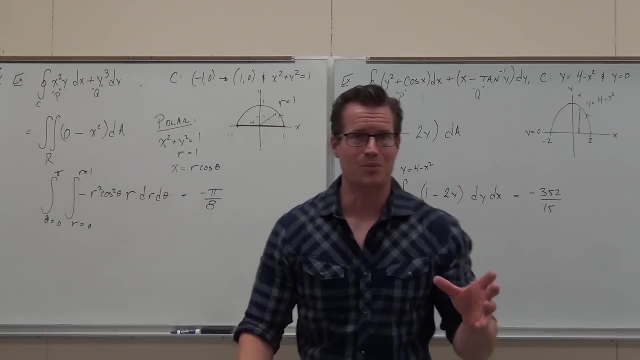 Evaluate it. Not a huge amount, It's not a huge amount. It's not a huge amount. It's not a huge deal. I want you to get negative 1 pi over 8 out of this. We're on a roll, but I've got to make sure that I'm not just killing examples here. 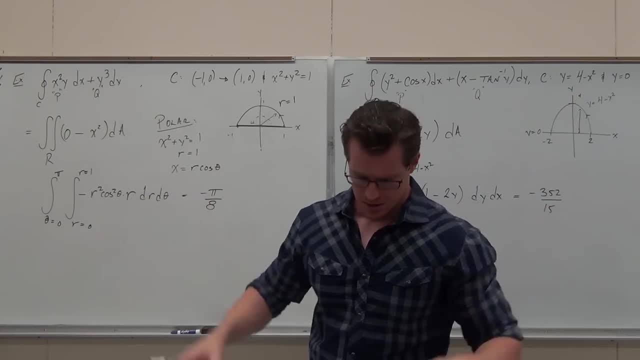 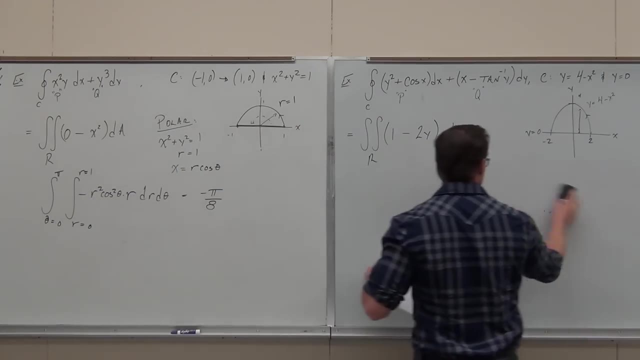 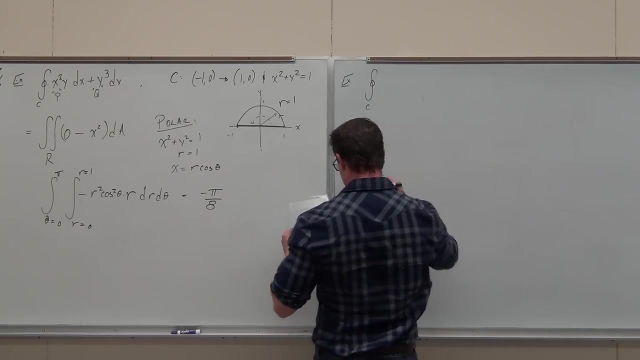 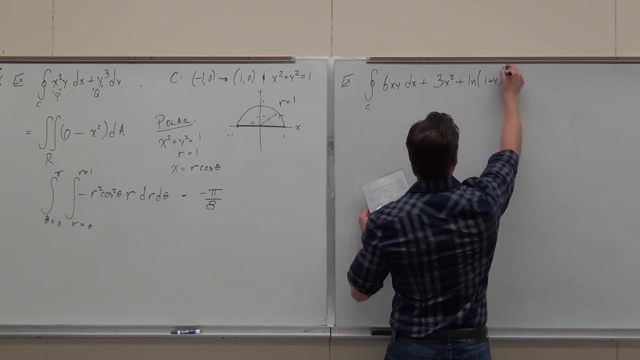 that I'm giving you something. Are you understanding the idea? Okay, Let's do. let me have you practice one more. Mm-hmm, All right. Okay, All right, All right. I think we're going to go over the same thing, which is we're going to have to divide the 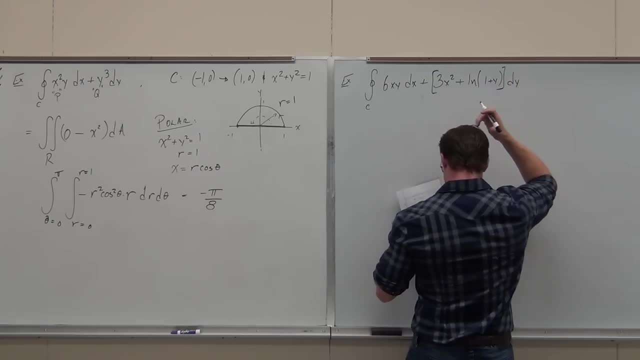 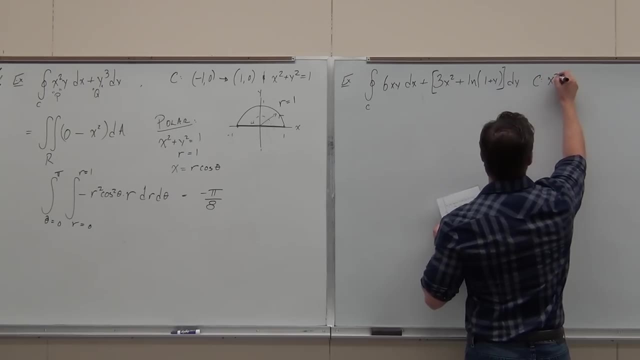 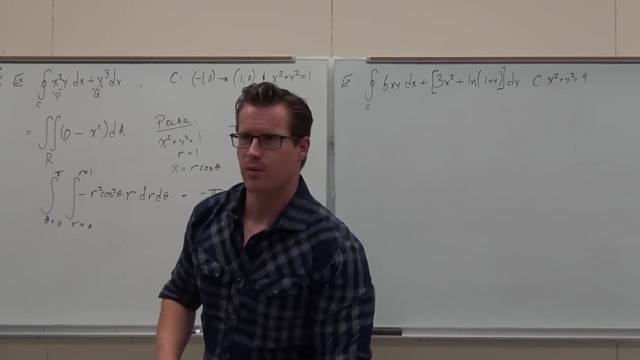 energy of that thing. We're going to know how to get rid of this thing and we're going to have to figure out how to get everything together. So you're going to have to do that. Go for it. I want you to do it completely by yourself. 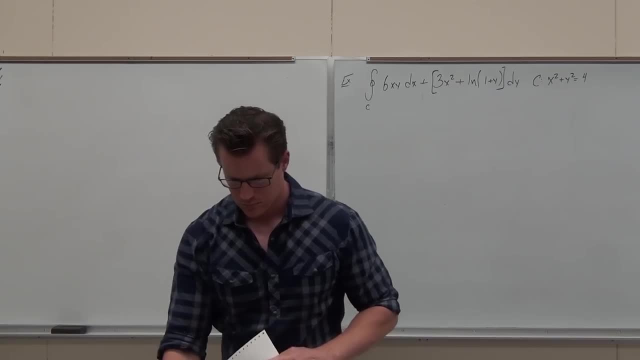 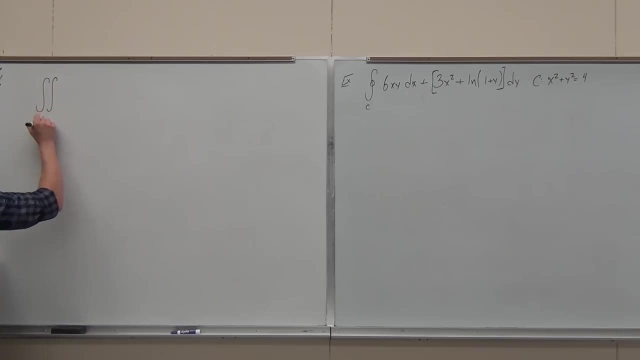 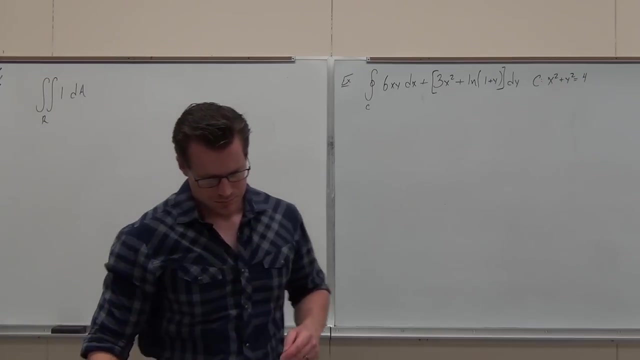 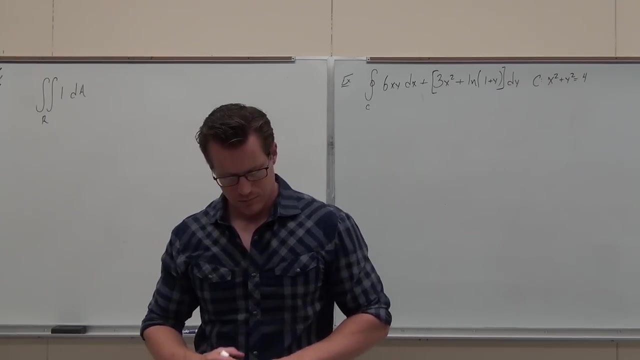 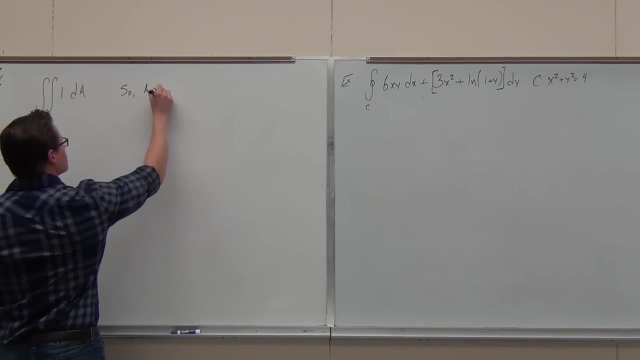 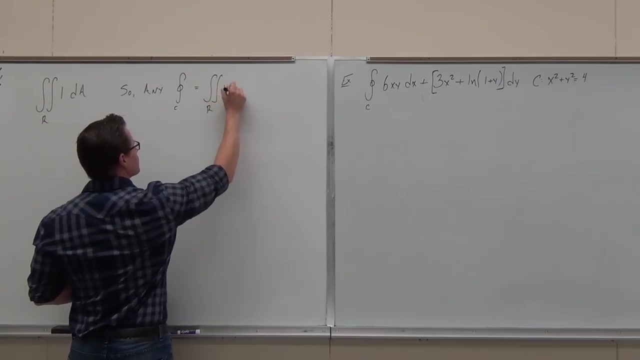 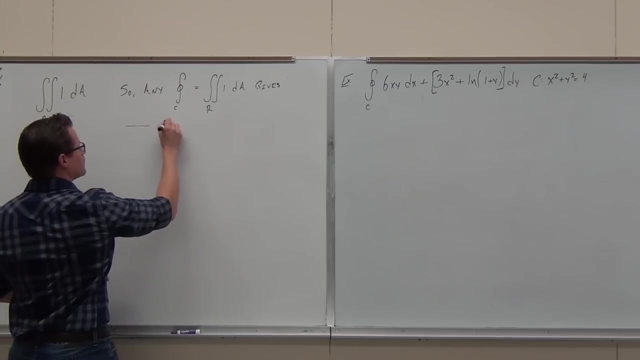 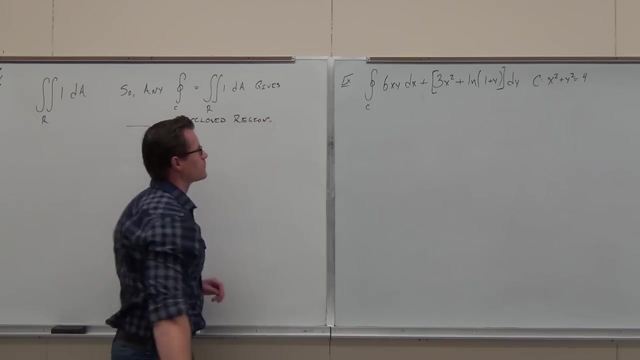 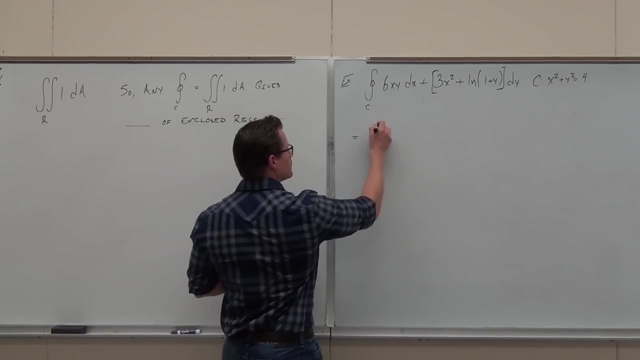 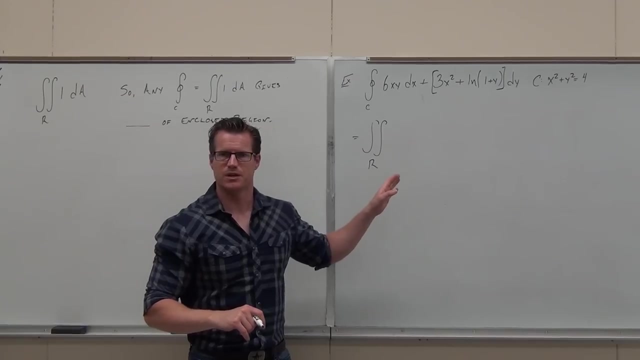 I want you to do it. I want you to do it completely by yourself. I want you to do it completely by yourself. That's why we don't do this. the second reason why we don't ever worry about the region is because when you start setting up Green's theorem and you go, hey, that's my p, that's. 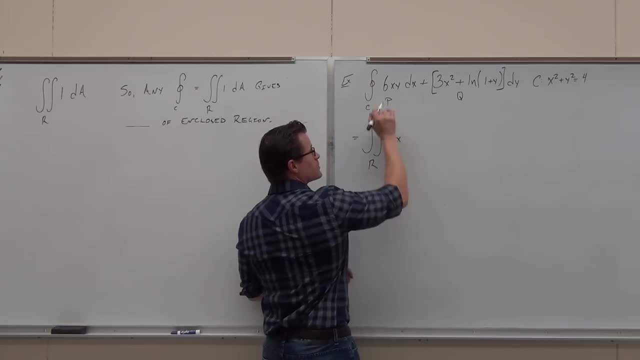 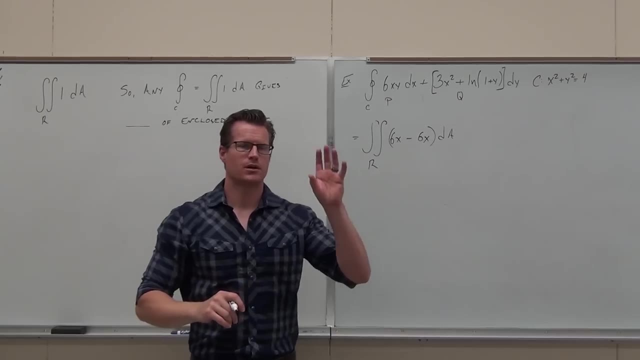 my q with respect to x gives me 6x. with respect to y gives me 6x. Tell me something about this vector field. Tell me something about a line integral of a simple closed curve, and I don't even care what it is. 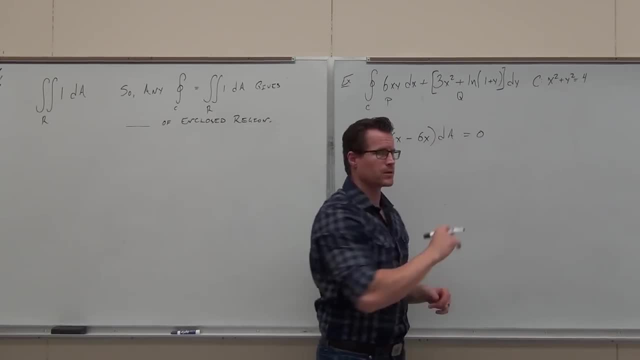 That's a simple closed curve over a conservative vector field. Don't even have to worry about it. I didn't draw it here because we don't even have to worry about it. That's kind of cool, right, Put the pieces together. 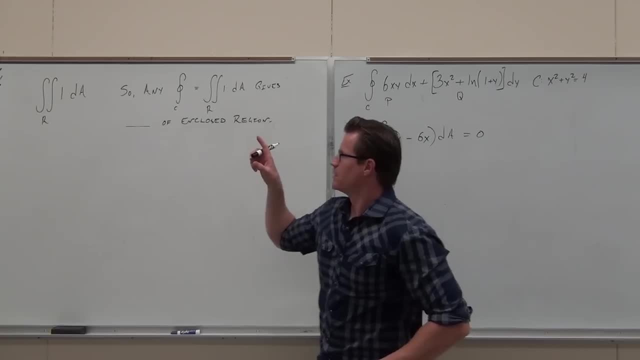 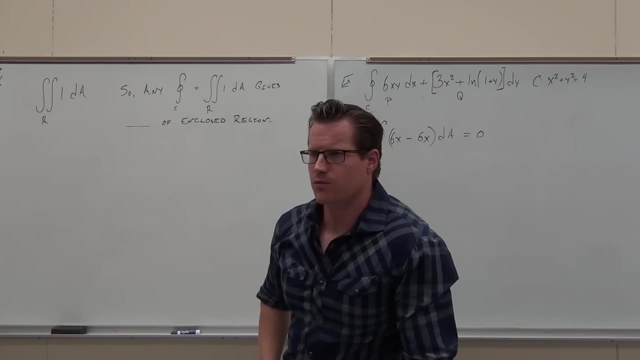 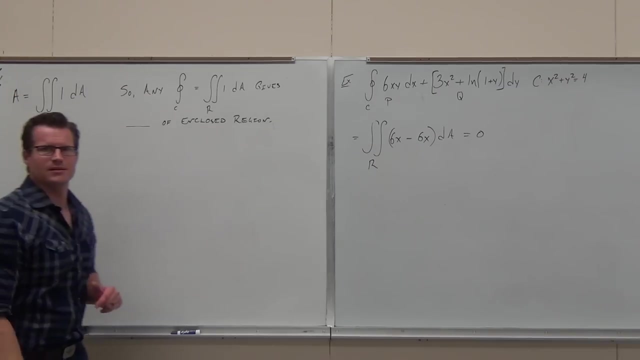 That's fantastic. Now let's ring a bell for a while. What's that give you? What's the double integral over r of 1 dA? It's area, Area of what Area of what Area of the region. 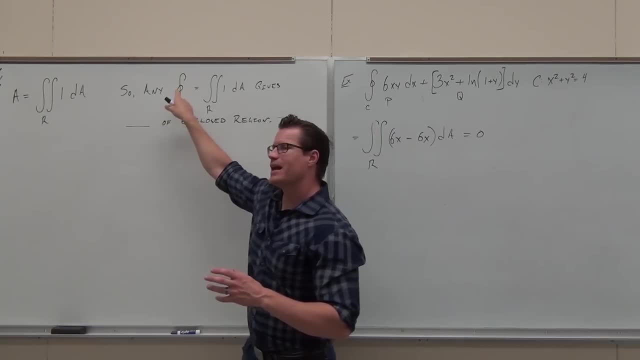 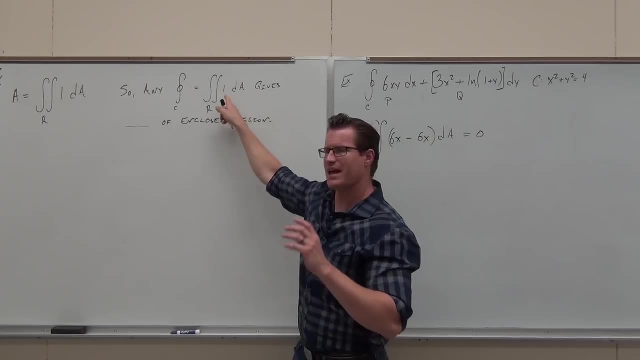 Area of the region. So if any line integral over a simple closed curve, ever by Green's theorem, gives us 1, double integral of 1,, if that ever happens, then what this is giving us is the area of the enclosed region of that curve. 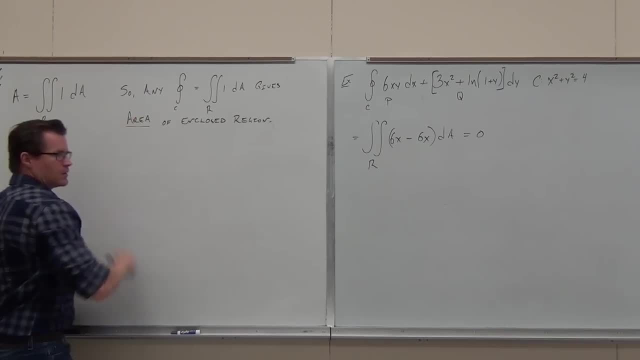 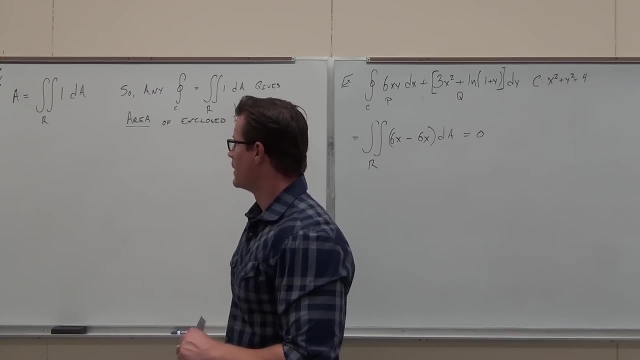 Now we're going to do some razzle dazzle. okay, We're going to invent something here. I'm going to work on this on the side, just to make sure you saw where it comes from. We're going to invent something. 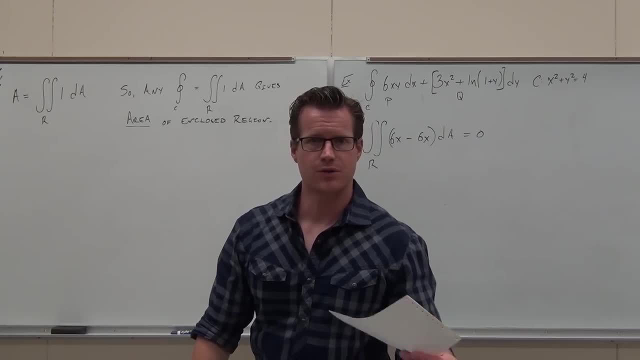 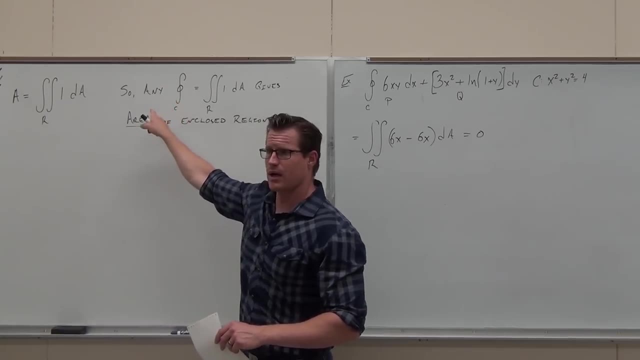 We're going to invent a formula that gives us the area of the enclosed region every time. You see, the problem is. look at the problem. We're never given that. We're always given line integrals, right, I want to create a line integral that's going to give me area every single time. 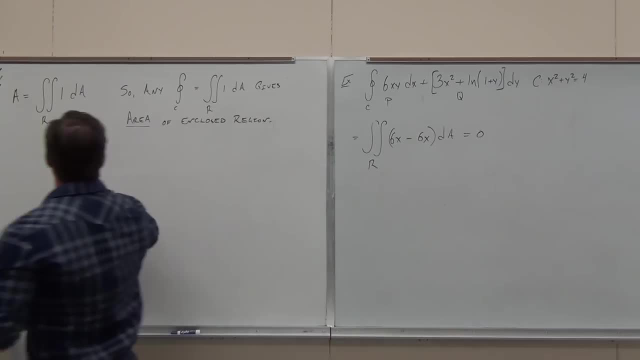 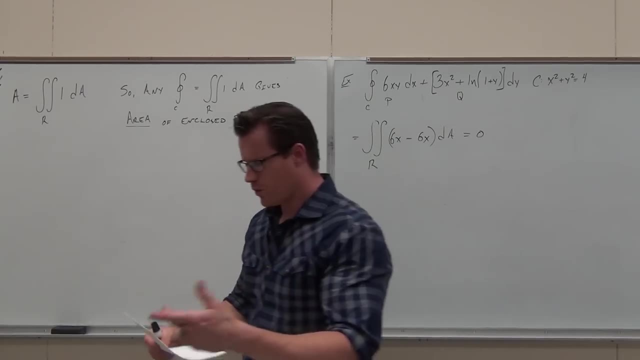 Are you guys following? So we're going to work backwards. Here's how we go. I want this to happen, okay? Well, if I want that to happen, then my goal is: I want to eventually make this double integral of 1.. 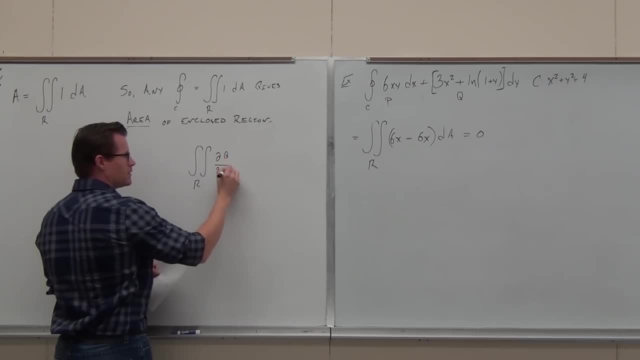 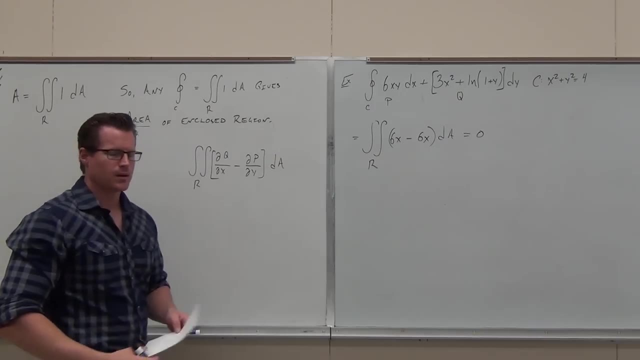 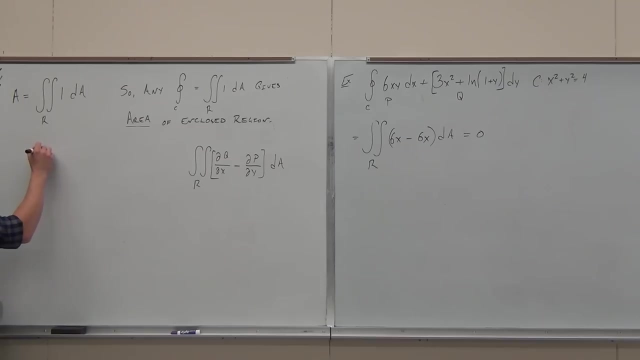 I want this to be a double integral of that. I want that, So I need something that I'm going to split up. So what I'm going to do here is I'm going to change this, I'm going to rewrite this as 1 half the double integral over r times 2, because I want to. 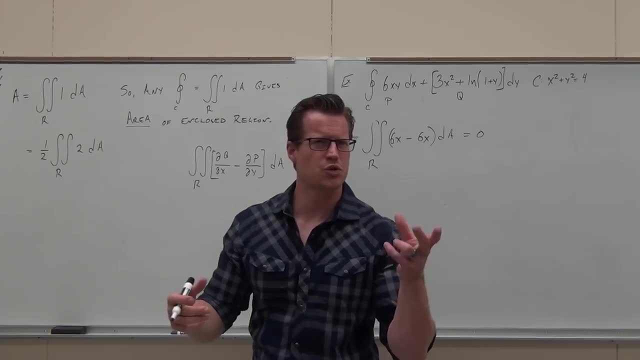 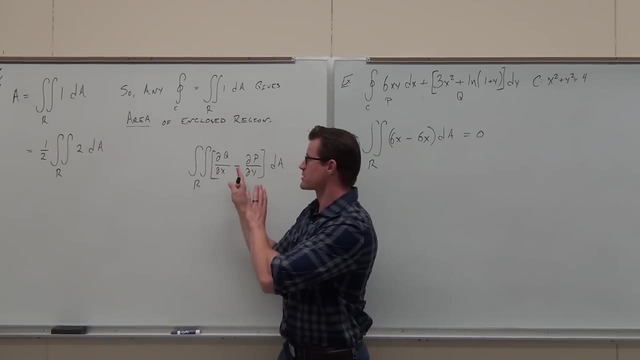 split this up somehow. I want something easy to split up And I know that 2 splits up really easily. I want something that splits up really nicely if I'm looking at subtraction. So here's my goal. I'm trying to get this to look like this so that I can create a line integral. 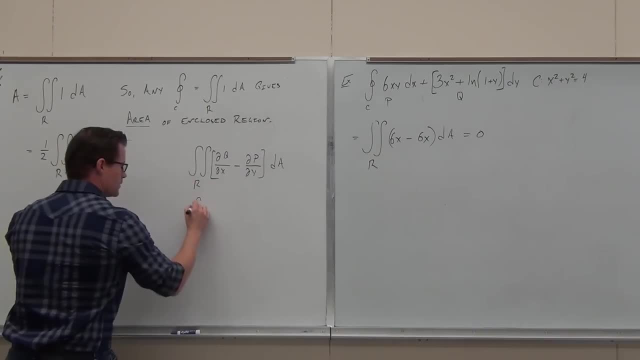 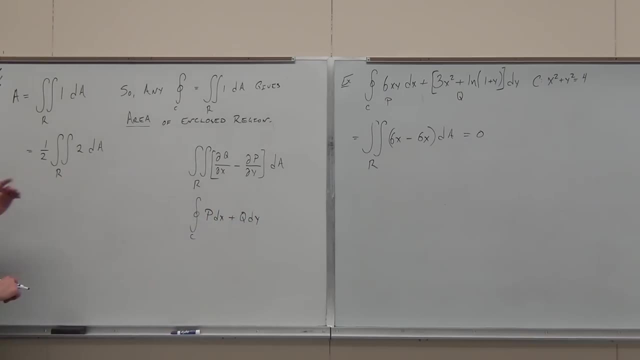 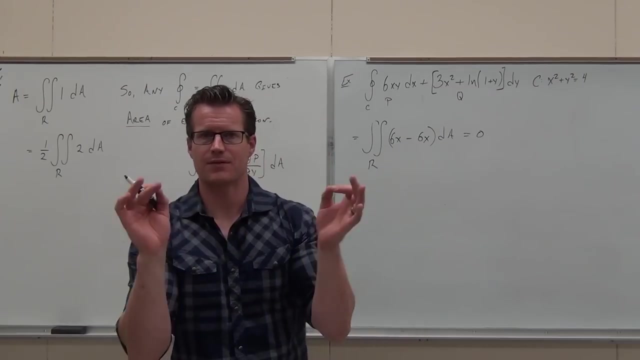 Does that make sense? I want that. So I want to get from here to here, So from here, okay. well, if I want subtraction, how can I split up 2, there's a lot of different ways. How can I split up nicely so that I still have 2, but I have a minus in the middle? 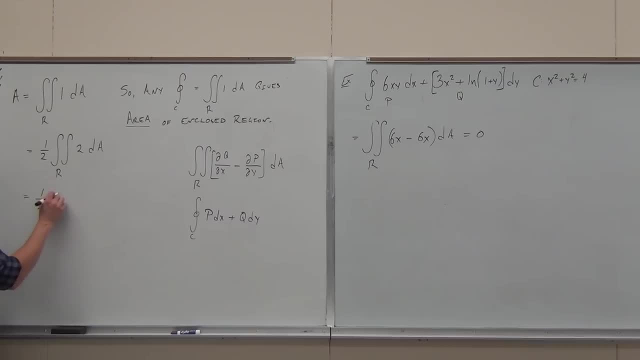 How could I do it? Minus 2.. Minus 1 and 1.. So I'm going to break down this up and make something easy and clear again. Any ideas? I don't want to look at this because I I want to. 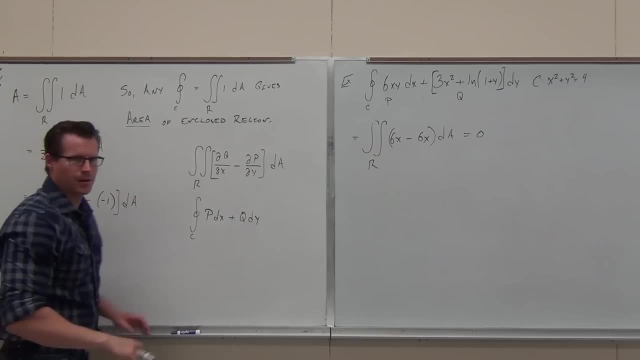 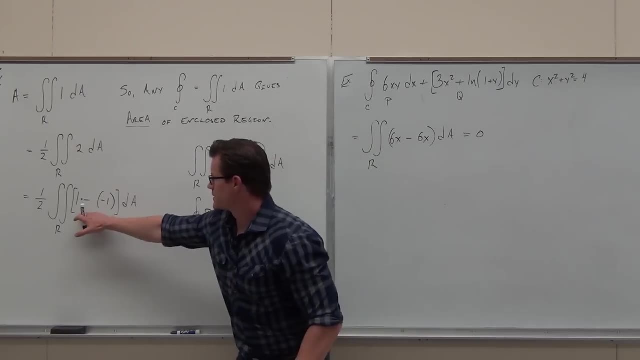 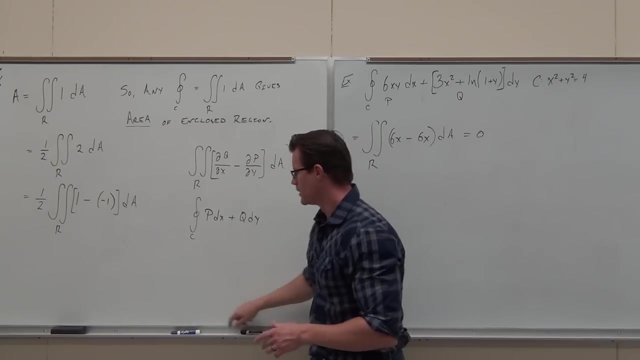 Okay, I've got an idea. How about that? Let's try that. Is that still 2?? Does it fit this model? Okay, So watch this, Watch this. This will work, magic happen that fits that model. then this piece has to be, or we're going to. 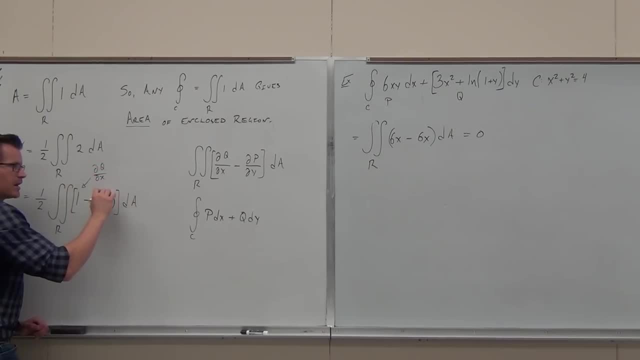 let it be the partial derivative with respect to X and this piece has to be the partial derivative of P with respect to Y. if we undo those pieces and put them here and here, how would you undo a partial derivative with respect to X? you integrate with respect to X, undo the partial derivative with respect to X. if we did it, 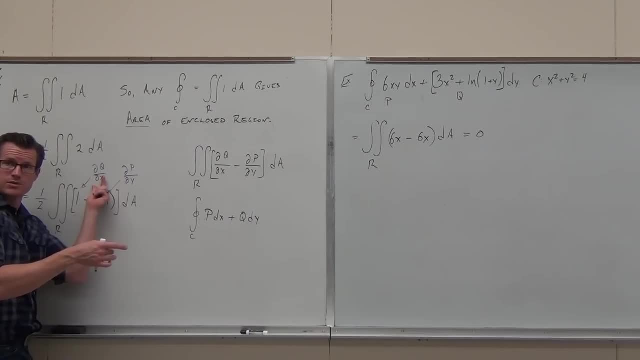 already we did the last section. take an integral with respect to X. it would undo that, hey, what's the integral of 1 with respect to X? it's X. that's giving me my Q. now let's try this one. remember this and this are equal. so we're structuring this in order to get. 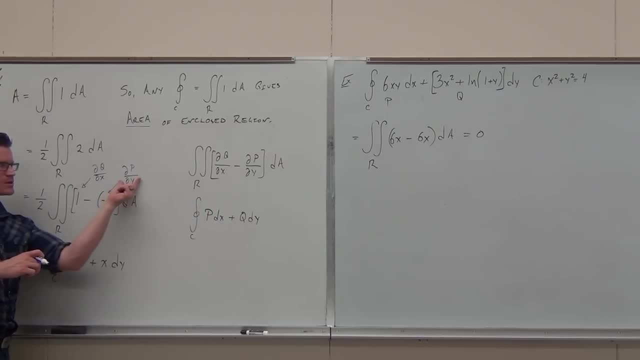 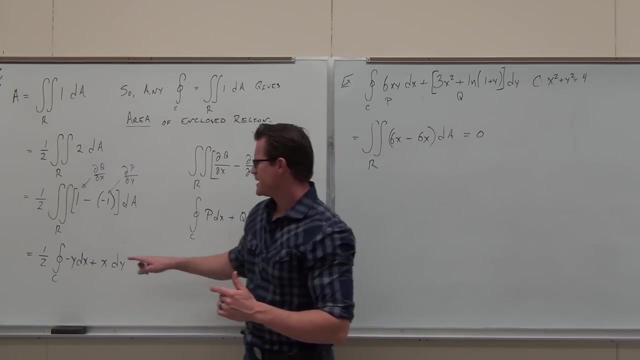 this. that's the idea. what's the integral- remember this was a partial derivative P, that guy- with respect to Y, it gave me negative 1. so integrate with respect to Y, what's it give me? integrate what's the integral of negative 1 with respect to Y, negative 1, and that goes here. let's double-check that. if I take: 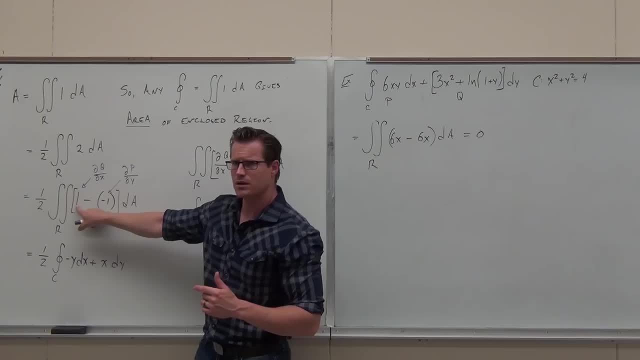 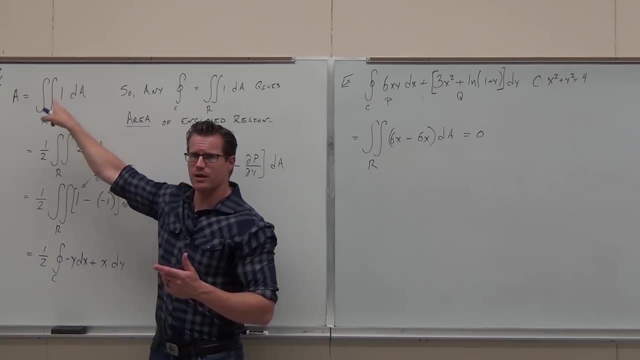 the Partial derivative of this with respect to x, does it give me 1? Yes. If I take the partial derivative of this with respect to y, does it give me negative 1? Yes. And if I add those together do I get 2 times 1. half give me 1?. 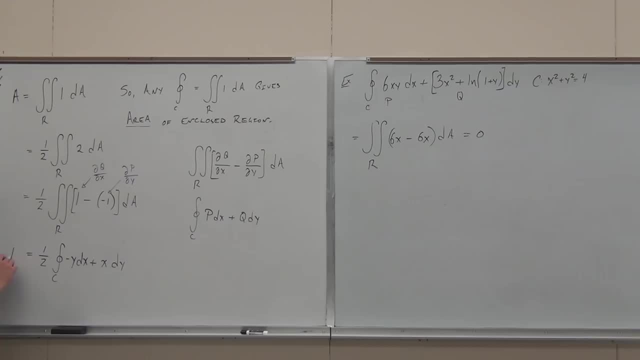 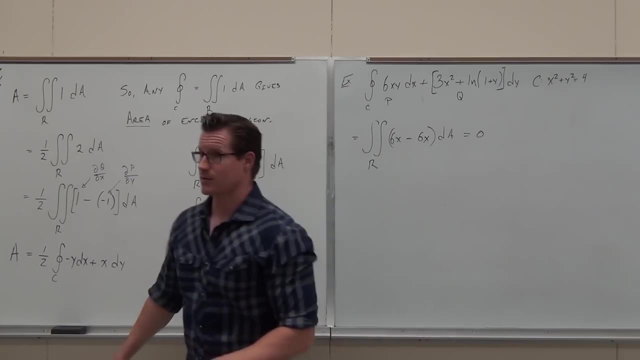 Then this is a formula for area. This is a formula for the- and you don't look excited. You should be kind of it's kind of cool. You're like, oh, I don't care, You should care. This is the formula for the area of any simple closed group. 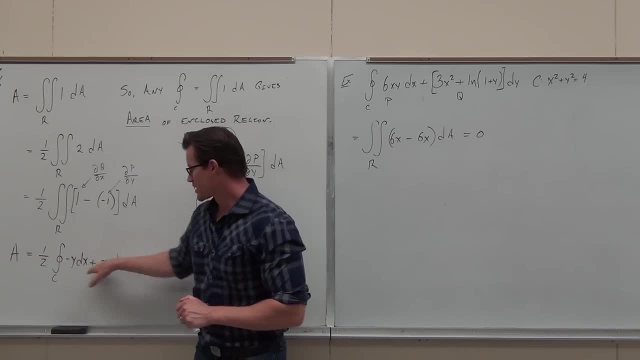 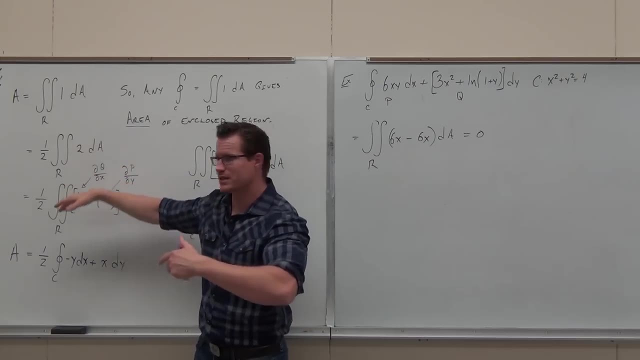 the region of any simple closed group. That's what that gives you. So where's it coming from? Kind of some math magic, granted, because I made it up. Well, I didn't. It's been around for a long time, but we just invented it. 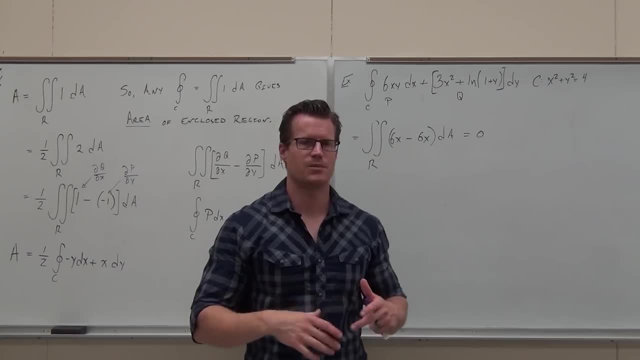 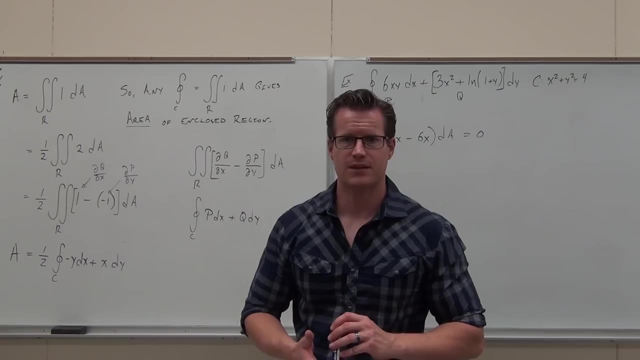 But that's a formula for the area of the region contained by a simple closed group. Are you guys okay with that? What that means is this: Take any simple closed group and, even if you have to re-parameterize it, you plug it in there. 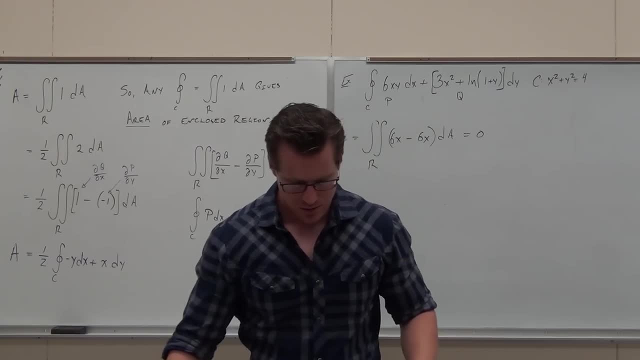 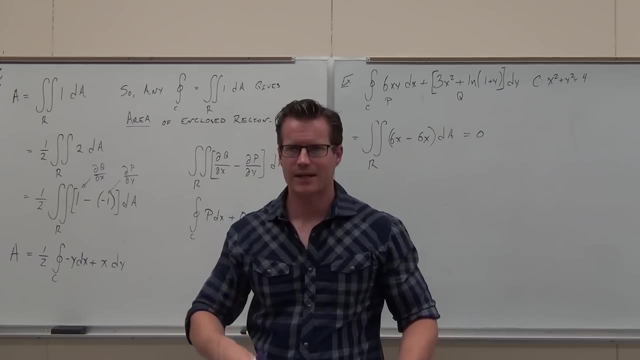 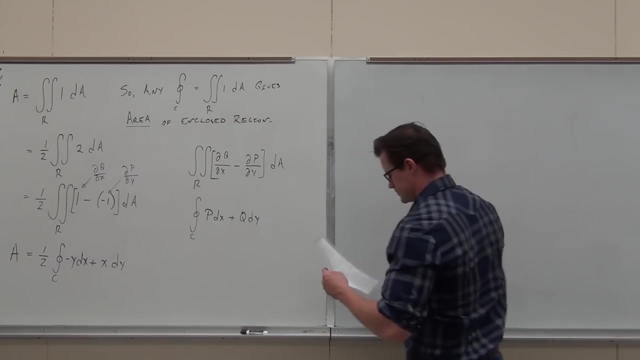 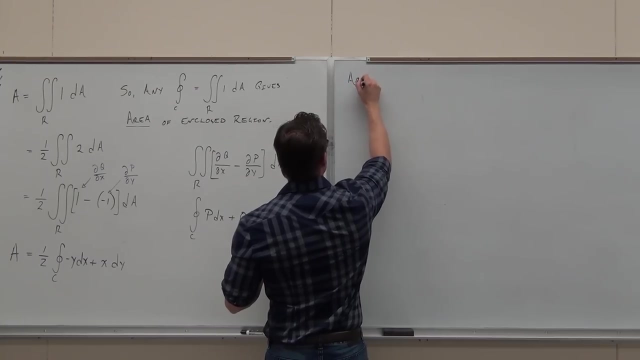 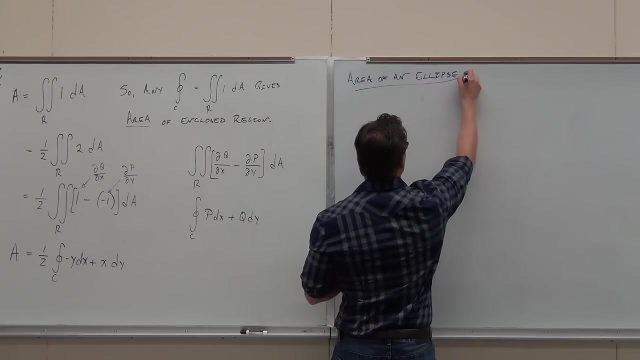 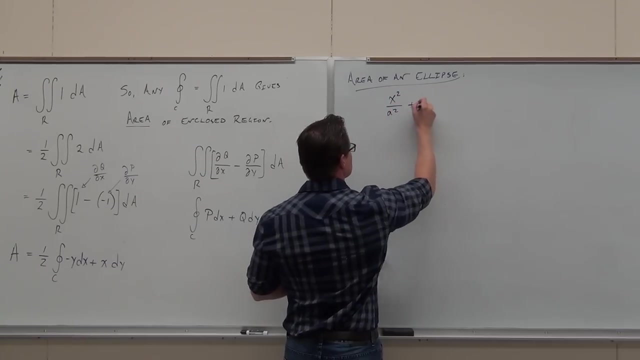 it's going to find the area. We're going to try that right now. We're going to try that with this. Let's say that we- Let's take a look at an ellipse for a second. That's your standard ellipse. Does it look familiar to you? 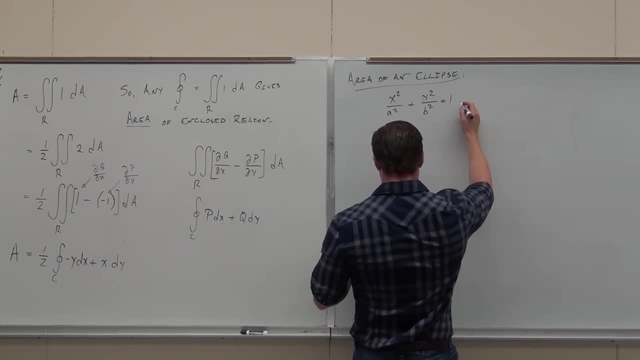 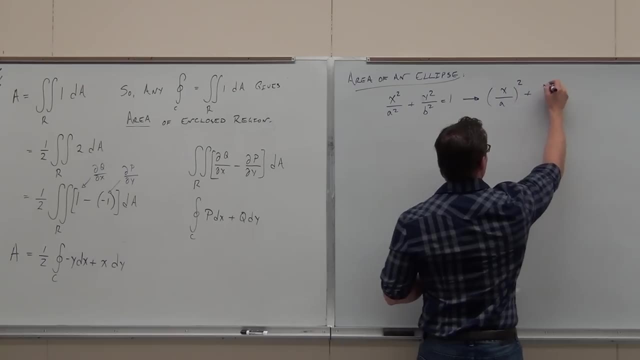 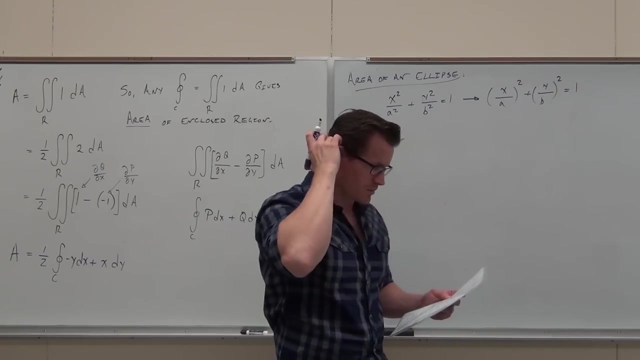 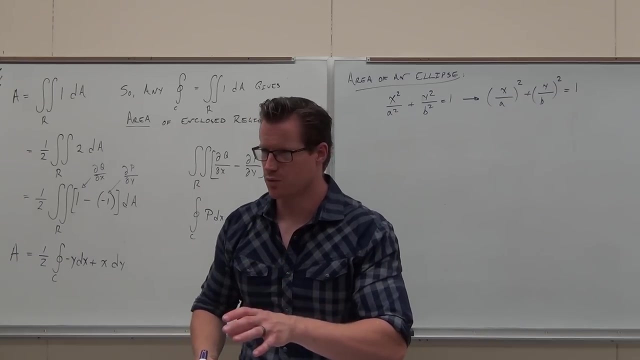 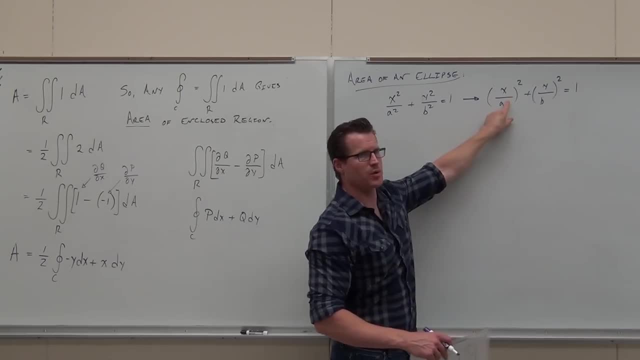 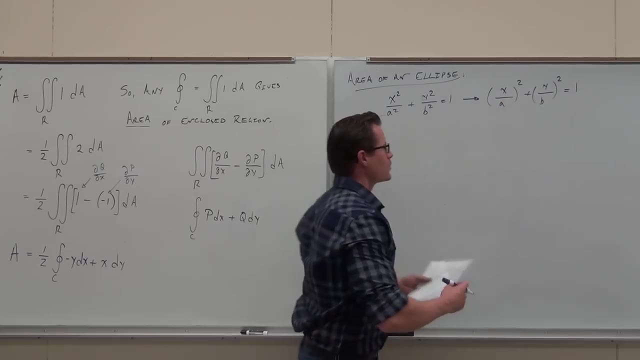 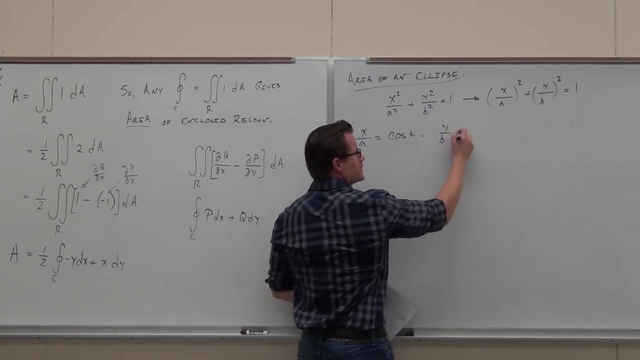 All right. so if you put all right and if you put write down on the top, we're going to have an ellipse. If you don't like the ellipse, you just have to read this one, If you remember. back to re-parameterizing things. 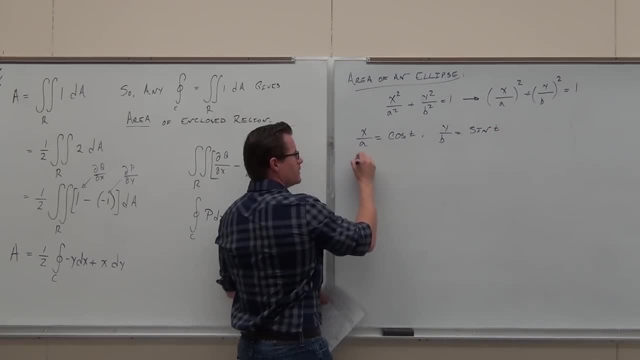 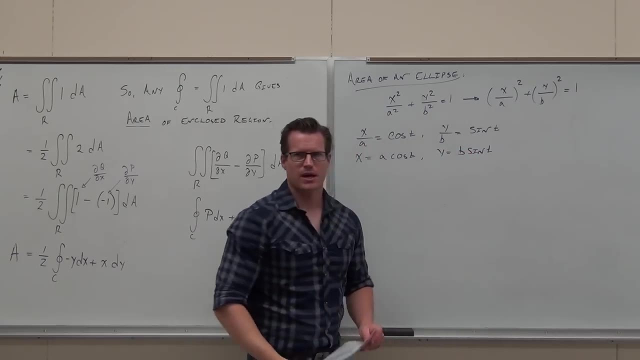 like circles and ellipses. any times we have something squared plus something squared equals a number. If I solve them, then X equals A cosine T and Y equals B sine T. Are you guys okay with that one? It's kind of basic reparameterization that you had in Calc 2.. 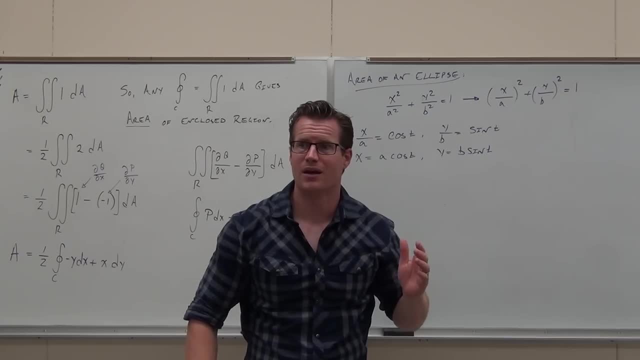 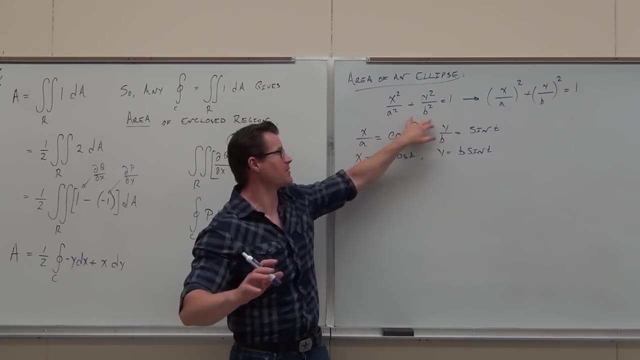 Now, what could we do with it? Well, here's the deal, If I can reparameterize. look, this is a general ellipse. I'm not making any statements about these right here. This is a general ellipse. I'm not making any statements about the values. 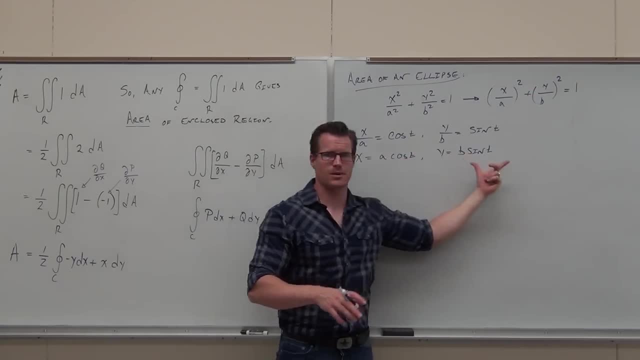 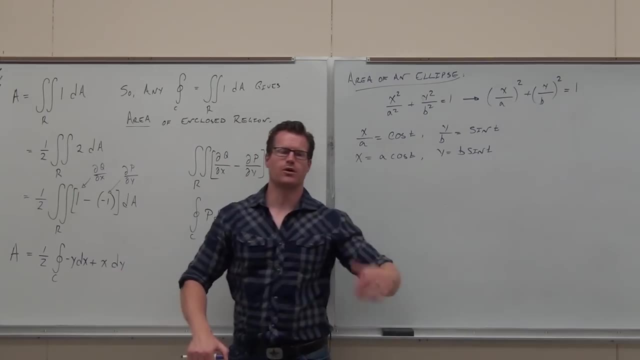 This is a reparameterization form: ellipse. I'm not making any statements about A or B. This is general. Does that make sense to you? Well, wait, If I want to find the area of the ellipse and true or false, an ellipse is a simple closed curve. 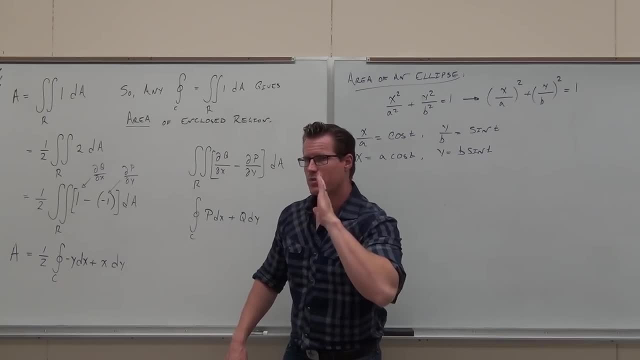 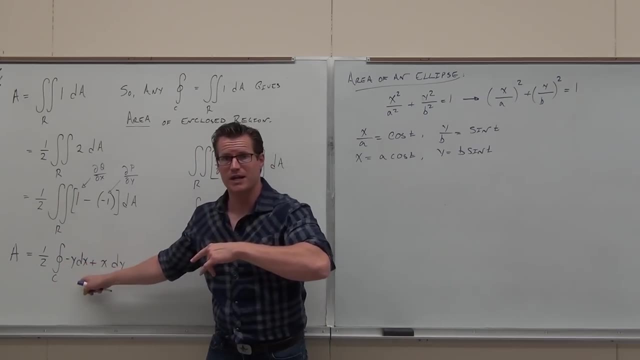 And if I want to find the area of that ellipse, if I can reparameterize the curve right there into X's and Y's, I can plug in those X's and Y's, It will give me the area of that curve. So we're going to try that. 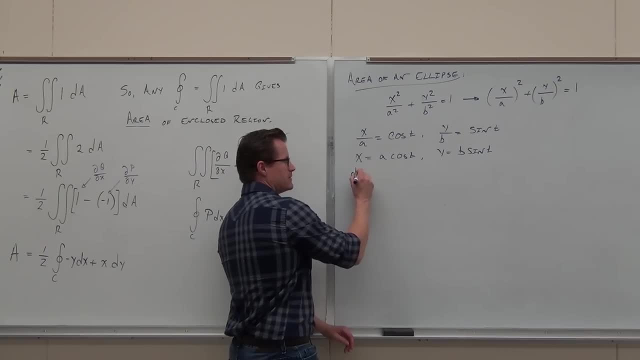 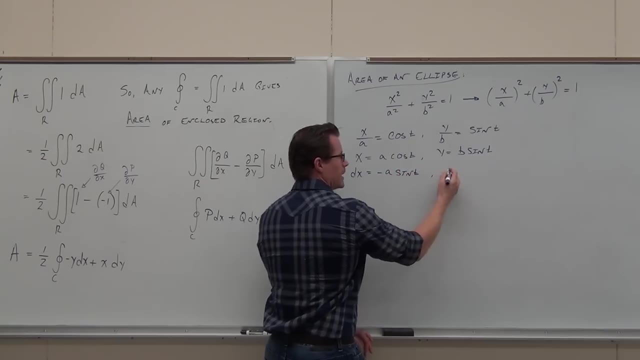 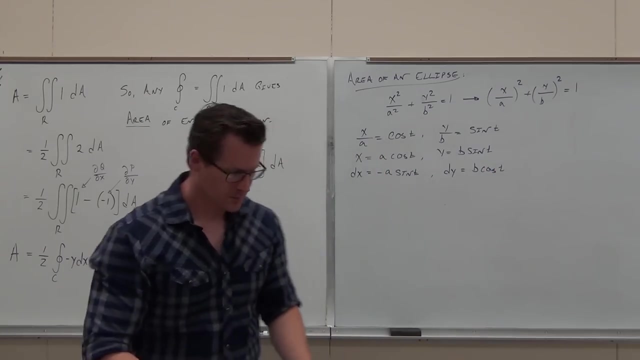 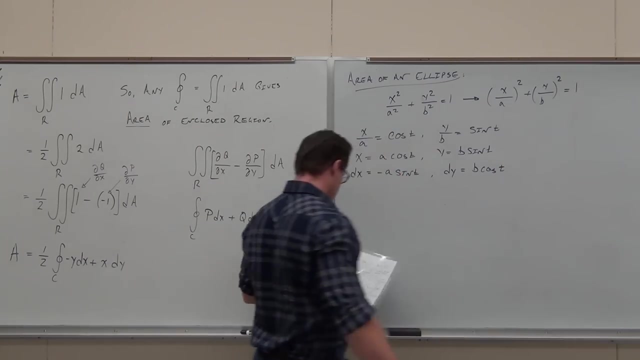 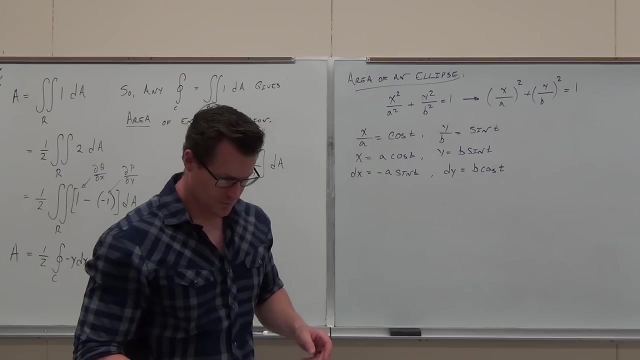 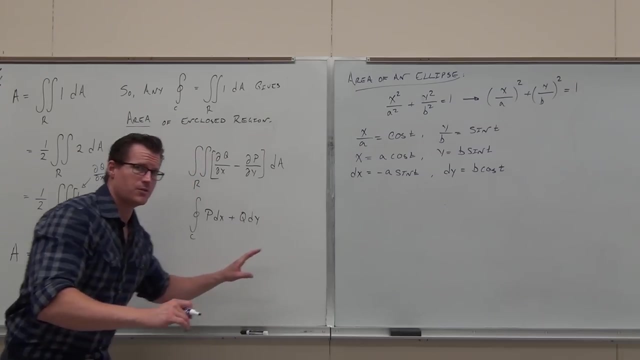 Okay, Well, in order to do it, I also have to have DX. You say, well, we have to have DX And I have to have DY. Okay Well, We're basically just reparameterizing this curve into something in terms of T, Everything's going. 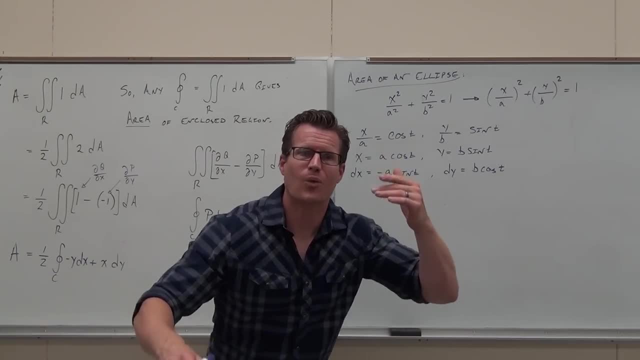 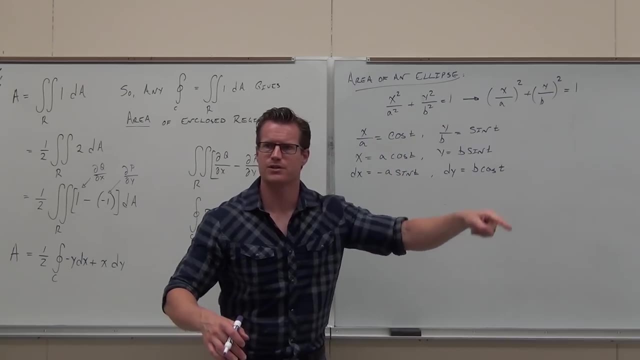 to be T. Does that ring a bell? Which means that all we need to know is what bounds of T give us that full curve. What's going to take us around the full curve of this ellipse? T equals what gives us around the whole circle. 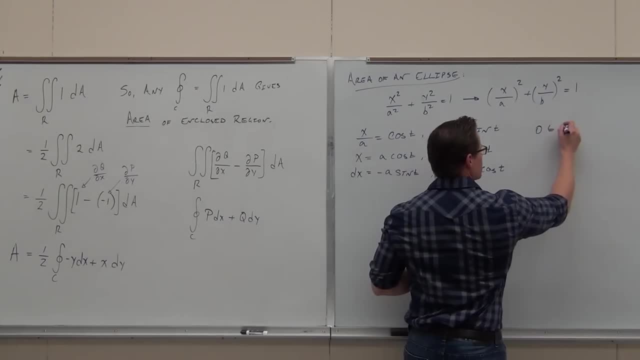 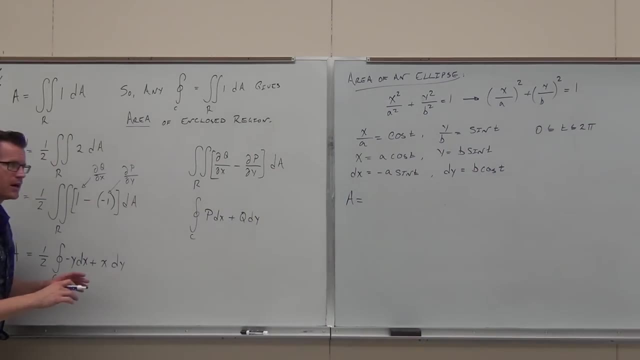 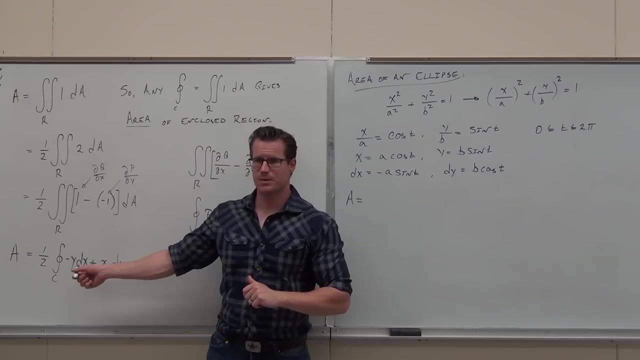 Zero to two pi. So our area. I'm not going to write it twice. What we're going to be doing right now is, for every X and for every Y, for every DX and for every DY that we find in here, we're going to be substituting it. 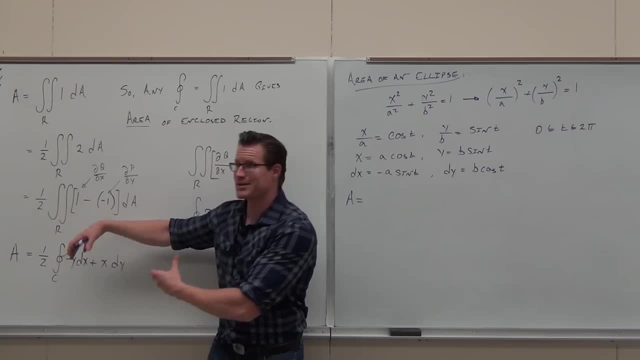 So we're going to be reparameterizing the whole thing. This is a formula, guys. It's going to give you the area that's enclosed by that curve. This is a curve, It's an ellipse, It's a simple closed curve. 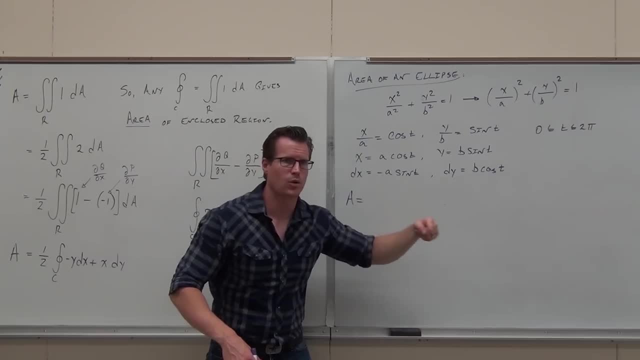 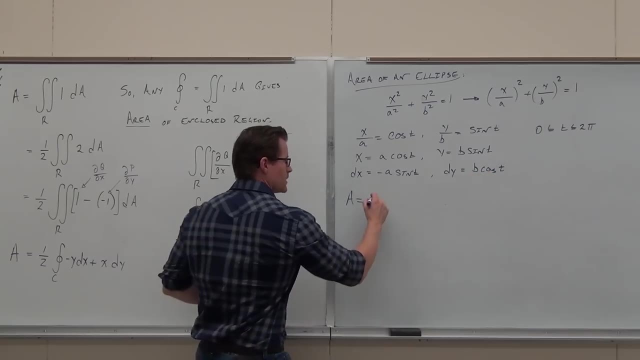 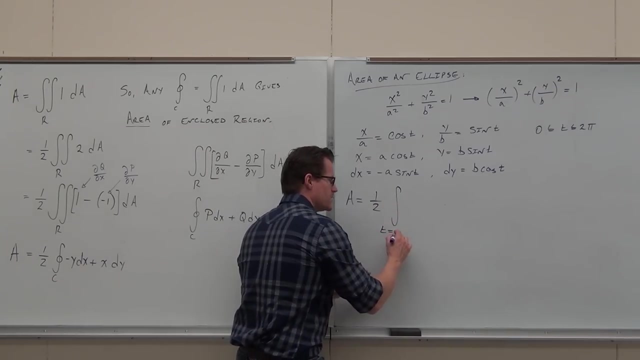 The zero to two pi for the T that we reparameterize in takes us around that whole entire curve. one time It sweeps out the entire area. Is this okay? So let's fill the formula out. What's a simple closed curve? Well, it's the curve that we've just reparameterized from T equals zero to T equals two pi. 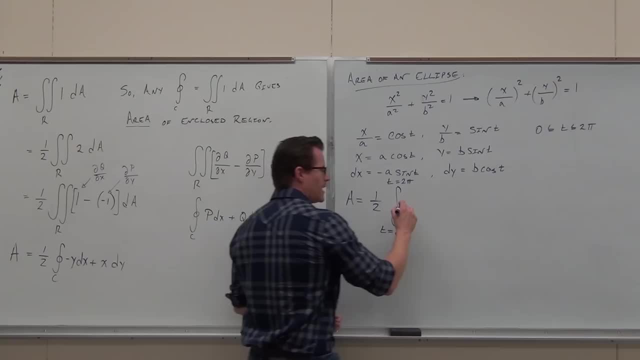 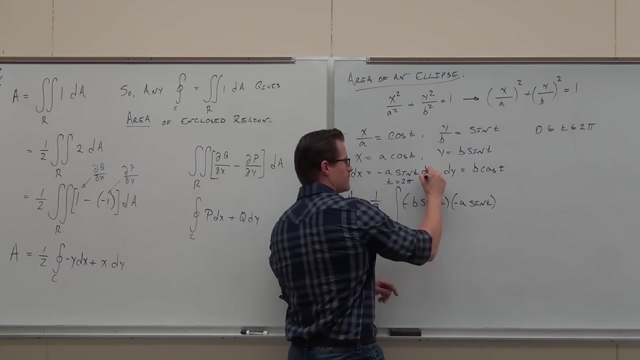 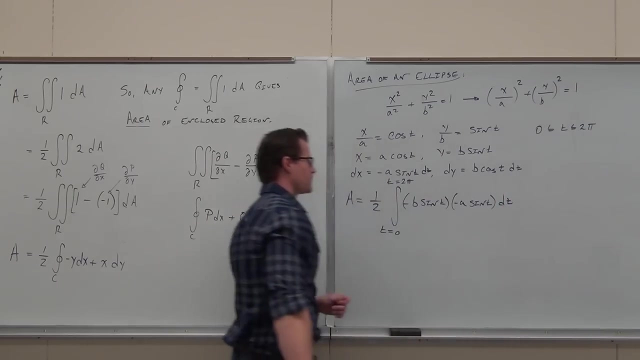 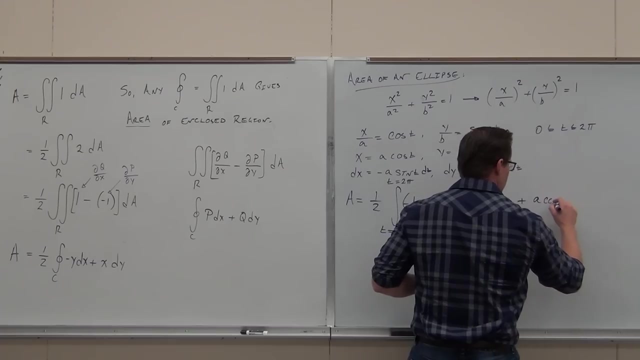 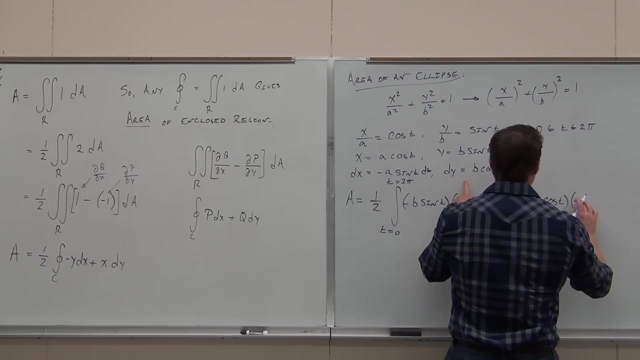 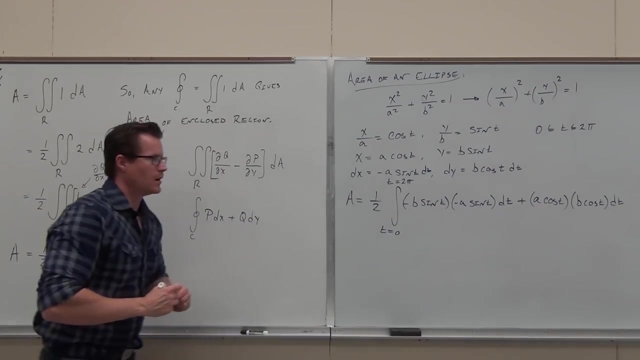 Inside, we have a negative Y, We have a DX, We have a Y Because we took derivatives with respect to T. we have a DT, We have a plus, We have an X, Then we have a DY. I want to make sure that you're okay with this. 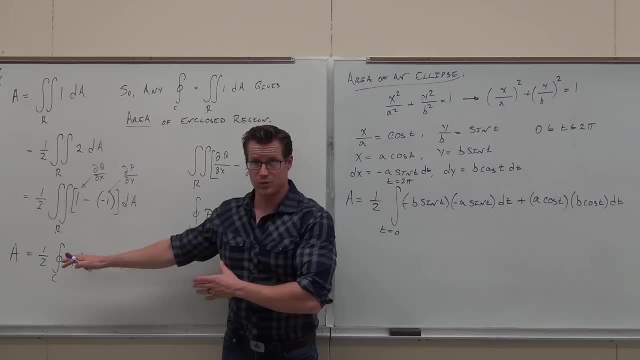 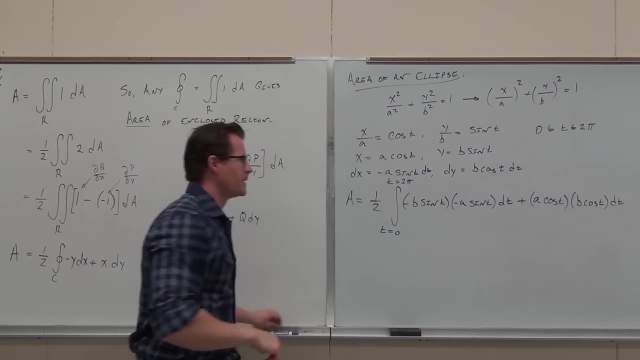 Do you see that? this right here is this formula as reparameterized by what we do, our ellipse Show of hands. if you do, you see that, Okay. So let's finish it up. Do you see all the beautiful things that are going to happen with this? 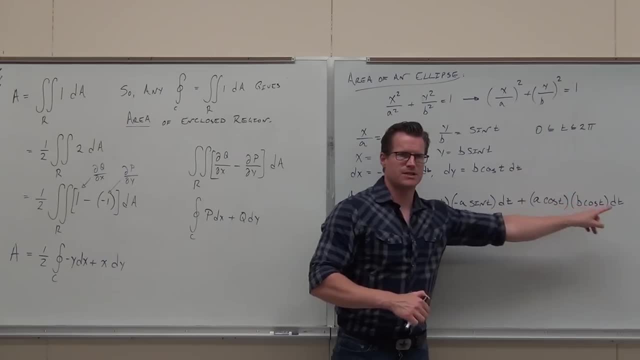 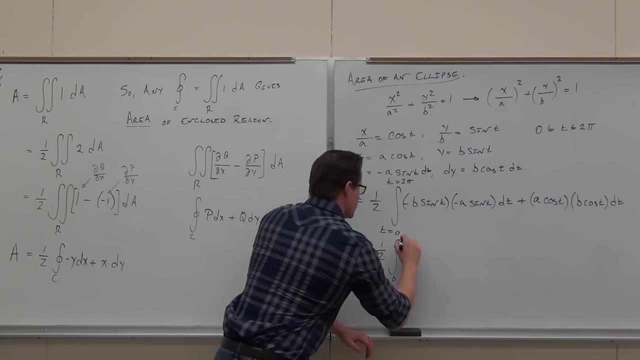 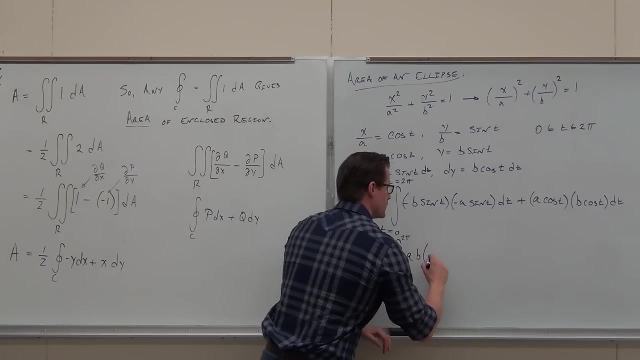 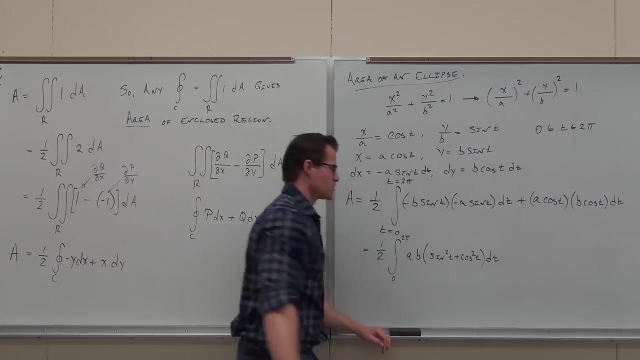 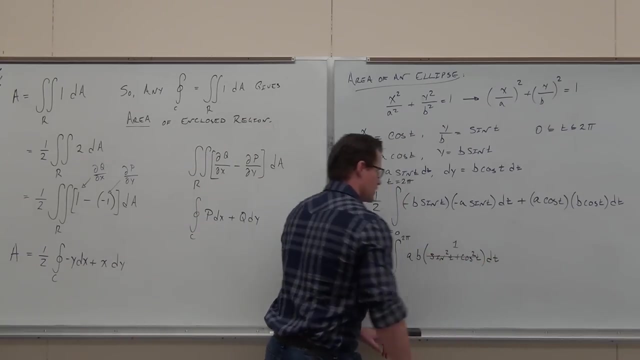 Negative times negative. Both of these have DTs. If I and both of these have A times B, Can you make the jump algebraically with me? Yes, no, How much is all of this One? So we end up getting one half. 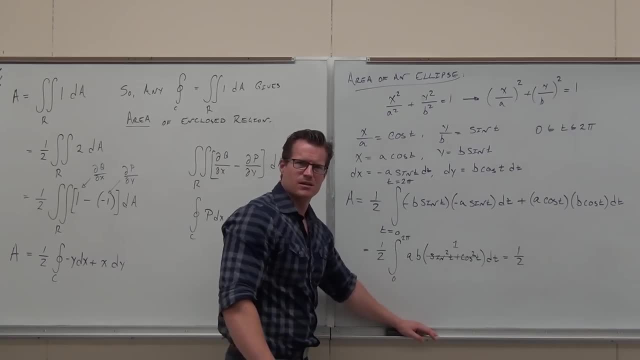 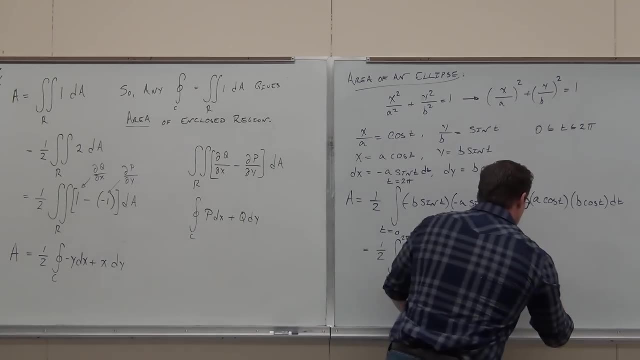 Okay, Fantastic AB. What's AB? What are AB with respect to T? What are those Constants? Constants? Integrate this with respect to T. You can pull AB out front. You're just going to get T evaluated from T equals 0 to T equals 2 pi. 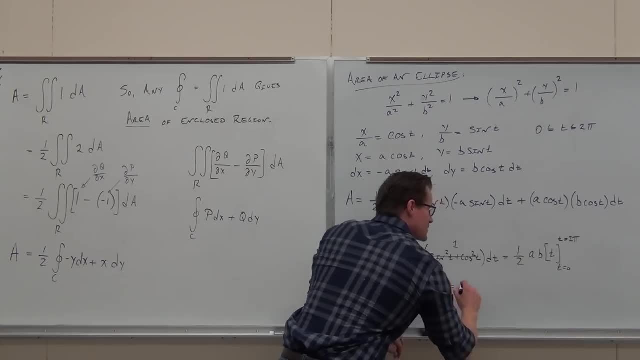 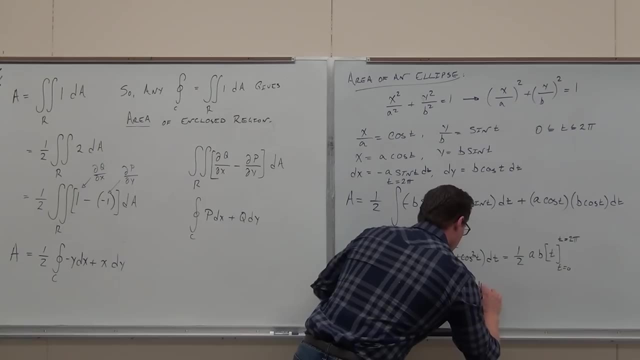 Looking pretty good to me. What this equals is: well, if I multiply by 2 pi, the 2's are gone. I get AB times pi And you go what? That is the area of an ellipse. Have you ever seen that formula before? 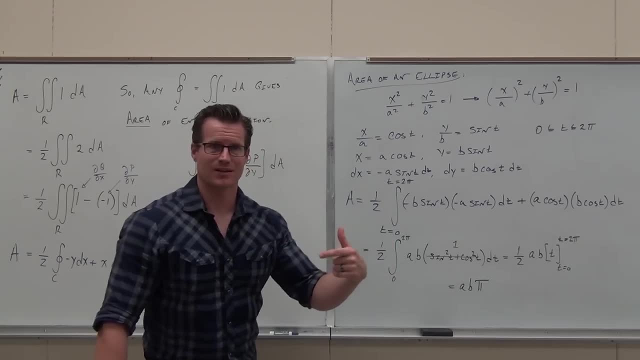 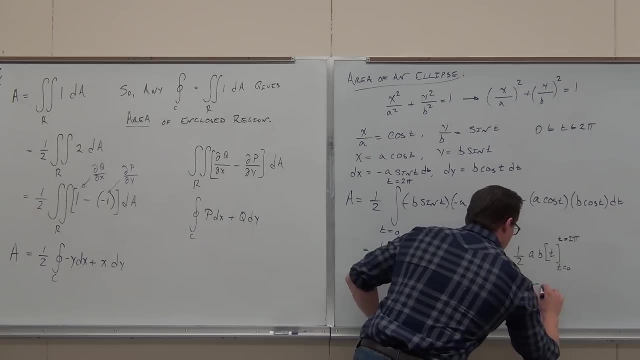 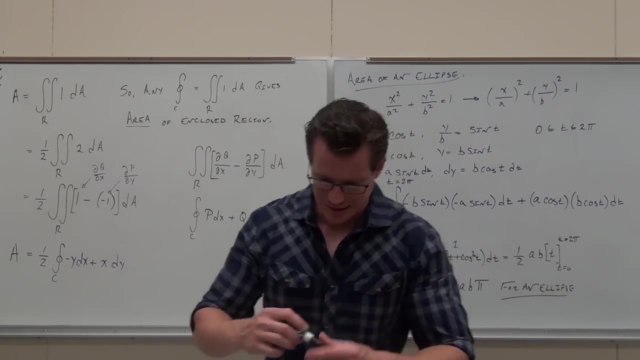 You might have, I don't know if you have. We just use calculus to solve that Analytic geometry. man, That's calculus. Boom Area of an ellipse. Now let's put it into practice. I want to do at least two examples on this so that you get a feel for it. 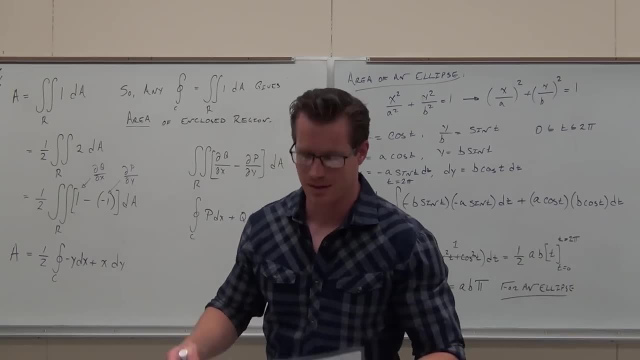 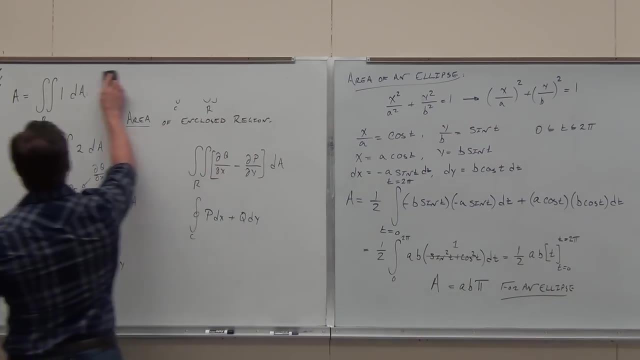 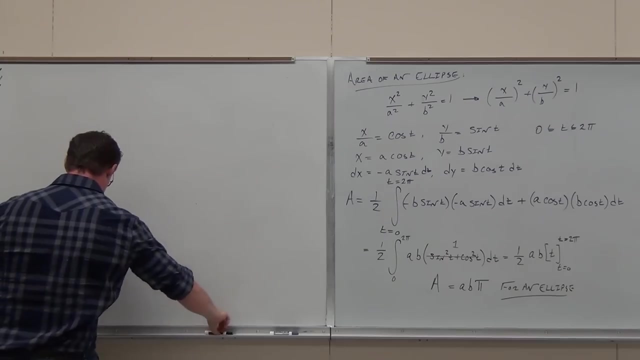 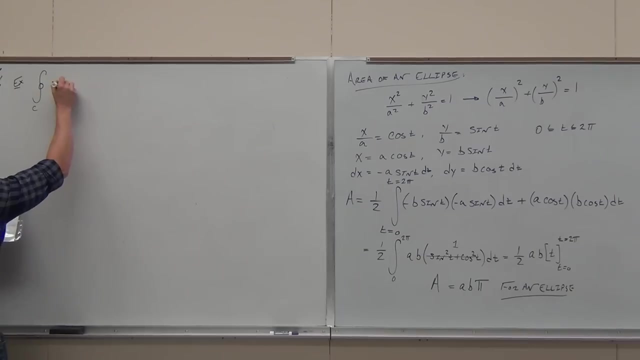 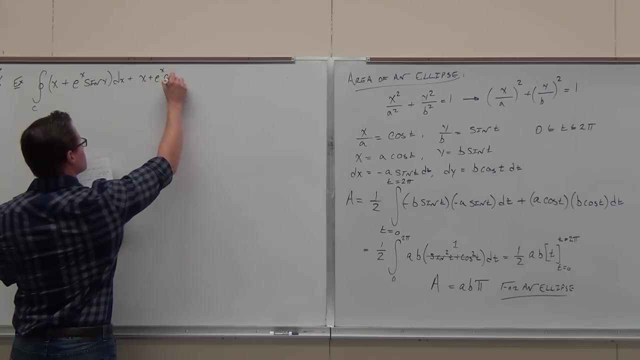 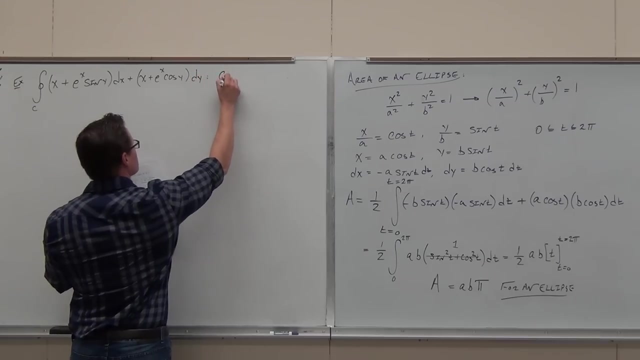 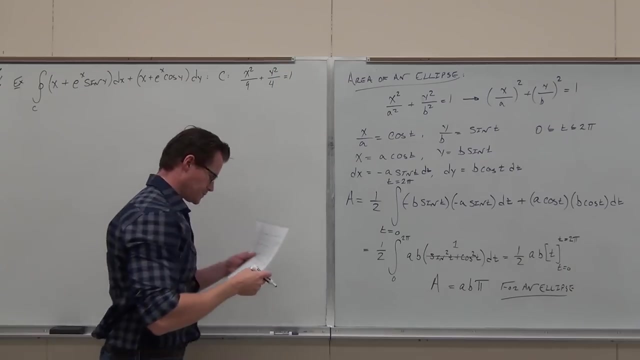 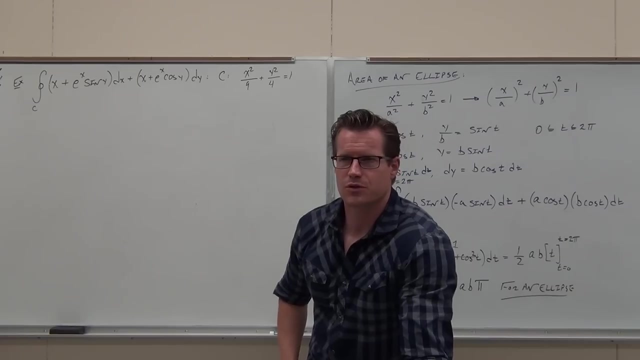 If we can do three or four, I'd love to. They go pretty quickly, but I think we're going to run out of time, So let's try one. Let's look at our curve- True or false? Simple, close curve. 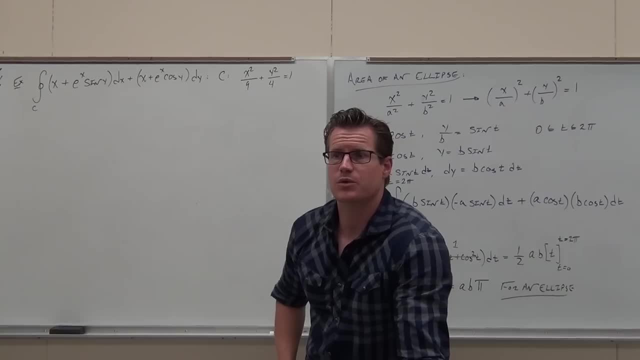 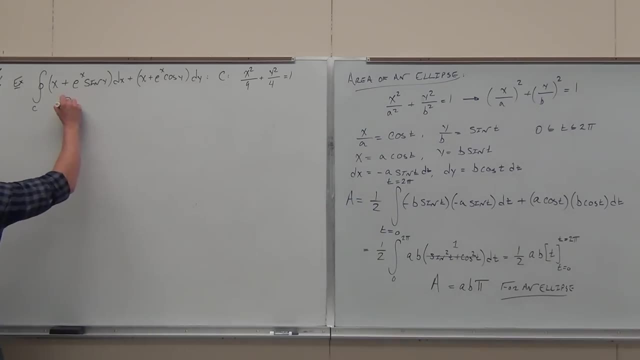 Does Green's theorem apply? Let's set up Green's theorem. Can you identify P and Q and set up Green's theorem? For the sake of time, I'm just going to help you out with it here. If we set up Green's theorem, you make the R every single time. 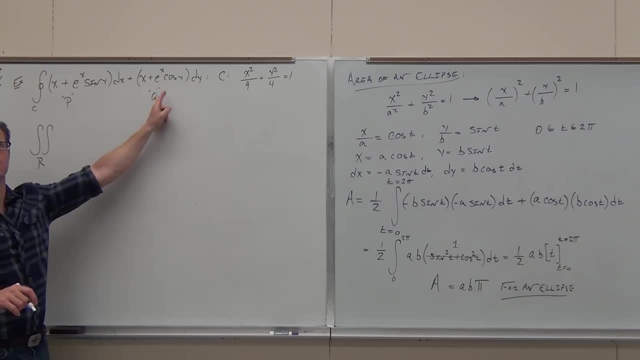 Take the partial derivative of this guy with respect to what, please, 1 plus e to the x cosine y. Do you see where it comes from? Minus, Minus the partial derivative of this with respect to what y, which would be e, to the x cosine y, dA. 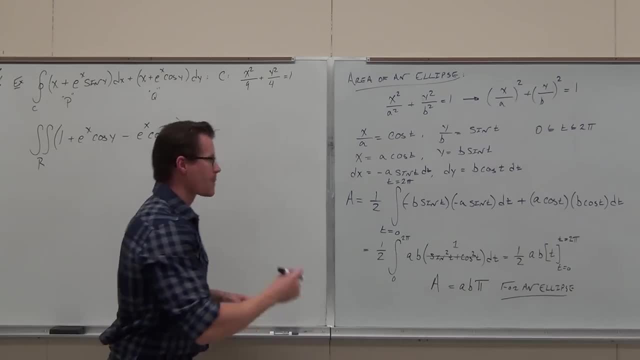 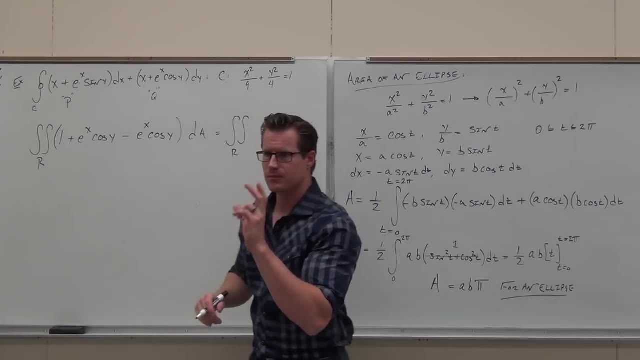 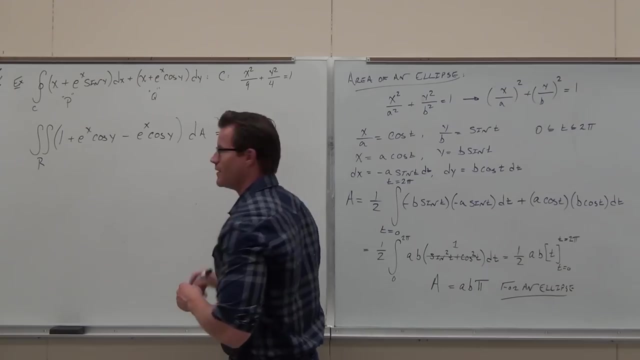 What does it give us? What's the argument to the integral? What are we going to have in there? Goodness, What happens? What's it mean? What's it mean? This is area. Area of what? Of the region? 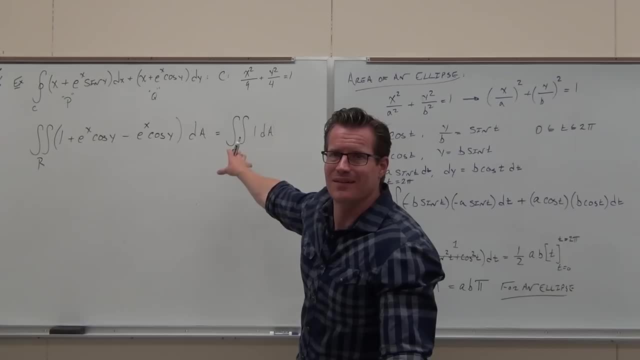 What's the region? Do you have a formula to find out the area of an ellipse? What's your a, What's your b? So the area of this ellipse, which is the region, Do you guys get it? That is the region that this simple closed curve contains. 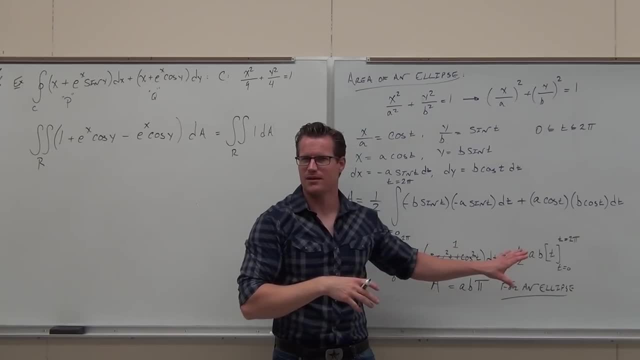 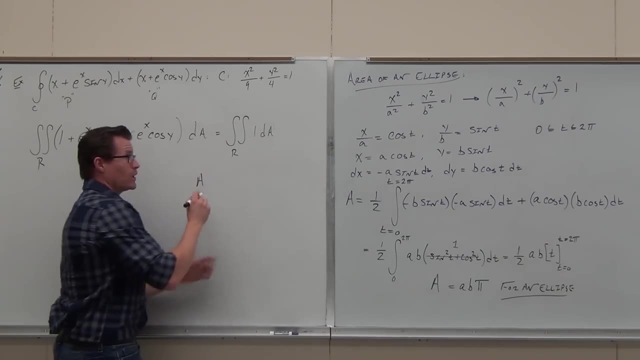 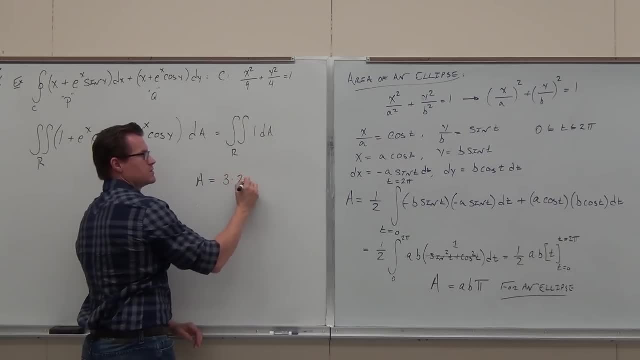 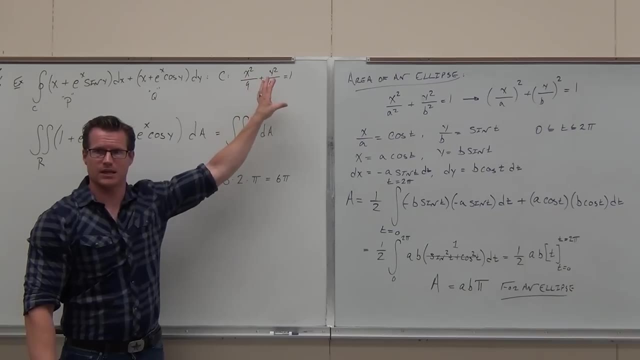 3., 3., 3., 3., 3., 2., 2., 2., 3., 2. 3.. We just found the line integral over that that ellipse by doing some kind of backwards work here. 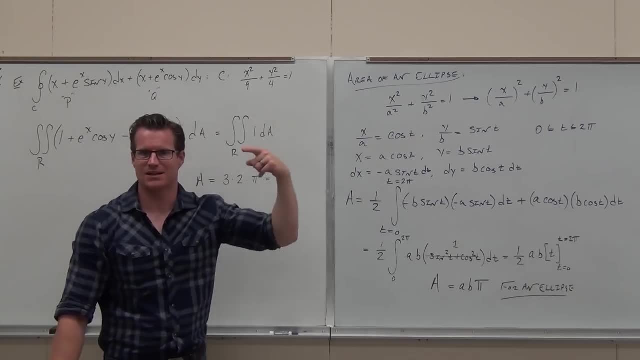 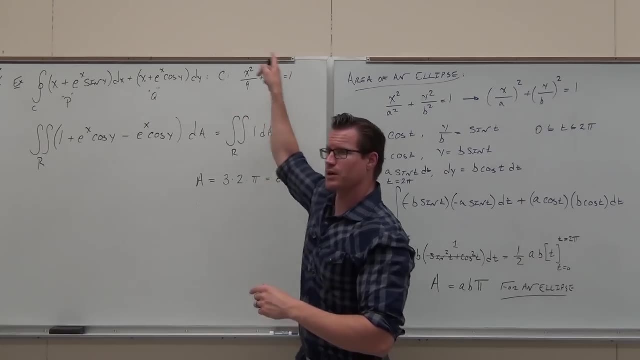 We found the area of the ellipse that that contains Isn't that kind of cool. So what's it mean? Well, that that's literally the work done. Going around that ellipse one time through whatever that vector field is, Make sense to you. 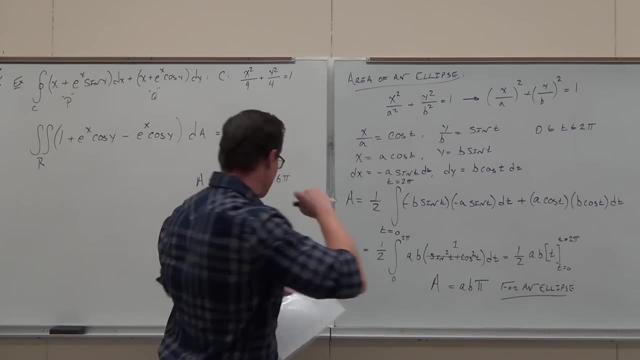 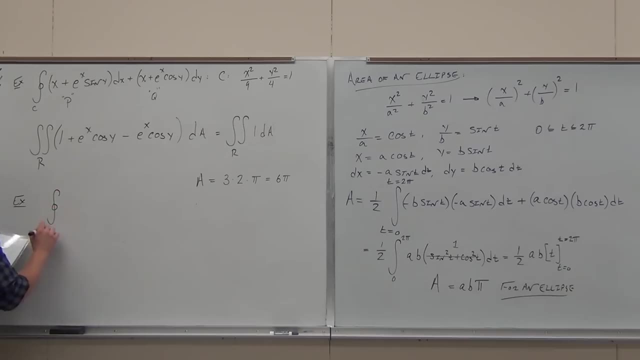 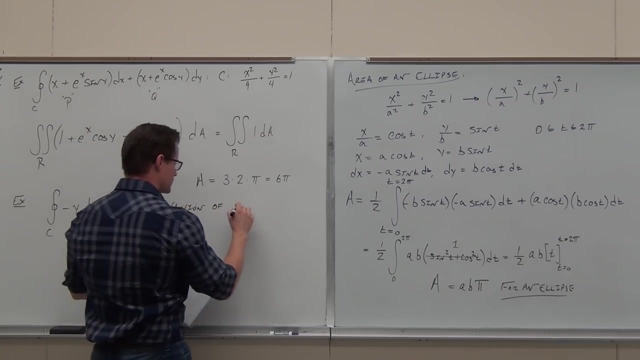 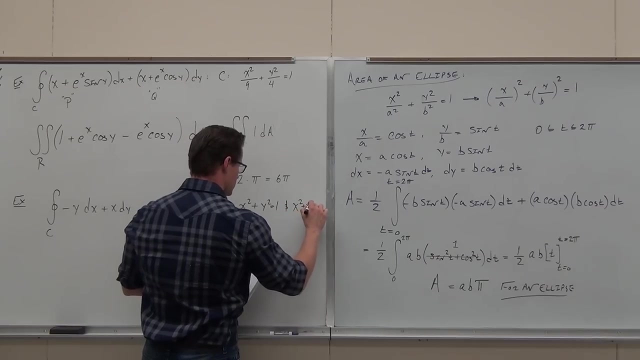 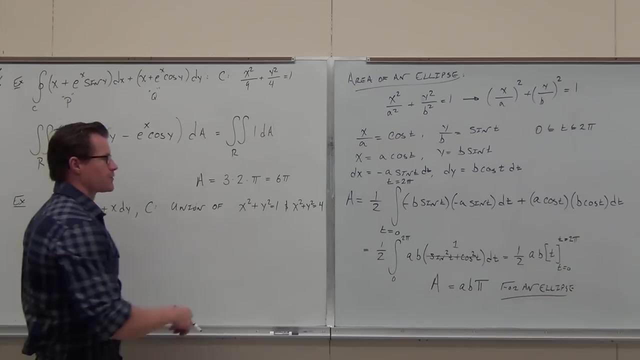 Let's go Here, we'll do one more, and then we'll probably have to call it good. If I can do one after that, I'll try it. After that I'll try it, but I don't think so. First, I want to think about our region. 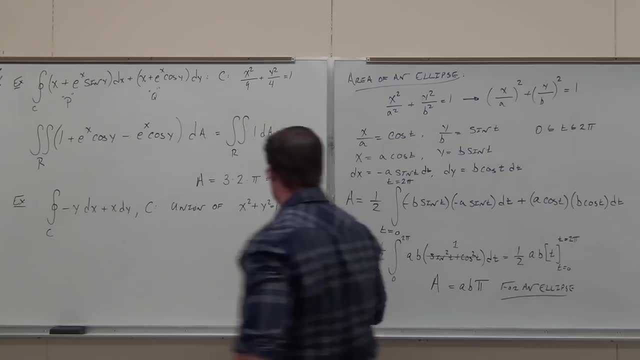 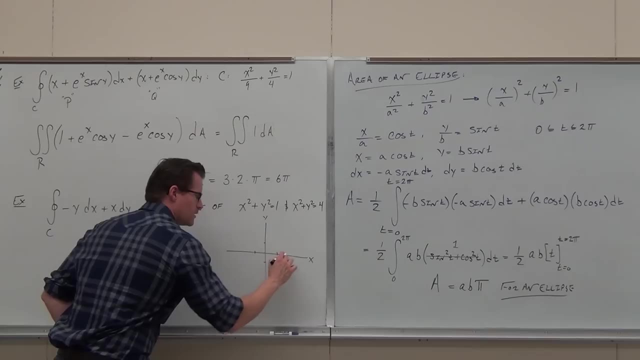 We don't have ellipses here. What do we have here? Let's draw these things. The union means that if we draw these, these are both centered at the origin. One's got a radius of 1.. One's got a radius of 2.. 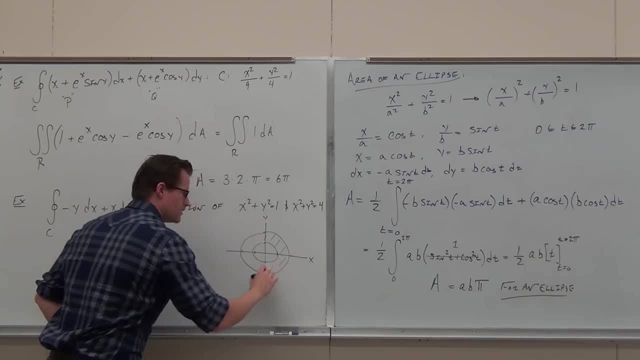 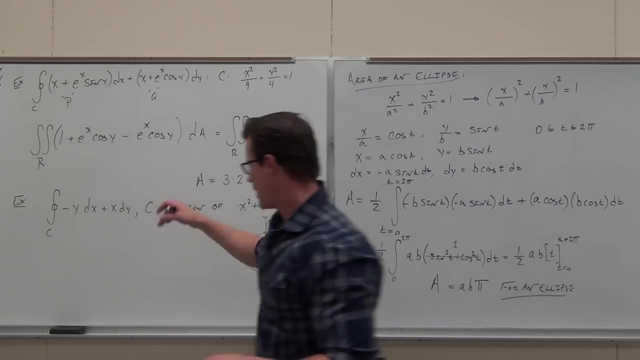 And what we're looking at is the area between those two things. Does that make sense to you? That's what we're looking at. Hey, let's see what happens here. Simple, closed curve, Well, yeah, but we're looking at the union of that. 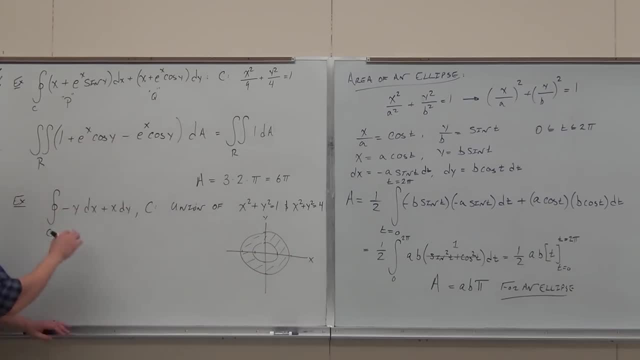 So this and that and this area between them? Well, let's see about this. If we try to apply Green's theorem, we have this P, this is Q. We get what? Oh no, no, be careful. The partial derivative of this with respect to X is 1 minus. 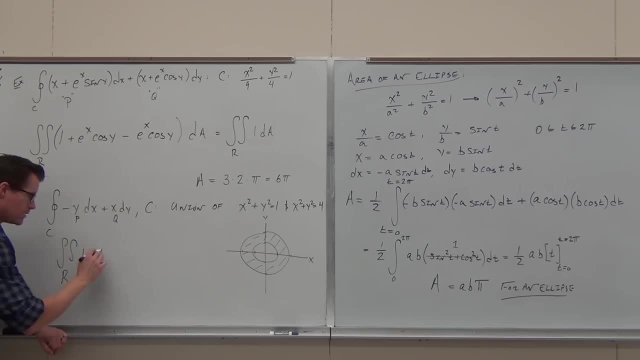 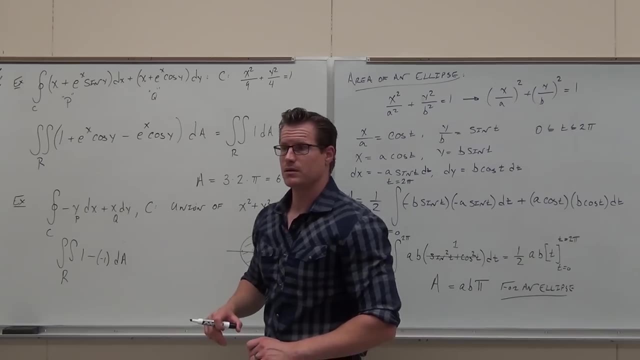 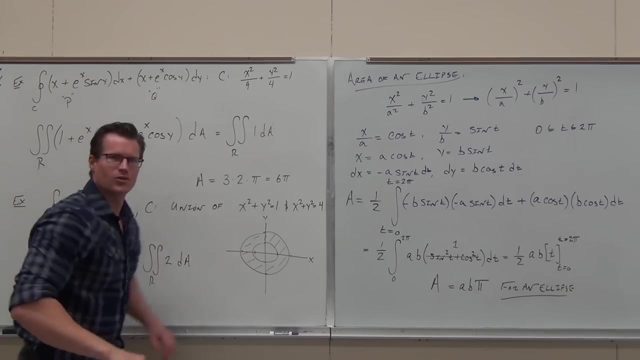 what's the partial derivative of this with respect to Y Zero, Zero? How much is it Two? Oh, but wait a second, I don't have anything that says about 2.. What can I do with the 2?? Take it out. 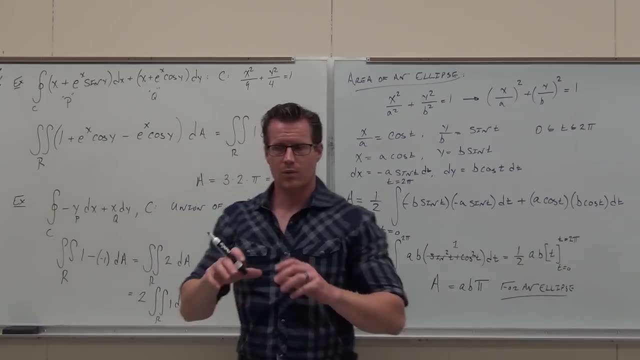 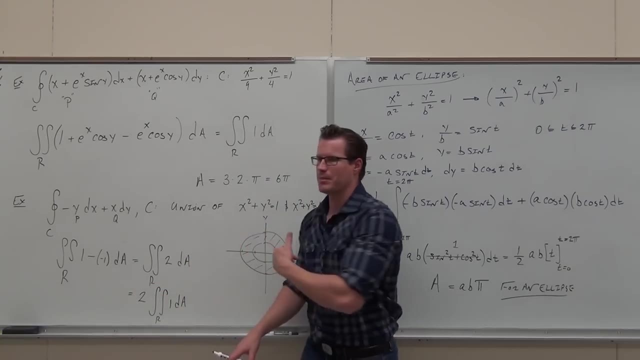 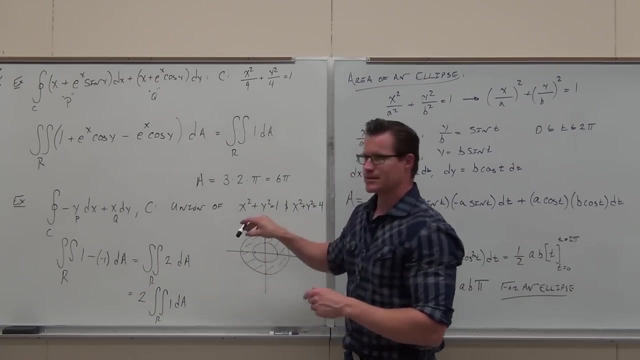 We're doing some pretty cool stuff here, folks. What we have here is 2 times Whatever the area of this region happens to be. That's what that line interval is going to be. That's what that says, The work done by traversing this and that. 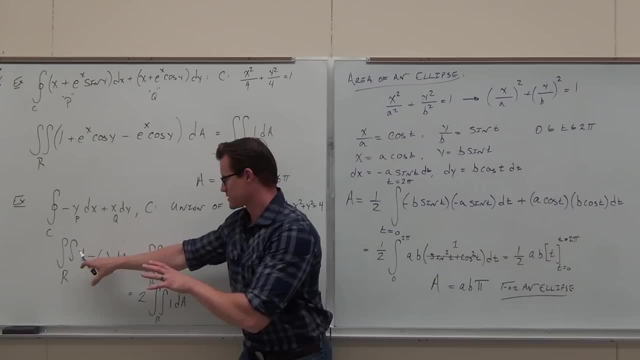 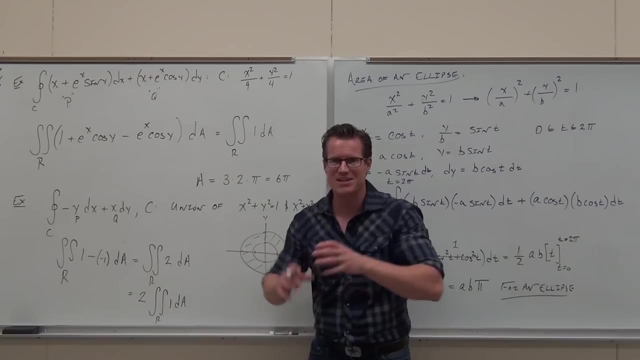 That's the idea. So okay, well, if we can figure out that this is Green's theorem, make it 1. This represents this area of that region that's contained by those things. Well, how do you find the area between two circles? 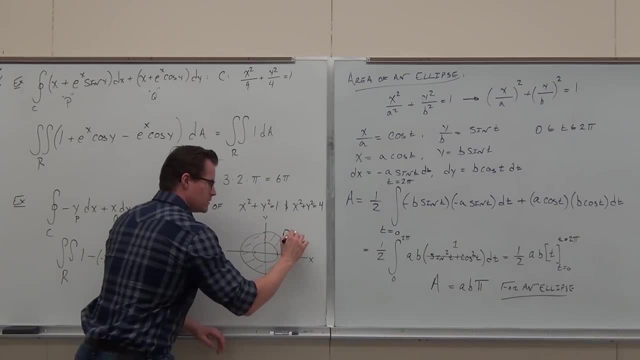 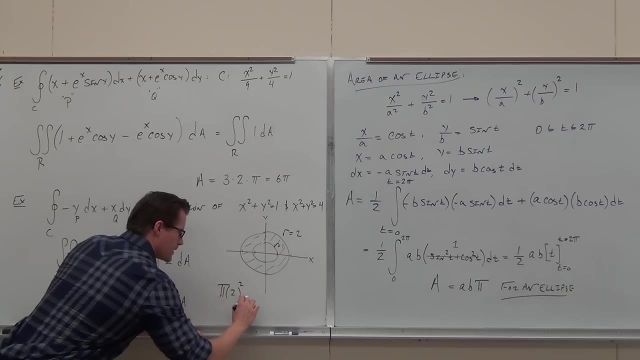 Well, okay, what's the radius of this circle? What's the radius of this circle? Well, pi r squared minus pi r squared Three, three, well, almost three pi. This would be. do you guys see where the 2 and the 1 are coming from? 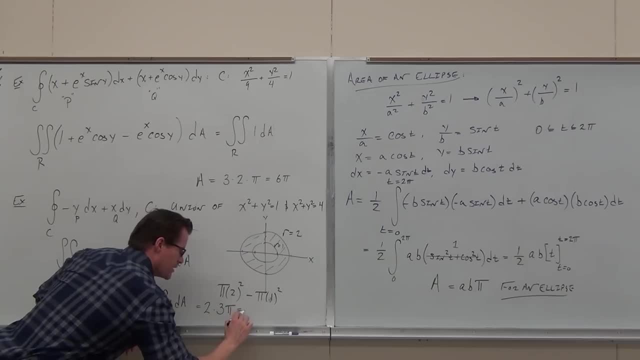 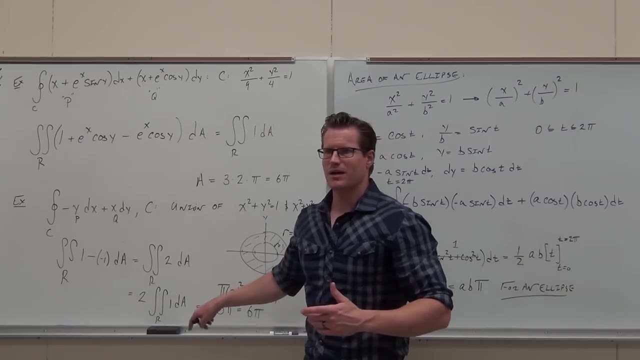 Well, this is 2 times 3 pi, 6 pi. I promise they don't all come out to 6 pi. Okay, just coincidence, here That comes out to 6 pi. We can use area because it represents area. 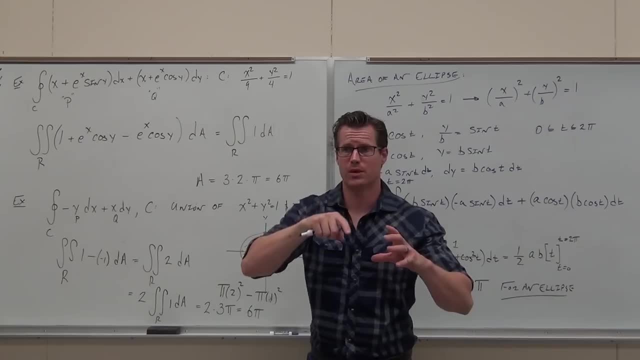 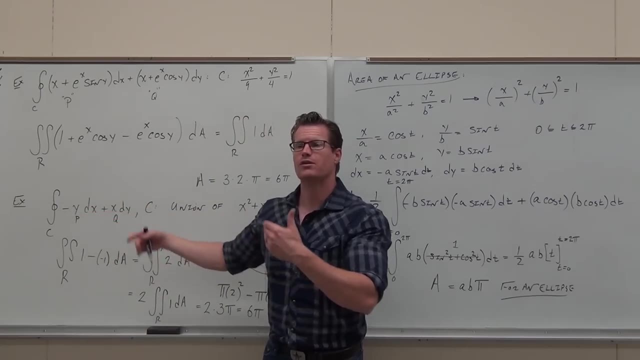 What this double integral over the region with an integrand of 1 represents is area of the region. If the line integral by Green's theorem also represents the same area, then we're solving line integrals by finding area. Does that make sense? 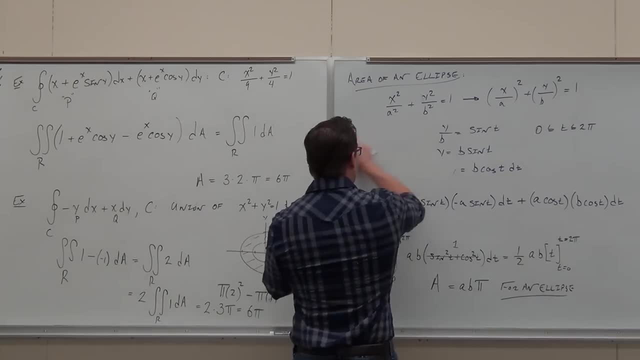 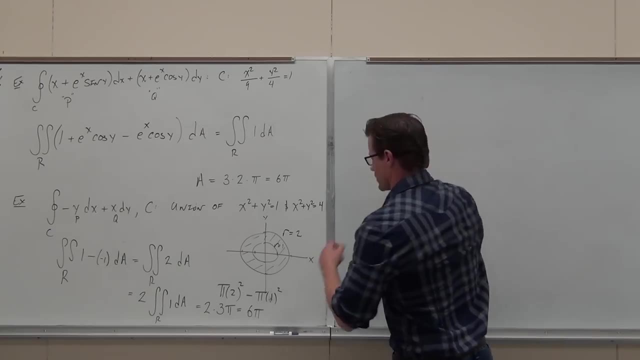 Let's say, if you didn't get any like- oh my gosh, I don't understand any of that- Could you still set up double integral? Well, sure, If you from right here, if you had 2.. 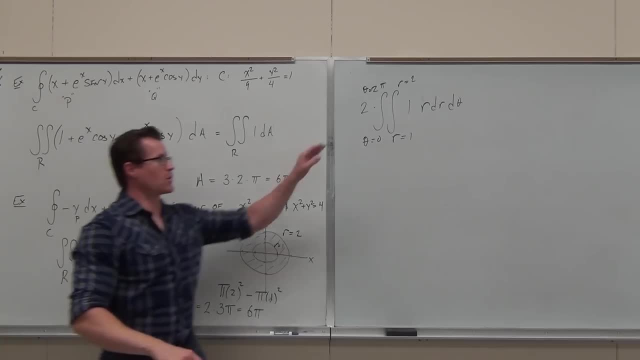 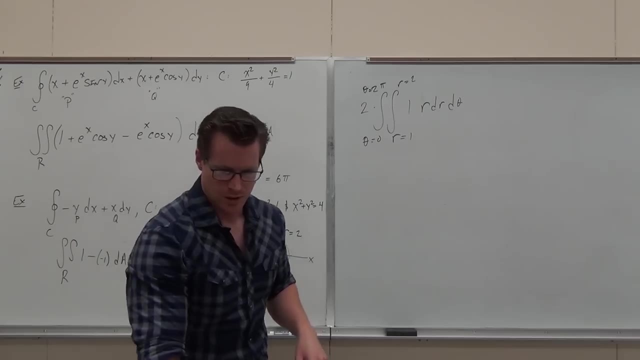 DA. this is why we always write it every single time. DA changes to rd, rd. theta You're now using polar R goes from starting 1 to 2.. We're going all the way around that joint circle, If you can see it. 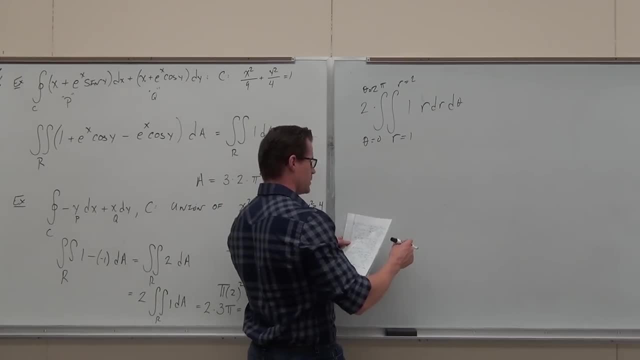 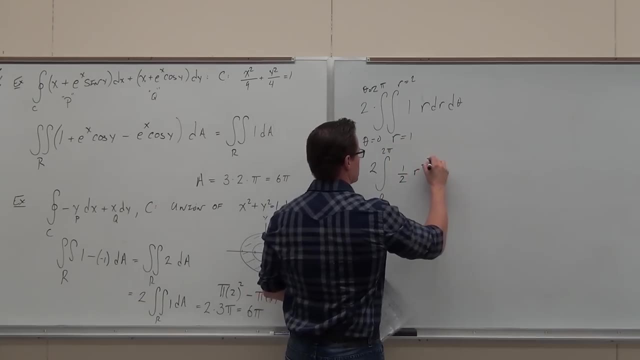 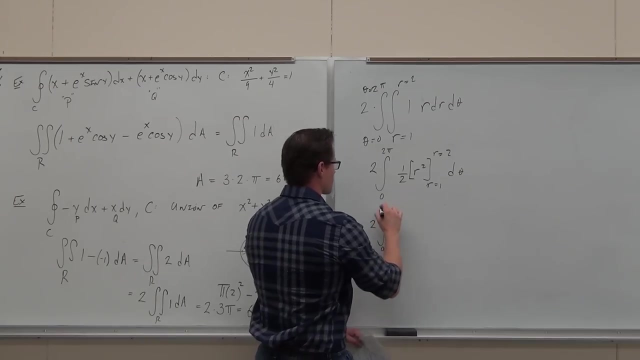 If you can see it, This would end up being: let's see, Actually, let's do that. 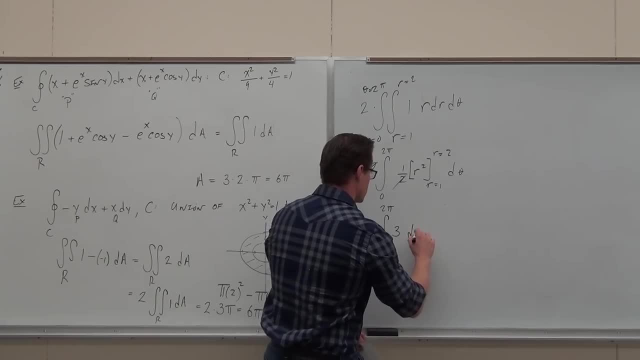 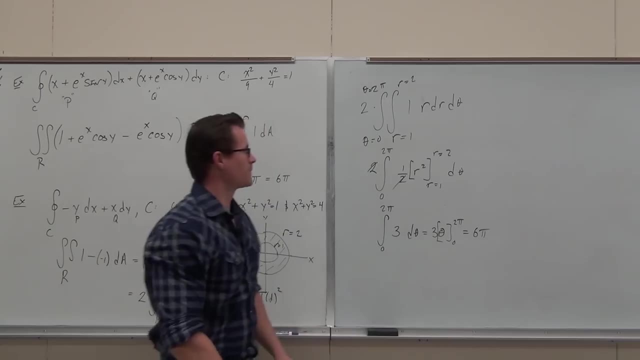 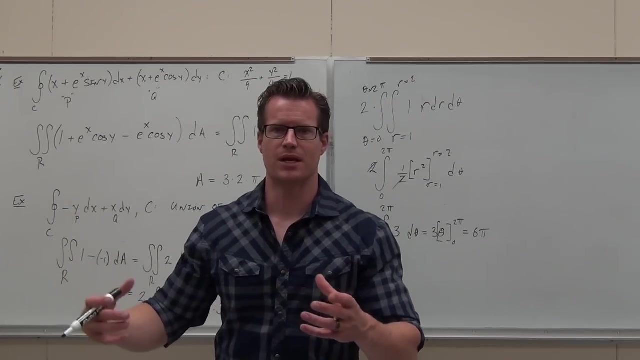 It's the same, It's the same concept. They represent the same thing. What I'm trying to get you to see is that they represent the same thing. 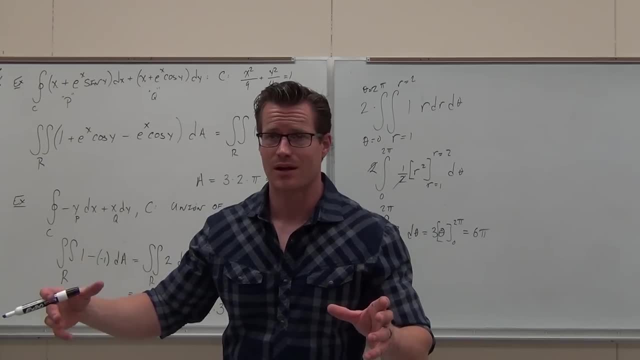 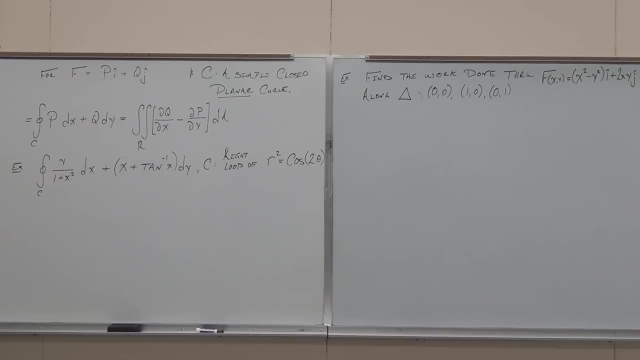 Have I done that? Do you understand the concept? I'm trying to get you to understand The idea of line hundred rules into double hundred rules. That's the Green's theorem. I'll finish up the rest of it next time. The last two examples from the Green's theorem: 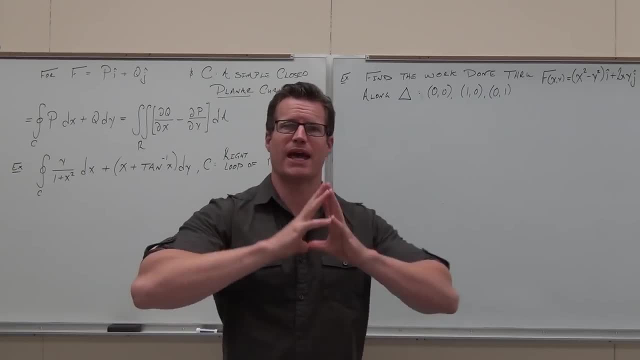 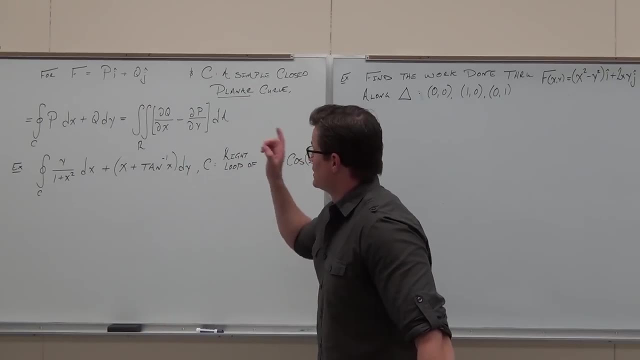 Let's review what Green's Theorem means very quickly. We're going to do our last two examples and I'll introduce you to the rest of the world for Calculus 3, what this all means. So what Green's Theorem says, if you have this vector field. 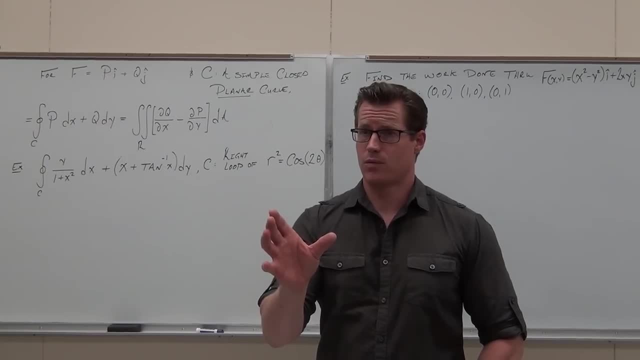 what type of vector field does it need to be for Green's Theorem to work? Conservative Right, because it's a vector field and through this vector field we're having this simple closed curve. And if we had a conservative vector field and started? 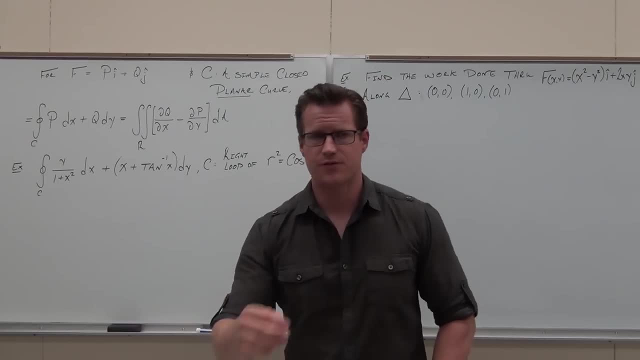 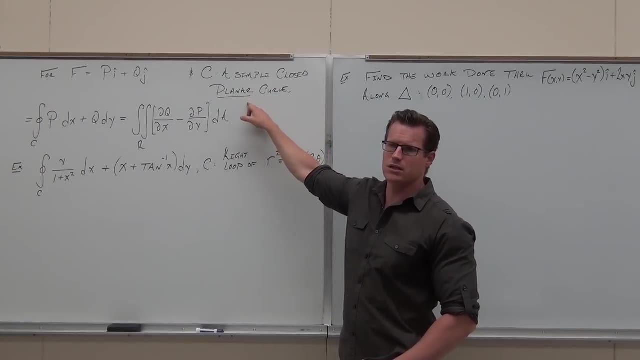 and ended in the same spot. we'd do zero work, And what Green's Theorem says is: find the amount of work that's done on a simple closed. this is a big word. can you please make a note? we talked about it earlier. 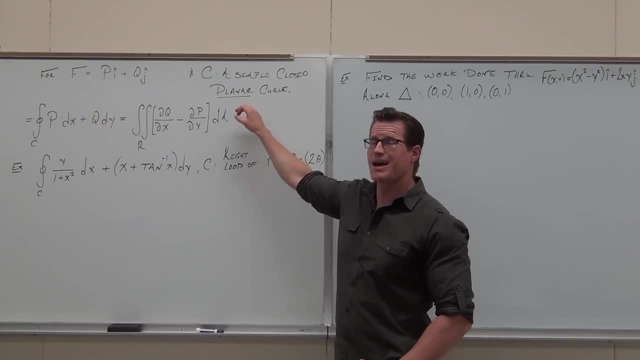 but I didn't make you write it down. we talked about how the curve for Green's Theorem it's on a plane. It's a planar curve. It is on a plane When we get into the next few sections, like Stokes' Theorem 15.9, it does not have to be on a plane. 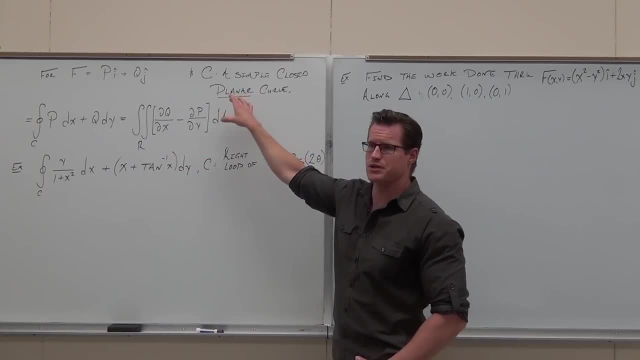 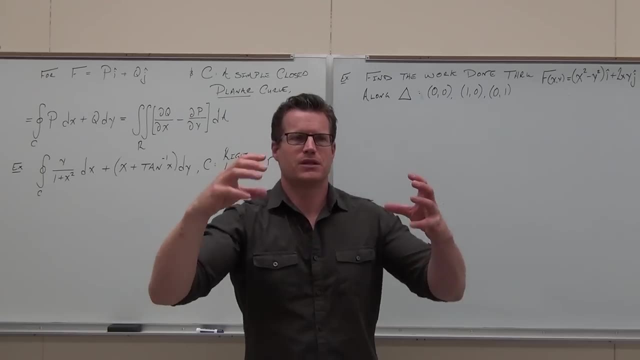 That's the main difference between them. okay, So this is a planar curve. for Green's Theorem to work, It says: if you're taking this simple, closed curve through a vector field- and it's a conservative vector field- you'd get work done at zero. 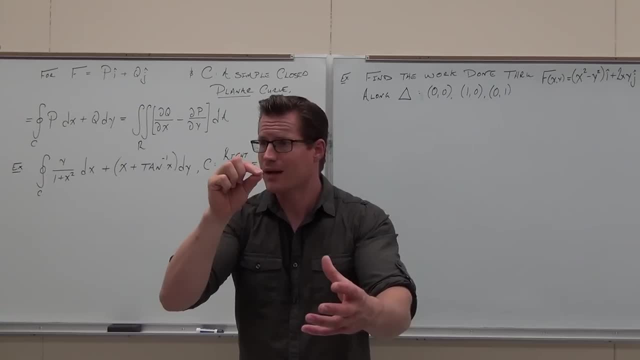 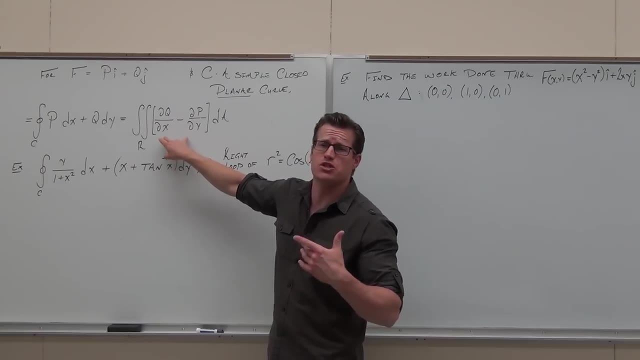 Start at the same spot, do some work and at the same spot, you're doing nothing on a conservative vector field. That's why this would look really familiar. If you have a conservative vector field, this is literally how you would check it. 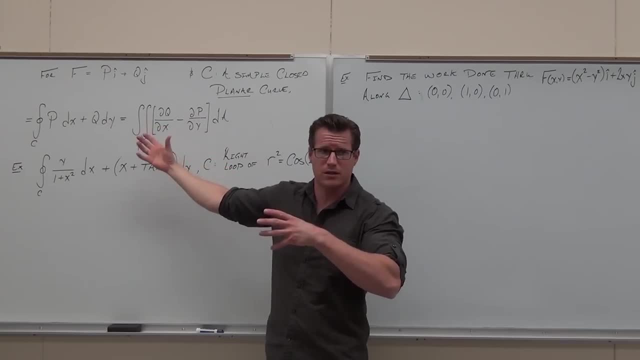 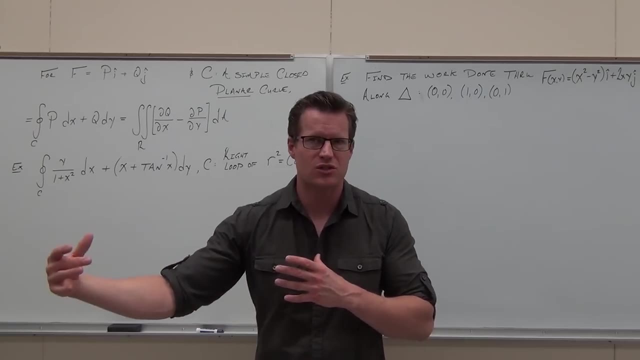 You'd check these two pieces and see if they're equal. If they're equal and you subtract them, you'd get zero And Green's Theorem kind of intuitively checks for conservative vector fields. You don't really have to even know if it's conservative. 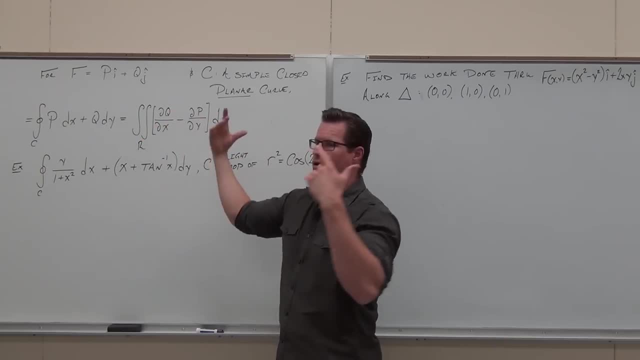 because it does it automatically. Does that make sense? And if you get zero you go: oh hey, simple, closed curve, conservative vector field, done zero. That's pretty easy. If it's non-conservative, this is relevant. 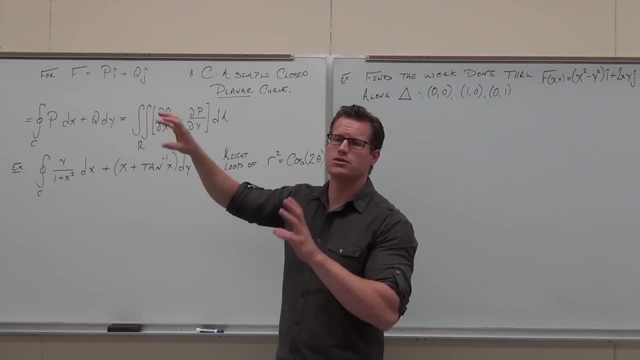 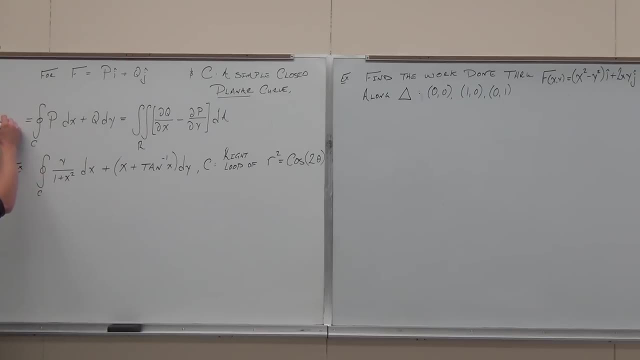 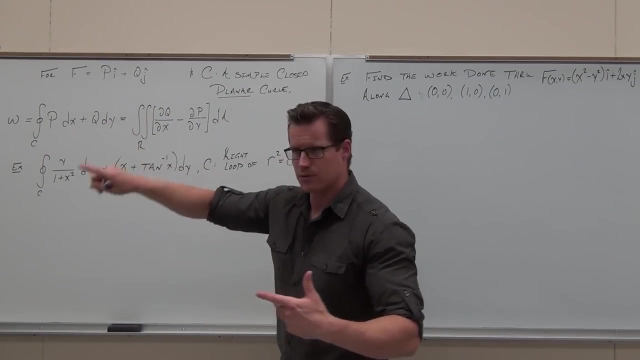 and this is what Green's Theorem says to us. If we have a non-conservative vector field and a simple closed curve, planar curve, going through it, this would represent a line integral or the work done through a vector field along a simple closed curve. 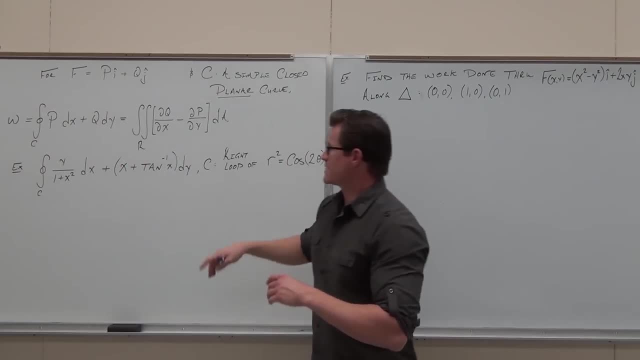 That's what that gives us. That means Green's Theorem gives us the same thing. That means that if we can determine we have a simple closed curve and we have a vector field, we can always set up Green's Theorem really nicely. 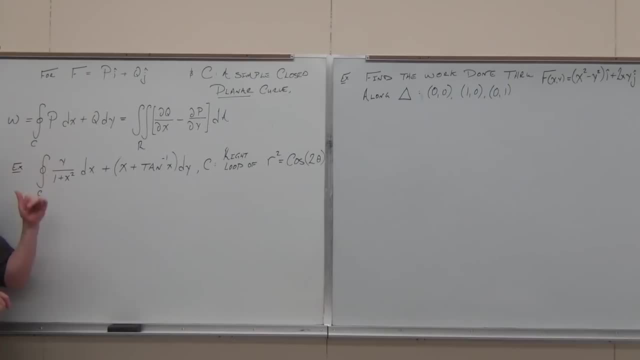 So when we're finding this, we're going to do this line integral over a simple closed curve where C it looks a little weird, so we're going to talk about that, But I want you to first understand that Green's Theorem works: simple closed curve. 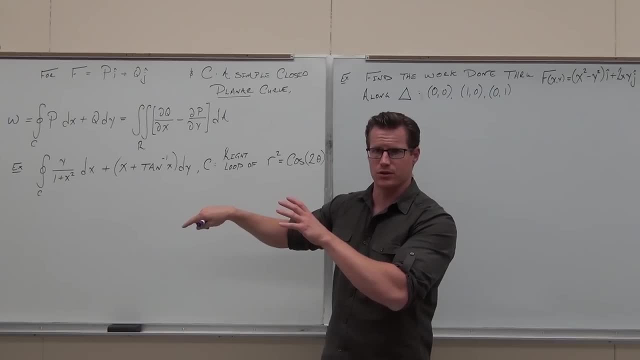 So Green's Theorem is going to work here because we have one loop of a simple closed curve. I don't know if you're okay with that one. Let's try right now to set up Green's Theorem, see how it works. 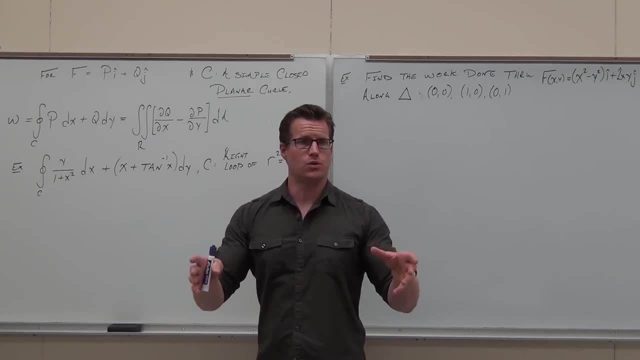 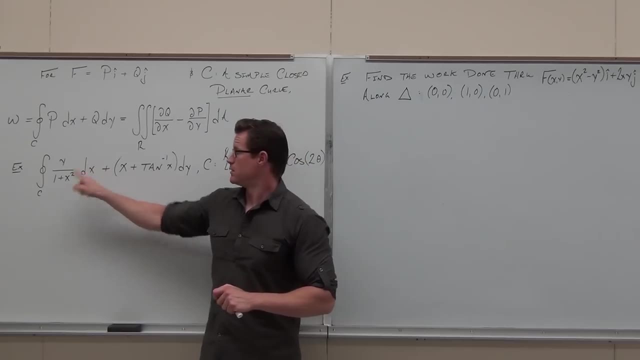 The first thing I told you is you need to be able to identify P and Q Basically. just look for the pieces of your vector field. Which one of these pieces is P? This one, because always join with DX. Please keep this in mind. 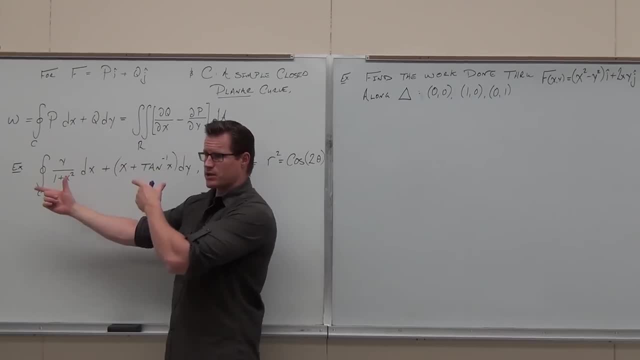 I mentioned this last time, A lot of times. these can be switched around, So I told you to label them, just so you don't start taking partial derivatives of the wrong thing accidentally. So I'm looking for the DX and the piece right in front of that is P. I'm looking for the DY. 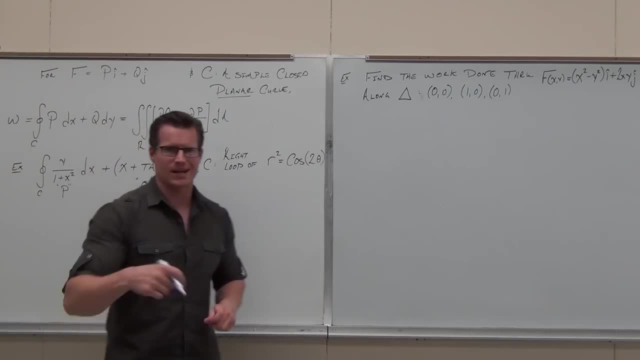 The piece right in front of that is Q. I know you guys know that I'm going to do that. I'm going to do that. You guys are okay with that, because you practiced that a lot last time. I don't know if you are okay with that one. 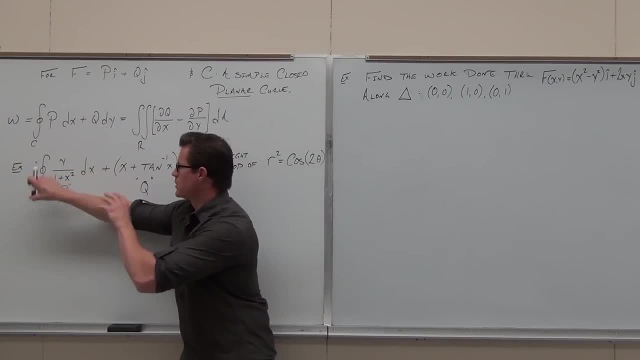 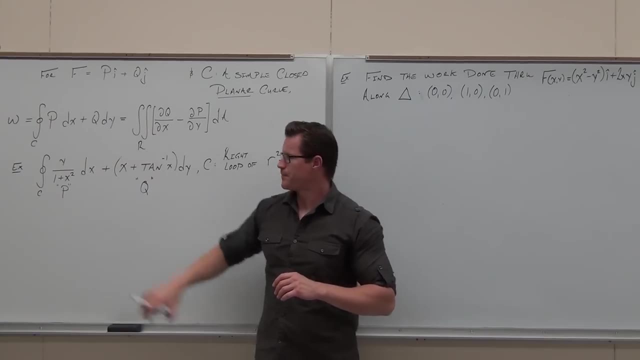 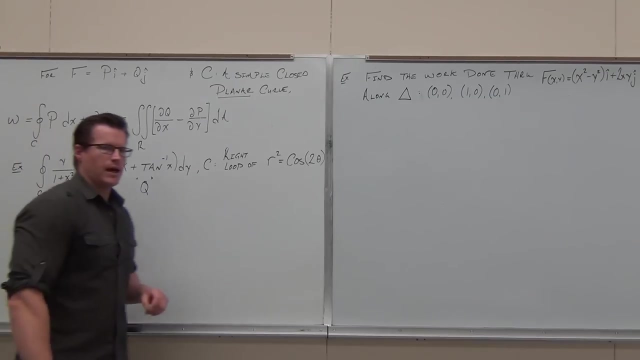 Now, because we have a line integral over a simple closed curve- it's representing work- Green's Theorem is going to apply. Can you please try to set up Green's Theorem for me As you're doing it? what Green's Theorem says is: 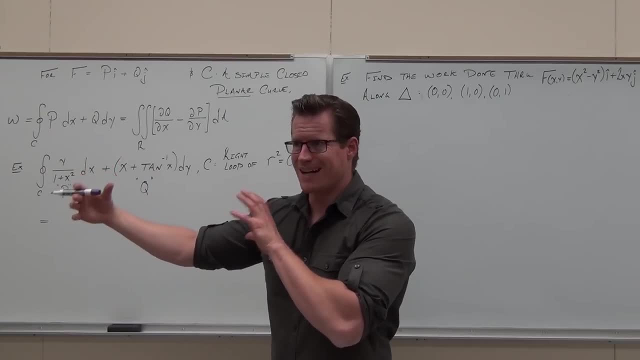 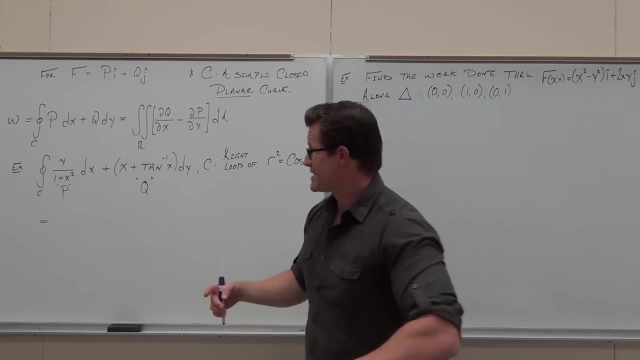 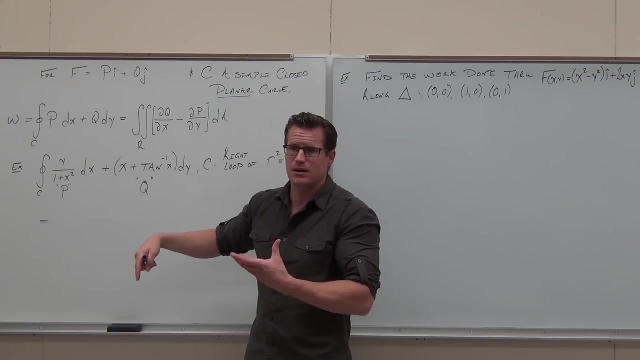 that it's kind of. it's really neat. The work done along that simple closed curve through a non-conservative vector field is equal to basically just the area that that curve contains. That's what it's saying. That's really neat. 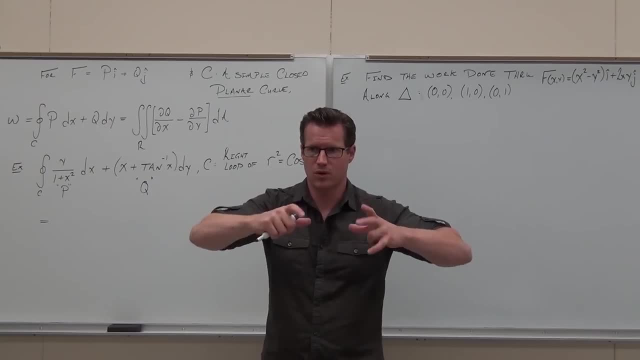 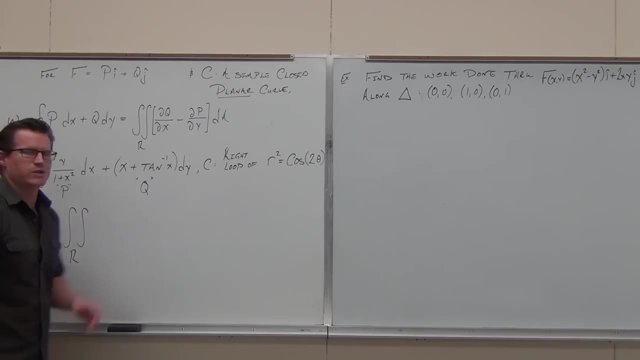 So we have a simple closed curve. It has this region right. It equals an integral over the area of that region. That's interesting. So we're going to do this, We're going to set this up. We always do this first. 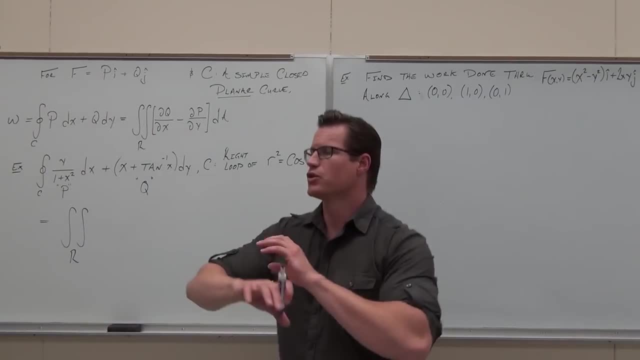 We don't skip that step. Always set the double integral over the region. Draw the region and then finish the double integral, But set the double integral over the region. Set it up this way first, And then we do Green's Theorem. 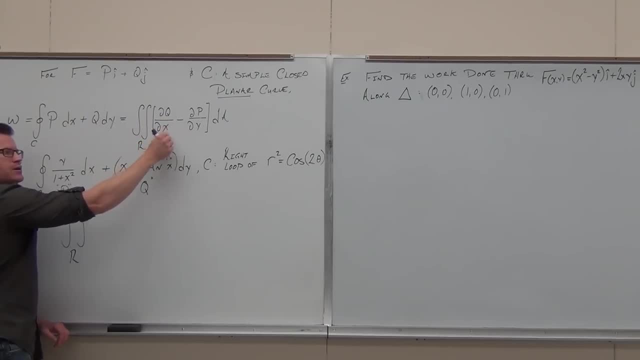 So Green's Theorem says: take the partial derivative of Q with respect to X. So that's why we label it, We go right here and go okay. well, hey, now what's the partial derivative of this thing with respect to X? 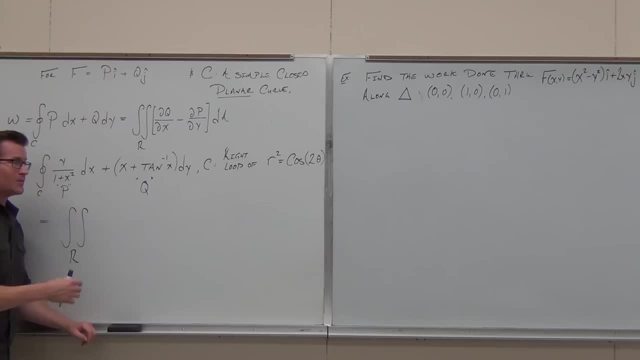 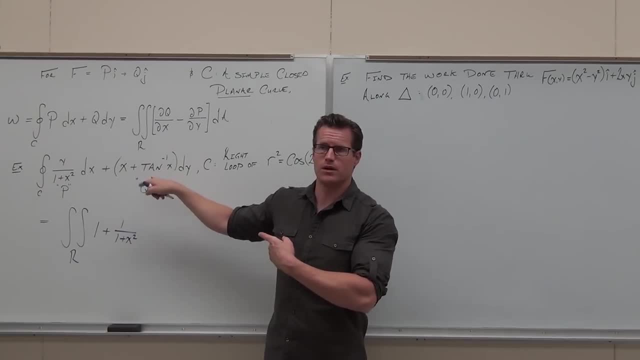 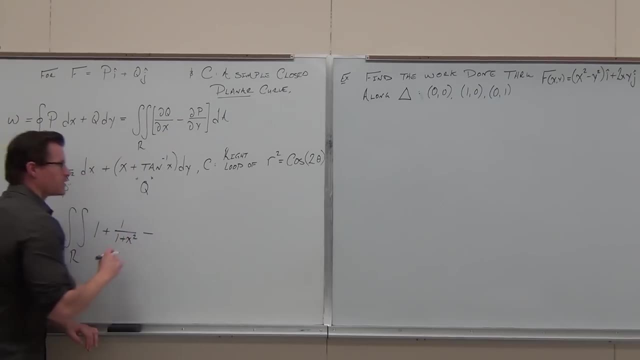 of this thing with respect to X is one. This is one over one plus X squared. That's what those derivatives are with respect to X Had nothing to do with that one And I said, okay, well, subtract the partial derivative of P with respect to Y. Well, this stuff would be like Y. 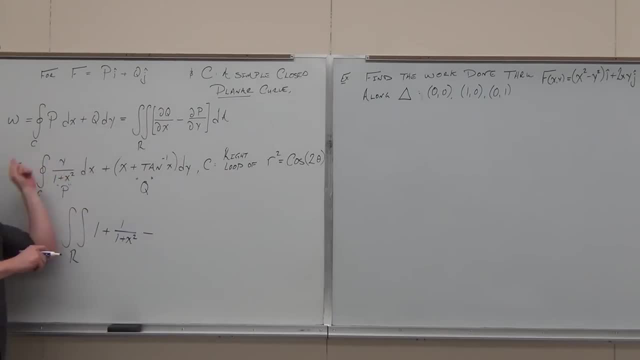 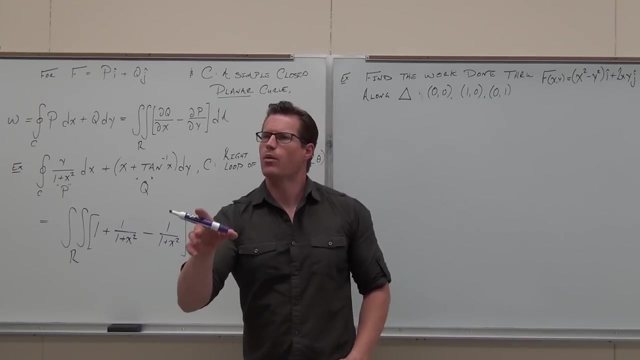 over seven. It's a constant. So what's the partial derivative of this with respect to Y? please, One over one, Before we go any further, Okay, Before we go any further, I want to ask you one question. If I told you, hey, I want you to give me what the vector field is. 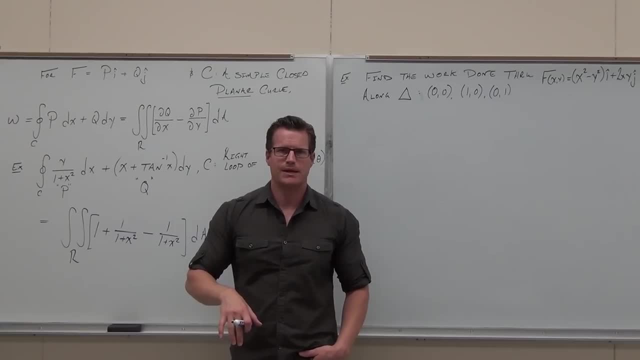 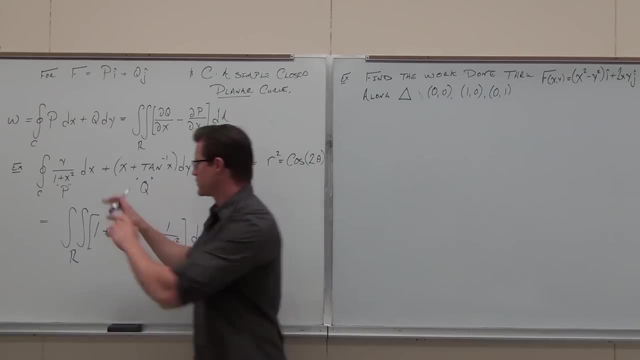 straight from this thing. could you do it? Yeah, It's not a hard question. The vector field is always just PI plus QJ. So if you wanted to find the vector field just off to the side here, the vector field that's giving us 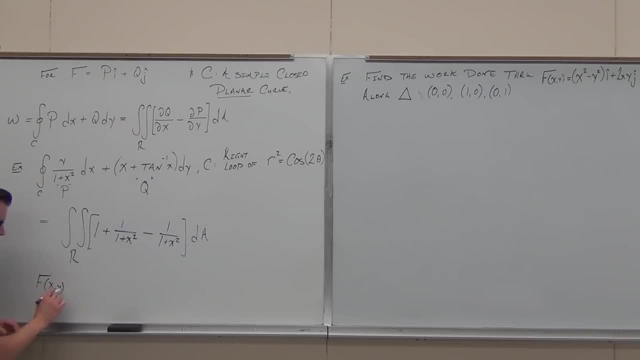 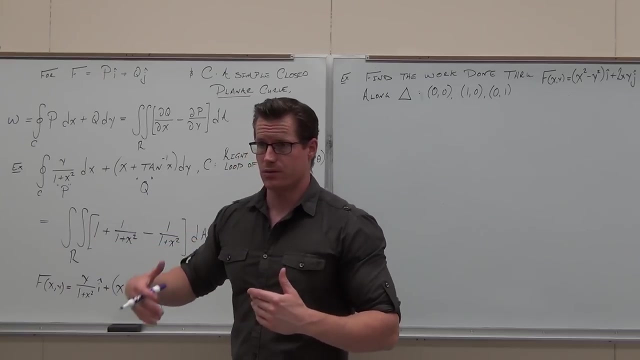 this line. integral would be P, I plus QJ. And I'm trying to get you to see that because I don't want you to forget, I don't want you to lose what this means, What we're doing here, when we're doing this stuff. 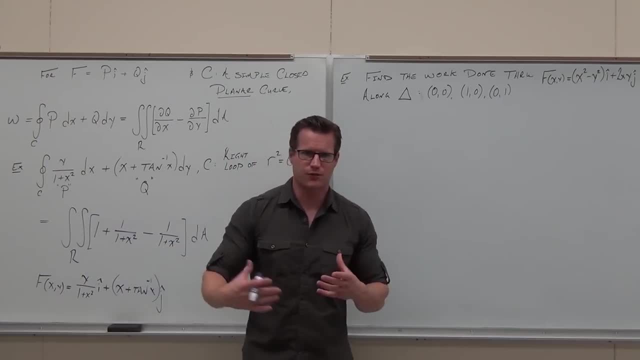 is we're finding the work done through a vector field. If you don't know what the vector field is, it really doesn't matter. Well, it does matter to me. You can do the problem, but I want you to put it all together. 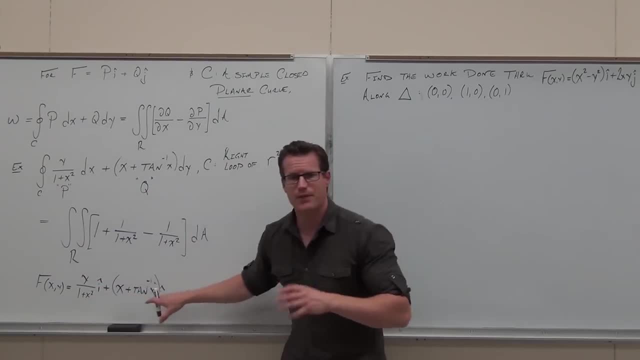 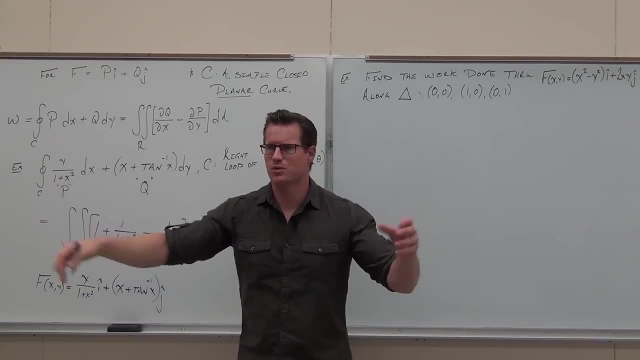 So we're doing work through a particular vector field. Which one? This one, That's the vector field We're doing work through along that particular curve. So if hands could go right with that one. So when we get done with this, we have found work. 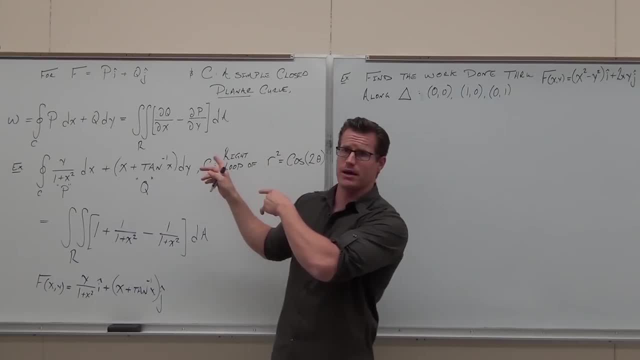 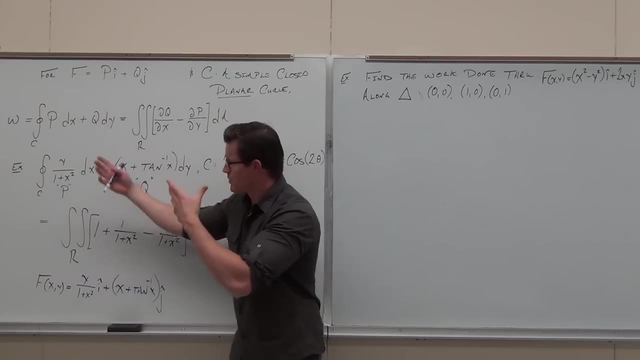 through that vector field along. whatever the heck that thing looks like- And we'll talk about that in a minute- The first step is see if your line and integral fits Green's theorem. It's a simple closed curve. It does Set up Green's theorem. 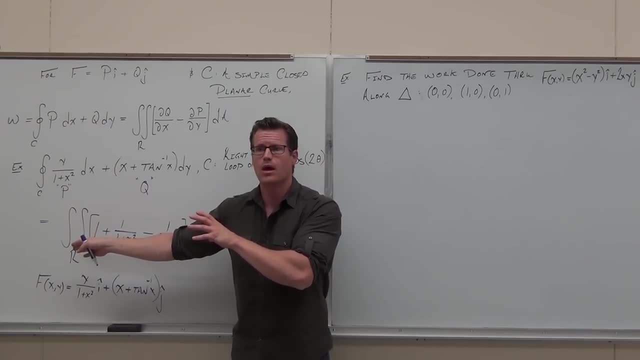 That doesn't mean you jump right to the region, because that can be kind of difficult. What that means: you take your partial derivatives, you write your region, you let it hang out for a second. and you write your DA, you let that hang out for a second. 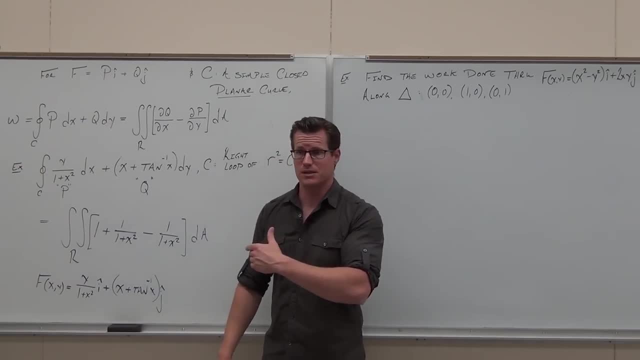 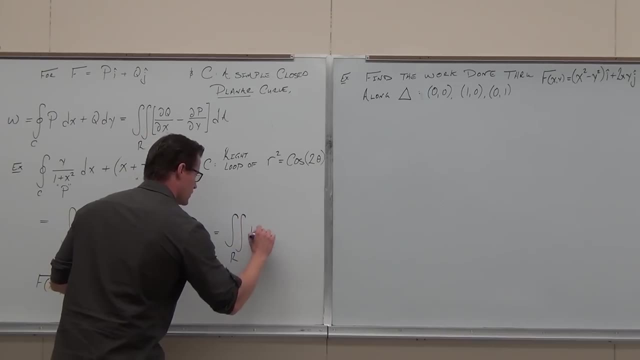 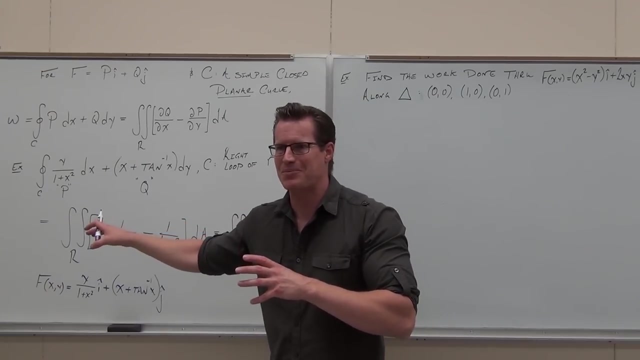 and you simplify as much as you can, Not? I know that when you wrote that down, you saw some things that simplify, right. So we also talked to one more thing. This is a good problem, right? It's a really good recap problem. 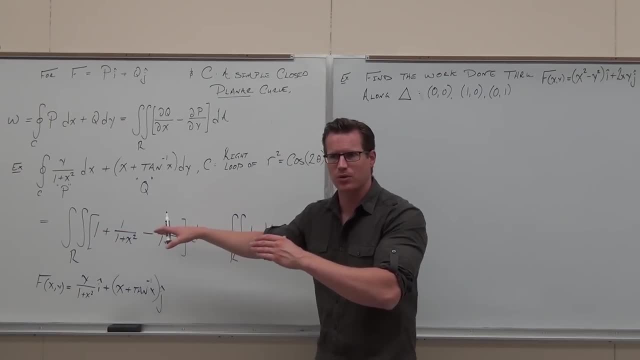 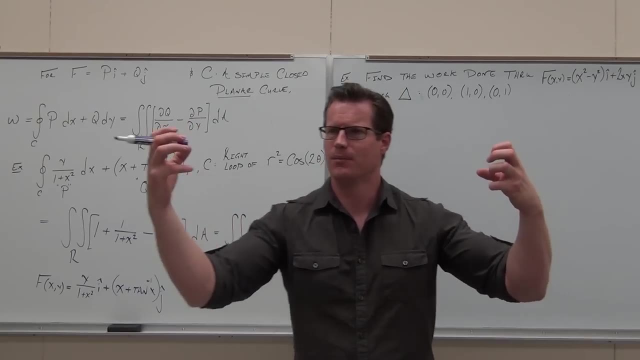 Because then it says, oh my goodness, we work this down, Then we have a double integral over some region bound by that curve of 1 DA. What's that? Come on, Everybody in class right now. Area, That's area. 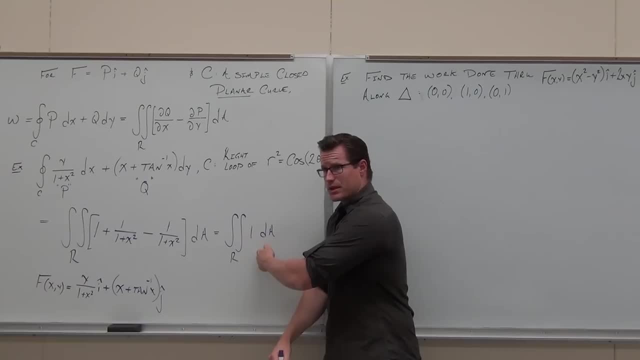 So what this is going to give us? This is going to give us literally the area of whatever that curve is. Does that make sense? Now, wait a second Before we did this. if you remember the last two examples, last time we had some nice circles. 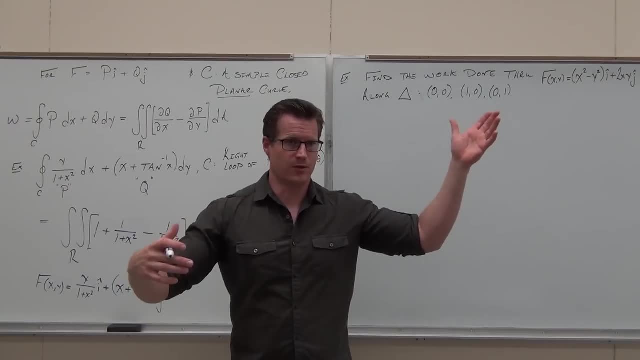 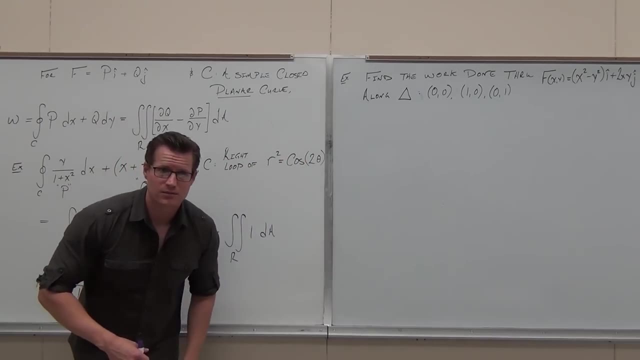 And we had some formulas for areas of a circle And we invented the formula for ellipse, And so we had a formula for that. Do you know what the formula is for this? I don't even know what that looks like. I think we could have done the problem. 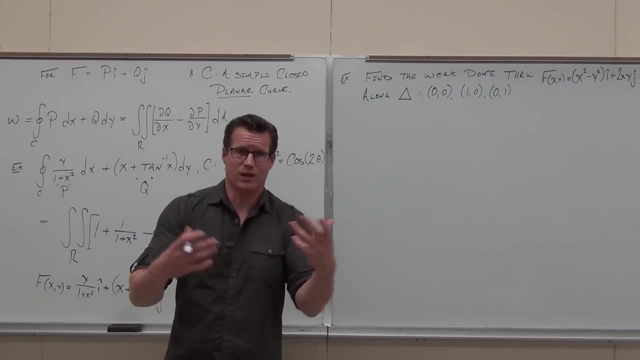 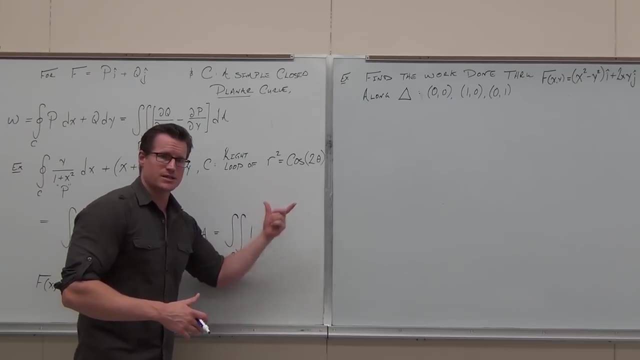 But let's say I didn't know what it looked like, I didn't have a formula for it. That's when we go: okay, well, Green's Theorem gave us this formula for area. let's see what this region is. 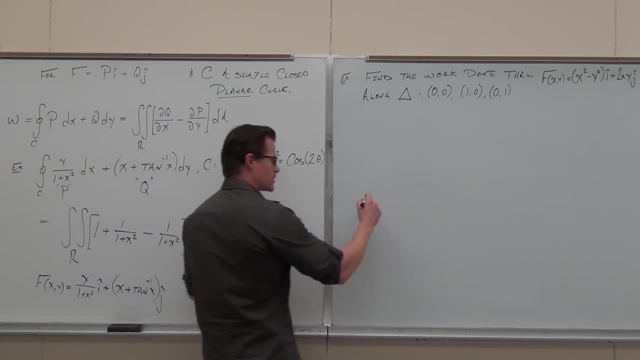 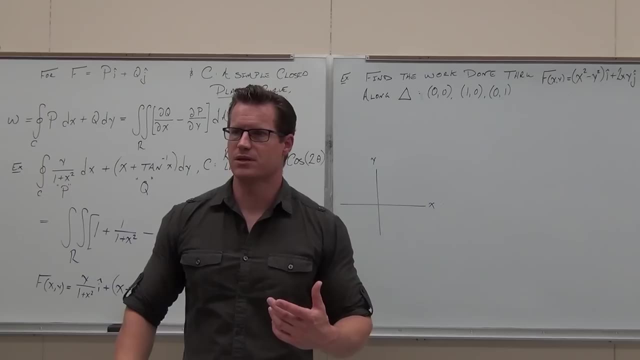 And that might take a little bit of work for you. So this region, what that looks like- and I'm not going to go through the whole process because we actually do this problem- It's called a Lemniscate Happens in Calc 2.. 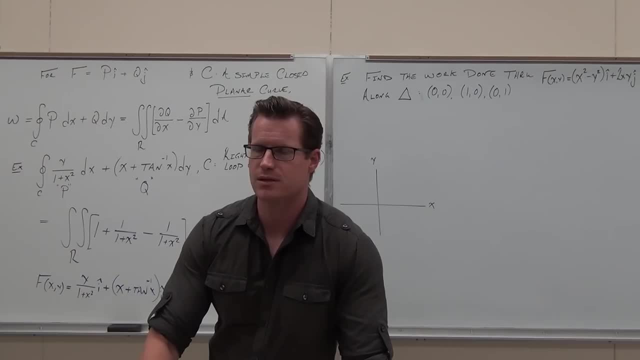 When you first learn about graphing polar functions, you might have seen this: R squared equals cosine 2 theta. What it looks like is just figure 8.. It just looks like this figure 8.. You had one of those. You had one of those problems in some of your homework, by the way. 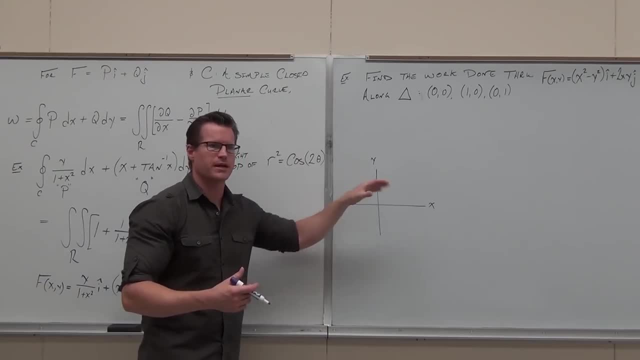 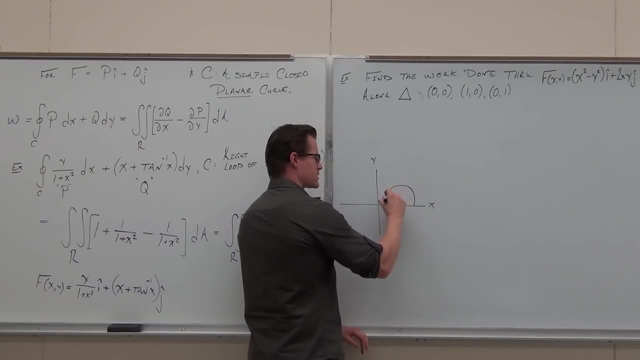 And how could you do it? Well, you could take the square root, just plug in thetas and see what it gives you. But what happens here is we have this loop that starts here, does this and comes back, and it's traveled in this direction. 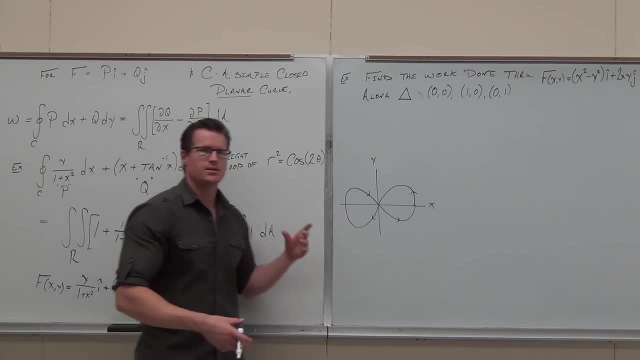 That's what that. that's what the whole thing looks like. Now. what I want is the right loop. Explain to me right now why I want the right loop and not the whole thing. Keep in mind, we're working with the greetings theorem. 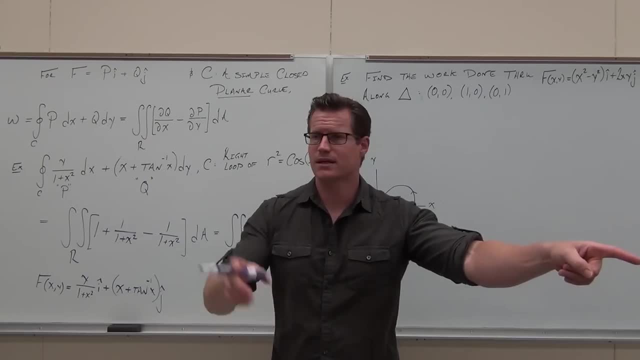 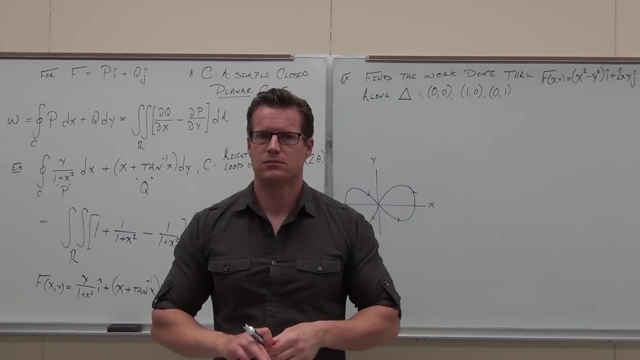 Why do I want just one loop of this? Why doesn't someone else? Why doesn't it work with the whole thing? Because you don't know how much seconds are working for it. You would Why? Because it's two ring curves. 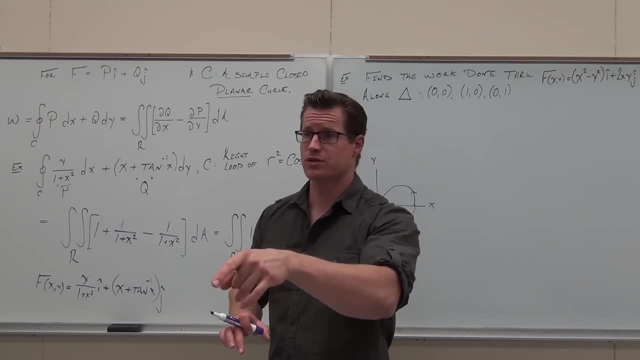 Nothing, because- okay, that's it. Because it's not a simple closed curve. This would be a closed curve, but it's not simple because it crosses itself. Does that make sense? It's on a plane, So it literally crosses itself. 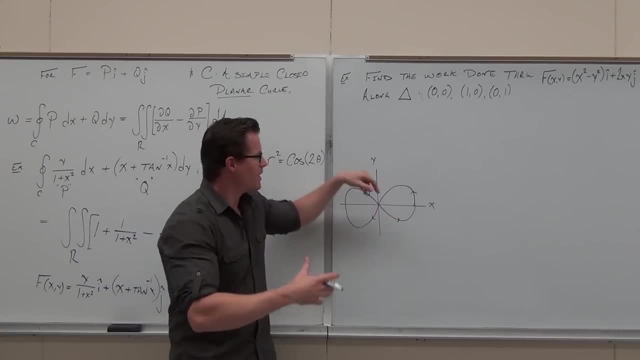 So on a plane, that's fantastic. Greene's theorem works with planar curves. I can't do this guy, so I'm just going to eliminate that and work on just the right loop. So what we're finding here, what this does, what this does, this finds: 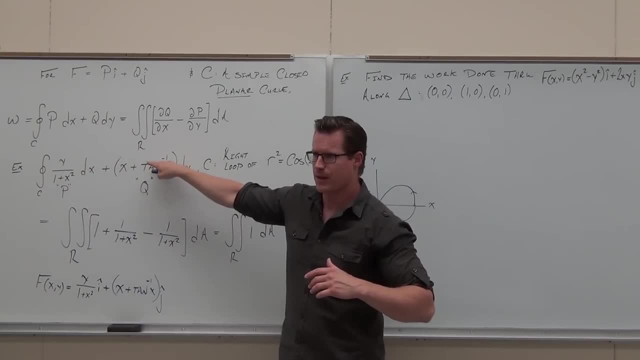 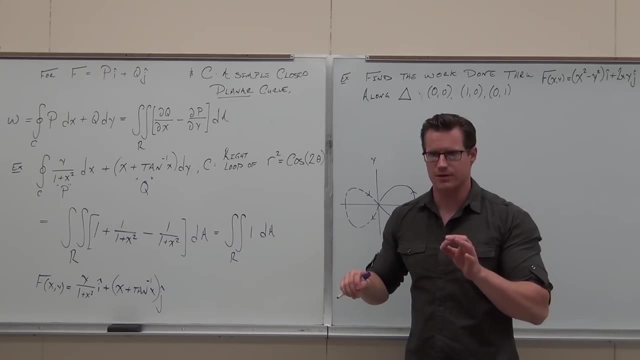 so just keep our heads wrapped around this. This finds the work done by moving a particle. one loop around this That this is what this is going to do. It's going to find the work done there. Does that make sense? It's also going to find through that vector field. it's also going to find the area. 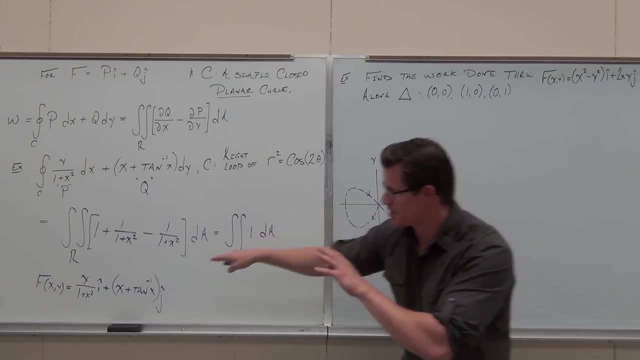 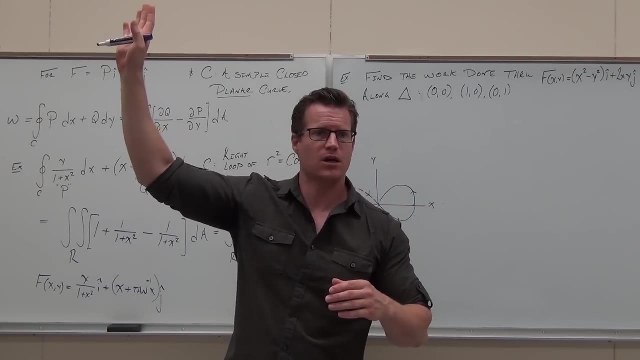 of that loop. Numerically, the work done along this loop through that particular vector field is going to be exactly equal to the area that that loop contains. Show of hands, if you're interested in the concept there. I don't want to over talk it, but I want to make sure that you're here. 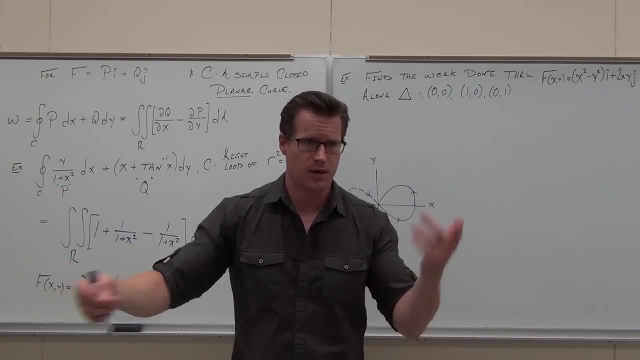 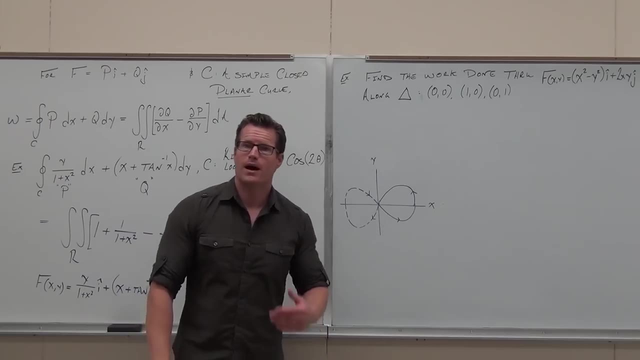 We've had a weekend between, so I want to make sure that you guys are with me. Are you guys with me on this stuff? Okay, cool. So how in the world are we going to do it? Well, I don't have a formula for the right area of the right loop of the Lemniscates. 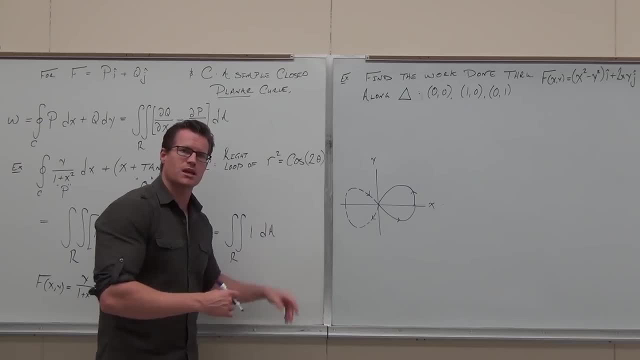 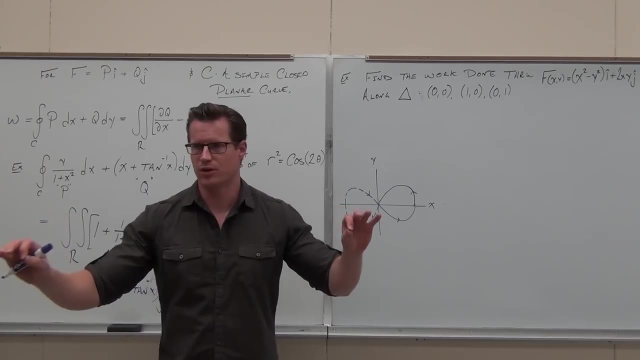 but I do know how to set up a double interval. So let's think about this, Since this is defined in r's and thetas and not x and y, and for heaven's sakes I don't want to do x's and y's here- 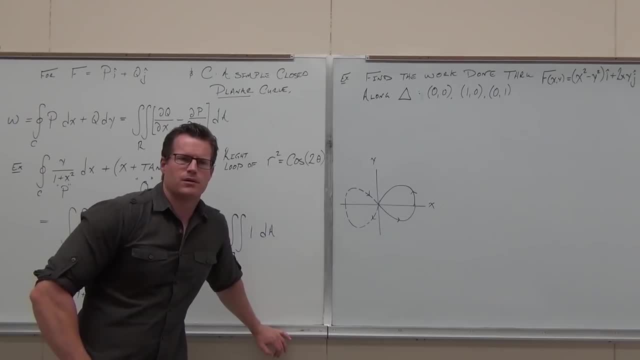 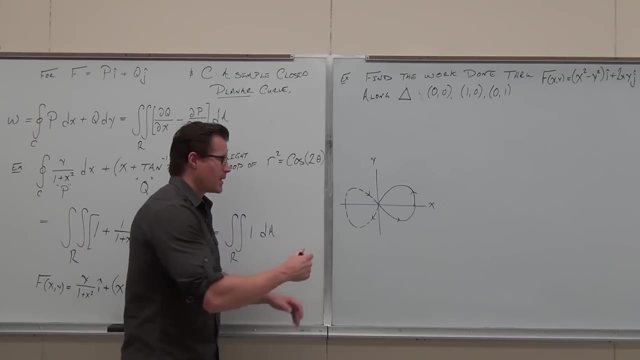 What type of double integral would you want to do? What do you think? One in xy coordinates or one in polar coordinates? One in polar coordinates? So let's start defining the region, Our region. if I look at this, if this is the area, I'm going to erase this. 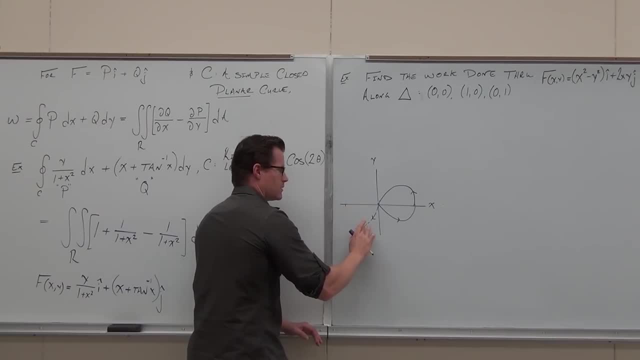 so we don't even think about it because you don't need it. Let's think back to our double integral, Our double integral base. If I start at the origin, am I immediately hitting the area of my region, right from the origin? This is the region. yes, 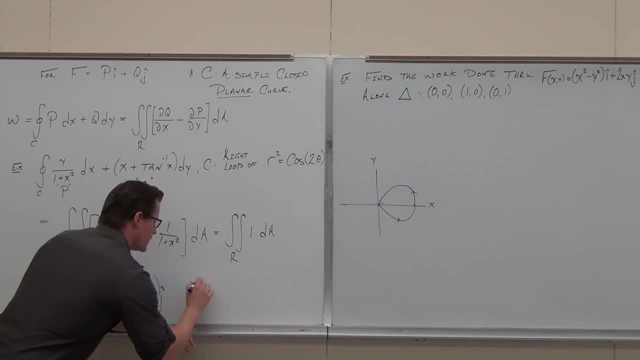 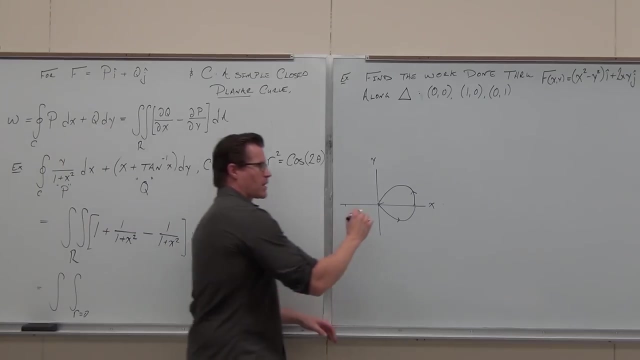 Yes, So my double integral goes from: come on, you know it, it starts from where Zero And then, no matter where I go, I'm going to be hitting this curve. Well, we've got to define that curve because we want r equal. 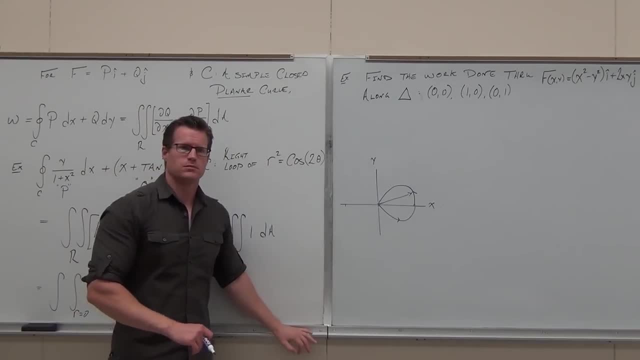 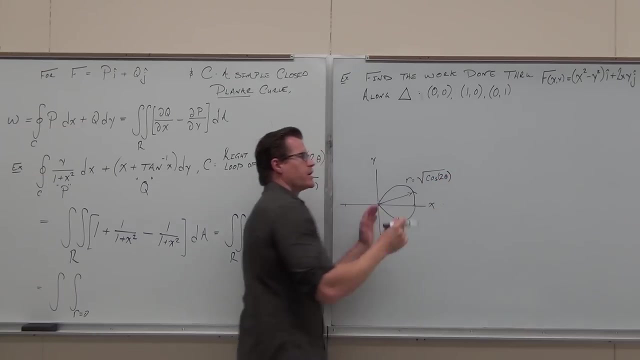 So we look back at our function. can you solve that for r? Sure, pretty easy. r equals what Square root of x? So as far as our region is concerned, when I set up my double integral and I don't have a formula for a nice shape like a circle or an ellipse- 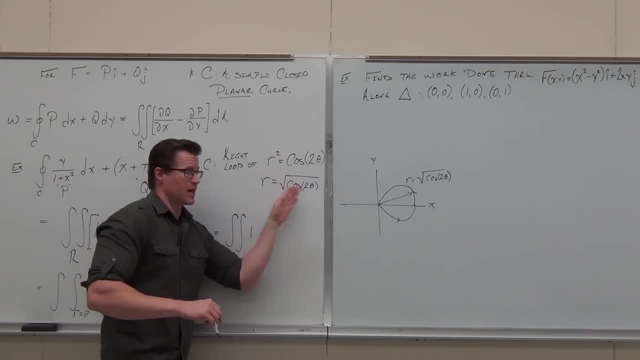 or something like that. then I have to go back to the actual polar function. I have to look at that, I have to graph it and I have to set up my region. My region starts from zero along the r to where it hits square root of cosine 2 theta. 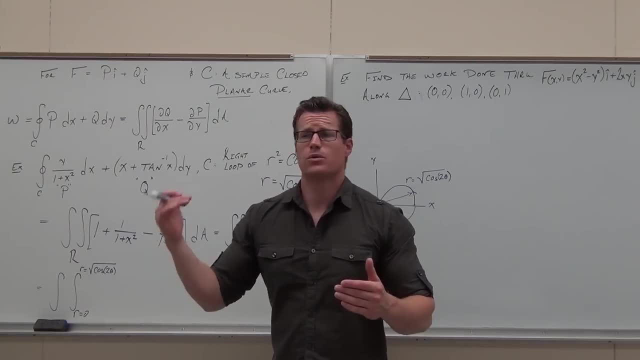 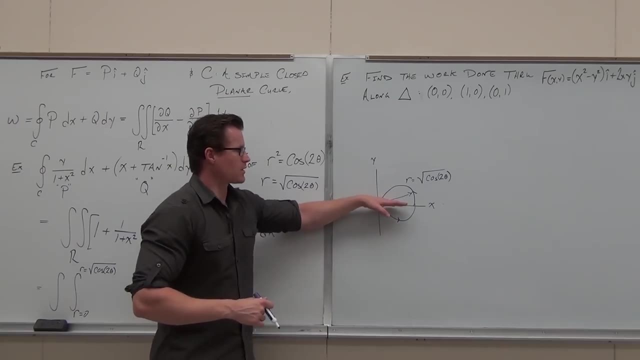 First question: are you guys okay with that one? Yes, So our r is just going through our region, That's it going from zero to the function itself, Now the theta. that can be hard. You see the problem with this curve: it starts at zero, it goes this way: 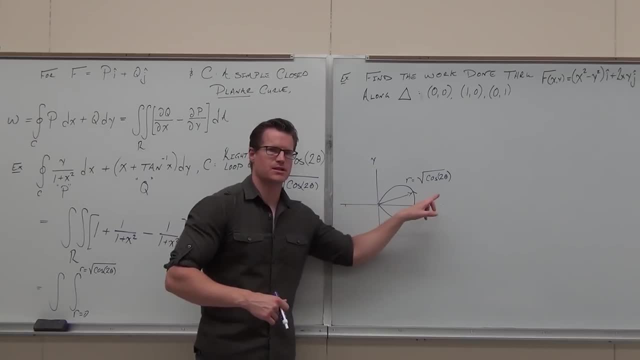 then it comes back down and does this before it hits this section. So if I want to go from here to here, I can't start calling it things like: well, when you graph this, you get zero, you get pi over 4. that gives me this. 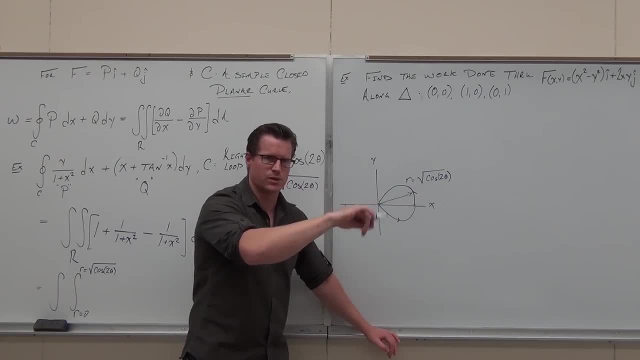 you get pi over 3.. You get pi over 2 and you get pi. Pi gives you one full rotation of this. But I can't do things like go from a larger value of pi to a smaller value of pi. Notice that the larger value of pi would be giving us this stuff when I plug in like 3, pi over 2. 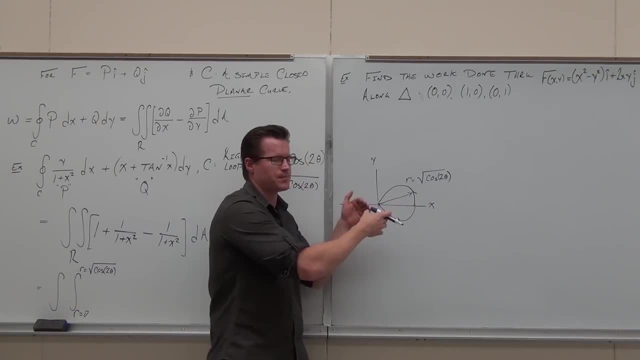 to pi itself. that sorry, 3 pi over 4 to pi. that's where I'd be getting this section of it. So instead of thinking about like pi over 4 to 3, pi over 4, I'd be thinking of maybe negative. 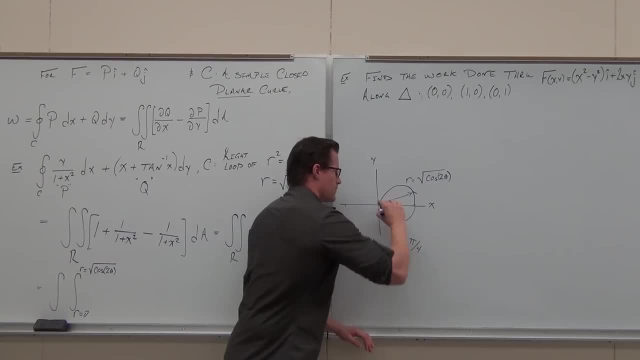 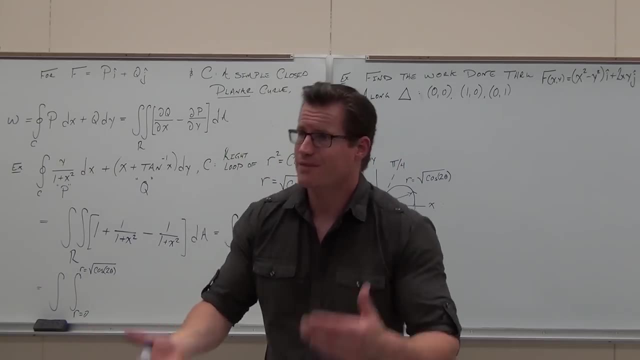 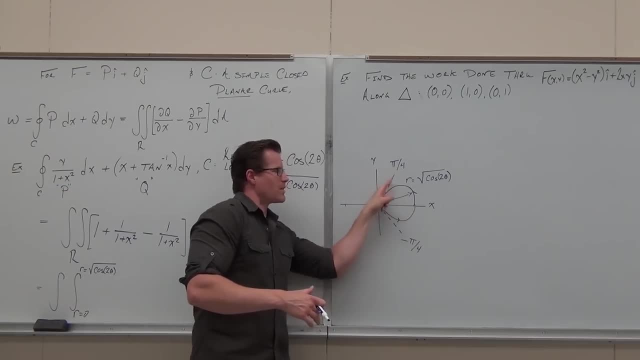 I got to say where this stuff starts and stops. But if I don't, if I don't want to go around the whole thing, I can't just go from like zero to pi or zero to 2 pi if you have one of those functions that creates a full circuit in 2 pi. 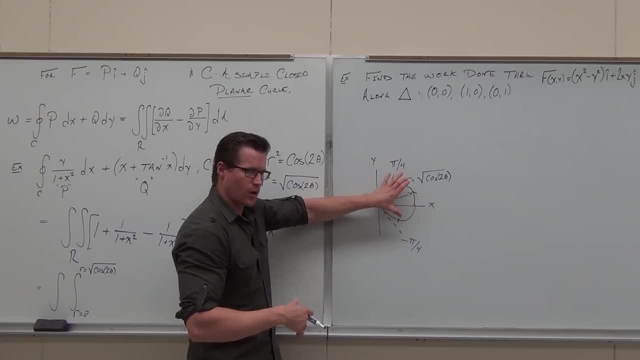 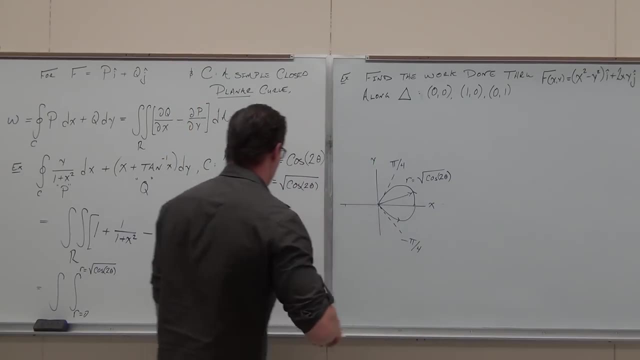 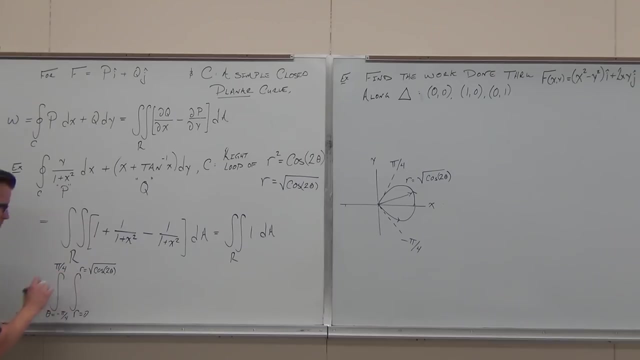 I'd have to think about what's going to create for me this segment And what creates for me this segment is this negative pi over 4 to pi over 4.. So that's an important idea. So when I finish this set up, we get beta equals negative pi over 4 to pi over 4.. 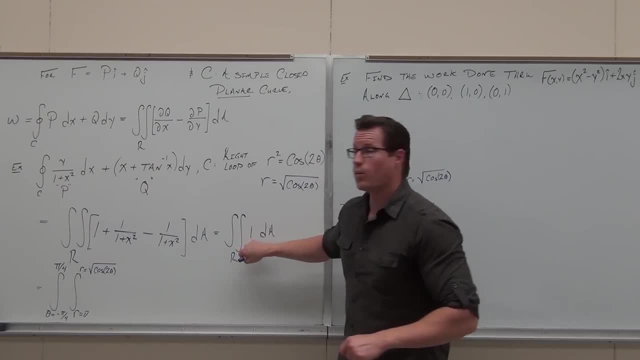 Now there's only one more thing. It's going to be a really easy thing. Do we need to change the 1?? Do we need to change the DA? Yes, Think back to polar. what's it become? A negative pi over 4 to pi over 4.. 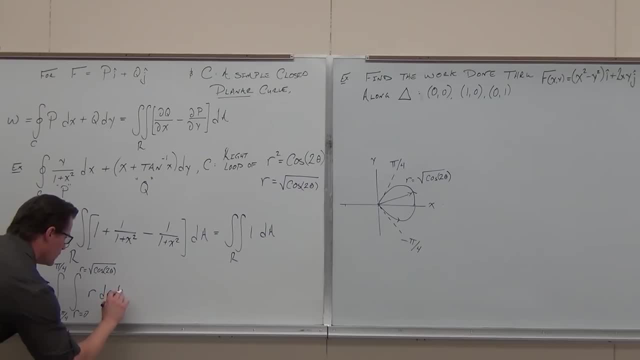 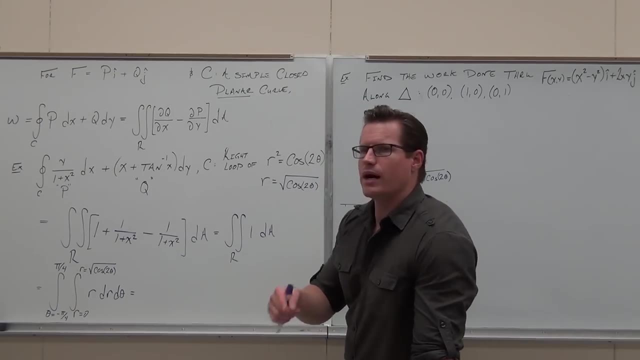 Beautiful. Would you know how to solve it from there? Yes, What would you integrate first, So you get this 1 half r Square root And then you plug in a square root. Pretty darn convenient, Yeah. Then you do a very simple integral on cosine 2 theta. 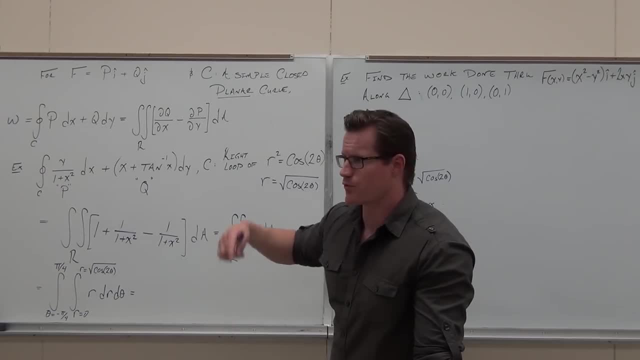 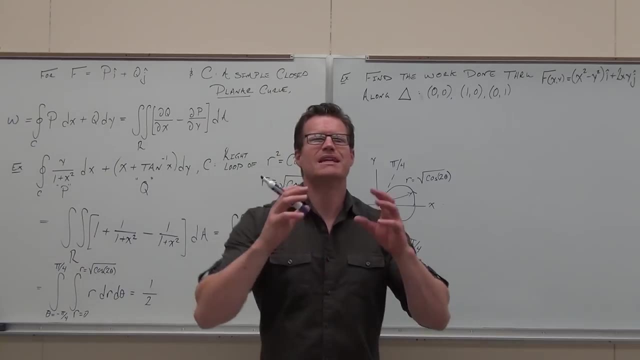 You get this like 1 half sine 2 theta. Plug it in negative pi over 4 to pi over 4.. And you shouldn't get any negative pi over 4.. It's just a point. get one half out of that now before we go any further. you tell me what that. 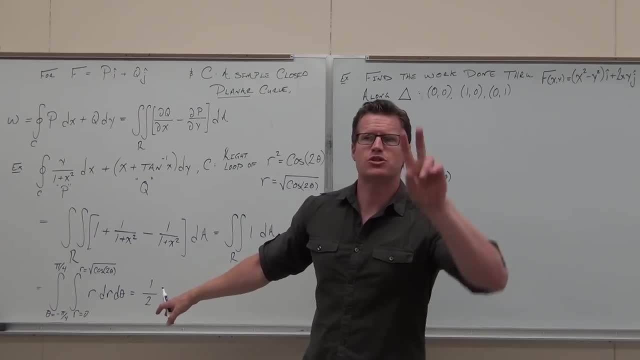 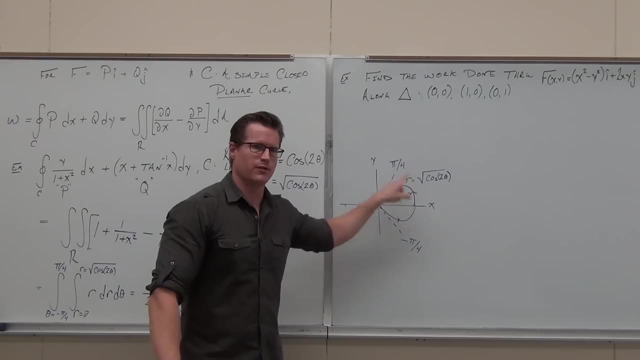 means. what's that mean? tell me two things that it means the first thing. what's it mean? that means area. we just found the area of this shape, the right loop of the lemma skate. that's, we just found that and not, if you're good that one, tell me the second thing. it's consider. 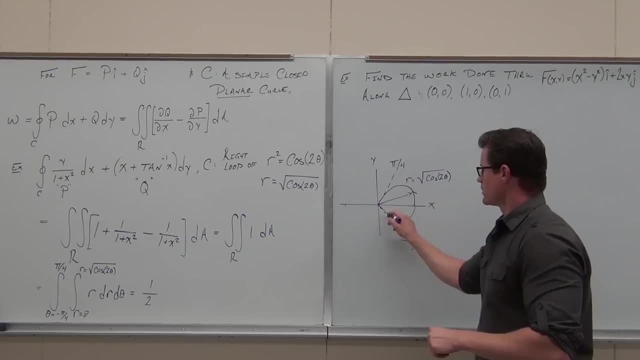 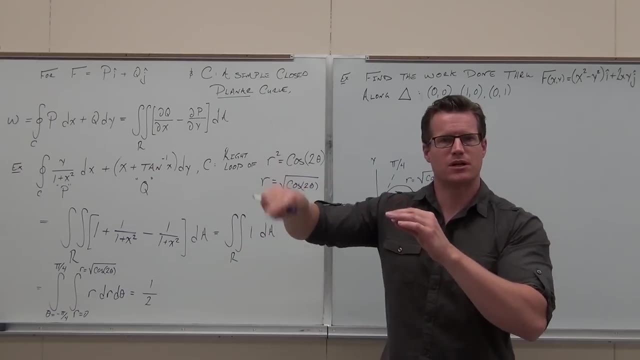 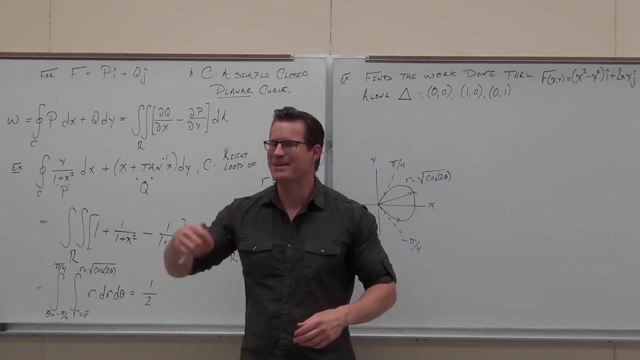 greenster, that's work done around this loop in the counterclockwise direction, but not just the work done around the loop. that doesn't make sense. the work done around the loop in this vector field. does that make sense? you're getting, you're getting. it should be making sense at this point to you kind. 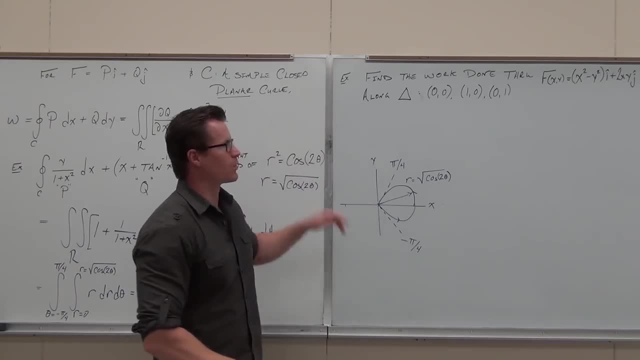 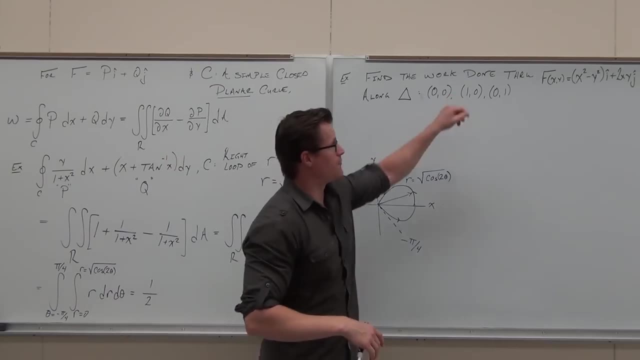 of cool, right? so if we're finding work, then we're gonna put this like in her: put yourself in a test situation. I say: look, I want you to find the work done through that vector field along this thing. let's think through what you could do with this. so, firstly, if we're finding work, 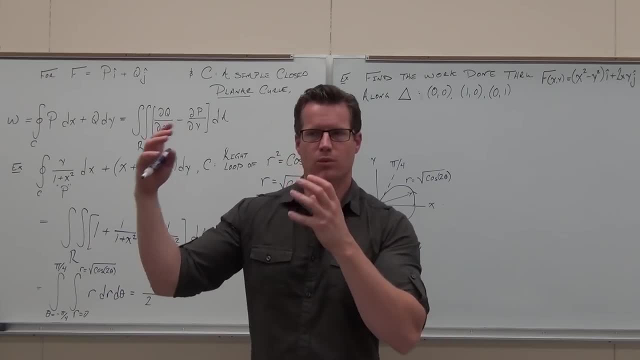 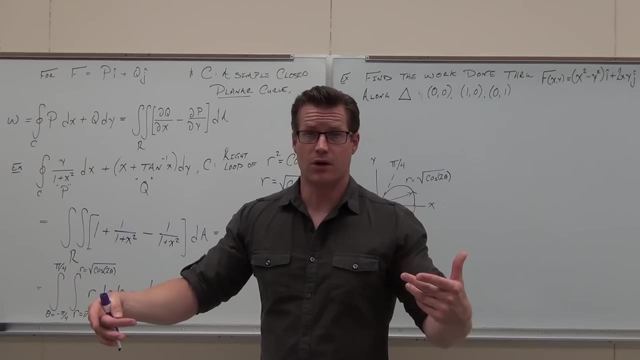 done around the loop. that doesn't make sense. then we're gonna put this like in here: so if we're finding work done along a curve, we got what? what type of a problem, what type of a situation do we have? find work done through a vector field, along a line? it's called a vine. what gives us work through a vector? 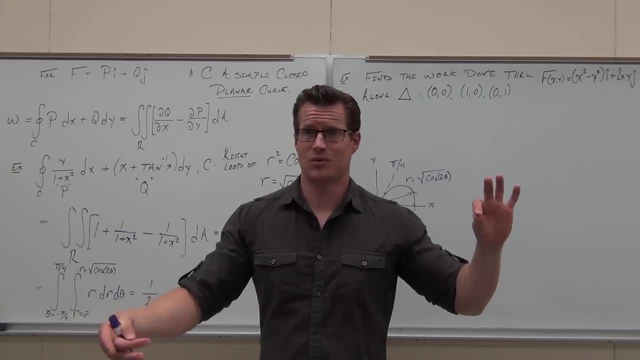 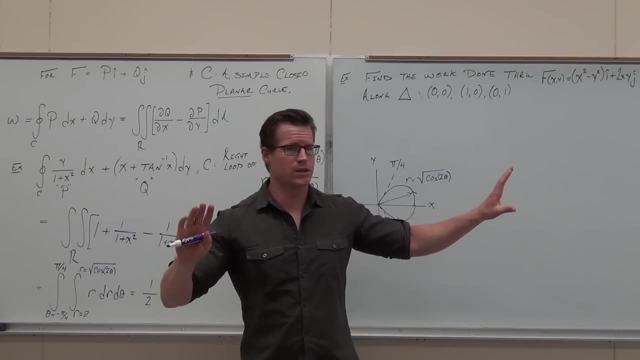 field along a line, a line integral. we got a line integral. we're just set up a line integral. we've talked about several ways to do that. we've talked about just basic line integrals when you don't have conservative vector fields. we just added up all the segments. you remember talking about that. then we talked about line. 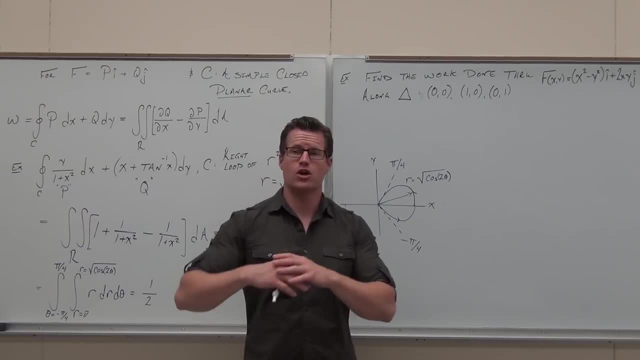 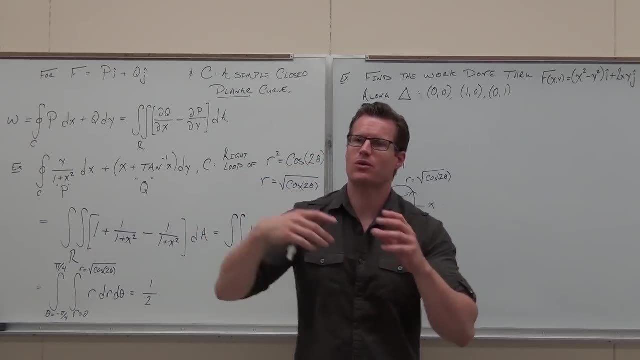 integrals on conservative vector fields. now we're talking about line integrals on non conservative vector fields, but where we have a simple closed curve on a plane. that's where we're at right now, so let's start thinking that way. we got a vector field, we're looking for work done and we have a series of segments that 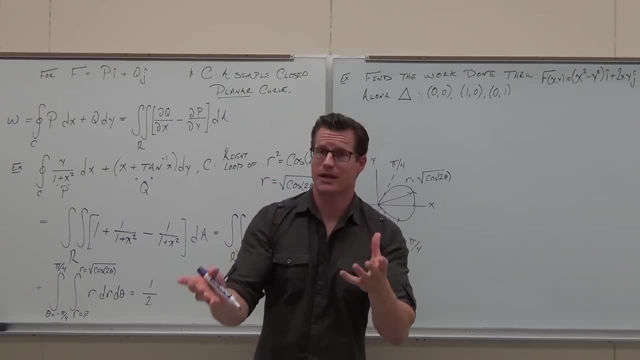 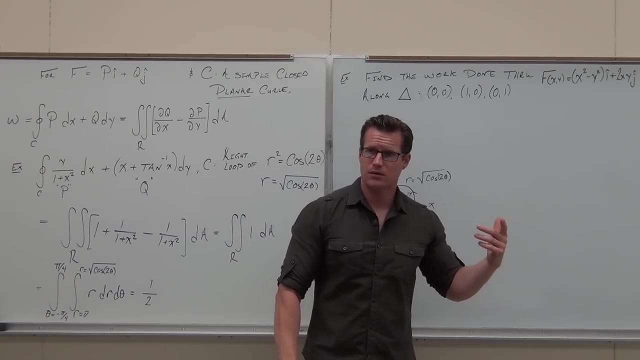 come together in the form of triangle. does that make sense? we have a line integral. there's three ways to do it. number one thought you might have is: well, check for conservative. you can do that. is it conservative? no, but you can check it very easily. partial derivative of. 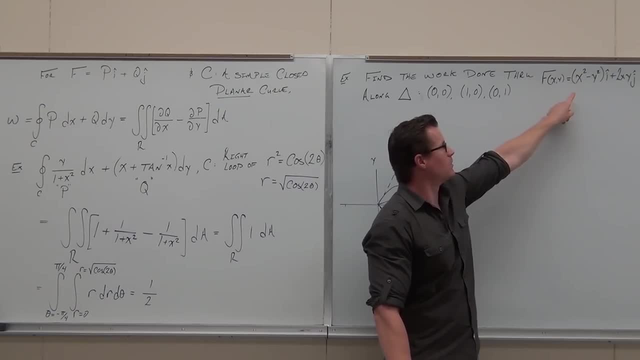 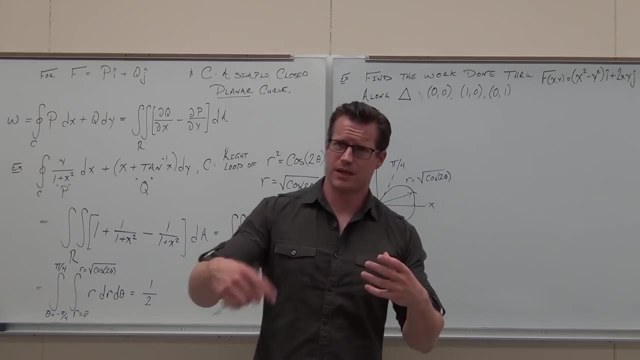 this with respect to X, partial derivative of this with respect to Y. they're not equal. does that make sense to you? you go okay. well, if they're not, this or our integrals, line integrals and conservative vector fields- that fails. we can't do that stuff we could do now listen. well, we're not gonna do it this. 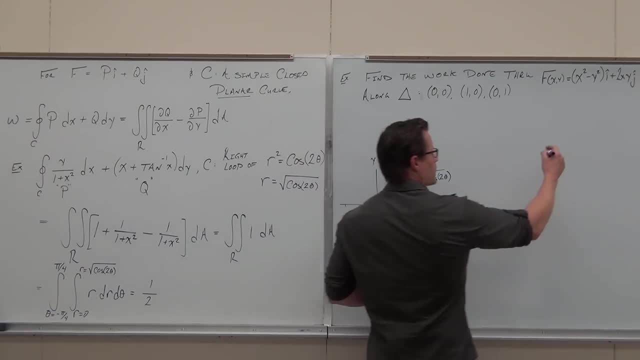 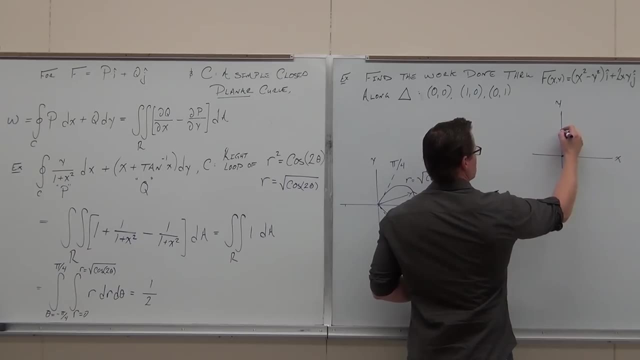 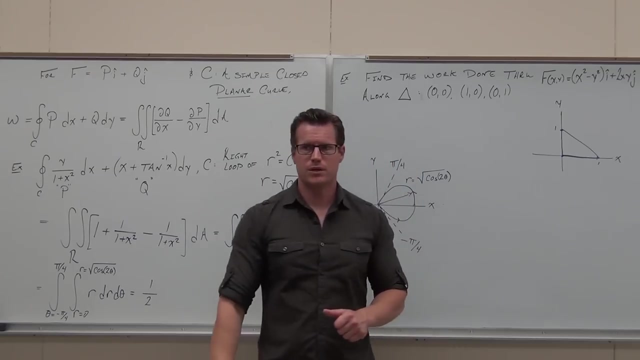 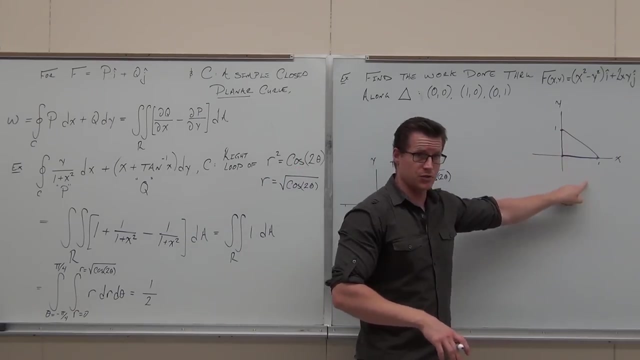 way. but we could do this, we could graph this region and we could do this. we could separate these three segments into one and two and three and we can parameterize them in terms of a vector function and we can literally do a very simple line integral for this and this and this using that vector field and add up. 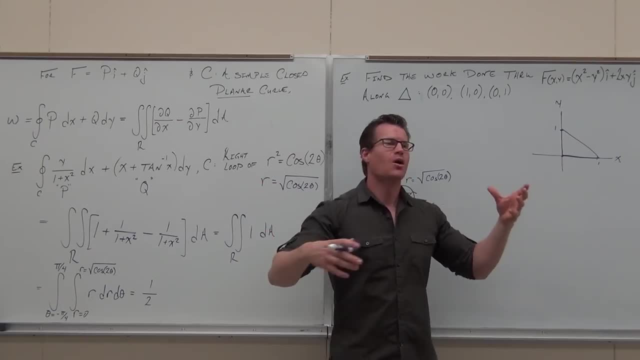 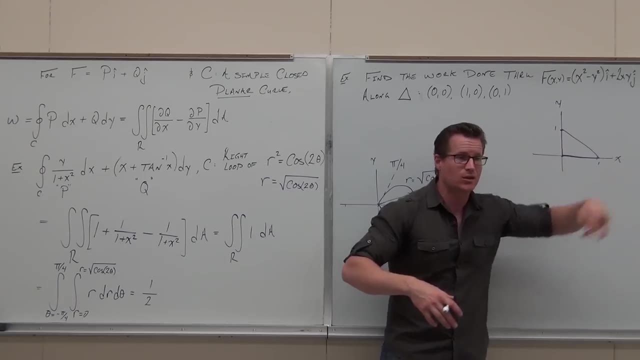 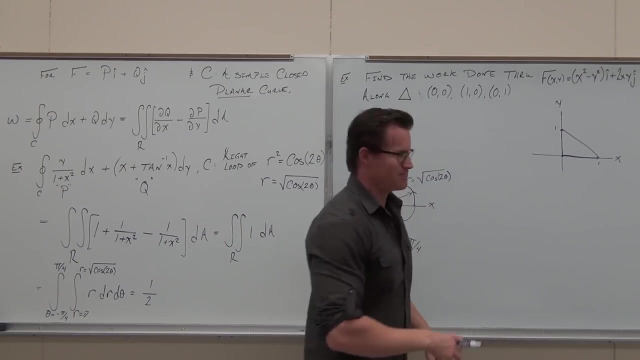 the results. remember that we've actually done it with segments, but we only had two segments at a time. why? because as soon as you have three segments that close a loop, what could you do, instead of adding up three different line integrals, what could you do? let's try this again. you for a lot of you, just. 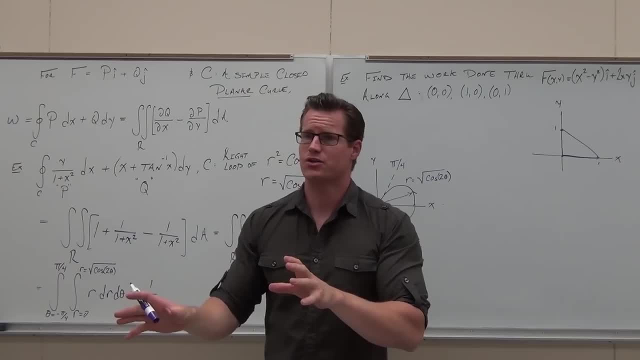 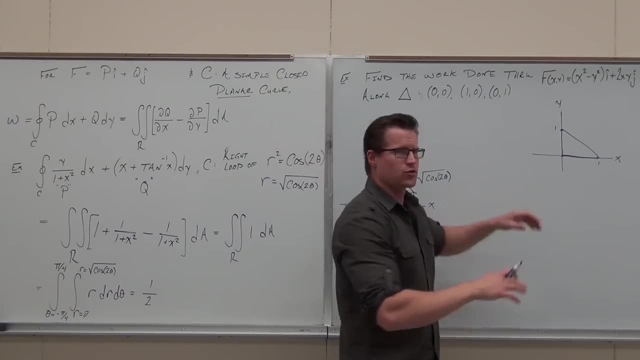 want right over your head. listen, the first thing you might try for any work done through a vector field along a curve, that's a line integral. folks, that's what that means. so, okay, line integral, absolutely. how many different ways we have to do line integrals three? 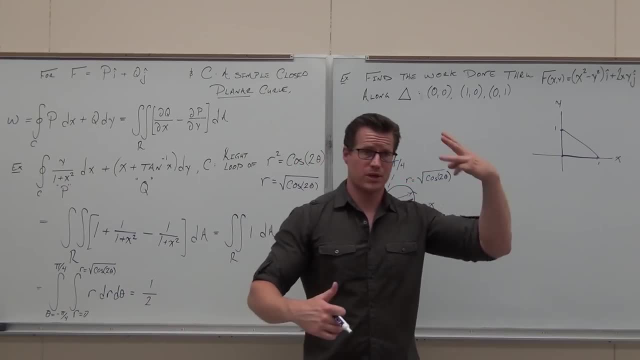 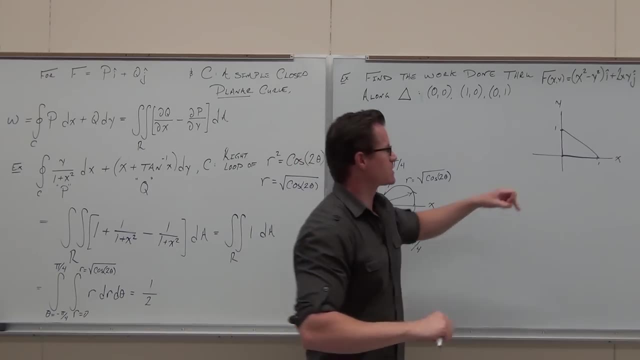 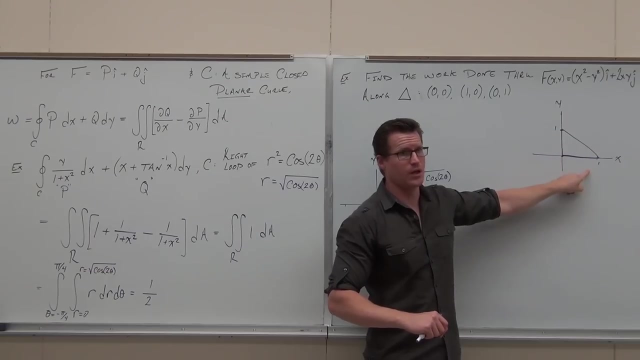 we're gonna have four by the end of this next section. so three different ways. one of those ways is just universal, through non-conservative vector fields. you just take each segment, go- hey, that's one line, integral of this one segment through that vector field. you parameterize it, you do it- hey, that's another segment. 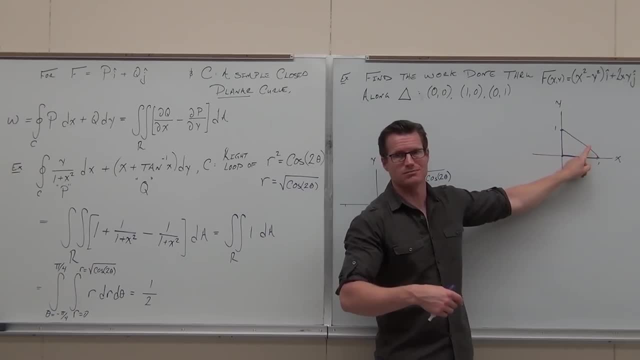 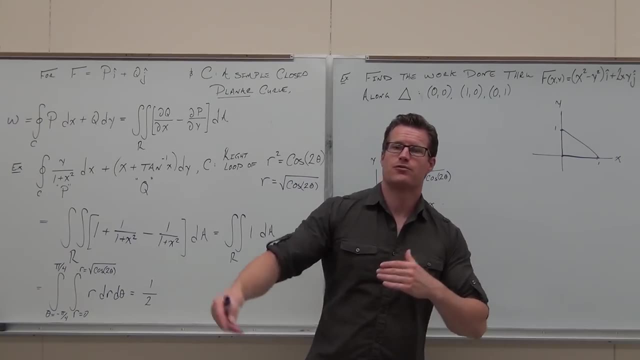 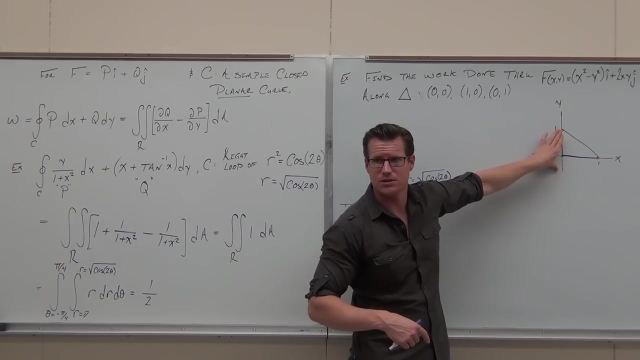 through that vector field, parameterize it, do it. hey, there's another one. through that vector, parameterize and do it, and then add up the result. that's one way you literally could do this. in fact, from before, if I don't have one of these legs, that's what you would have to do. does that make sense to you? you'd have to do. 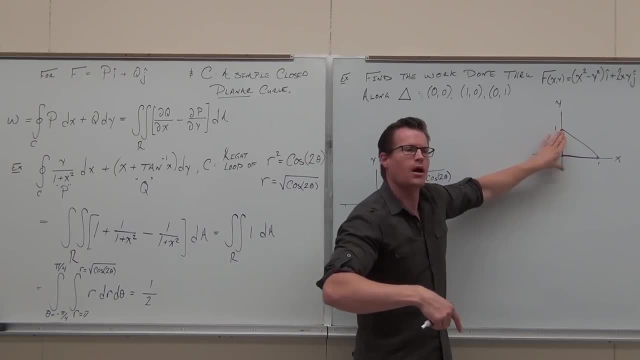 that because it's non-conservative vector field it doesn't make a loop, then we go okay, if it's non-conservative I can't use the conservative stuff, but if it's non-conservative and it creates a loop, then I don't have to add up all three line integrals. I now have what line integrals through? 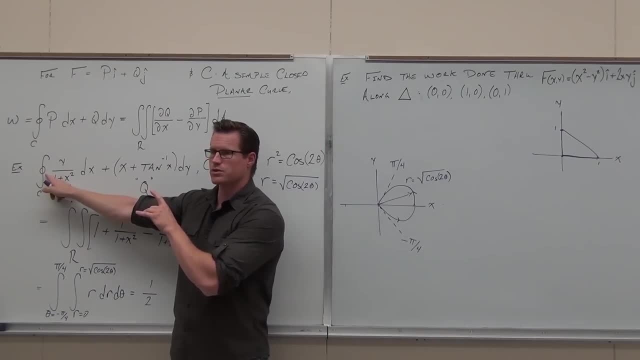 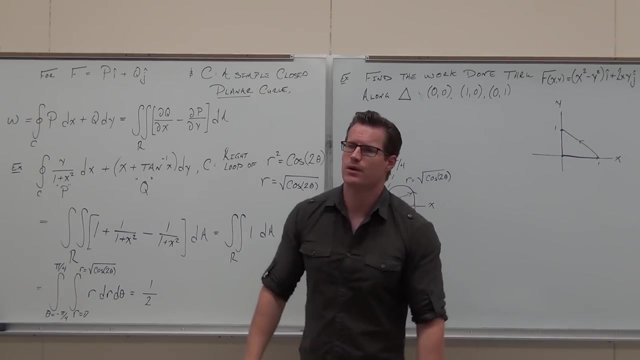 non-conservative vector fields that create a simple closed curve. you go triangles, not a curved man. yes it is, it's just a silly looking curve, it is closed, it's simple, doesn't cross itself. that's a simple closed curve. and if we traverse that in a positive, counterclockwise direction, what green? 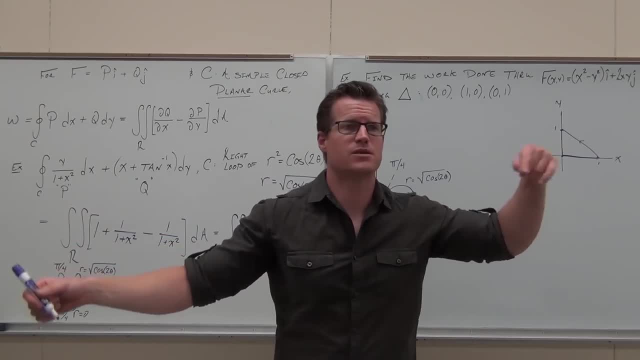 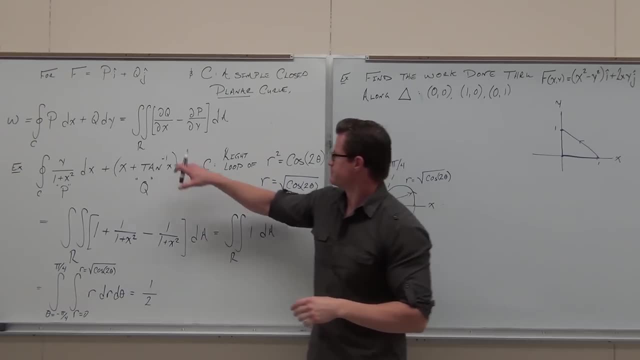 stem will give us is the work done of along that simple, closed curve that contains this region, by looking at the double integral of that region, of the this thing from your vector field. That's the whole idea. Is it making sense to you? I don't want to bore you to death. 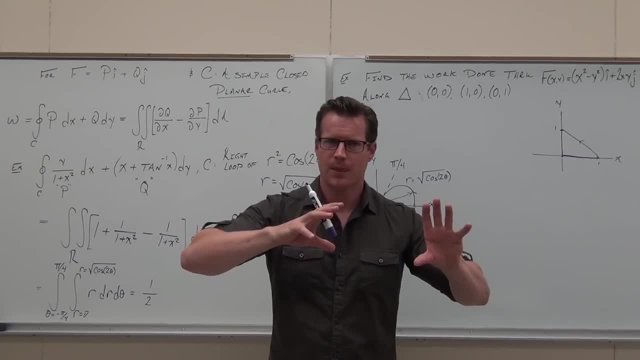 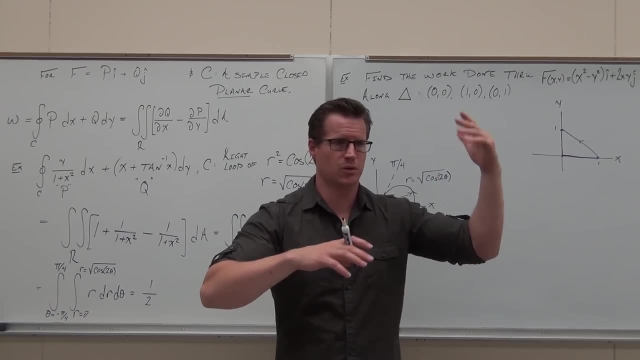 but I want you to see the connection about how the last three sections you're finding the same thing. It's just you have different scenarios. Number one: universal, non-conservative. add them up, Just do an integral, non-integral. 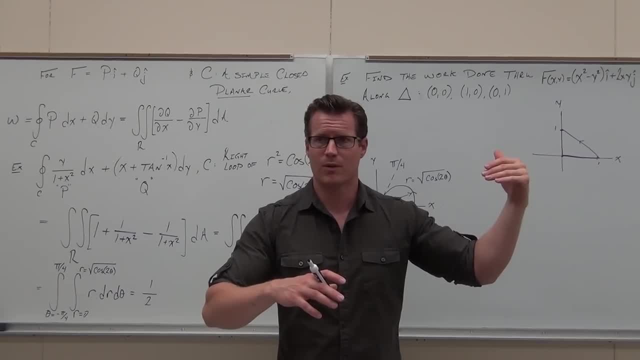 for every single different segment. It just sucks, It's hard. Then you go: okay, what about conservative? We have a very special case for conservative. It's pretty cool, It's pretty easy. You just do your anti-derivatives. 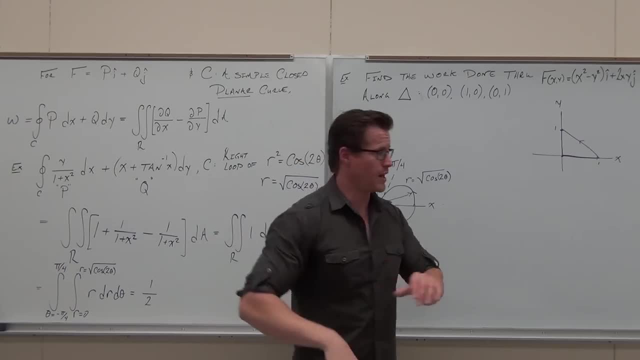 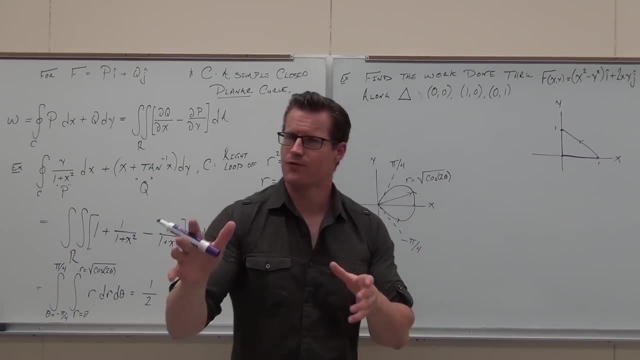 Done, Plug numbers in Now and it's independent path. You recall that Now it's: hey, let's suppose you're back to non-conservative, but you've got a simple closed curve, Man Green's theorem. So right now I need you to verify for me. 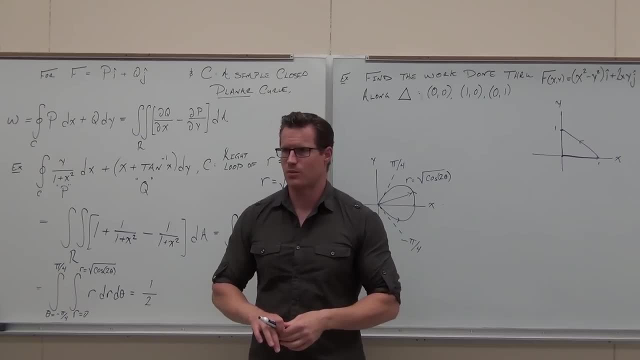 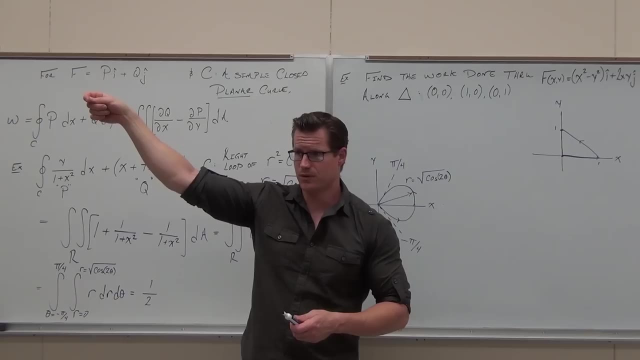 if this was on a test or something, you would recognize Green's theorem right here. Show of hands if you do It's work done. Is it a simple closed curve And do you get a vector field, Green's theorem Done? Set up Green's theorem right now, would you? 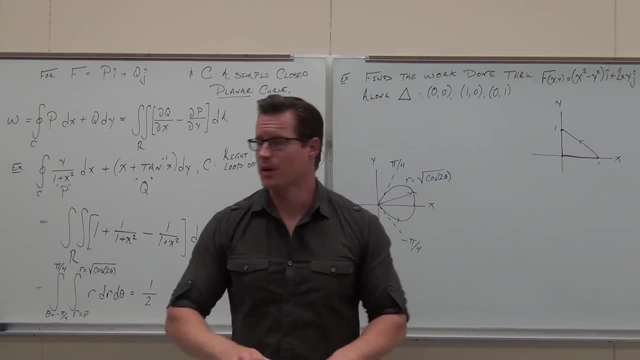 I want you to look at this. I want you to label P, I want you to label Q And I want you to set up Green's theorem. Do not skip down to this step. Show me this step and simplify, if you can. 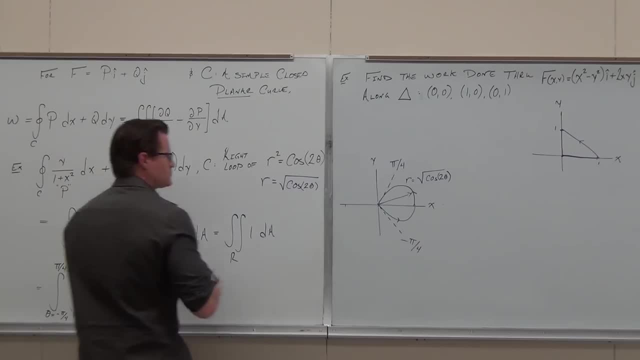 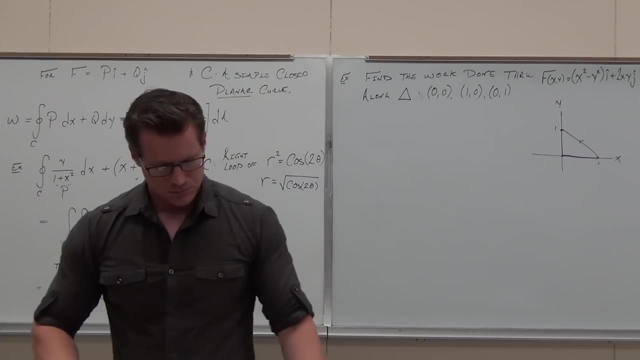 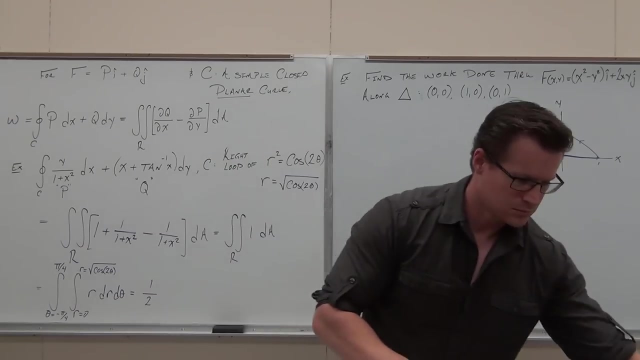 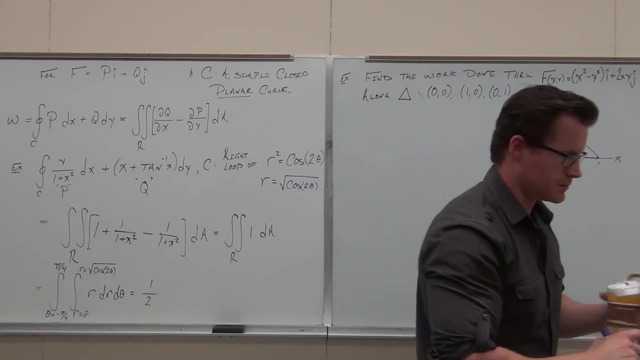 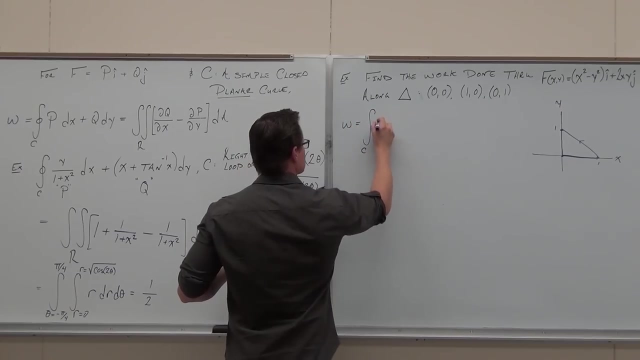 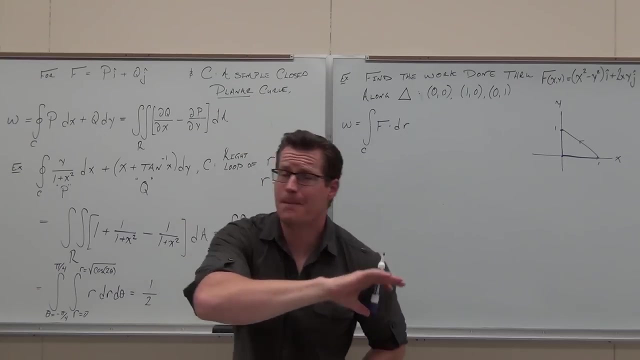 I want to see that That right. there is just basic work done through a vector field along a curve. That's what a line integral is. Does that make sense to you? Then we go. well, now let's look at our curve. 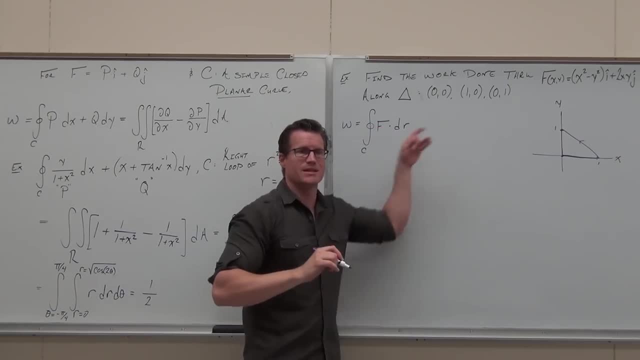 If our curve does this, which is what it does now. Green's theorem. you guys see the difference. Look you ready Ready. Green's theorem No No Two sections ago. Non-conservative vector fields. add up the segments. 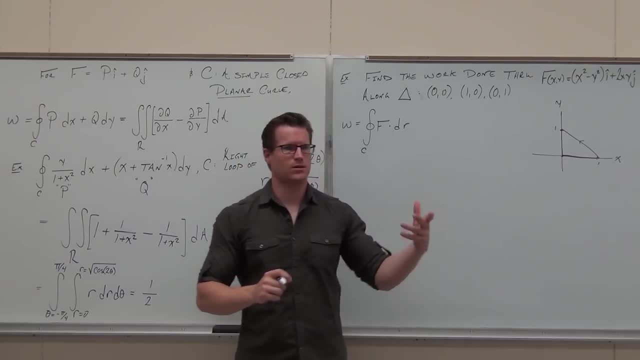 Green's theorem: Yes, Simple, closed curve. And since we have one, that's our setup. Now I do want to show you- I wouldn't do it this way, I'd do the shortcut, but I'm going to show you the. 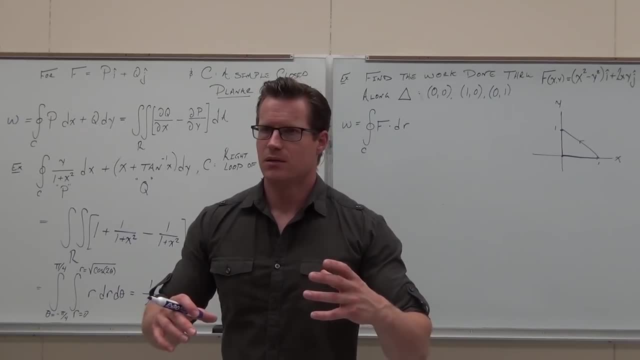 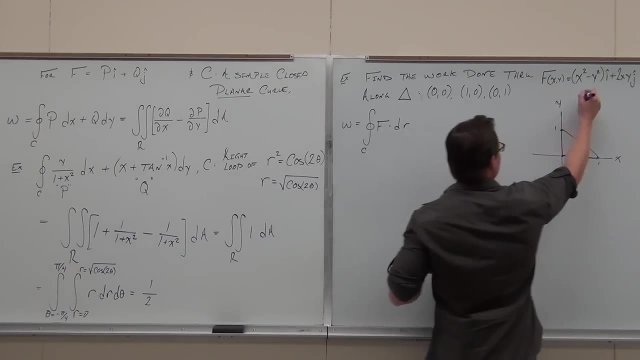 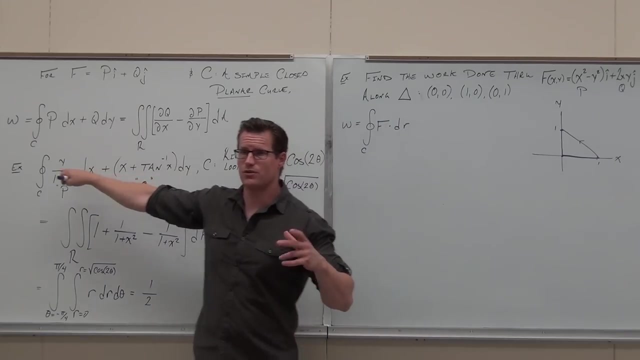 like where this all comes from, and then I'll show you the shortcut. Does that make sense? Maybe I'll show you the shortcut first. Can you identify what P is from your vector field? That means that's Q, yeah. So hey look, if this always gives you work done over simple. 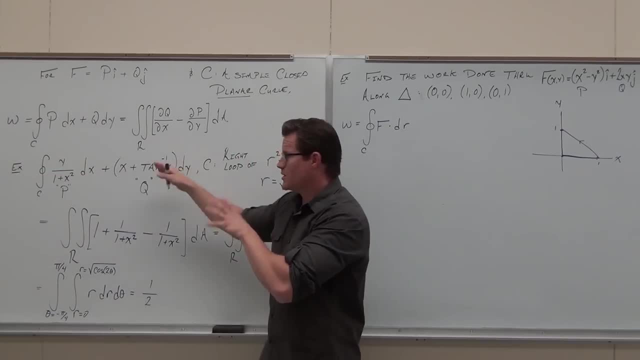 just work done in general, and you know your P and you know your Q. you can jump right to that. So, even though this looks a little different from what we're doing, we will be getting this from this thing And all you got to do is write P. 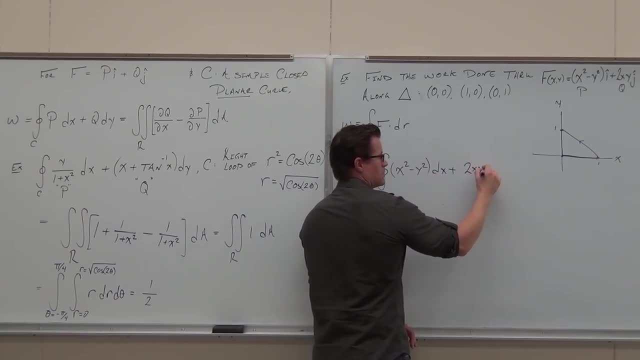 dx, plus, and then you're going to get this, So you're going to get this, So you're going to get this, So you're going to get this P plus Q, dy, and that's going to be exactly the same thing. 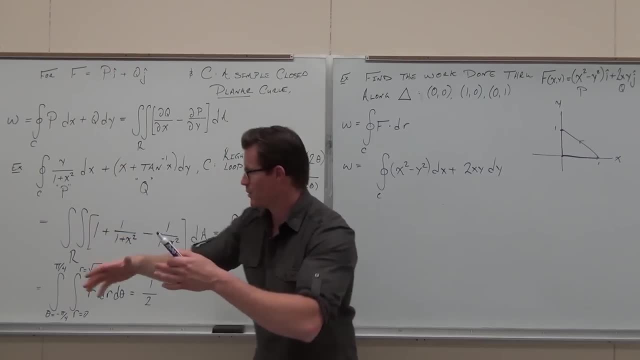 So if you see where it comes from- that's what I mean- when we got the vector field from this thing, we should be able to get this thing from the vector field. So if you have P and Q, you can literally go back and forth. 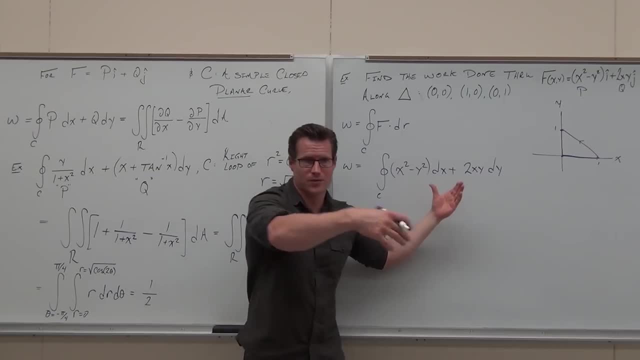 between a vector field and the work done on over that vector, through that vector field, along that planar curve. Now, if you want to see the math behind it, here's the math behind it. The math behind it says: well, what is F? 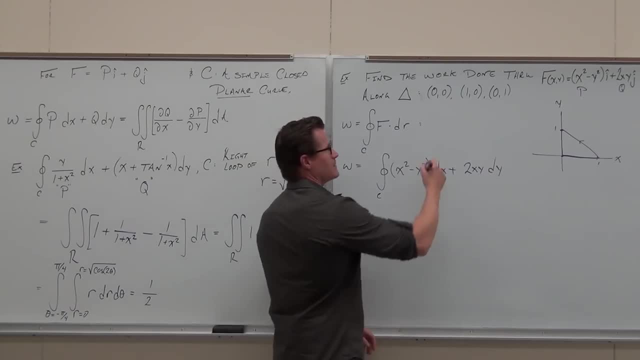 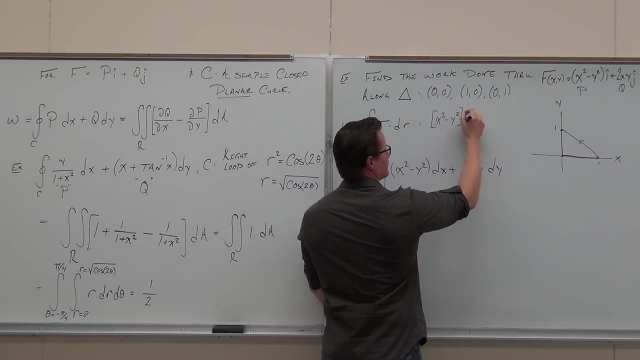 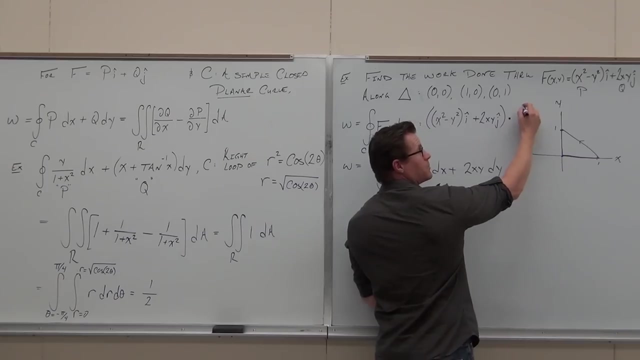 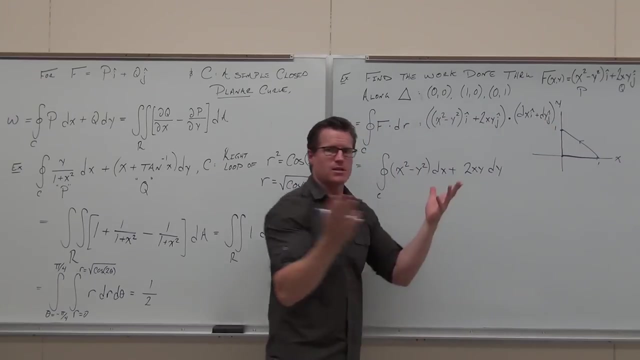 F dot dr. Well, F dot dr is F dot dr. is simply this dotted with this? Hey, that's F, that's dr. do you see how, when you do a dot product, you get this here plus this here. It's the same thing. 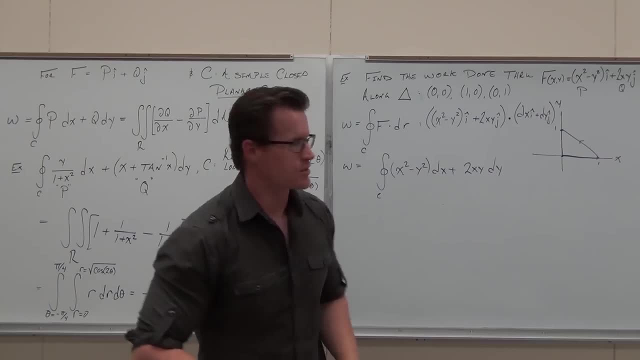 You have to get the same thing. And just so we can shortcut it, because if you don't want to do a dot product, you go: hey, put P with dx, put Q with dr. you have a line in your rule, right then? and there, 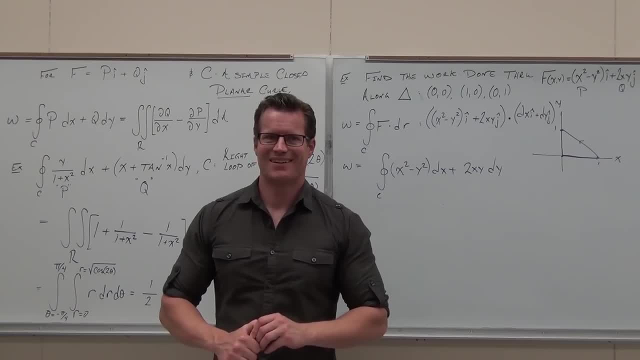 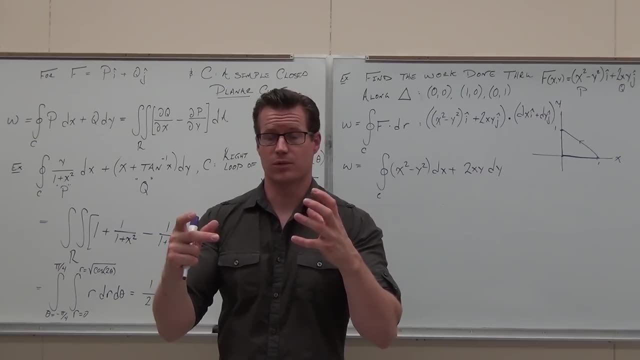 You still okay with that one, You having fun yet? Yes, Interesting, Is it starting? Am I starting to wrap this up for you? Because the next section is going, the next. we're doing it four at once, but the next four sections are going. 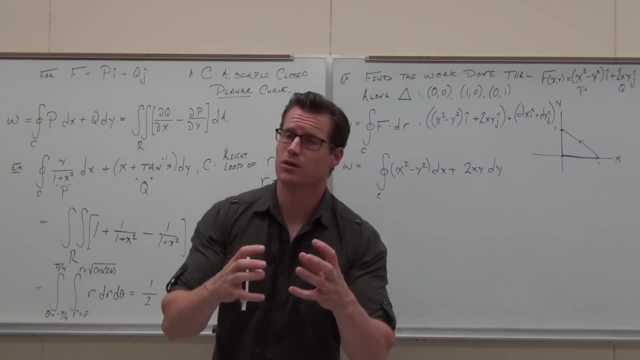 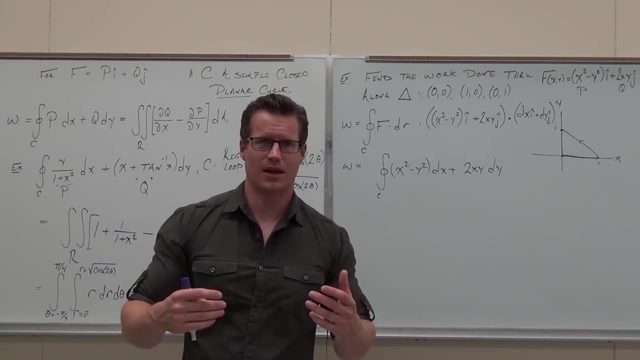 to put everything together for this whole chapter. I need to make sure you're good at this stuff before we get there. Do you feel competent with Green's theorem right now? I see a lot of head nods, but I don't see a lot of. 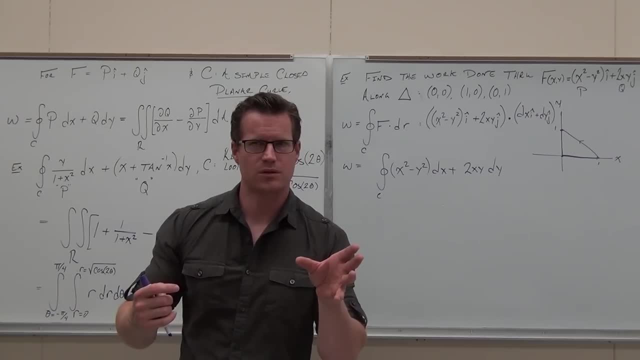 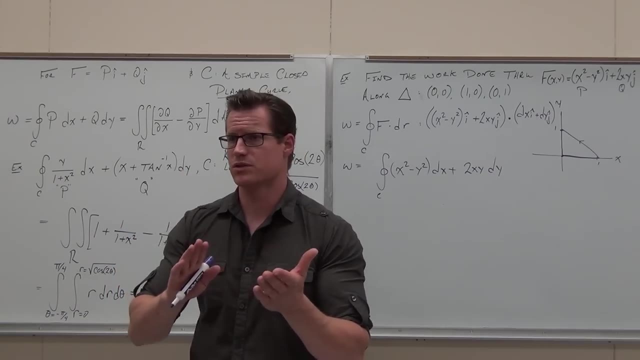 I don't hear a lot of words. Do you know when Green's theorem works? Yes, Over vector fields, along what Simple, closed, Simple, closed, Simple, closed planar curves. That's what I need you to know, If you have one Green's theorem. 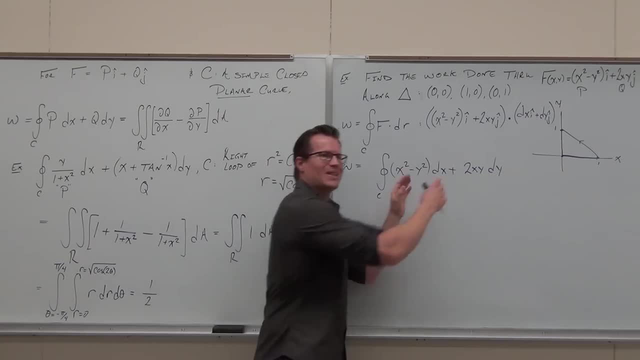 So did you make that for at least Now? because we've got a line integral over a simple closed curve- boom, let's go ahead. let's set up Green's theorem. If you haven't done that, I want you to do Green's theorem right now. 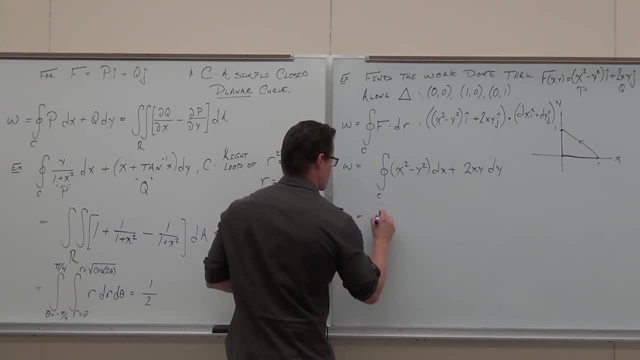 Did you? I don't want you to do anything with the region, Not right at the start. I just want you to leave it there and then consider your region. okay, We would have. hey, the same P, the same Q. 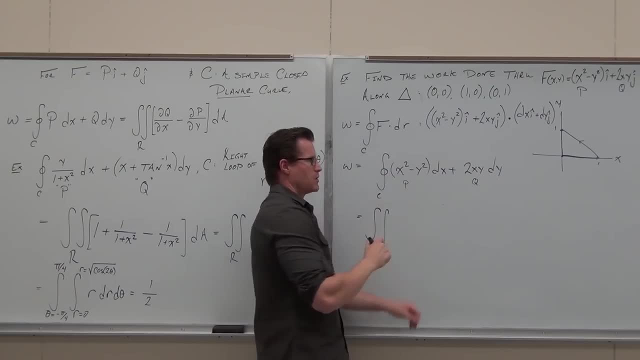 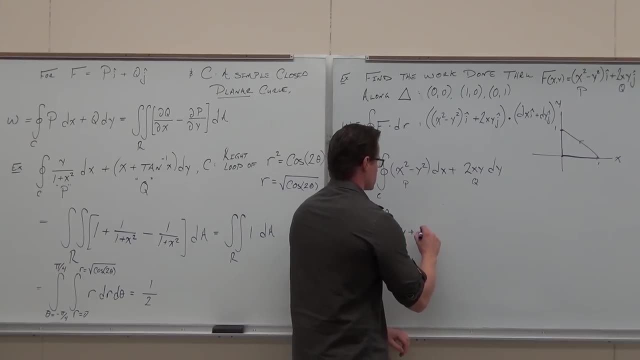 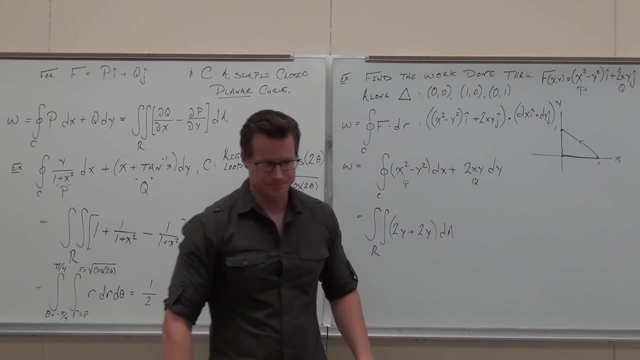 It literally has to be the same. Just take the partial derivative of Q with respect to X. Subtract the partial derivative of P with respect to Y. DA, Head nod if you're okay with that one. Now, that's what Green's theorem says. 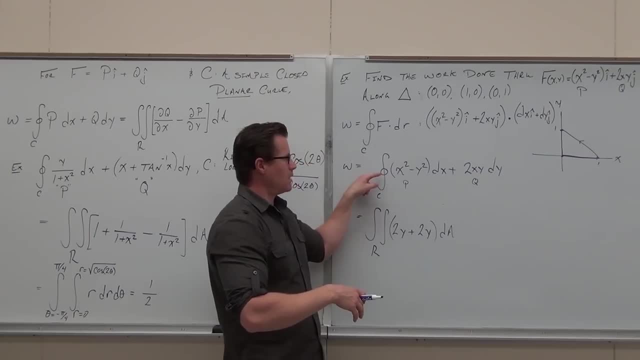 It says: hey, the work done Along this or, sorry, through that vector field, along this simple closed curve, is equal to the double integral of whatever you get out of this, whatever this thing is over the region that that curve encompasses, encloses. 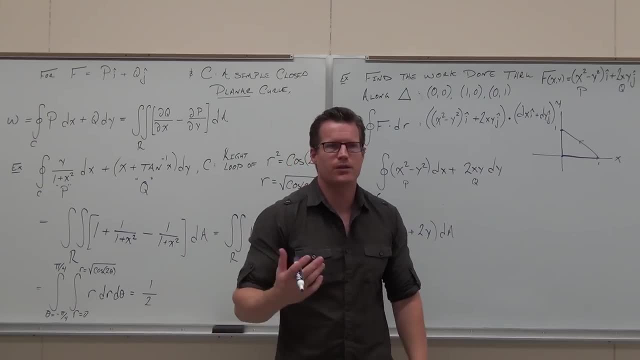 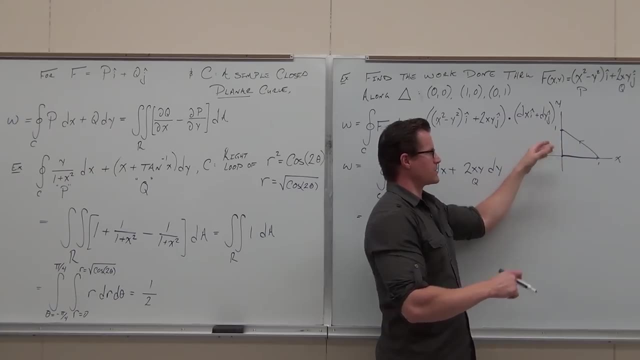 That's what it says. All we have to do is define, just define the region In this case, since we're going from 1 to 1, or 0, 1 to 1, 0,. this line oops. 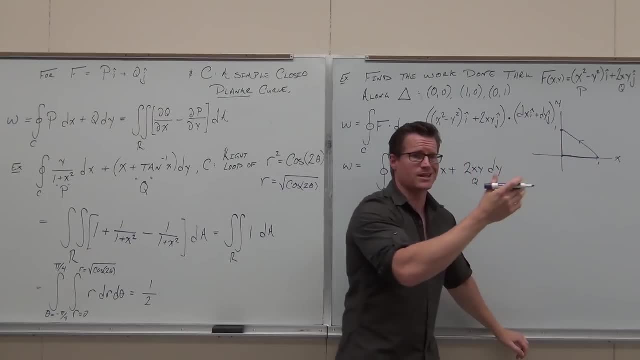 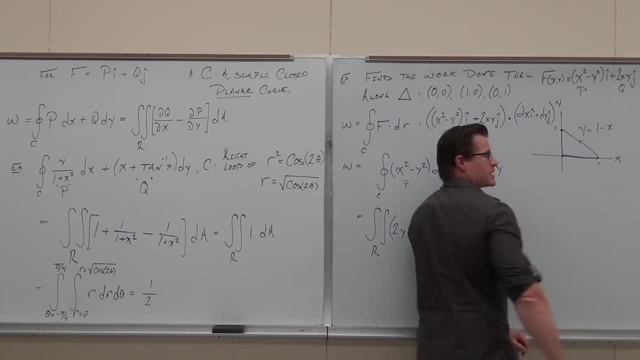 this line right here could be defined in a couple different ways, and it really doesn't matter. It's a pretty basic region. Me personally, I like going DY first. I define this as 1 minus X. Y equals 1 minus X. 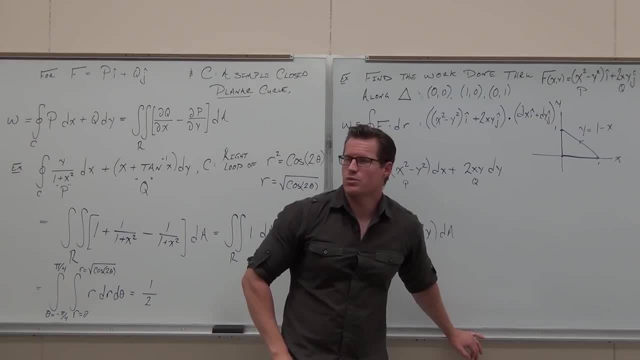 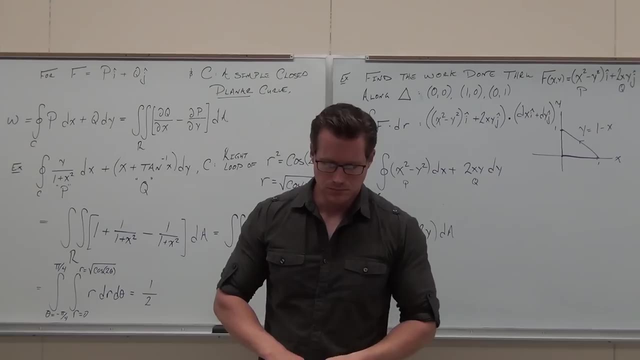 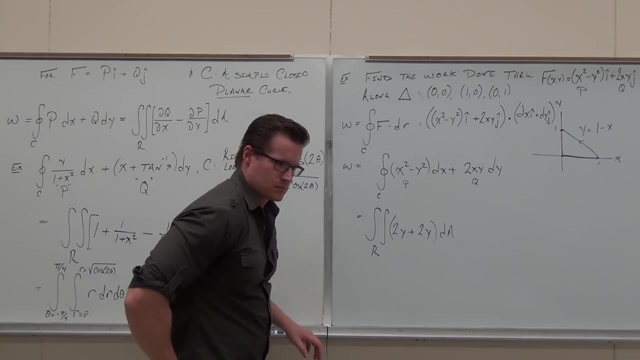 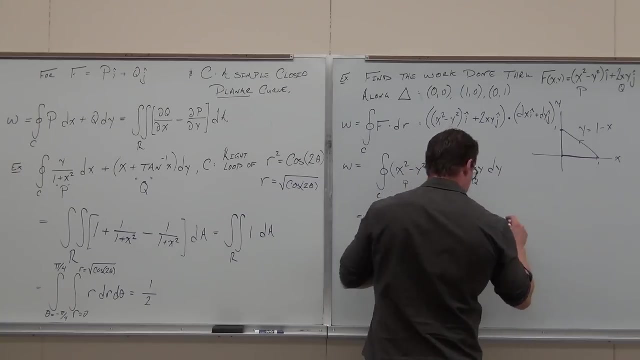 Head nod if you're okay with that one. So if I define this as Y equals, would I be going DY first or would I be going DX first? Set it up. I want you to set it up. Tell me quickly what's Y going from and going to, please. 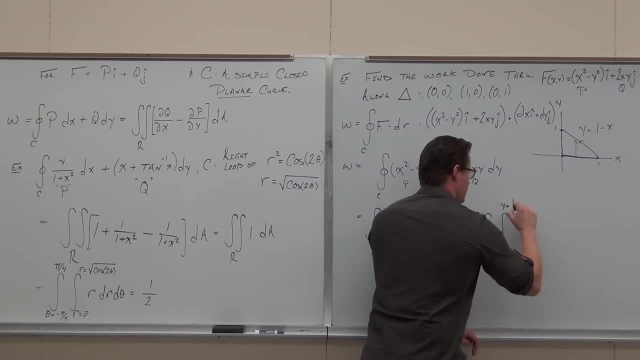 0 to 1 minus X. Beautiful, Since I'm going DY first. oh sorry, from Y equals to Y equals, it's Y, simple, I need DY. And then X goes from 0 to 1, beautiful, DX. 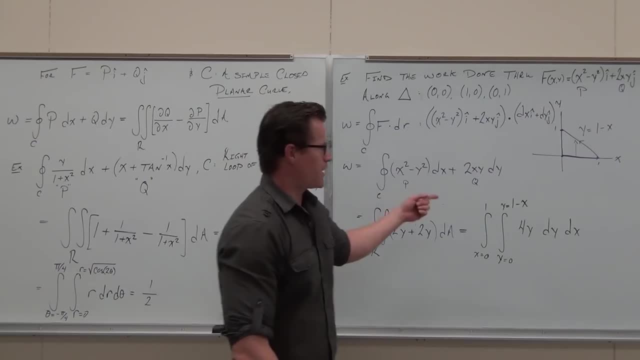 Could you have switched it around? Absolutely It doesn't even matter If you want to solve that for X. that way you avoid integrating with respect to Y. you could do that as well. Does it matter? Not really, Maybe for some distribution you might have done that one. 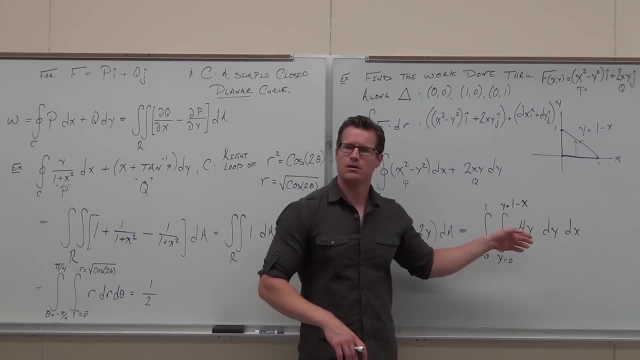 Me personally, I didn't. Would you know what to do after this? What would you do? Yeah, I might have. actually, if I had thought about this a little bit more, I might have solved, done DX first, Just so that I avoid dealing with that Y, first step. 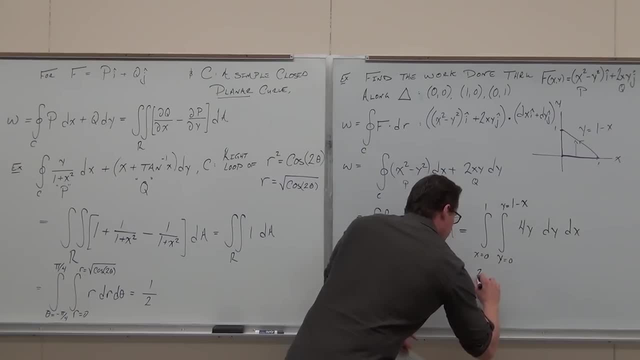 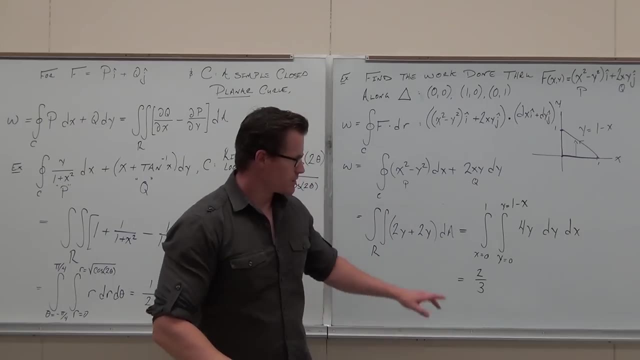 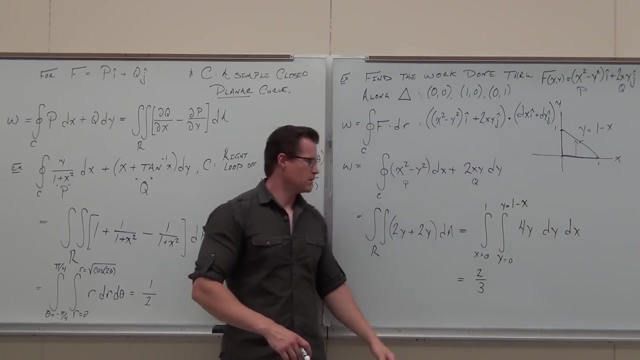 But either way, any way you want to go, this needs to give you 2 thirds. Quick question before we end this: Is this the area of that triangle? No, Why not? If the interval is, if the interval is, if it's not 1.. 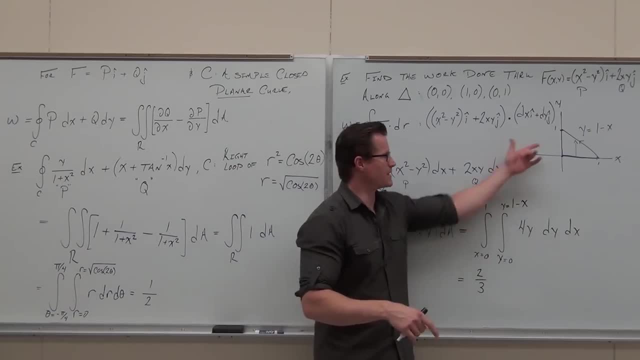 If it's not 1.. If this had been 1, that would give us the area. Obviously, that triangle would have an area of 2 thirds. The base times height divided by 2, and I'm going to give you 2 thirds. 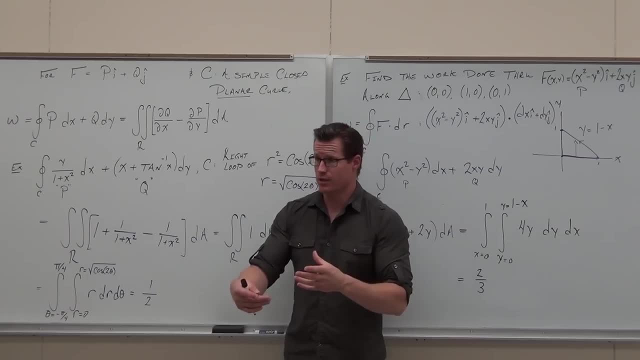 It's going to give you 1 half, So it's not giving us the area here. What it's giving us in this context is the work done along that simple, closed curve through that vector field. That is exactly what I want you to know, and that's how Green's theorem works. 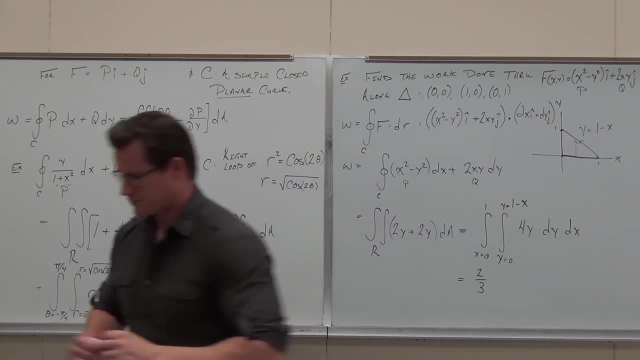